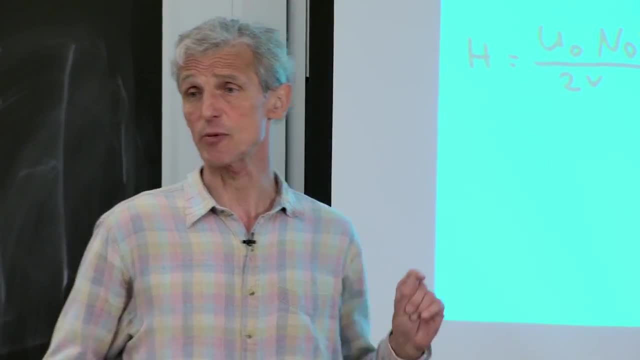 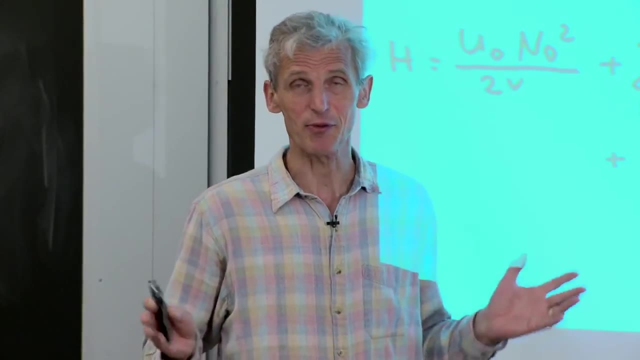 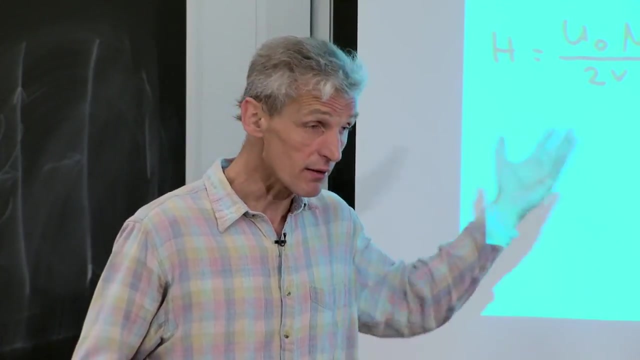 And the superfluid properties are determined by the interactions between the atoms. So the purpose of those lectures is number one: to acquaint you with important phenomena in cold gases: superfluidity. superfluidity in lattices, superfluidity in 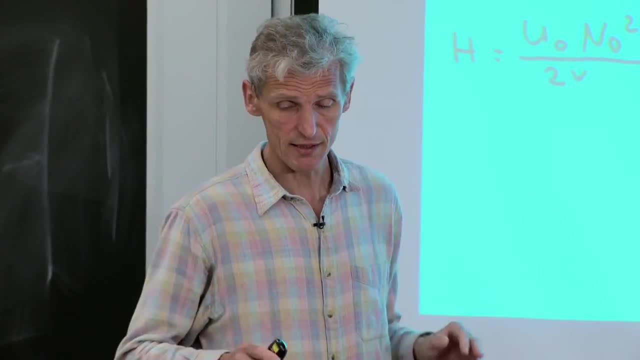 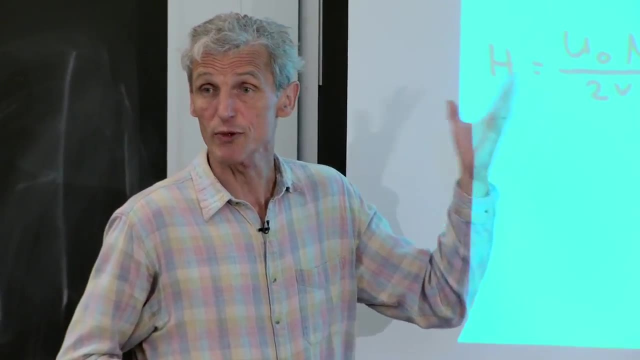 ah ah, Just in free gas, in a normal gas, without lattice and superfluidity of fermions. But at the same time I also want to have sort of a theme for you how we deal with interactions And that deal and that kind of theme. 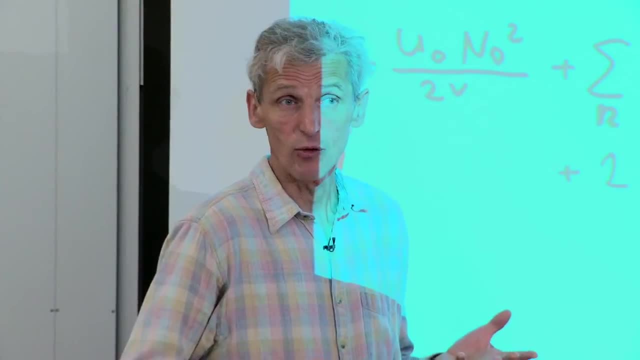 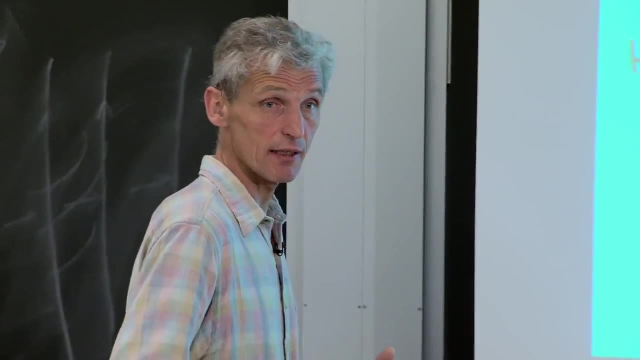 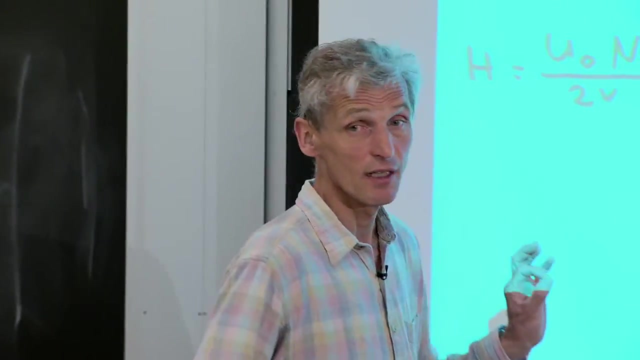 is that how theoretically we reduce unsolvable Hamiltonians to Hamiltonians which can be solved, And you will see that actually appearing in different situations with well, similarities, Similarities, but important differences. So, just to remind you, we started out with the interacting Bose gas in a homogeneous system. 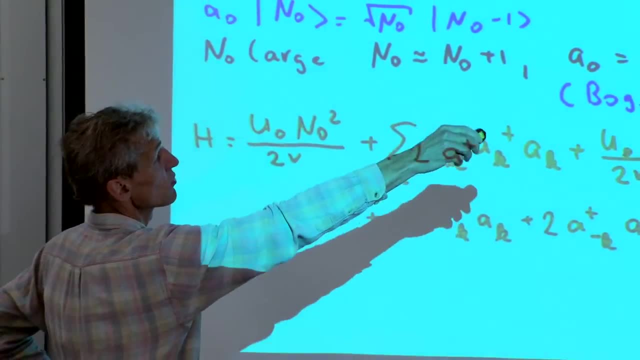 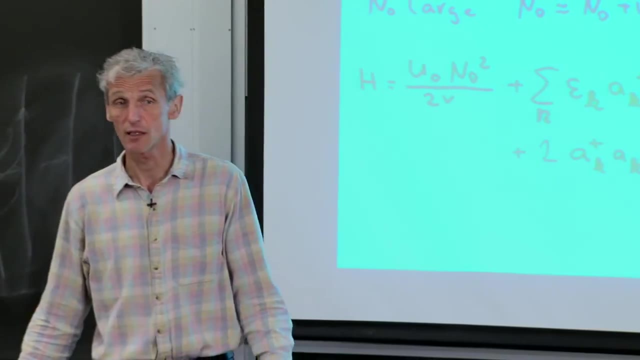 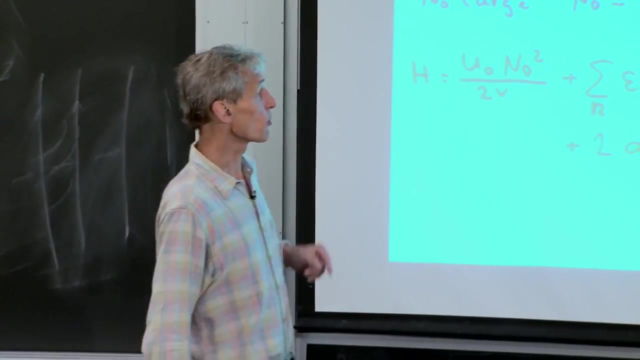 We have a very general way to describe scattering: Two particles with initial momenta disappear and two particles with momenta appear. This is a scattering event. Now this means we have products of four operators, which is very difficult to solve, And the Bougoulioubov approximation. 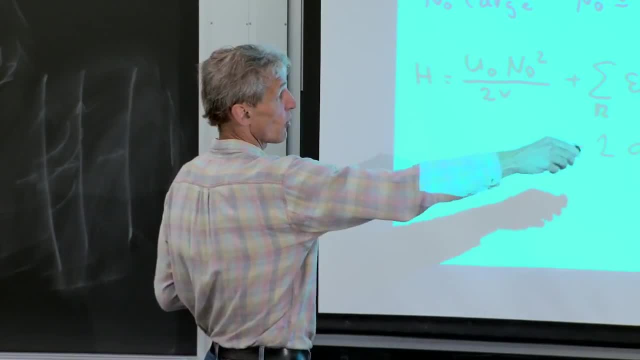 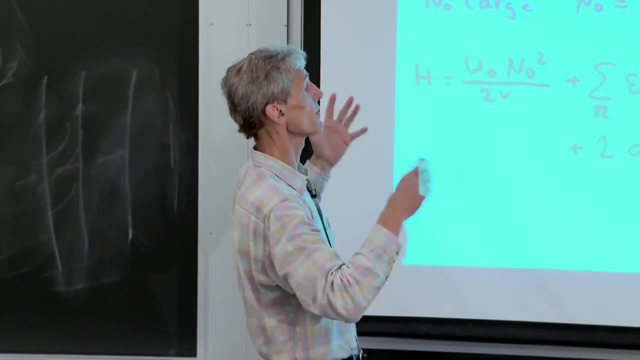 which we discussed on Monday, replaced on the basis, the operator for the condensate, for the zero momentum state, with a C number saying that well, n-odd, n-odd plus 1 is the same. a little bit waving your hands. 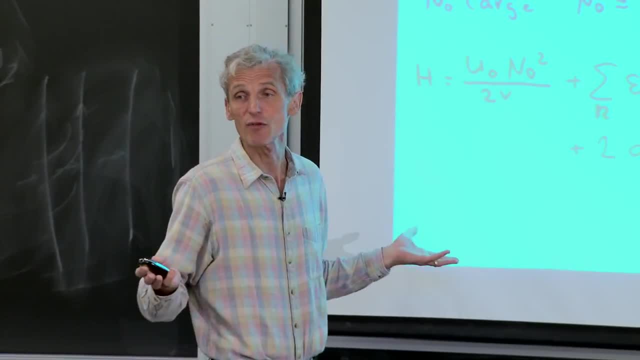 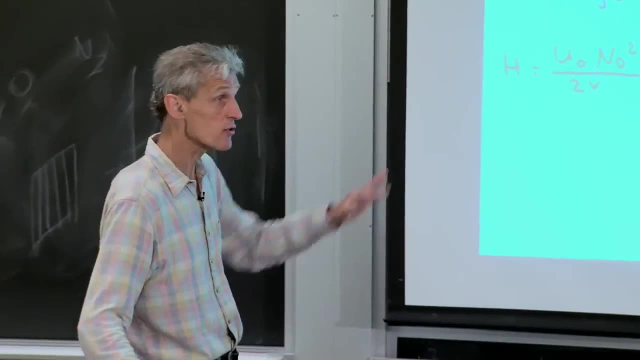 But it's also, you can say, the macroscopic limit. When we have a photon field with many, many photons, we can use a C number in our Hamiltonian to describe the electric field. So that's the same spirit. So maybe- yeah, I should emphasize it. 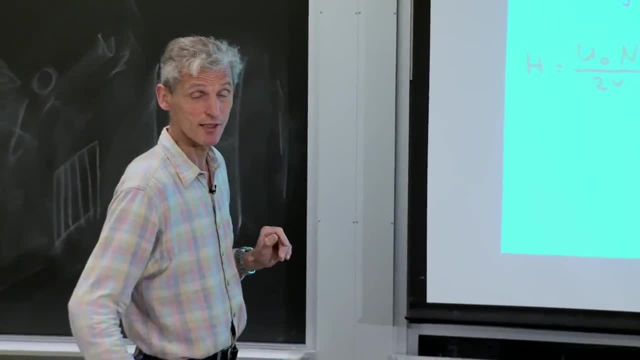 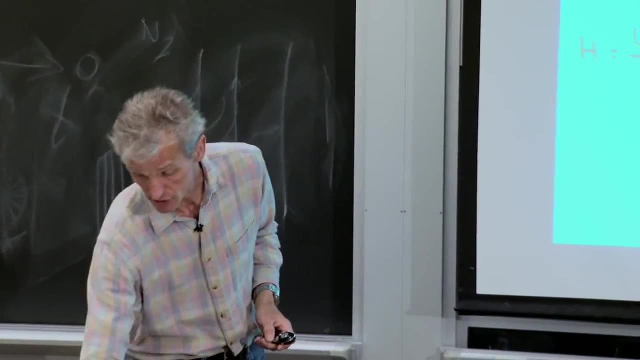 This is for atoms what you're used to do with photons for your whole life. OK, with that, we have transformed the Hamiltonian into a bilinear expression, And so the moment you have a bilinear expression, you do a Bougoulioubov transformation. 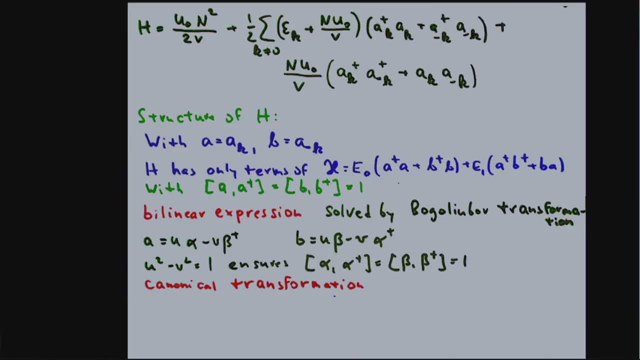 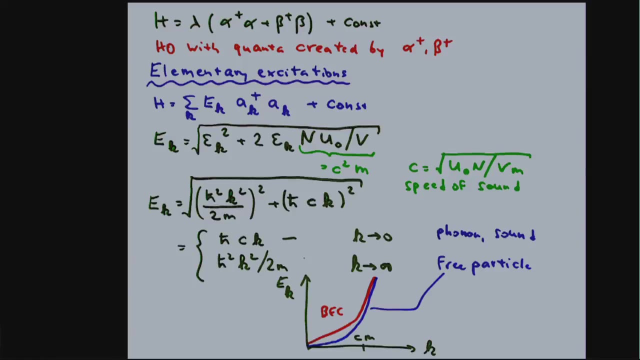 You simply diagonalize it by finding a new set of operators where the cross term between a and b or between a of k and a of minus k disappear, And then you have solved it, And this is what we arrived at at the end of the last lecture. 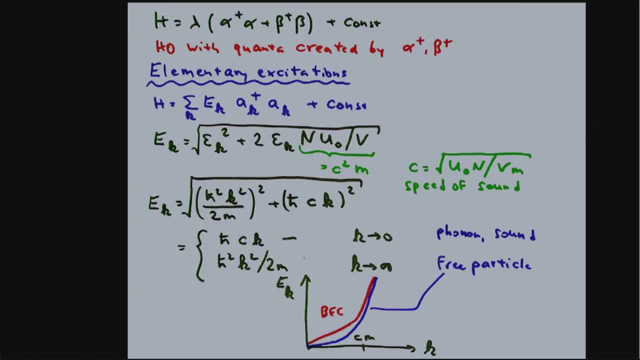 We have with those approximations. we have diagonalized the Hamiltonian. Our Hamiltonian is now, you can say, a harmonic oscillator Hamiltonian. Or you can say it has become a gas of non-interacting quasi particles. Each of those operators creates a quasi particle. 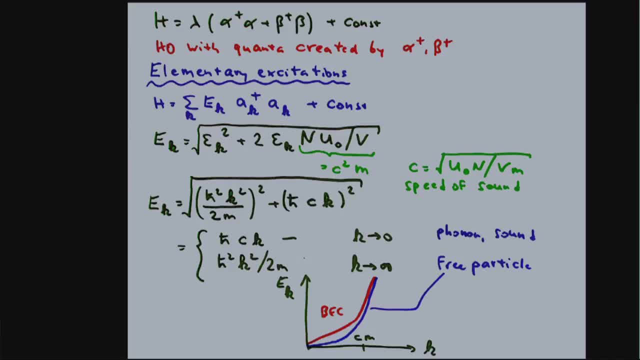 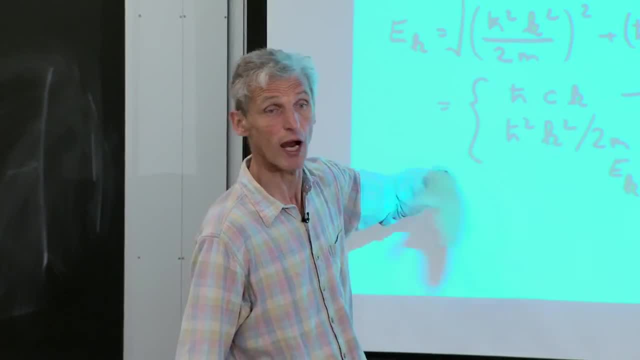 And the quasi particle energy is e of k, And I explained to you that, as expected, the quasi particle energy is a k. OK, OK, It's simply particles with momentum h by k for high momenta, because a high excitation in a Bose. 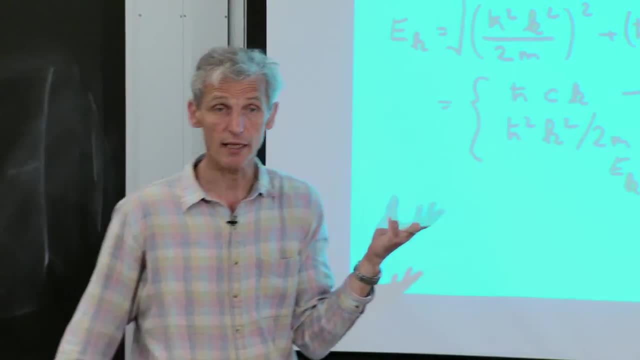 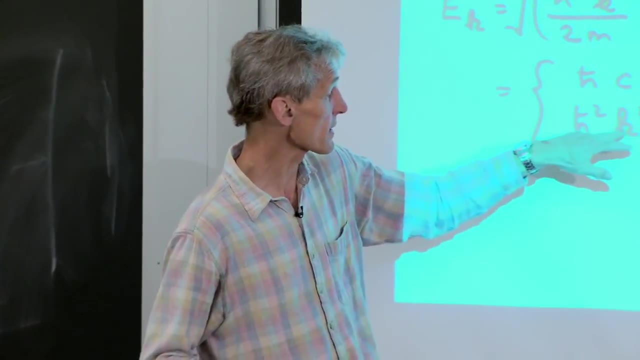 condensate is a free particle, But a low-lying excitation is affected in a major way by all these interactions with a Bose-Einstein condensate And that turns the quadratic dispersion relation into a linear one, Or you can say that turns a free particle. 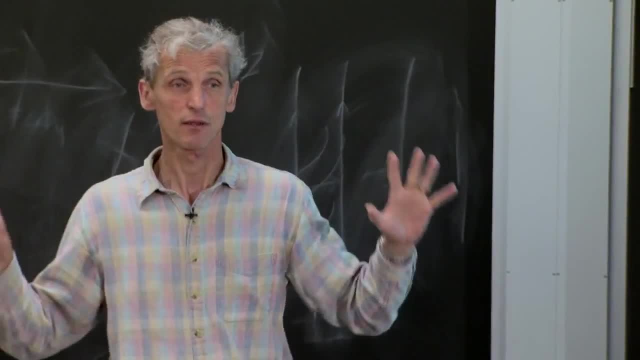 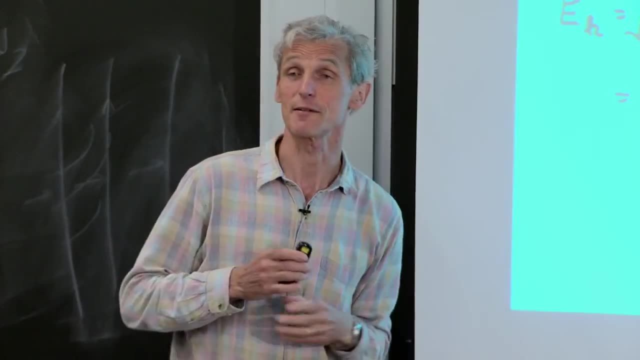 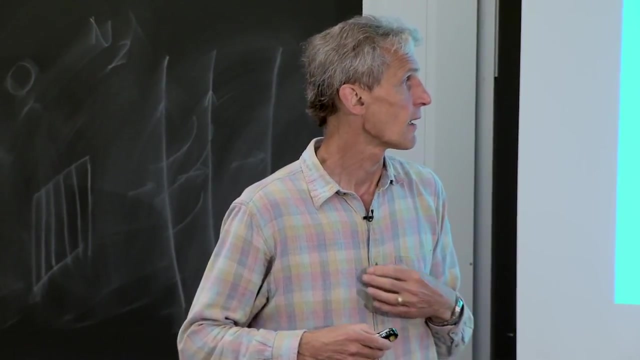 into a phonon or a sound wave. So that's my review of last class. Are there any questions? before we go further, Colleen, So does this require low density and weak interactions, or one or the other? We come a little bit later to that. 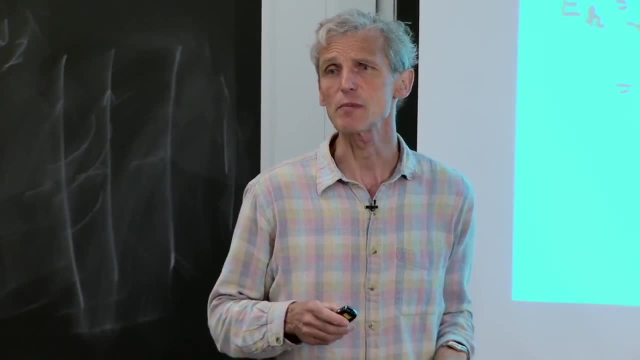 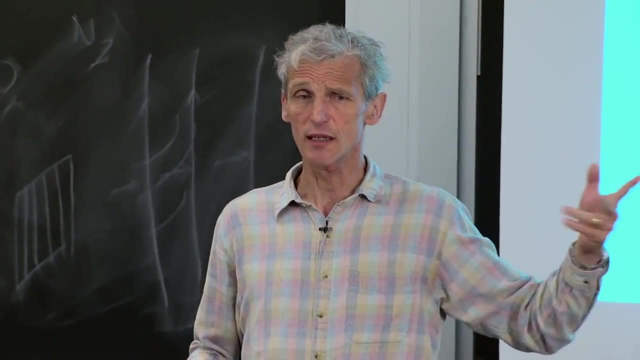 But in the end there is a small parameter. The small parameter will be in a cube. the gas parameter In the density, a cube, the scattering lengths, It's often, it's usually the dimensionless combination of the two which decides whether we are in the weakly. 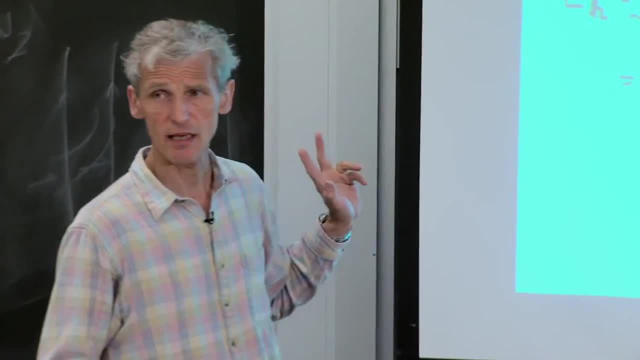 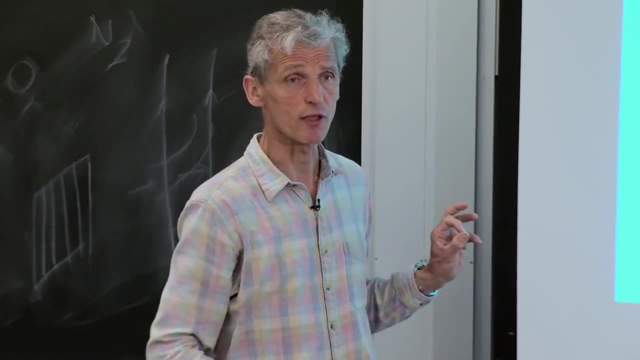 or strongly The acting limit. There is another assumption which we have made here, But it's related to that, as you will see in a few moments, that most of the atoms are in the condensate We assumed. N0 is peak. 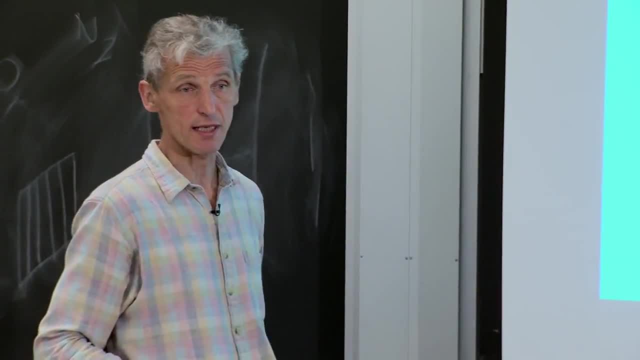 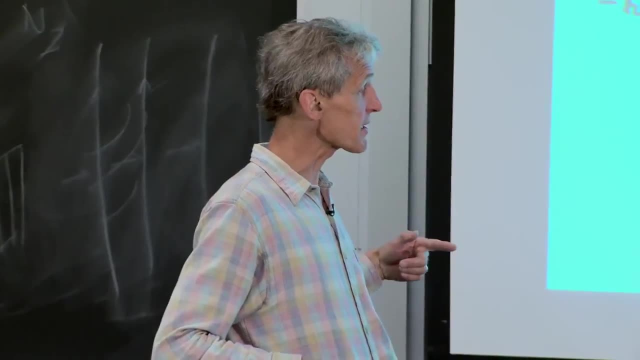 The condensate depletion. the number of atoms who are not in the condensate- at t equals 0, is small. But let me just first show you- I want to mix in theory and experiment- how sound can be observed. I should actually say this experiment. 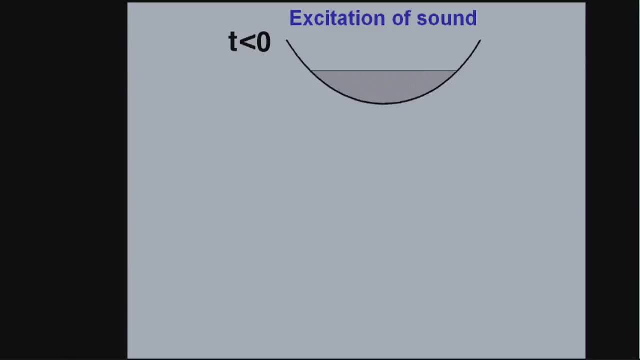 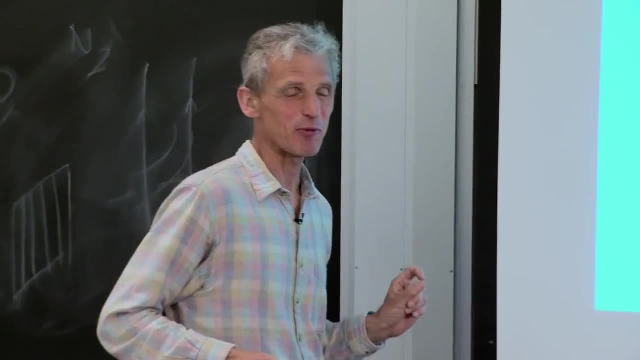 is sort of dear to my heart, Because at some point it clicked to me how the new world of atomic physics connects with condensed matter physics. Soon after we had realized Bose-Einstein condensates, a famous condensed matter theorist said: hey, Wolfgang. 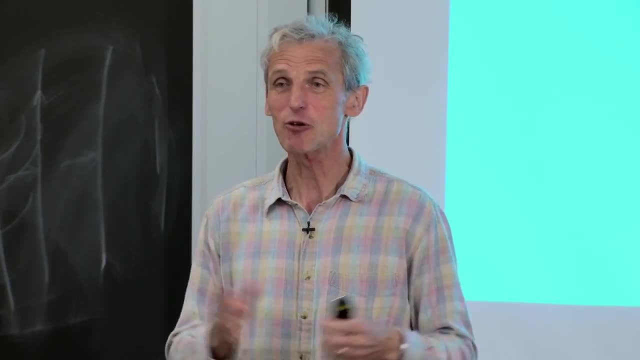 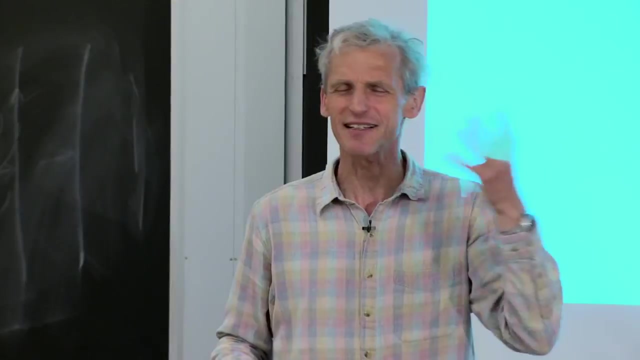 you should now observe sound. Sound is important, Yeah, OK, But how do you observe sound? You know, use a piezo and just kick the system and create a sound wave. And I said, oh gosh, this guy doesn't know that if we put 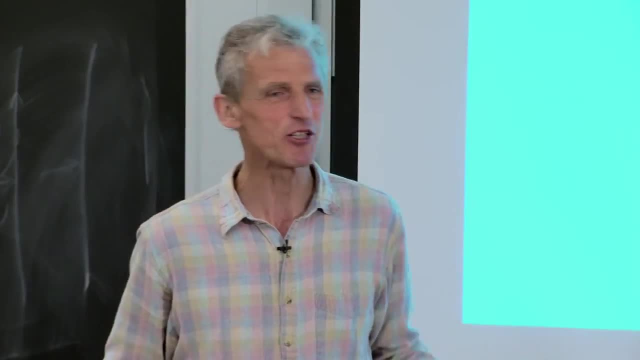 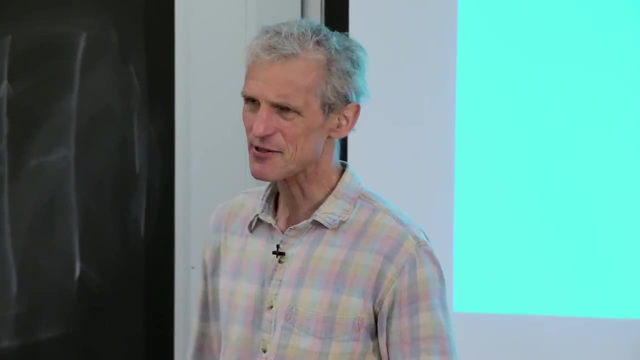 anything in contact with a quantum gas. it's a piezo. The gases will just stick to it. He has no idea what our system is. But then I said: wait a moment, We have to translate. He says: use a piezo. 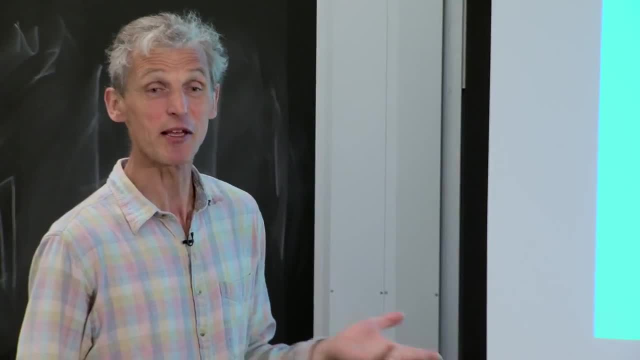 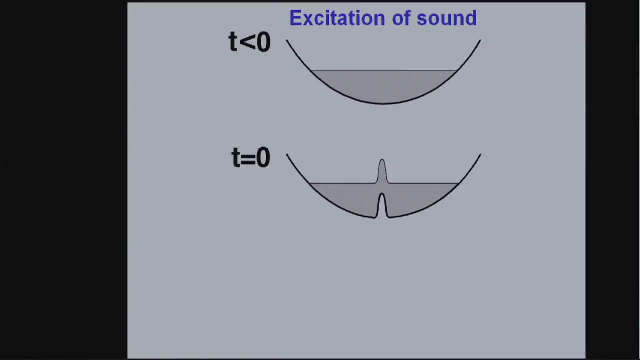 Well, I have to translate In atomic physics. how do we kick atoms With a laser beam? And in that moment I had the idea that we can take a Bose-Einstein condensate, suddenly switch on a blue-detuned repulsive laser. 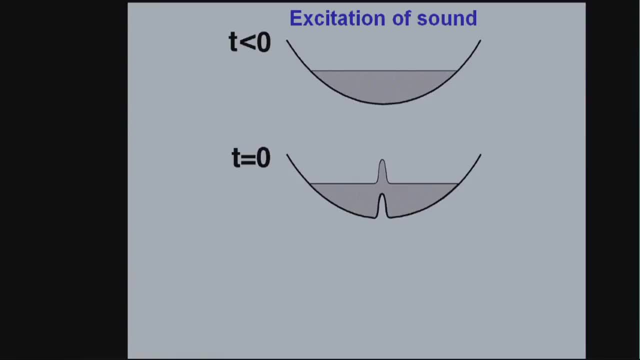 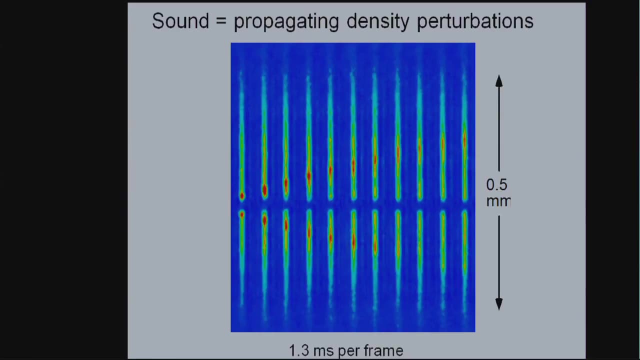 beam. This will do exactly as a piezo: create a density perturbation And then the density perturbation will propagate with the speed of sound. And that worked. That was just when Bose-Einstein condensations were very fresh, One of the first scientific experiments done. 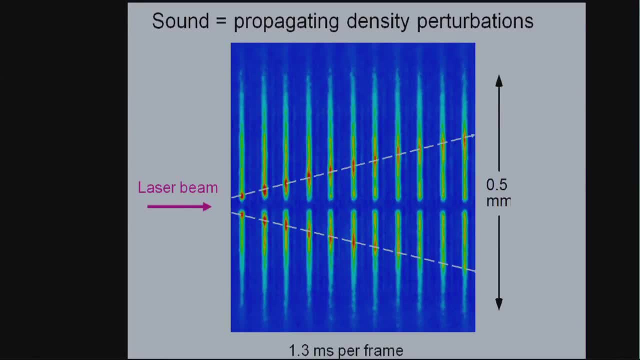 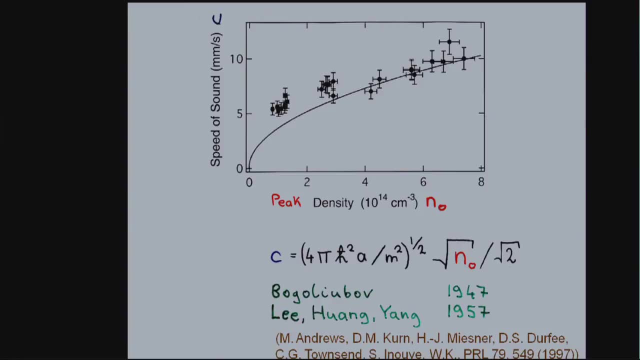 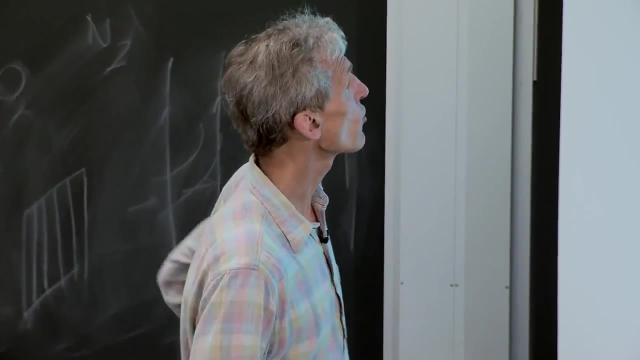 we switch on the laser And you see, color-coded in red, the density perturbation which propagates outward, And the slope of this line is the speed of sound, And here we determined the speed of sound as a function of density. So that's how phonons can, or at least how the speed. 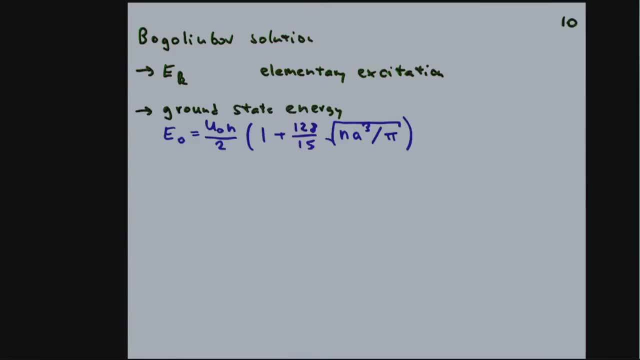 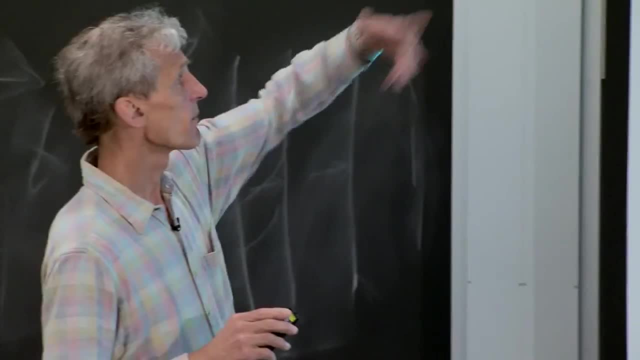 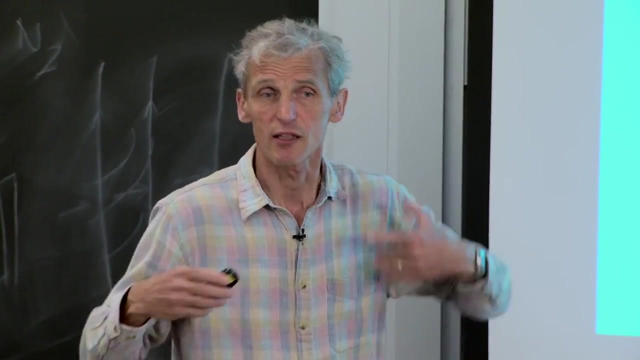 of sound and wave packets which propagate with the speed of sound can be prepared. I come back to phonons and collective excitations in a few moments, But let me first say, when we have diagonalized the Hamiltonian, we know everything we want to know. 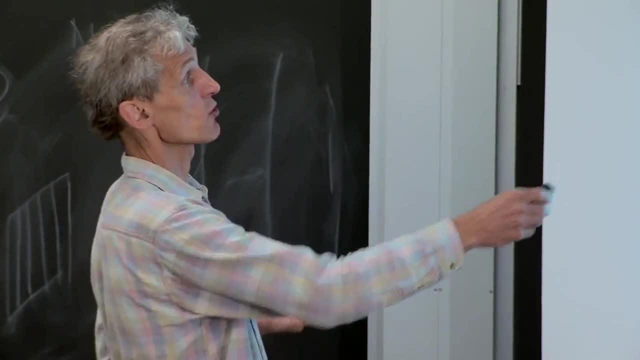 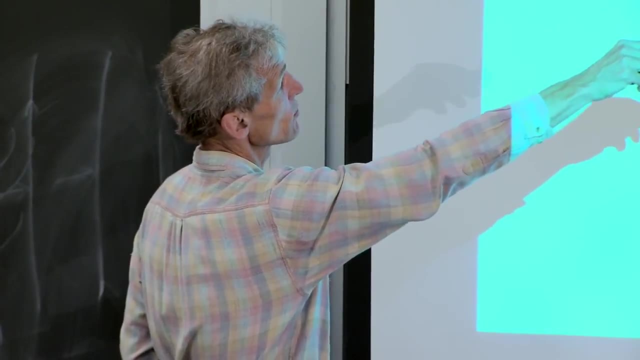 I just focused on the quasi-particle energies, But you also know the ground state energy And actually here, Colin, you see that the corrections to the ground state energy scale with any. So this is really the small parameter in the system. 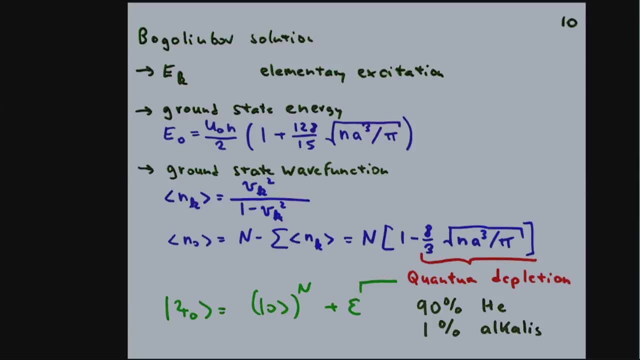 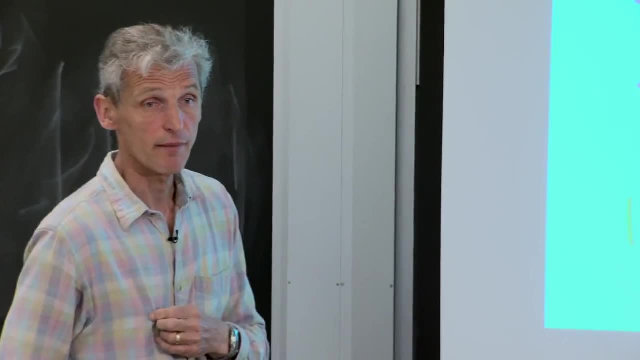 But we can also find out what is the ground state wave function, And let me use that to introduce an important concept to you called the quantum depletion. When you have two atoms in the condensate at zero momentum and you switch on the interactions, 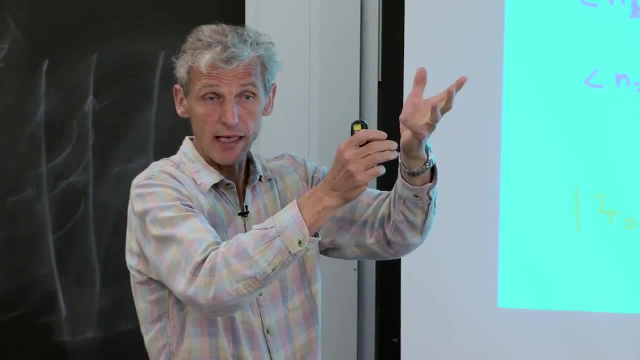 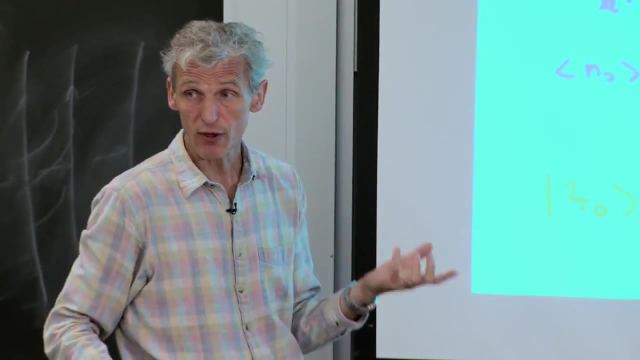 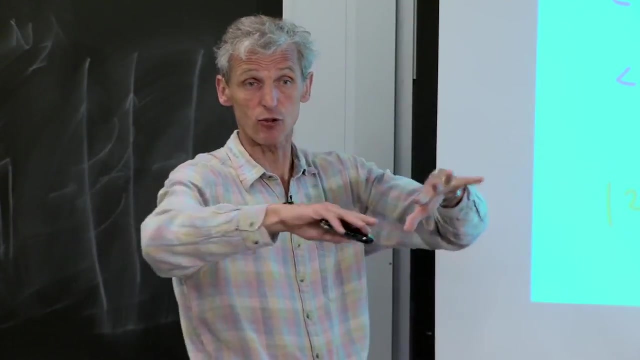 the atoms. the interaction, the delta function, interaction couples zero momentum state to higher momentum states. So therefore the effect of interactions is that the condensate is not just at zero momentum, It has some probability or some admixture of finite momentum states. 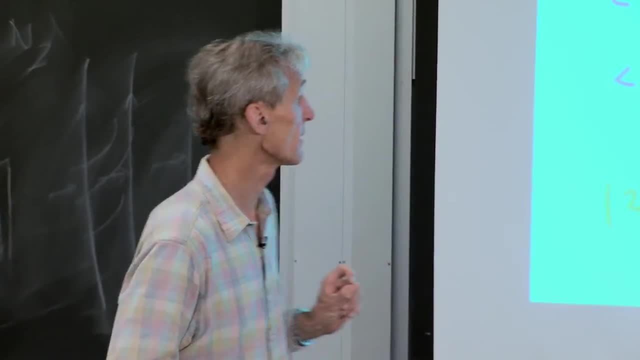 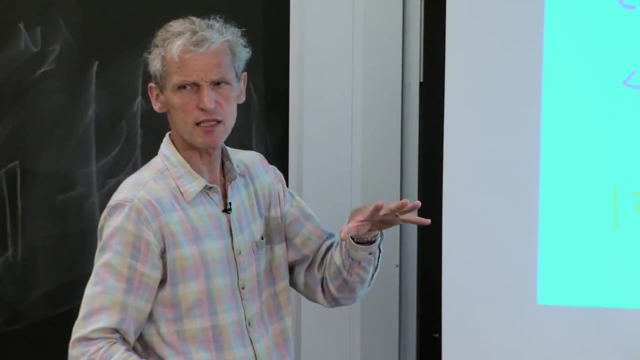 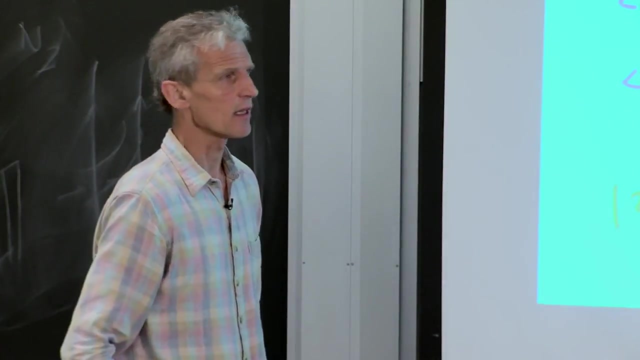 This is the ground state. This is how the Hamiltonian is diagonalized. So from the Bogoliubov approximation, where we introduce this v and u parameter to transfer from one set of Bose operators to another set of Bose operators, those coefficients give us the proper. 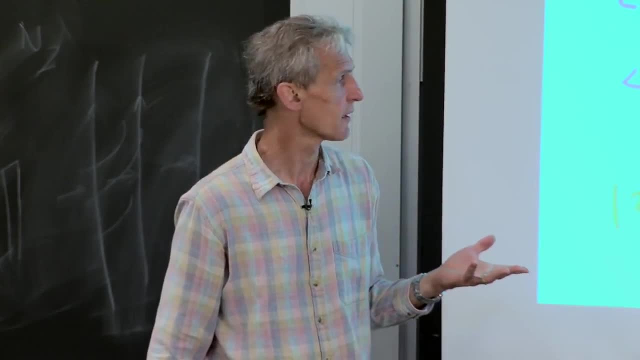 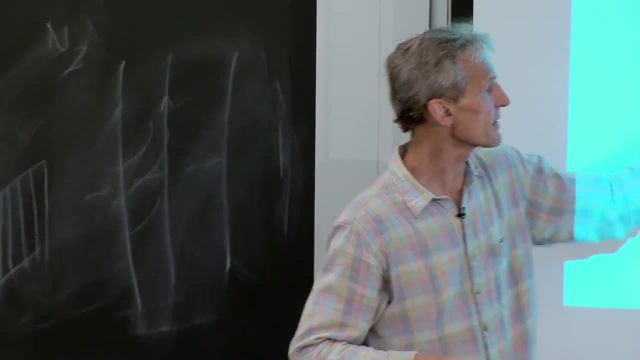 Population of those momentum states in the ground state of the condensate. So if I now ask: what is the condensate fraction? What is the number of atoms in the zero momentum states? It's all atoms, but those who have finite momentum. 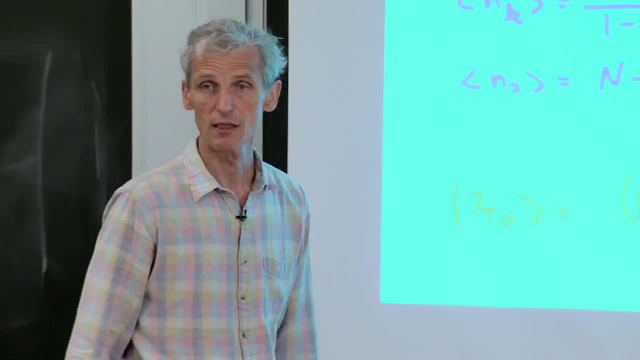 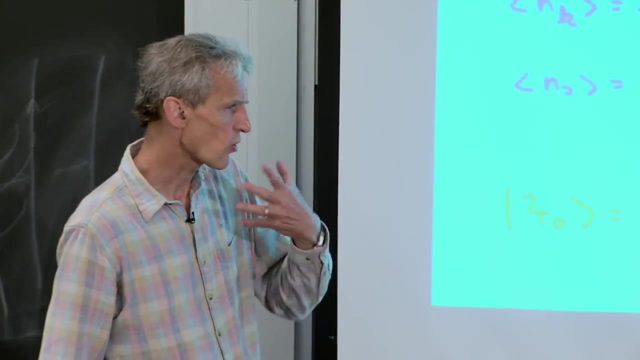 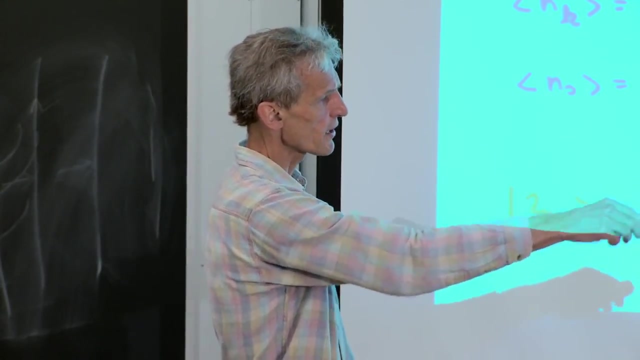 And we find again the small parameter na cubed. Now, this quantum depletion allows me now to make a difference, a distinction between the cold atomic gas condensates and superfluid helium-4.. In cold atomic gas, In cold atomic gas condensates, this correction is about 1%. 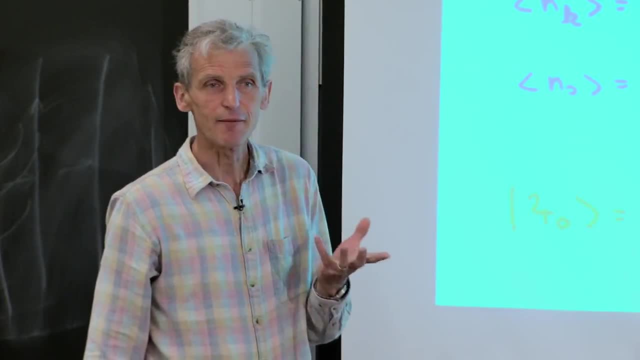 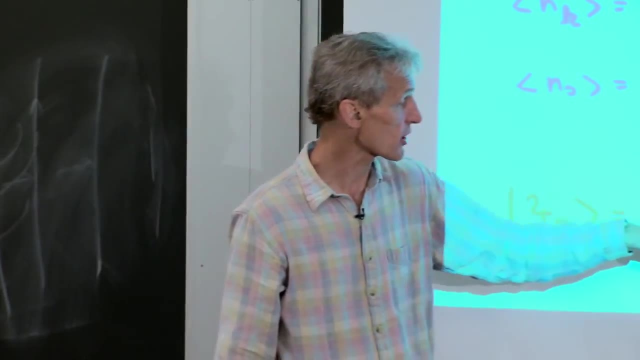 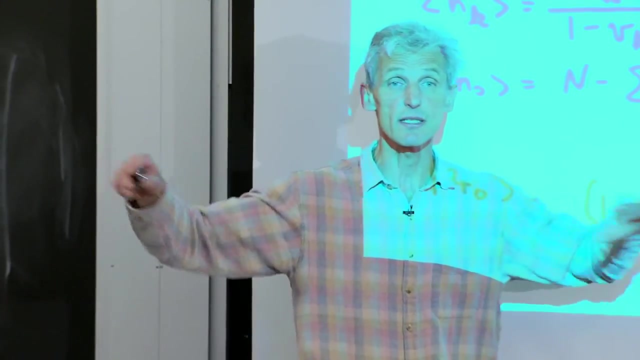 So therefore I can say with 99% probability or with 99% weight, the condensate, the many-body wave function of the condensate, is just a zero momentum state to the power n And this very complicated admixture of correlations. 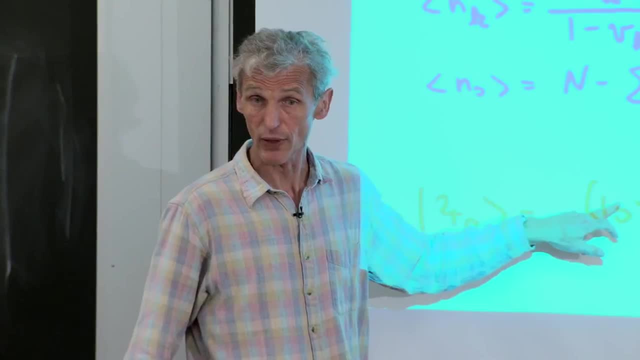 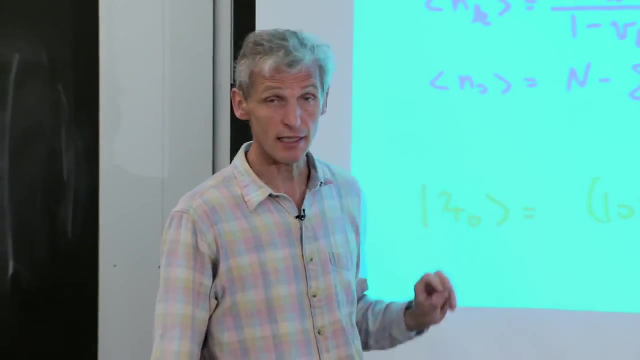 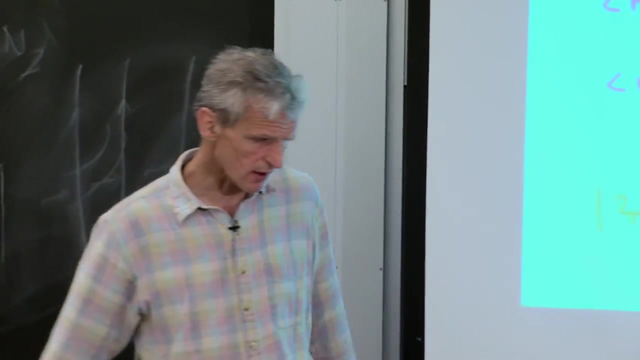 into the ideal. gas wave function is only 1% for alkali gases, But for liquid helium the condensate fraction, even at zero temperature, is only 10%. So when people use neutron scattering, it would be a long story in itself how this is done. 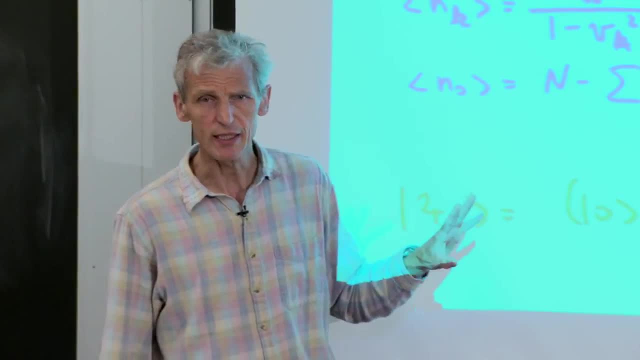 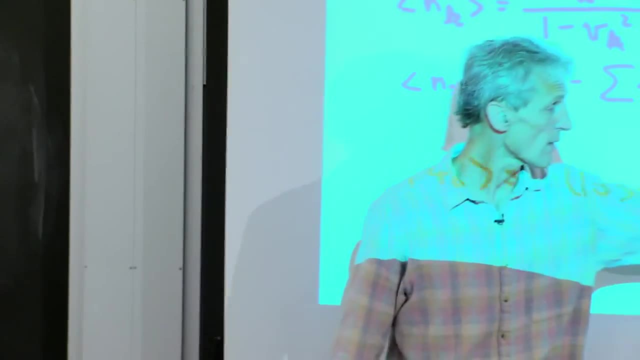 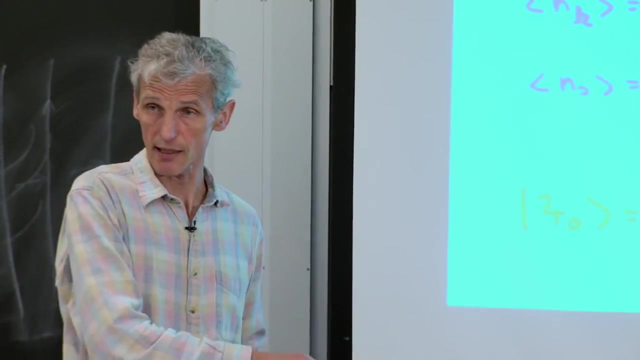 But when they use neutron scattering to analyze liquid helium at low temperature and figure out what is the fraction of atoms which have zero momentum, they found 10%. The quantum depletion is 90%, But that's just the difference between a quantum gas and a quantum liquid. 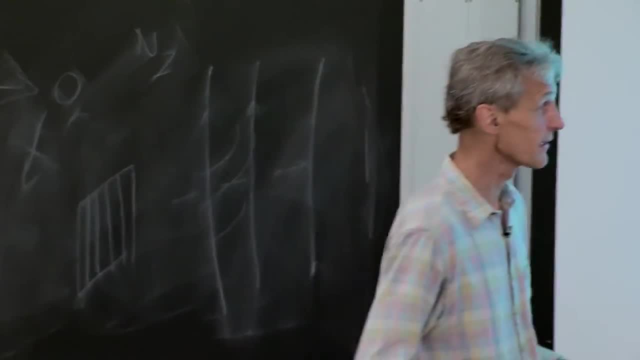 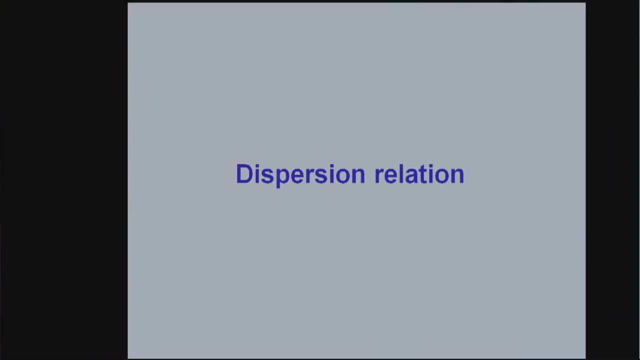 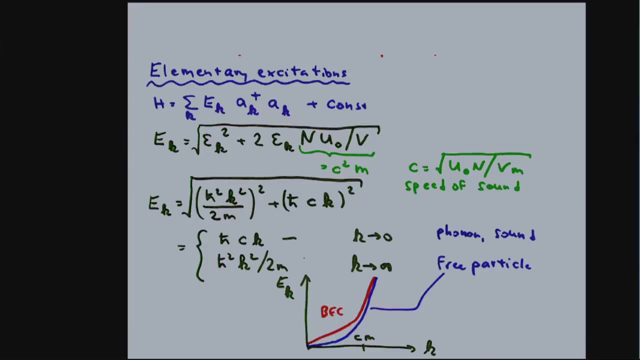 And in the quantum liquid, in liquid helium n a cubed is on the order of unity. OK, I mentioned this dispersion relation. These are sort of quasi-particles And I at least showed you how you can measure the slope of the quasi-particle dispersion. 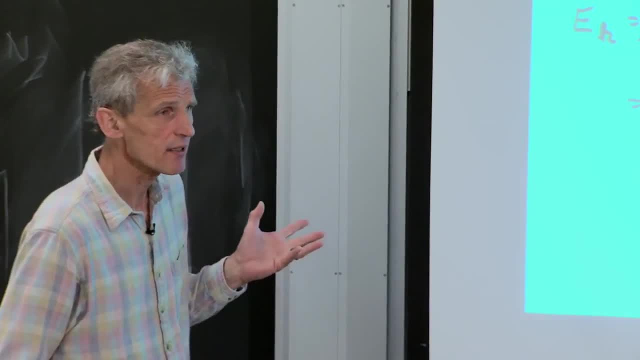 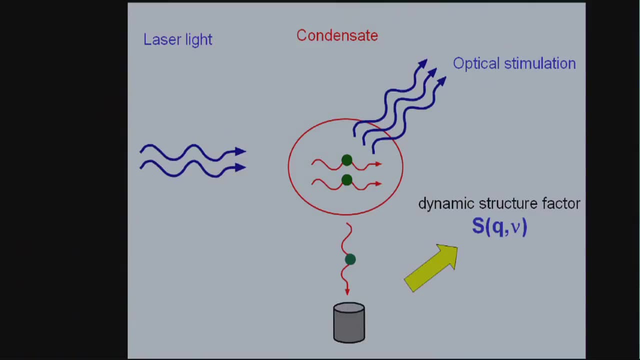 relation by propagating sound waves. But let me now tell you how we can observe quasi-particles, elementary. We can observe elementary excitations directly, And this is actually simply done by light scattering. If you scatter a photon and the scattered photon. 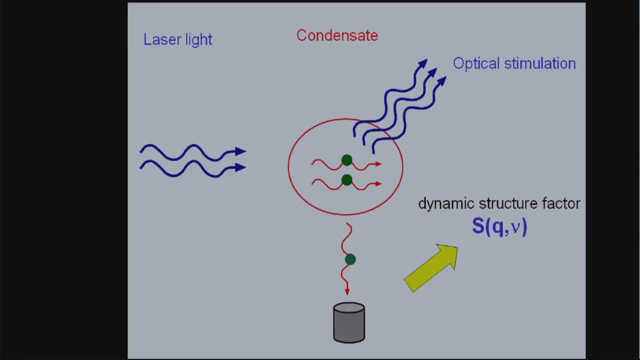 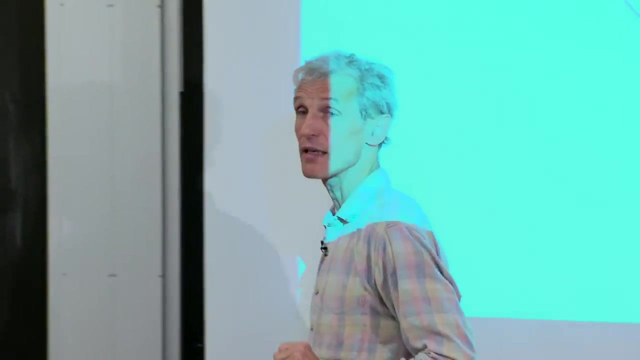 loses energy h bar nu and it is scattered at an angle. therefore it transfers momentum q. This process can only happen if there is an elementary excitation with momentum q And energy h nu, So in other words on a photon basis. 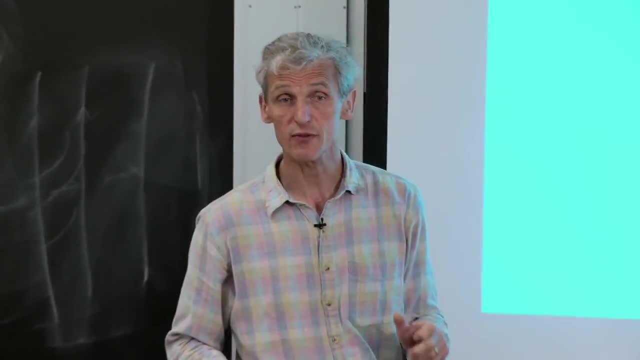 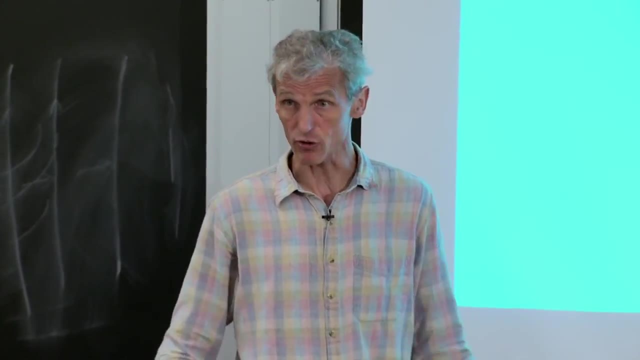 you can see photon by photon. if you scatter a photon, the photon transfers momentum and energy. The process can only happen if you can form a quasi-particle with this momentum and energy. So, since this is sort of the direct way of mapping out, 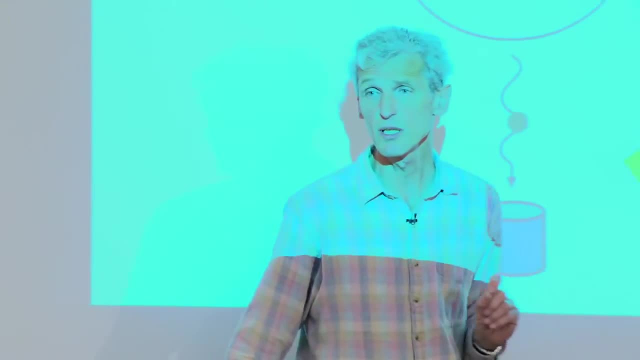 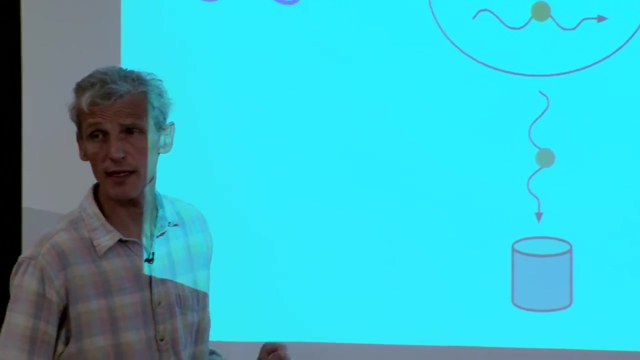 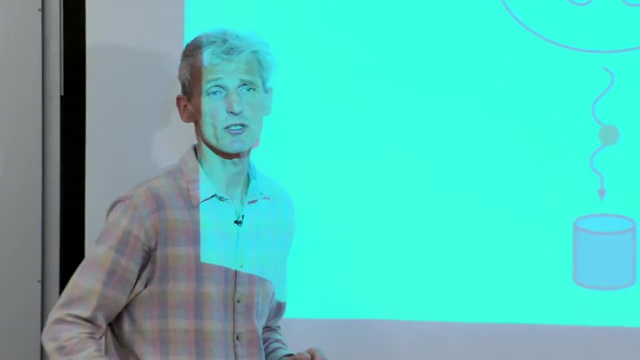 whether the system has the possibility to absorb momentum q and energy h, nu. this has sort of a name. The scattering probability is called the dynamic structure factor, and the dynamic structure factor is just an integral over all the possibilities that a many-body system can absorb momentum and energy. 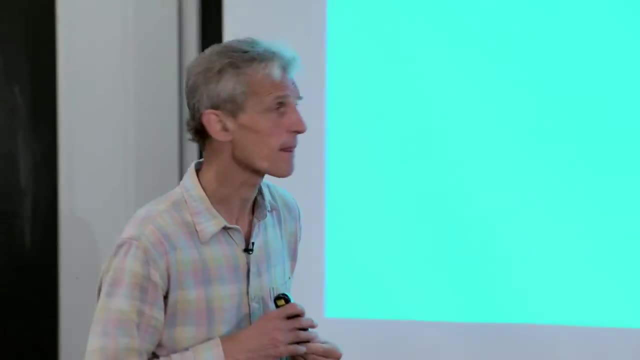 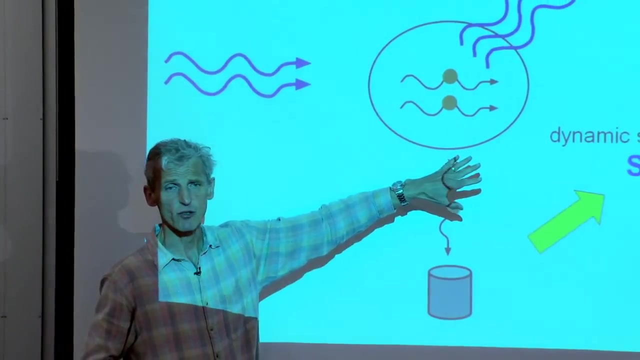 Now there is one nice feature which was introduced by us here at MIT, And that is, if you want to measure the dynamic structure factor, often you do it with neutron scattering. You scatter neutrons or x-rays and they scatter spontaneously at an angle. 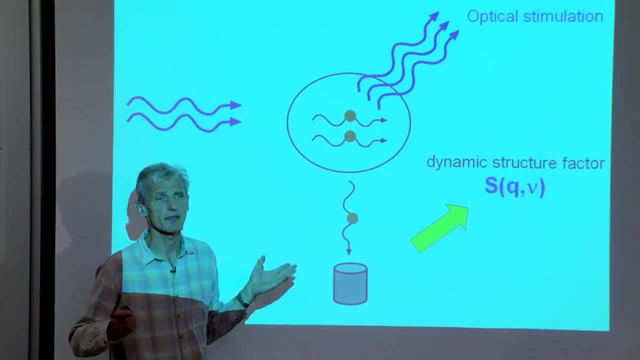 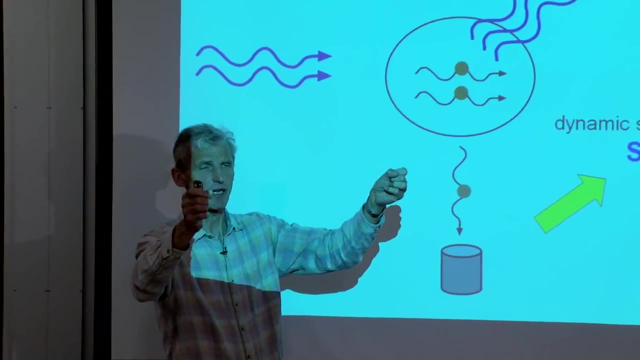 And you need a detector to detect the scattered particles. But in our case, because the gas is so dilute, the distance between atoms is on the order of the optical wavelengths. We don't want neutrons, We don't want x-rays. 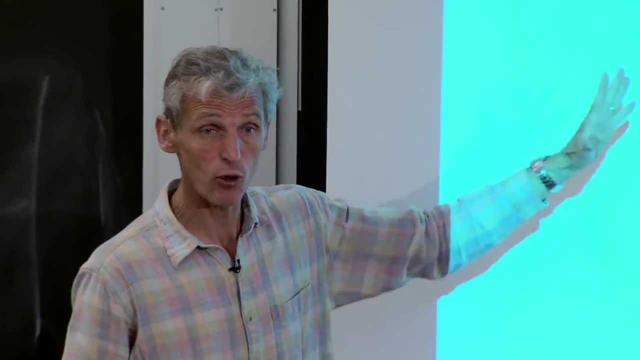 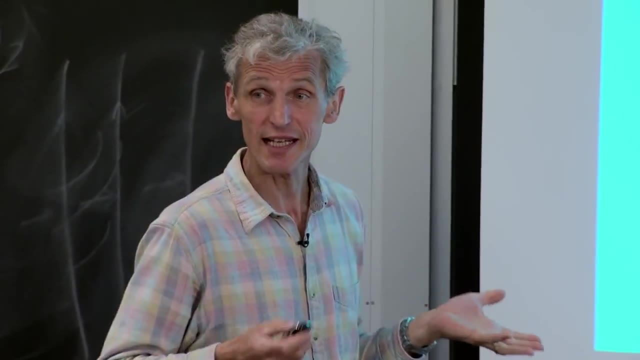 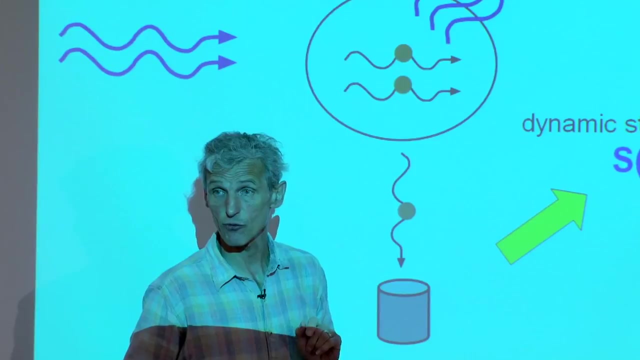 We want photons, because the wavelength of photons is perfectly matched to the properties, to momentum transfer and such we need for our system. But photons, we have photon lasers. So instead of in a painstaking way analyzing the frequency and the momentum of scattered photons, 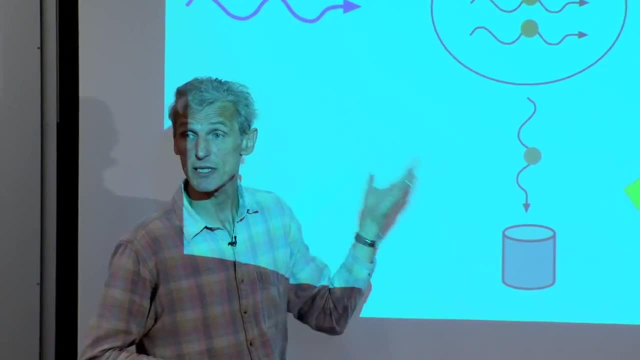 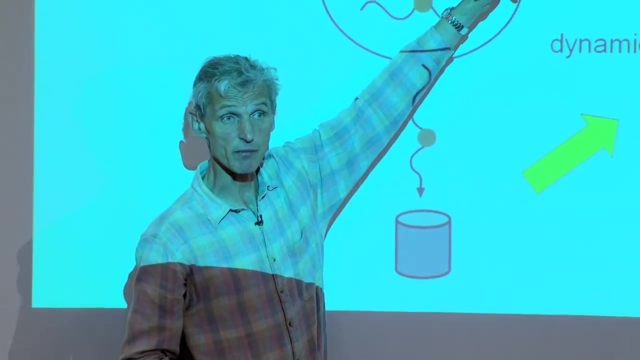 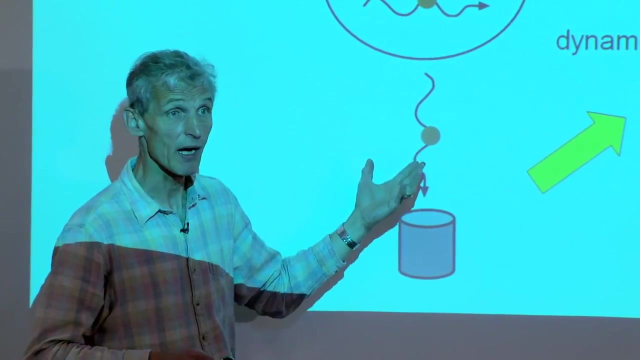 we don't do the spontaneous scattering process, We do a stimulated process. We use two laser beams and we stimulate a photon to be scattered into the other laser beam. And by having the two laser beams at frequency difference- delta, omega- we are really asking the system. 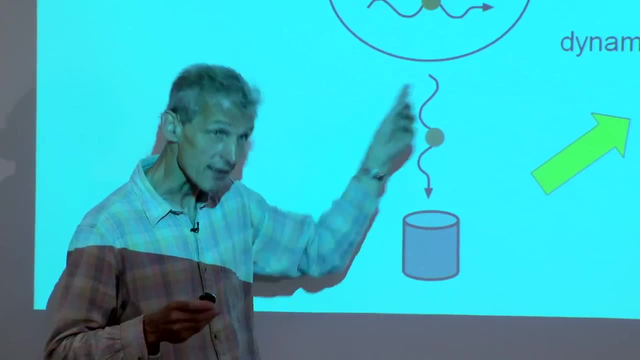 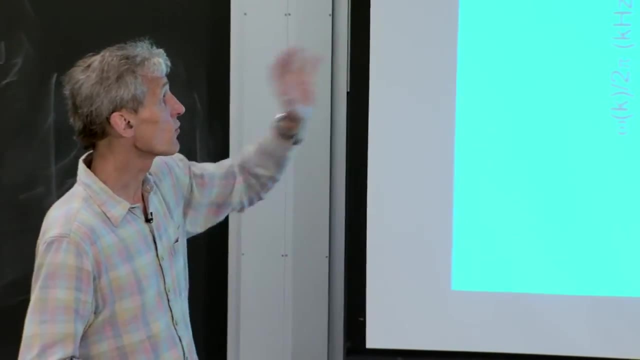 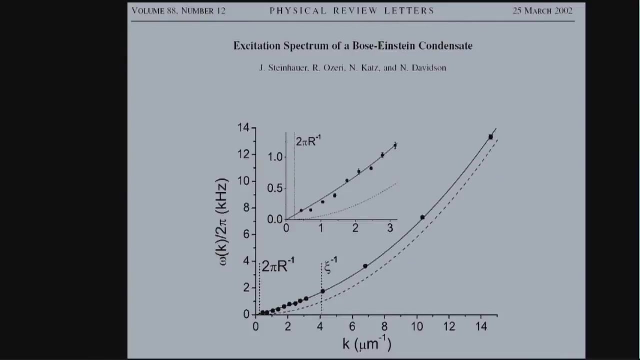 are you ready to absorb delta omega energy? If yes, then you have a quasi-particle. So this is how we do quasi-particle spectroscopy, And a few years later this method was refined by the group at the Weizmann Institute. 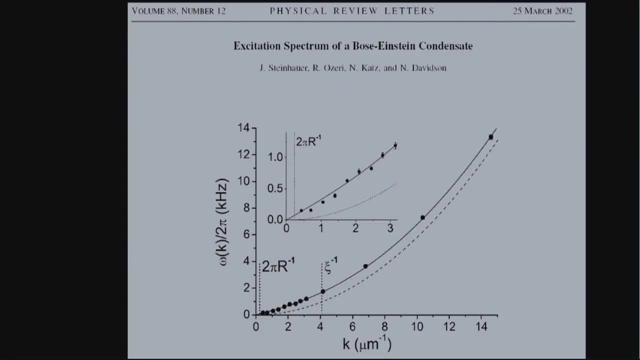 And what you see here is they varied the angles between the two laser beams, realized different momentum transfer And what you see is the linear dispersion relation for low momenta and then the quadratic part at high momenta. So this is called Breck spectroscopy. 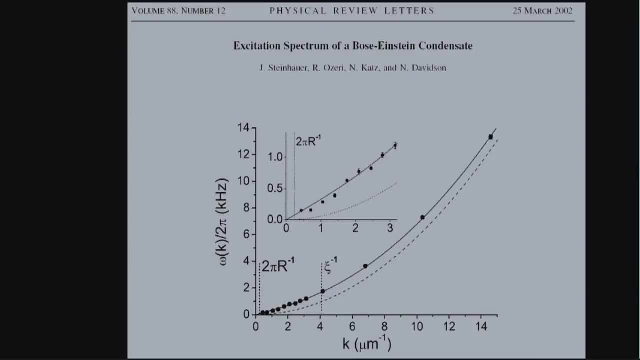 It's a variant you can see of Raman spectroscopy, where you go from a 0-quasi-particle state to a 1-quasi-particle state through a stimulated Raman process And this is how the dispersion relation is determined. 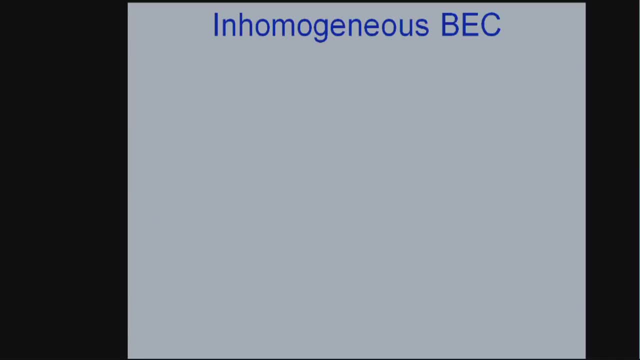 OK, So I've so far dealt with aspects of a homogeneous Bose-Einstein condensate, where, of course, if you have a homogeneous system, you formulate everything in momentum space. But now we want to deal with the situation that our condensates are finite in size. 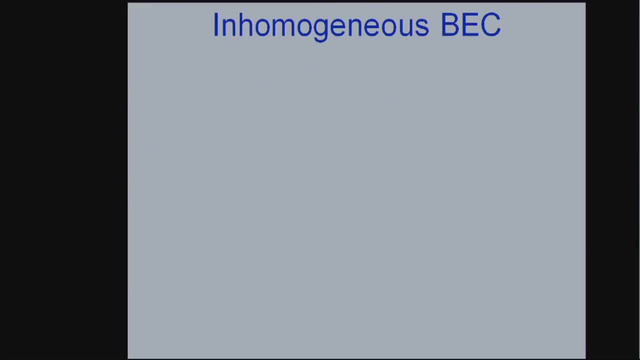 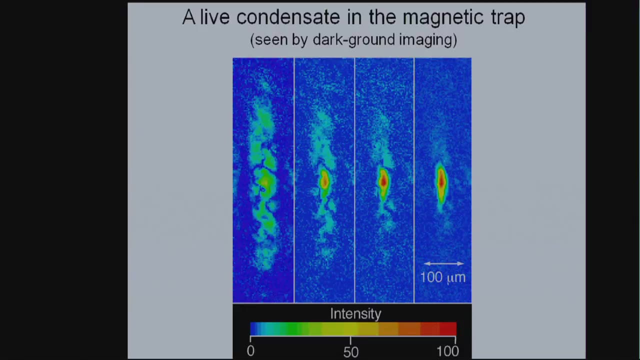 And in addition they are usually in a harmonic oscillator potential And therefore their density is inhomogeneous. Let me start the discussion with the inhomogeneous Bose-Einstein condensate by showing again a picture which brings in some 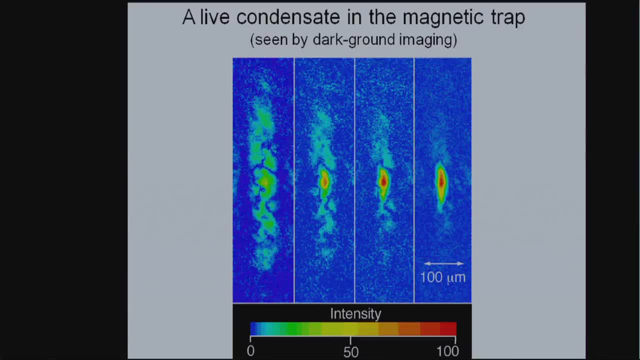 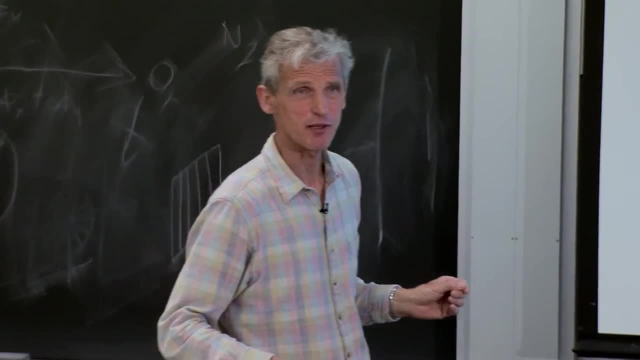 again memories of 1996.. It was the first time that we could see a Bose-Einstein condensate in the trap- Before people have just seen it by time of flight- when it was pretty much already destroyed or it was just flying out. 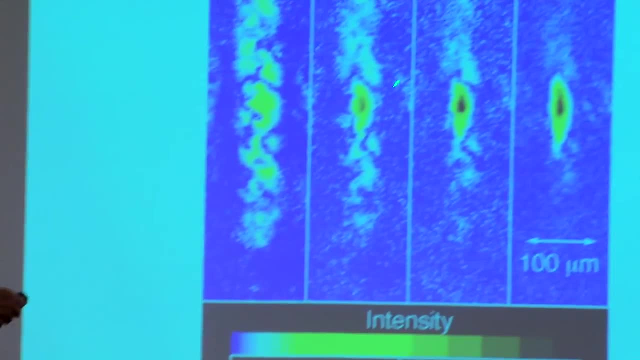 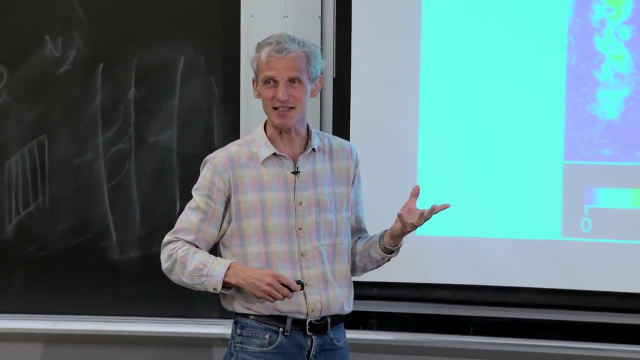 But here we see the trapped Bose-Einstein condensate, And we could even take multiple pictures of the same condensate. So you can see this was the first time that a condensate was seen alive. What you see here is actually the bimodal distribution. 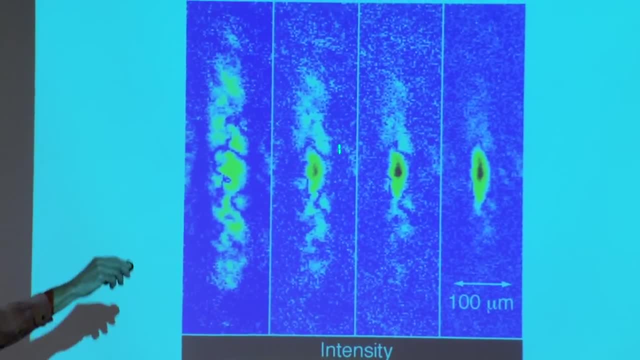 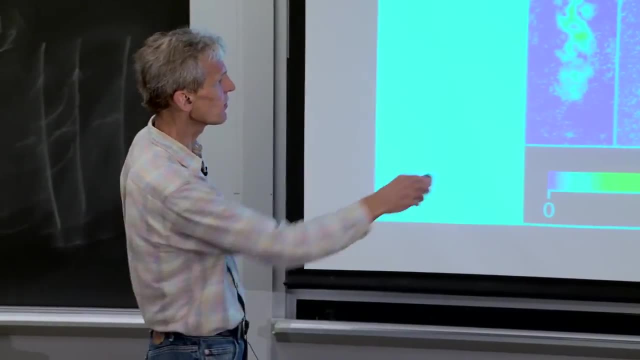 You see the condensate And then, due to speckle pattern, the thermal cloud looks fragmented. But this is just a speckle pattern due to the signal-to-noise. But here you really see, now not in ballistic expansion- 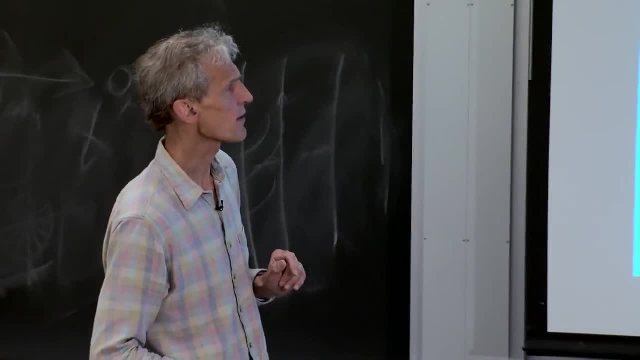 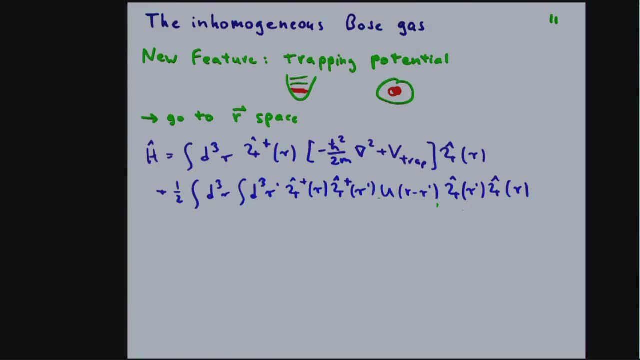 as I've shown you on Monday, but really in situ, the size and shape of the condensate. OK, how do we describe it? Well, the message is Pretty much exactly the same way as we did with the Bogoliubov approximation and such. 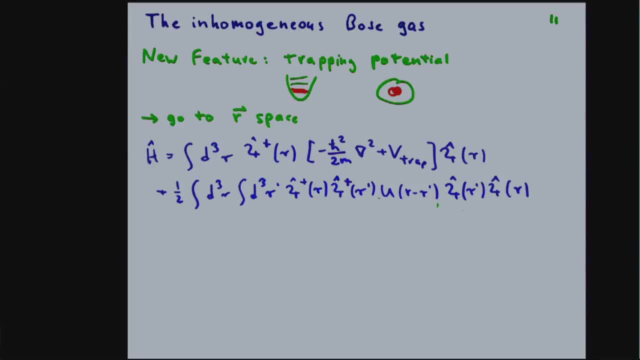 But instead of in momentum space, we do it now in position space. Actually, I have to say, this week I go through a lot of material, But what I'm trying is to give you sort of a spirited and animated overview that you really 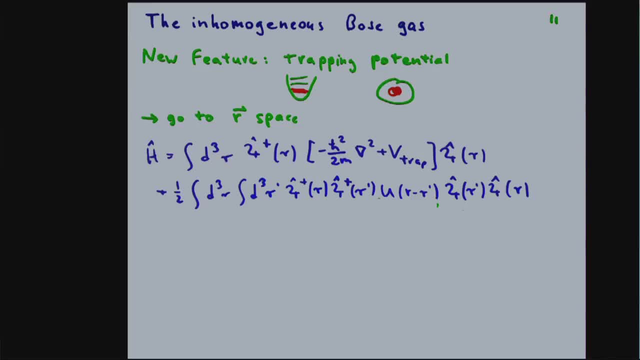 know what is important. Where is the same concept appearing again in a different way? The details I've posted actually the original art articles, references, summer school notes, some of them written by myself on the website. So yes, it's a little bit different character. 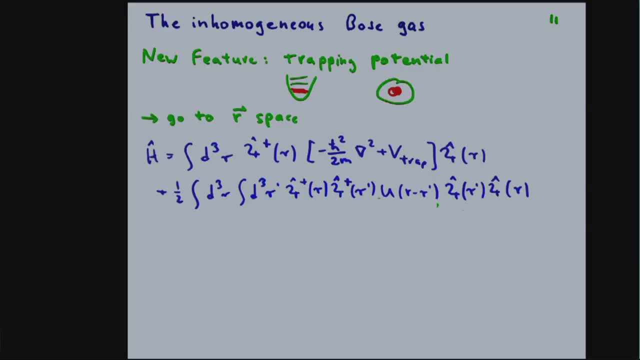 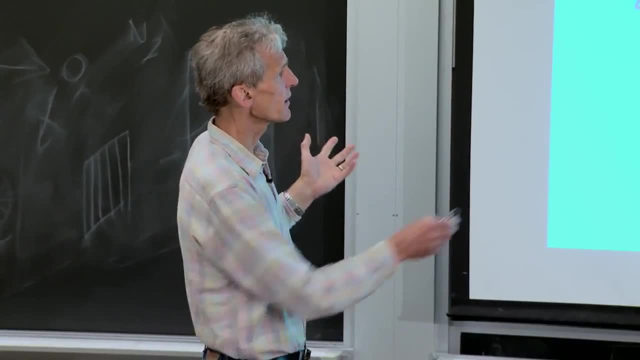 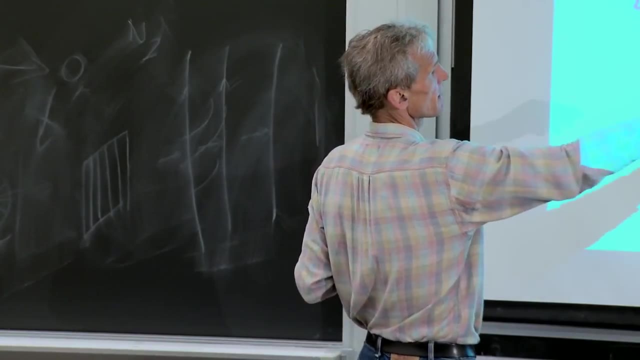 than other lectures. I want to show you a lot of things and put a special emphasis on the ideas. OK, so in second quantization we are now using field operators which create and annihilate particles at position r. This is sort of the single particle Hamiltonian. 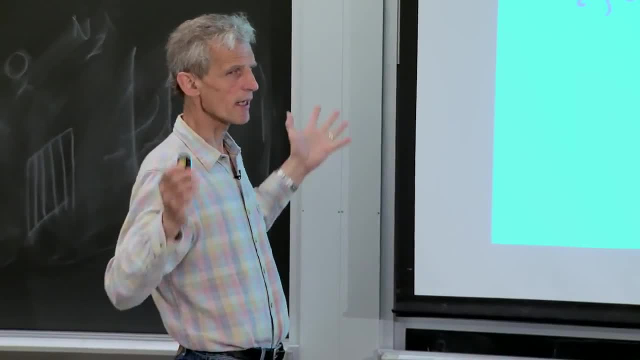 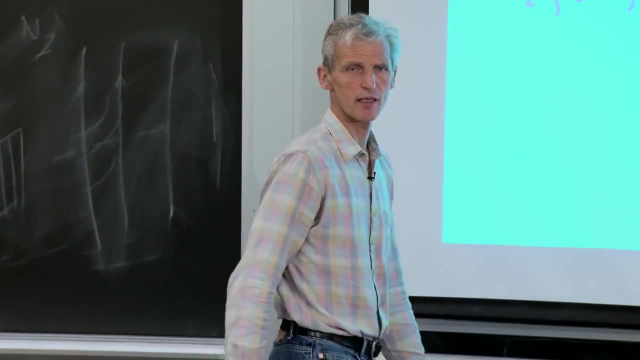 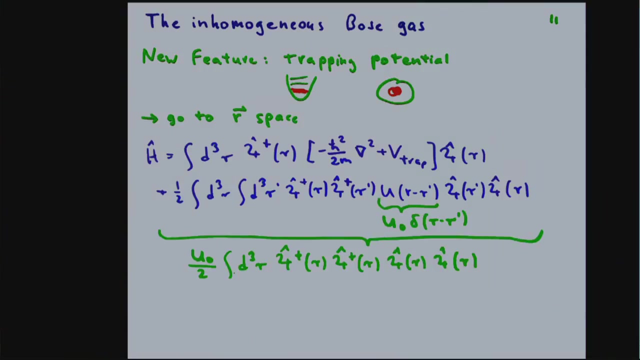 kinetic energy and potential energy And our interaction. Interaction term has now again four operators: two annihilation operators, two creation operators, But they are now formulated in position space. We do exactly the same as we did in the homogeneous gas. 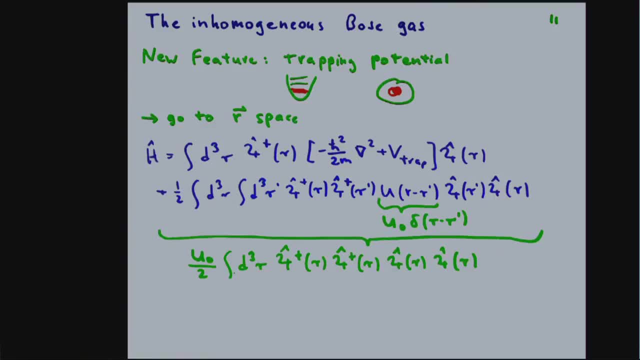 We assume the potential is short range. That means delta function And that means we can get rid of one of the integrations in r and r prime, But we still have product of four operators. We can formally solve the equation by writing down Heisenberg's equation for the equation. 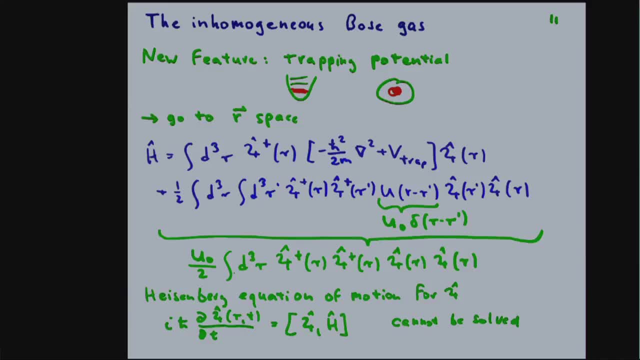 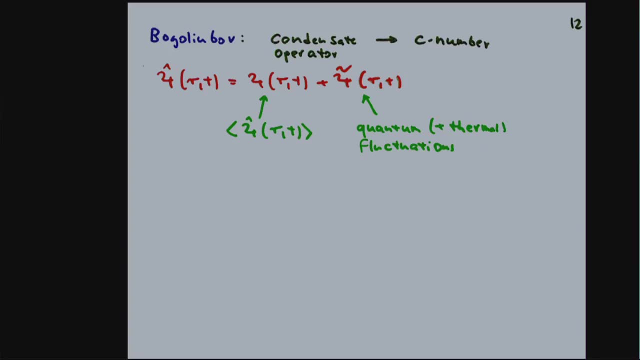 of motion for those field operators. But of course this cannot be solved. Remember, products of four operators are hard. We have to reduce it to two operators And this is actually done by the Boboliubov approximation, again, But it's done here in the following way: 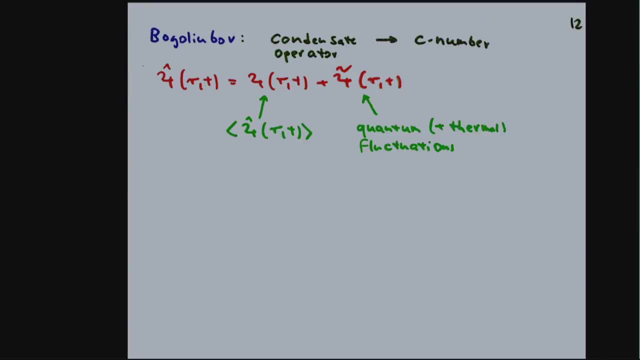 Remember, in momentum space We replaced a0 and a0 dagger by the square root of a0. What we do here is we say this is sort of a quantum field, And when we have a superfluid, this field operator has an average value. 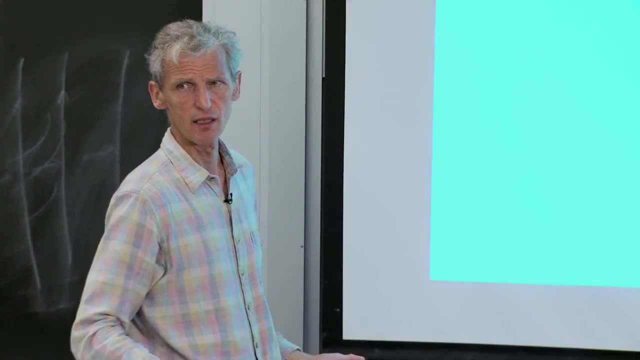 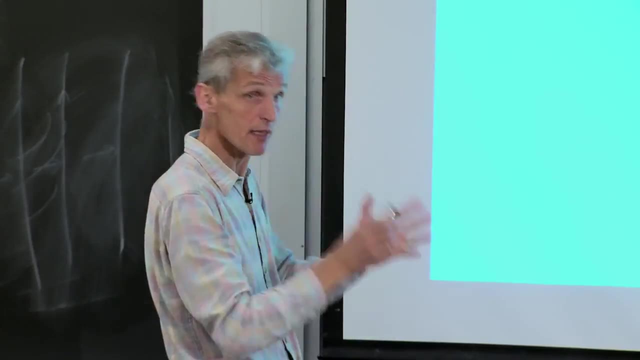 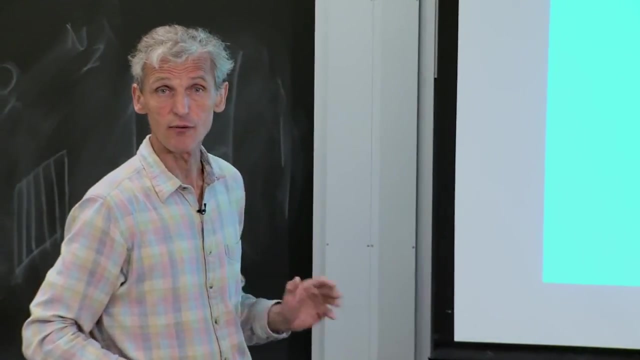 It's actually the macroscopic superfluid order parameter. So we replace the operator by an average value which we assume is large, Because many, many particles are in the superfluid state, And then we have fluctuations which are small, And what we will do is: well, it's pretty clear. 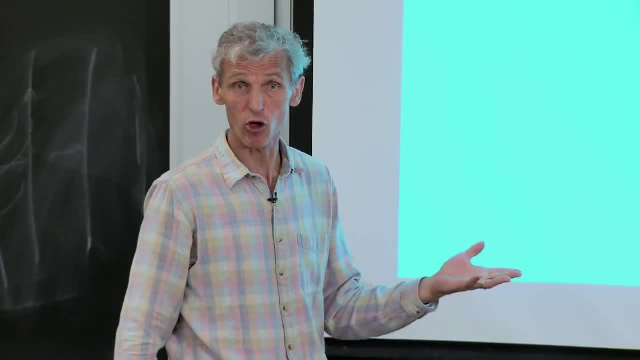 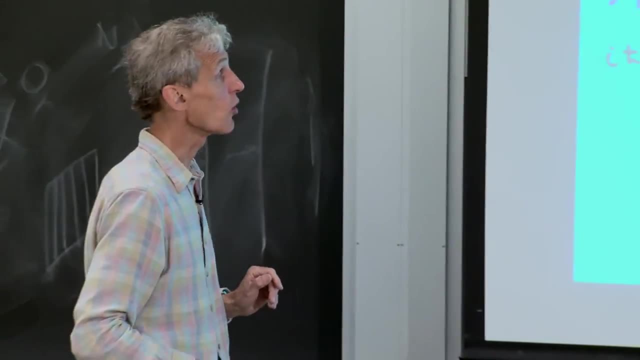 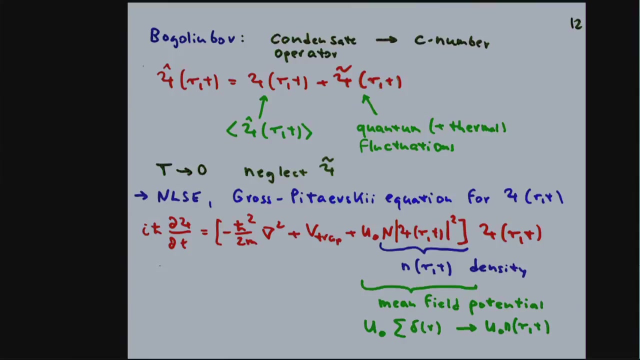 When it comes to the fluctuations, we will neglect higher products, products of four fluctuation operators And we are down to c numbers And, as you will see, two operators We can, and this is even more dramatic. It wouldn't make sense in momentum space. 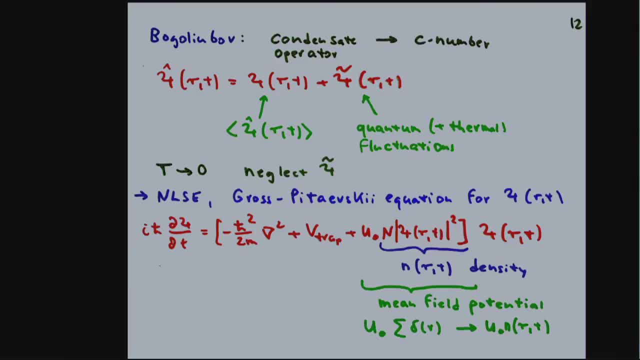 But it does make sense. in position space We can even do a first approximation where we completely neglect those fluctuations, And then what we have is when we simply insert a c number into- let me just go back into this- Hamiltonian. we have then an equation for this number. 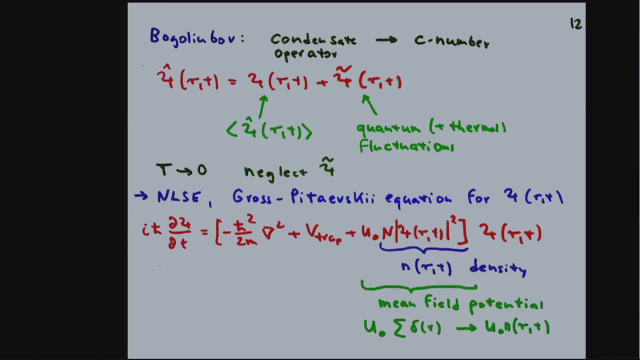 for this function, psi, And this is the nonlinear Schrodinger equation, also called Gross-Pitayevsky equation, which is now the analogy to Schrodinger's equation. but now for the macroscopic wave function, which is occupied by many, many particles. 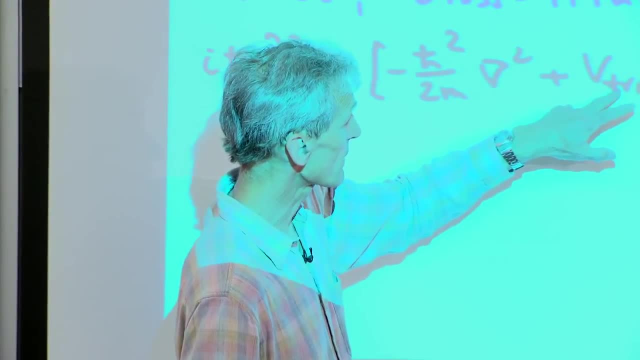 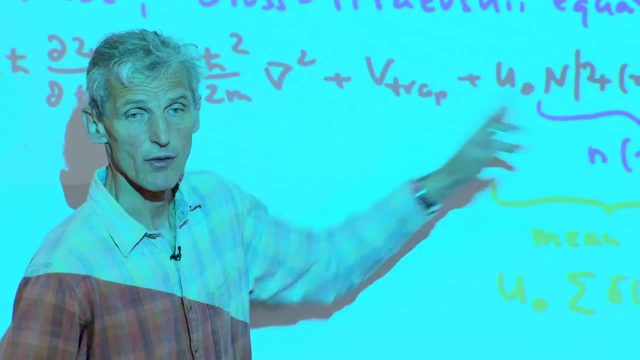 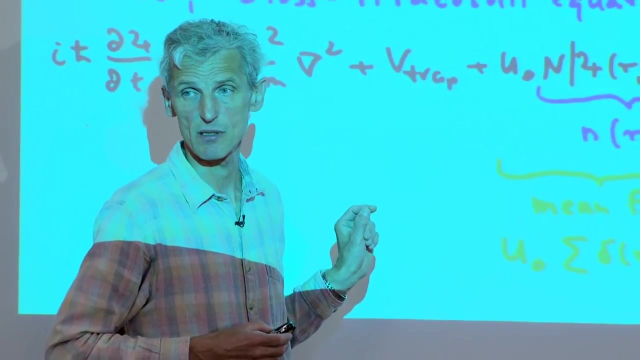 And in addition to the kinetic energy and the trapping potential, the external potential, it has a term which is proportioned to the density- And this is just a mean field repulsion- which one atom feels exerted by the other atoms. I should say 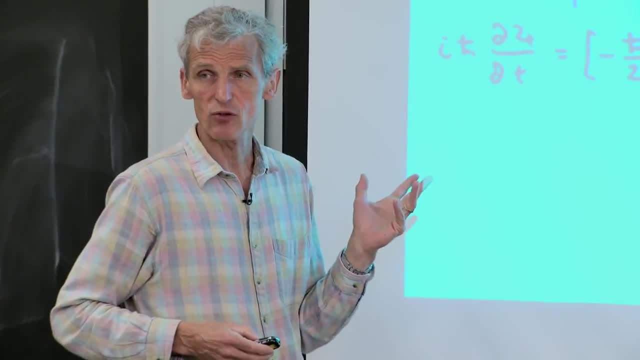 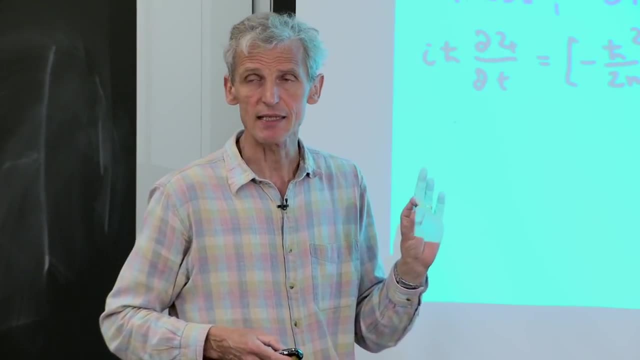 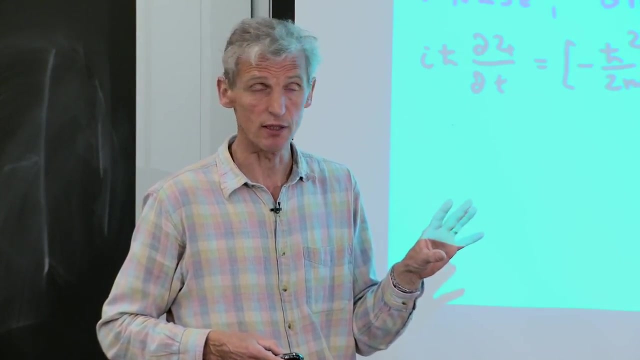 So just to connect it to what I've said earlier about the quantum depletion, you can regard the function psi as the best approximation to an ideal Bose-Einstein condensate. So if you want to write your many body wave function as a function psi to the power n, 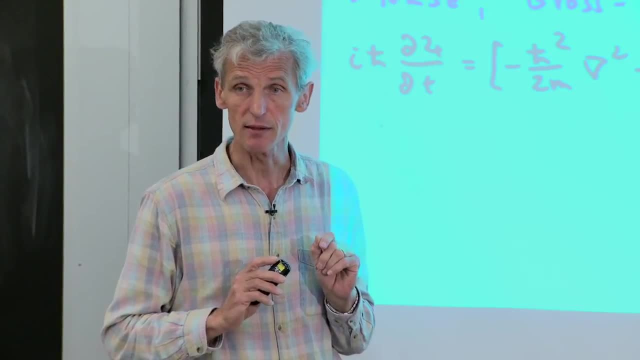 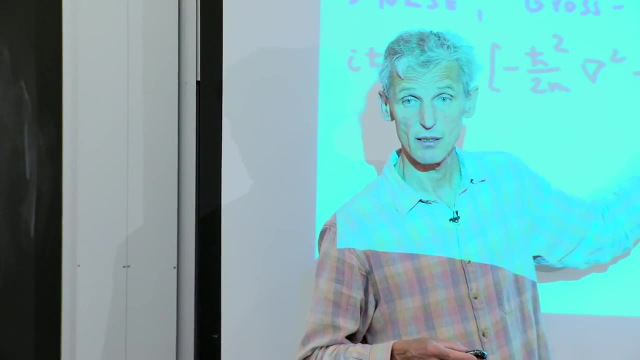 all particles are in the same quantum state, Then a variational calculation would say that this function, psi, should obey this equation. If you want to read up what I've said, I've posted a recent paper from which I found very pedagogical where they 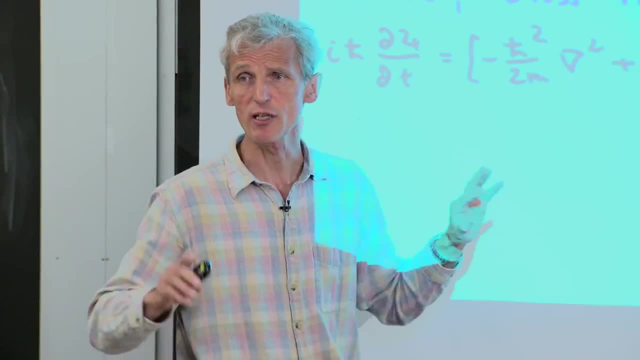 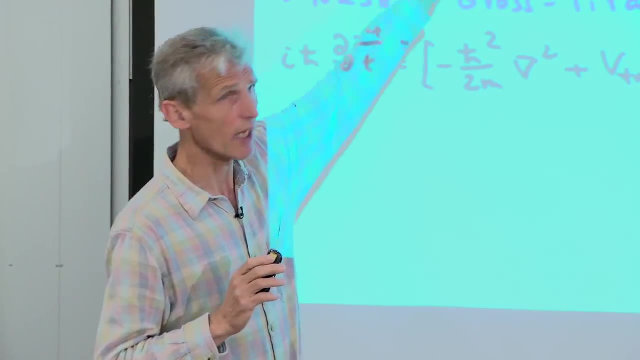 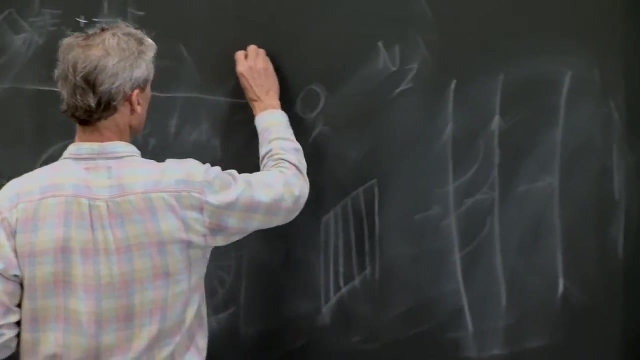 say we can get where they derived the Gross-Pitayevsky equation without even using an operator, psi dagger, without using any second quantization. They just say we have a Hamiltonian for an interacting system and we try to write the complicated many body wave function as a wave. 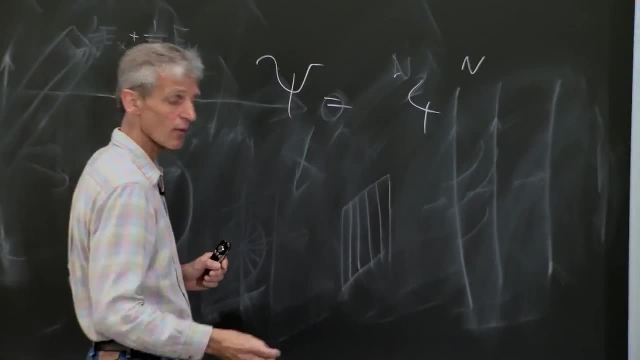 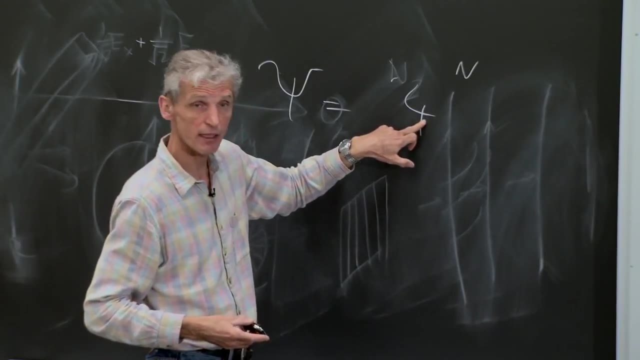 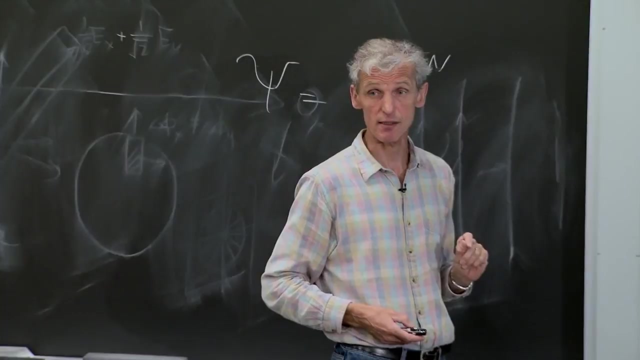 function to the power n. And then you put these answers into your Hamiltonian and do a variational optimization: which single particle wave function, psi, if taken to the power n, minimizes the total energy of n particles including interactions? And the answer is this equation: 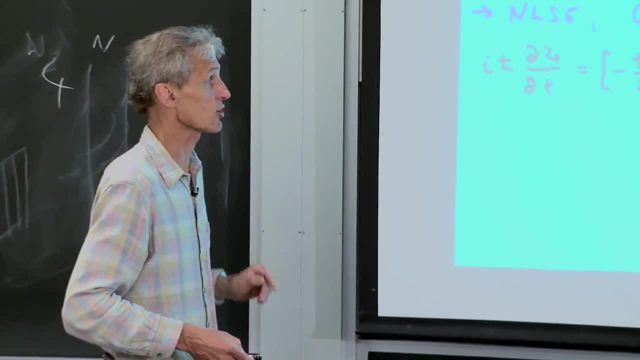 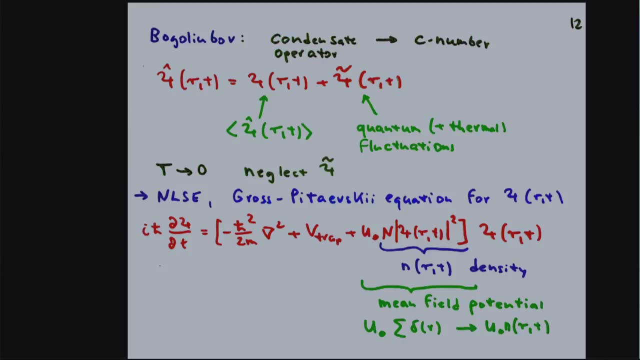 So there are many ways this equation is sort of very natural. Now. you all know about single particle physics, kinetic energy and external potential. Let's now learn what this density dependent term does. Well, it's pretty clear. there is a price to be paid for density. 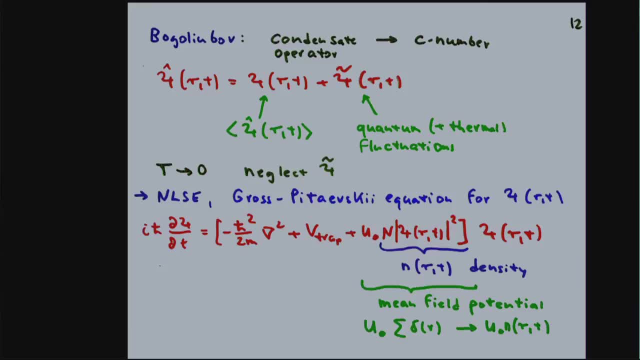 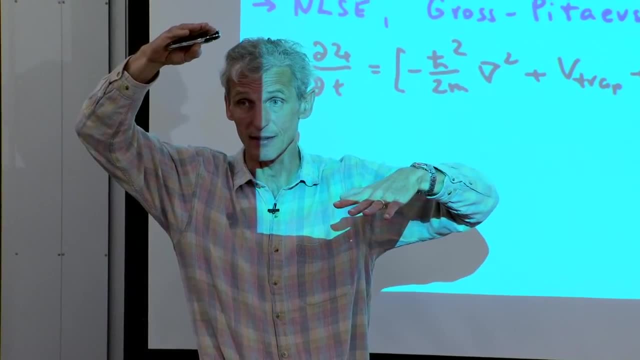 And well, the total integrated density is, of course, given by the total number of particles. That means if you lower the density somewhere, you have to increase the density. But because this is a nonlinear term, if you have an average density and you lower it here, 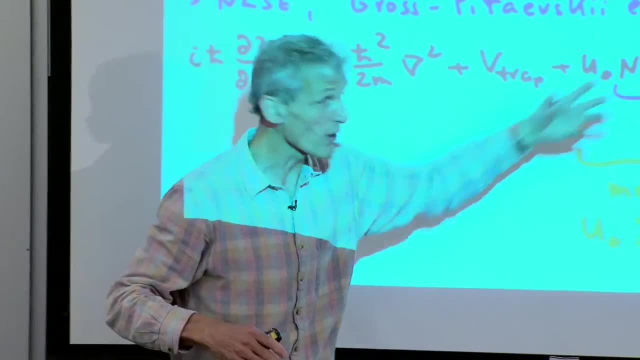 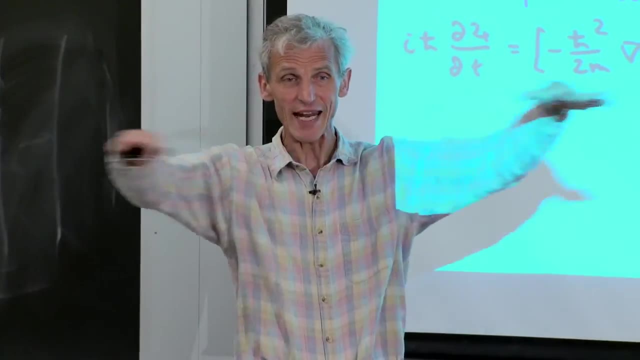 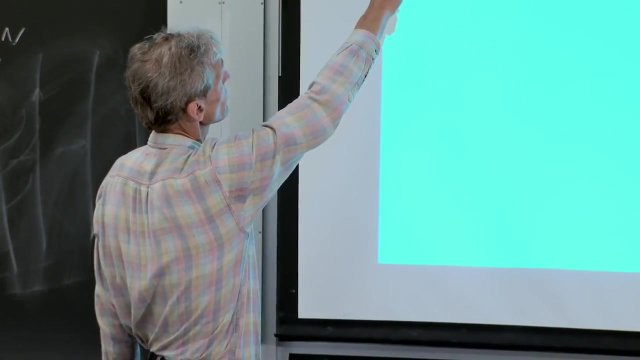 and increase it. here you have actually more repulsive energy than if the density is flat. So this term has only one goal: It wants to flatten out densities. So therefore, if we have a box potential and you know the ground state in a box, 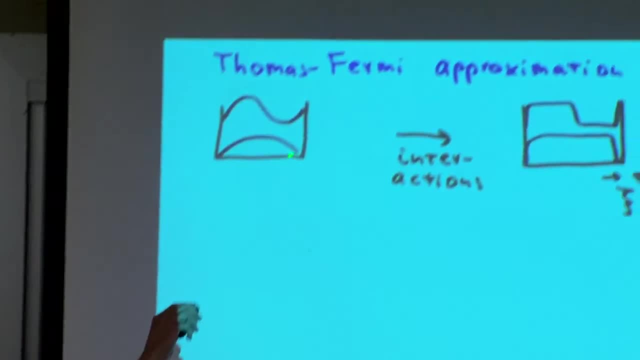 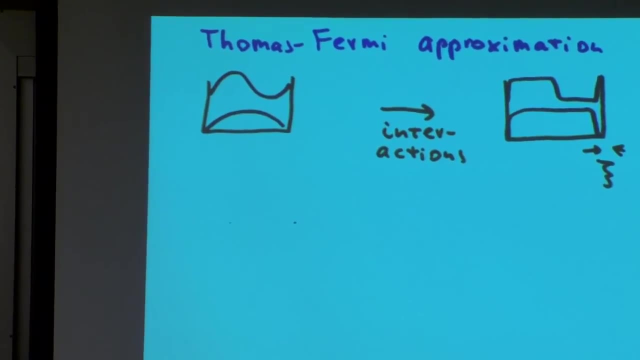 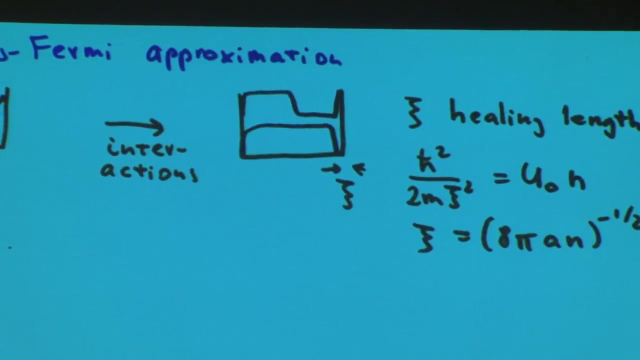 is just half a period of a sine function. if you now put in strong interaction, this is a non-interacting condensate. This would be the macroscopic wave function in a box potential. But if you now put in strong interactions, the strong interactions want to flatten out the potential. 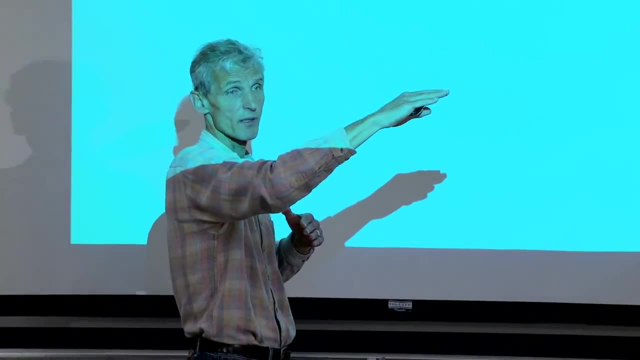 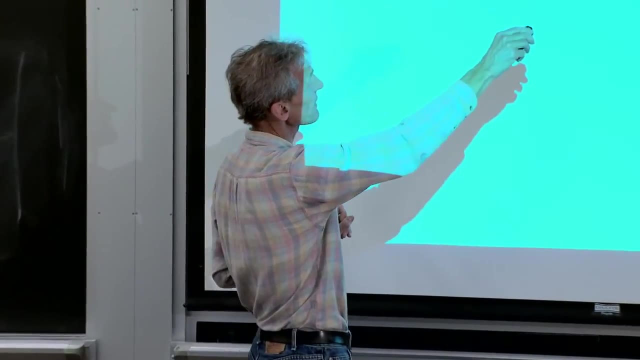 They flatten out the potential, and only at the very last moment. all right now, it's time to go down, because we have to meet our boundary condition And the length scale where you eventually go down it has a famous name: the healing length. is the length scale where the kinetic energy due to the curvature of the wave function is now comparable to the interaction energy. If the system would curve down earlier, it would cost too much repulsive energy because the density is not kept flat. 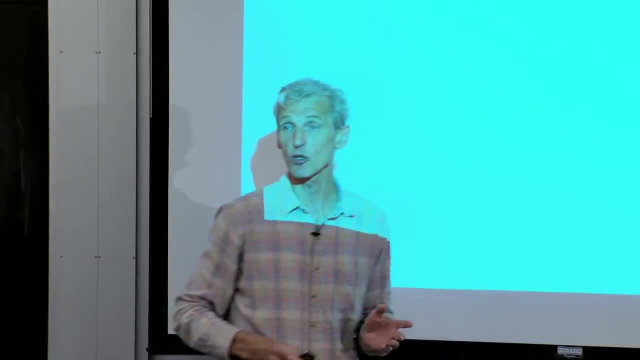 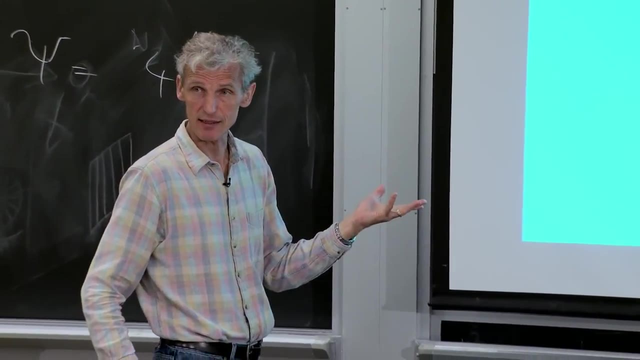 If it would curve down too late. the enormous curvature would mean a lot of kinetic energy, And this is just the best compromise between those two criteria. So that's how you derive the healing lengths, The healing lengths. The healing lengths is now the length scale. 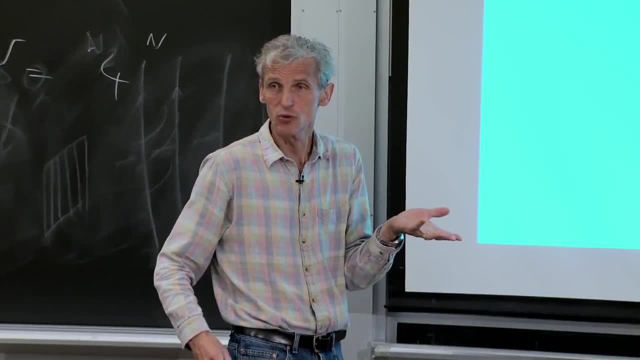 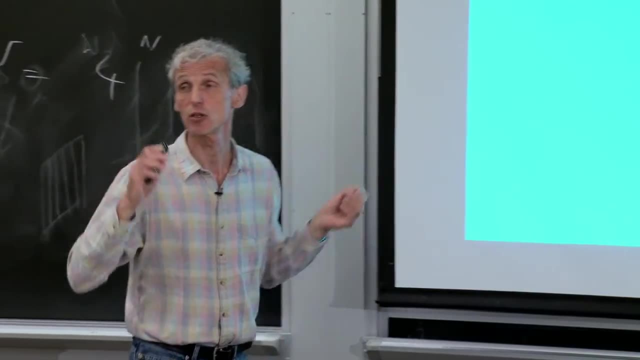 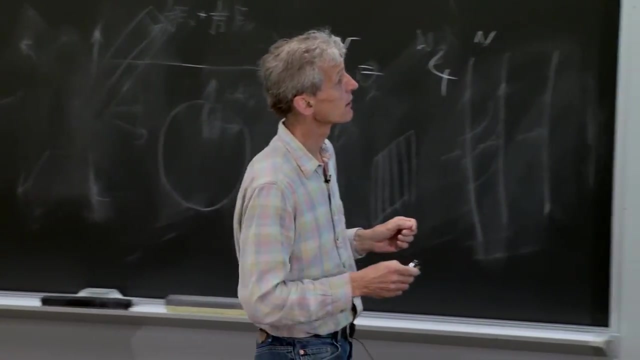 over which the system is willing to meet boundary conditions and not stay flat, as flat as possible. Timo, I'm just curious in that equation that the atom is the mass of each individual. The mass is the mass of a single atom. 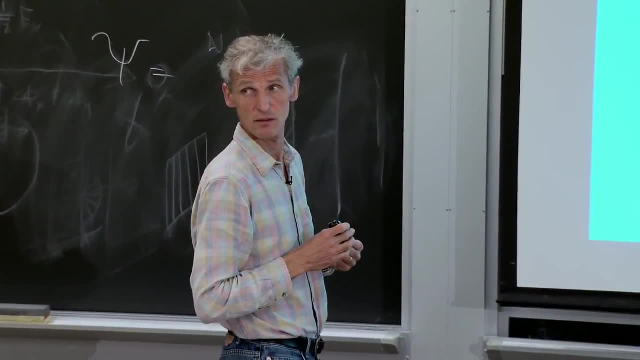 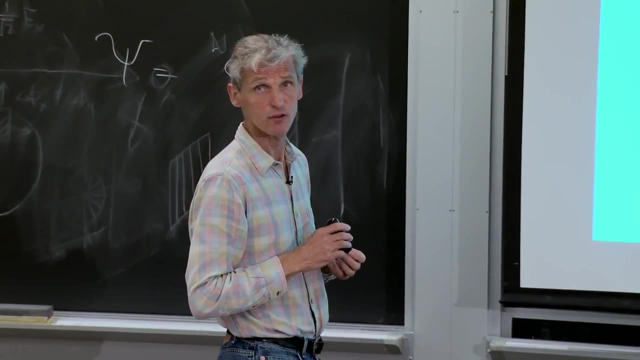 A single atom. It's not a- I don't sorry I wasn't here last class, but the quasi-particles of the same mass or whatever it is, In the Gross-Einstein condensate they are. We don't- we haven't changed the mass. 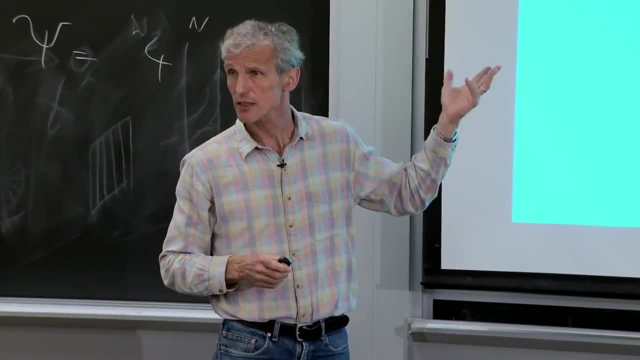 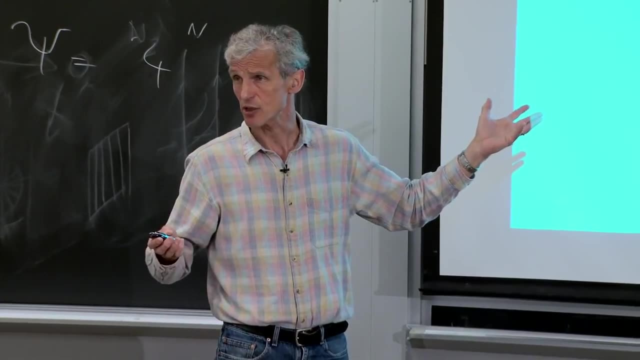 But we're not talking actually about quasi-particles, We're simply actually. we're really talking about here qualitative features of the solution of the Gross-Pitayevsky equation. And the Gross-Pitayevsky equation is sort of a single-particle equation. 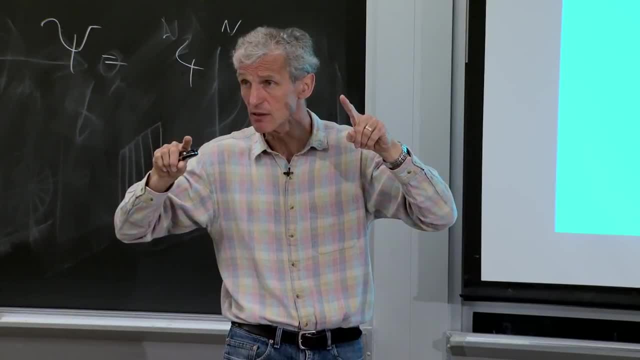 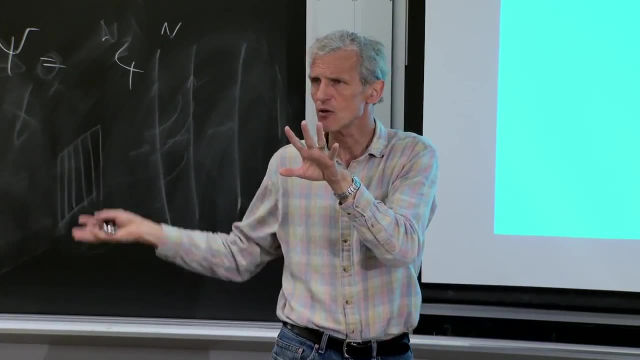 for particles of mass of the original bare mass, m. It's a macroscopic wave function, but I sometimes say it describes a wave function of a, z. It's a single particle where all the other particles are included at the mean field level. 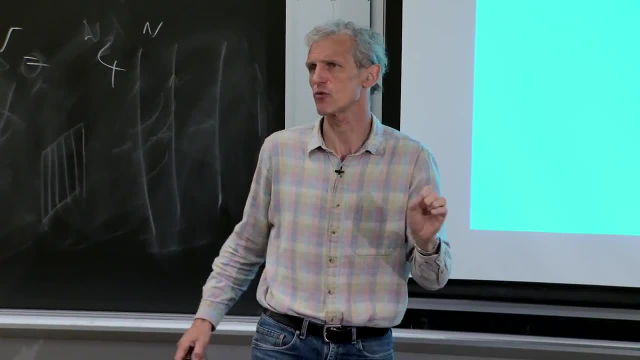 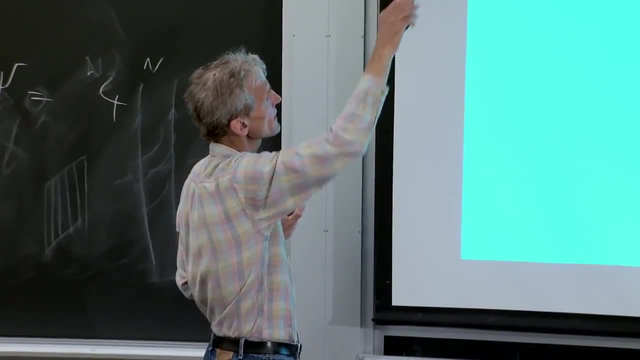 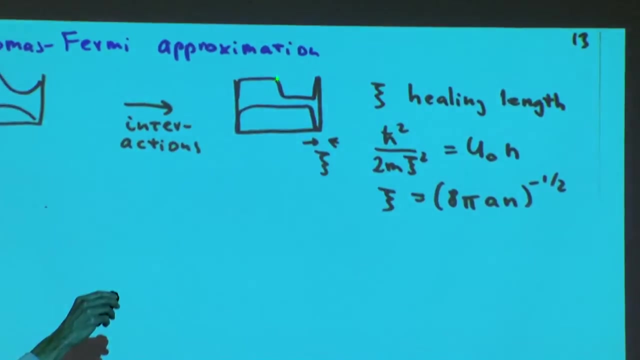 So therefore, it is really this the atomic mass, and not any form of collective mass here. Well, if you would now ask how do interactions transform the first excited state in the box, potential? Well then it's again flat. as soon as, as much as possible. 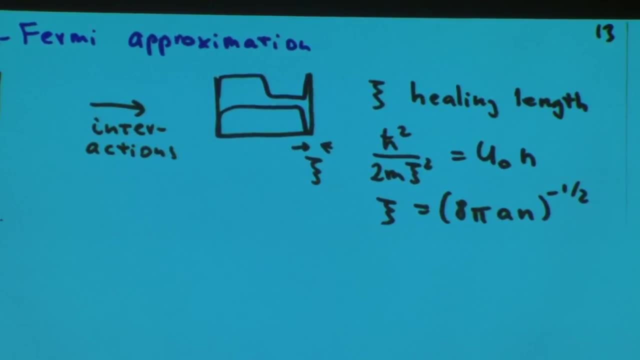 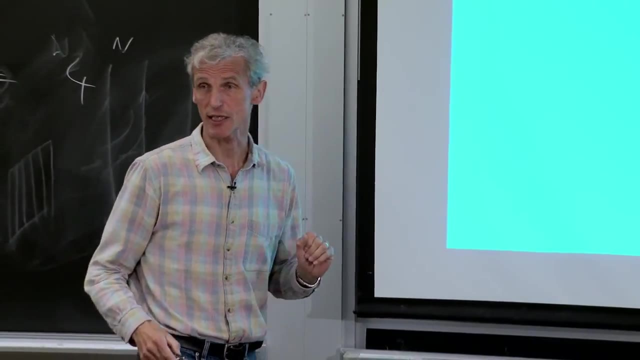 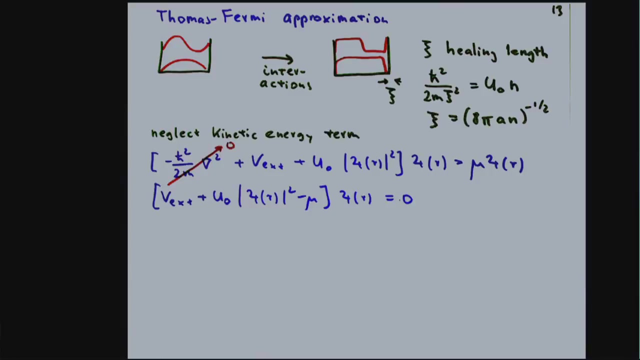 But then if you want to maintain the parity of the wave function, then it's only close to the zero crossing within a healing length that the system says OK, now I change sign. So that's sort of what is inside the Gross-Pitayevsky equation. 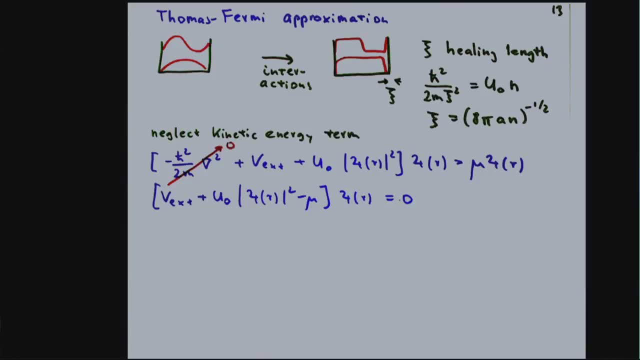 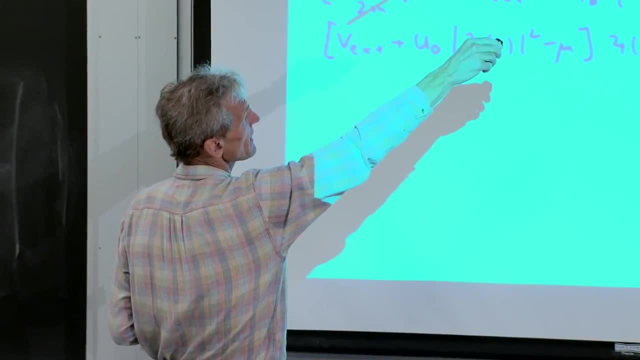 Now, once we realize that we can take it to the next level and say, well, if we neglect- let's say we're interested in the ground state and we neglect this boundary region where the kinetic energy becomes important, maybe we can simplify the Gross-Pitayevsky. 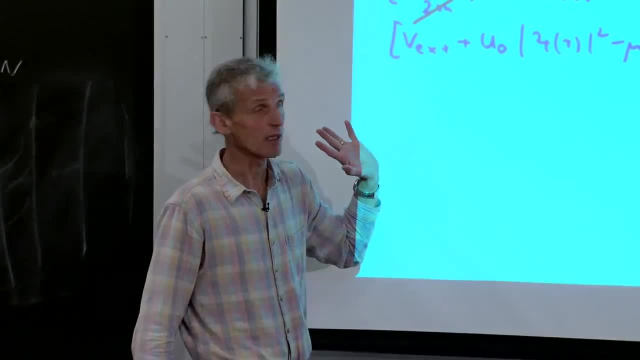 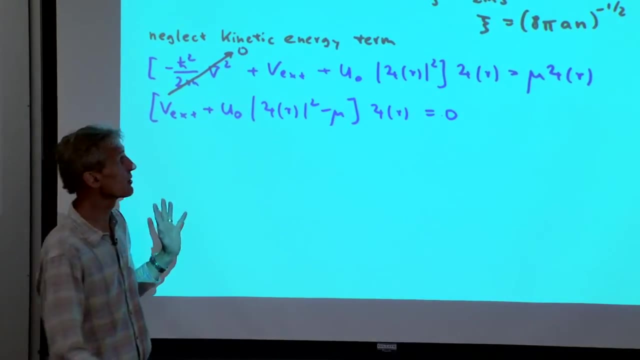 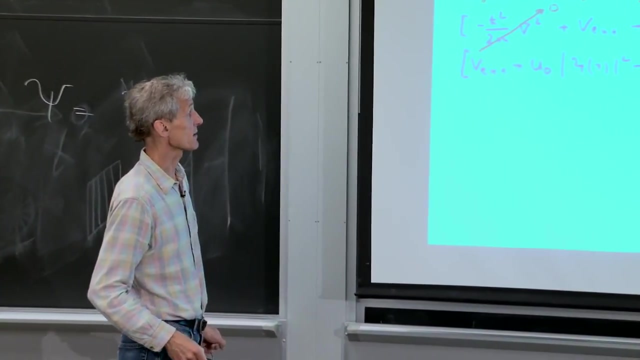 equation by neglecting the kinetic energy. If potential energy dominates by far, we can neglect that, And then we should get a good description which will not be valid in the wings of the wave function, but in most of space. But now, if you look at this equation, 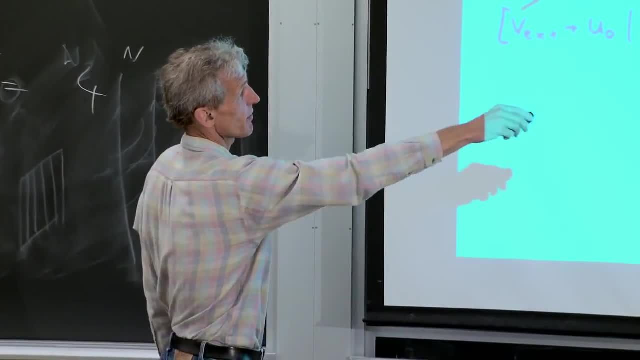 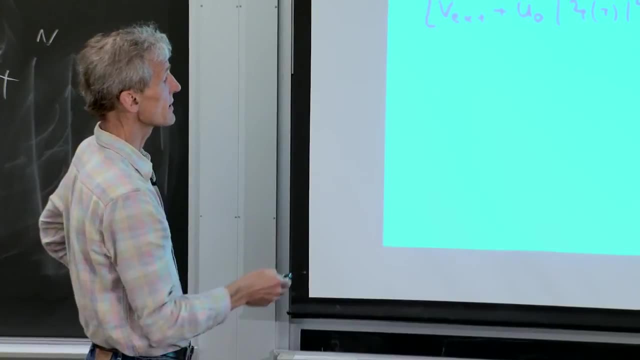 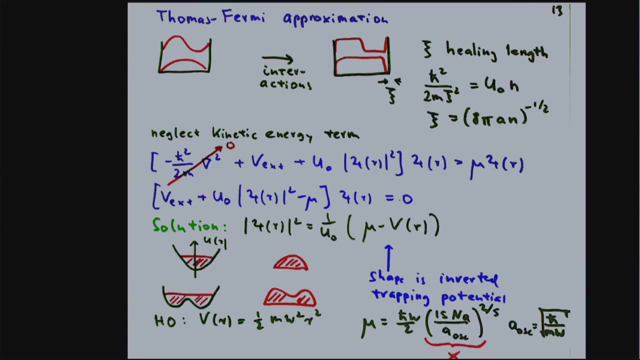 it's no longer a differential equation, It has no derivatives, It's just something which applies to the wave function psi itself, And we can simply solve that by. the solution of that is that psi squared, the density is nothing else than there is a constant minus the inverted. 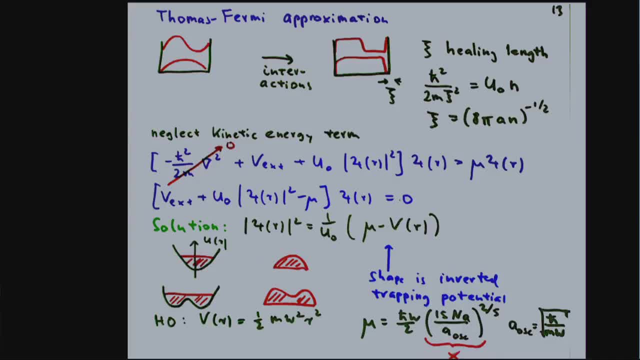 trapping potential. So therefore, in this Thomas Fermi approximation where we neglect the kinetic energy completely, you just take your trapping potential, turn it upside down and then you fill it up with density until you have accommodated the number of atoms. 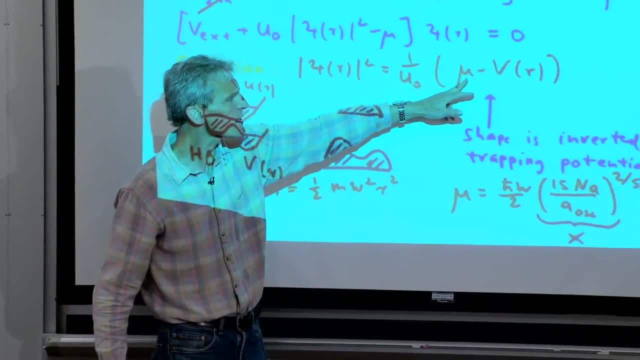 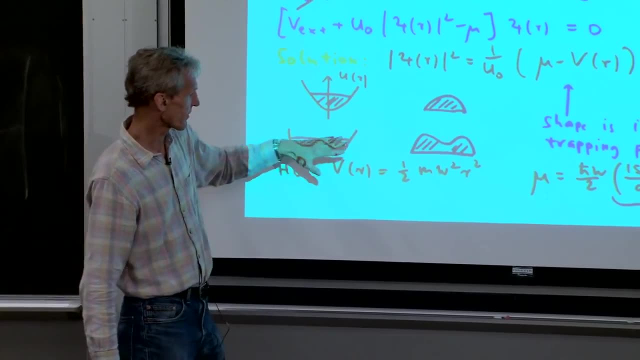 you want to accommodate, And this is, of course, the number of atoms. The constraint in the number of atoms is determined by the chemical potential. Or, if you have a more complicated W-shaped potential, the same construction: flip it over, fill it up. 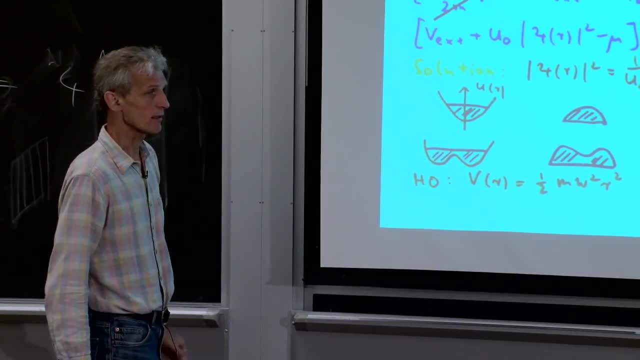 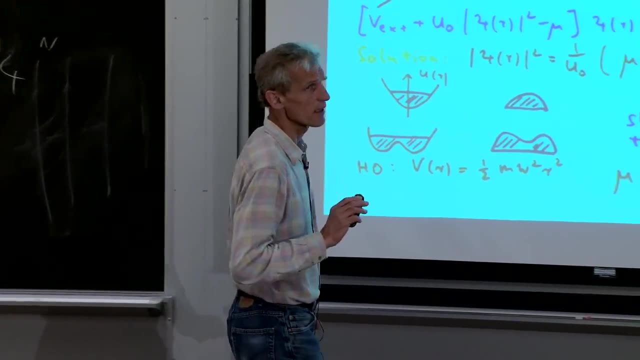 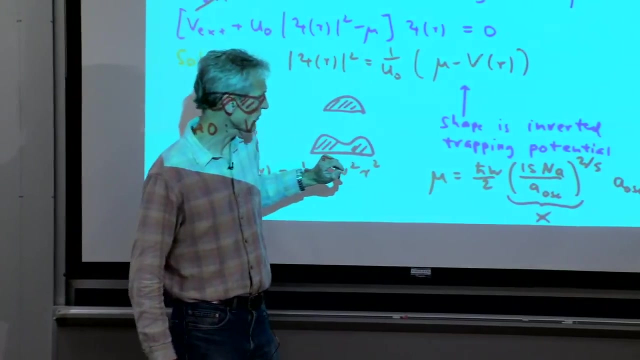 gives you the condensate wave function, the density distribution of the condensate in this potential. I don't want to belabor it. but, coming back to the question of the small parameter, if you look at those equations you can identify a parameter which is now: 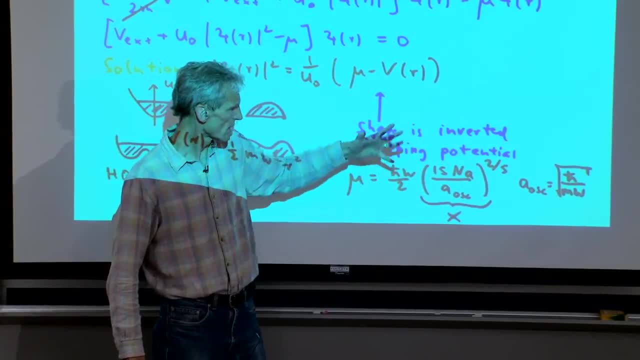 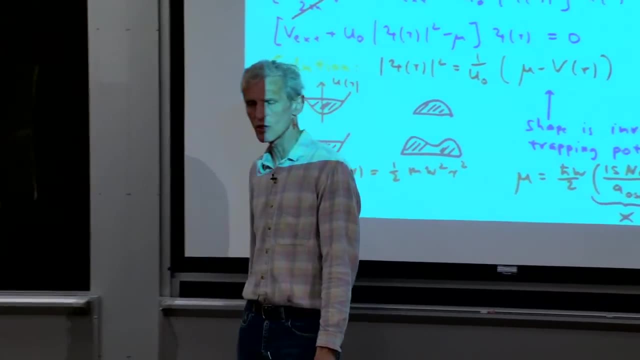 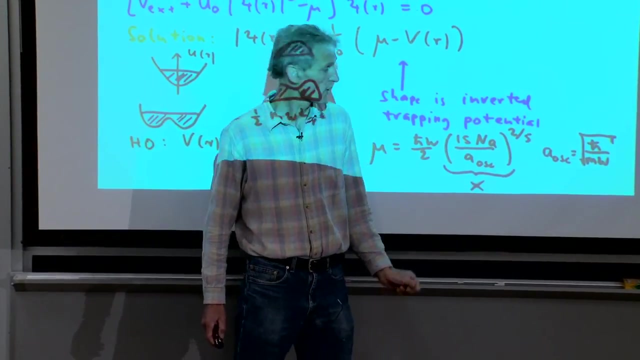 the small parameter or the parameter in the system, which is the important dimensionless parameter. It depends on the number of atoms And it depends now on the ratio of the scattering lengths which characterizes the interaction and the harmonic oscillator links. 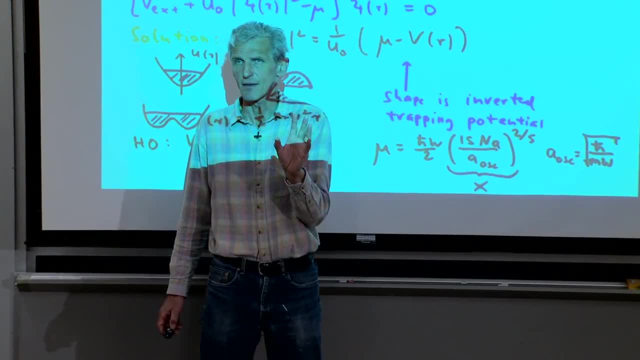 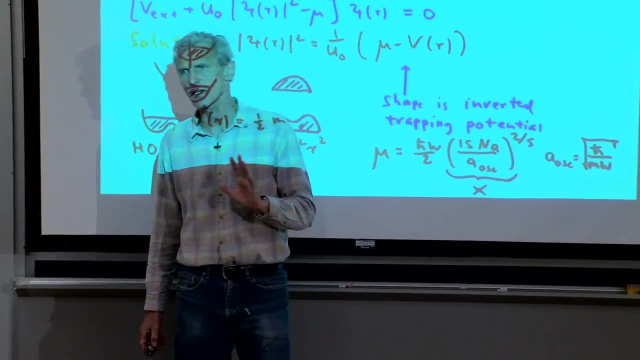 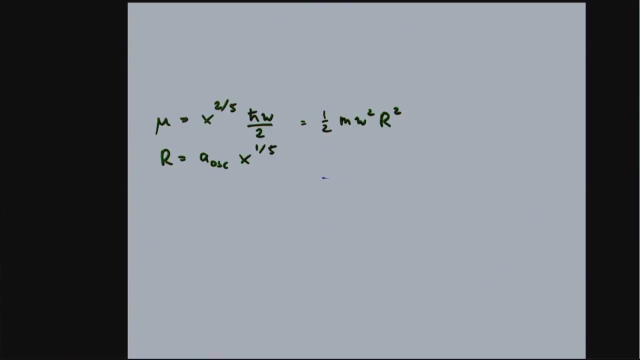 You can say the harmonic oscillator links is the Ideal wave function harmonic oscillator. So this parameterizes the importance of kinetic energy, whereas the scattering length parameterizes the importance of interactions. And all those solutions can be nicely written as what you would have in an ideal gas. 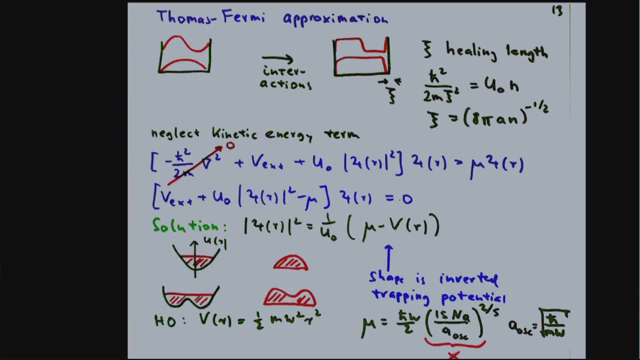 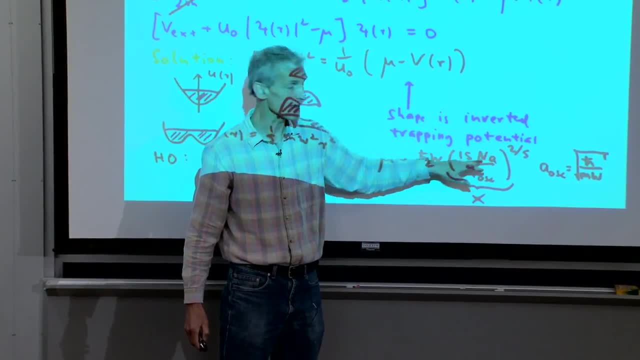 and then this parameter x. So in typical experiments nA, n is a million. The scattering length is smaller than the oscillator length, but n is a million, And this parameter x is usually large. So therefore, and I'm simply just 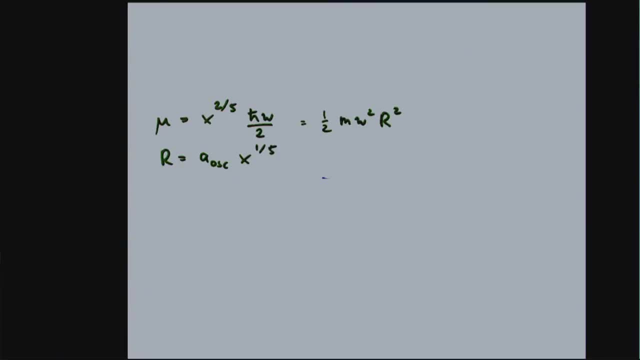 talking about this solution, we have the situation that the chemical potential is larger by a power of x than the ideal gas solution, which would just be the ground state with its zero point energy in the harmonic oscillator potential, Or the width, the size of the wave function. 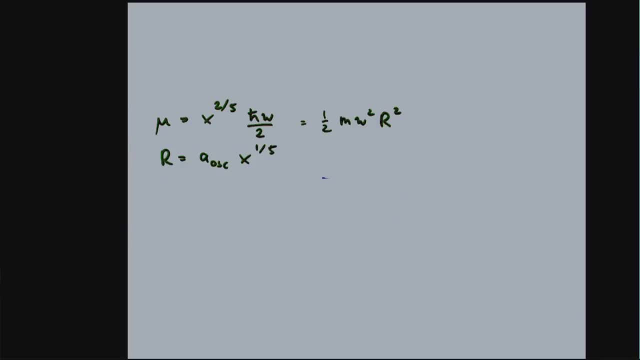 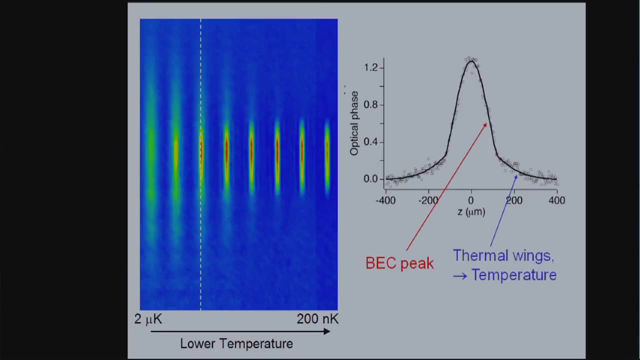 is larger than the ground state of the harmonic oscillator, But only with an exponent which is 1 fifth. Well, we can see that these are now again somewhat improved pictures of condensates inside the trap For the expert. the previous picture. 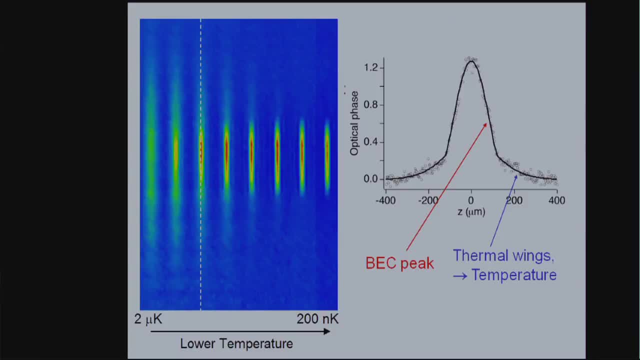 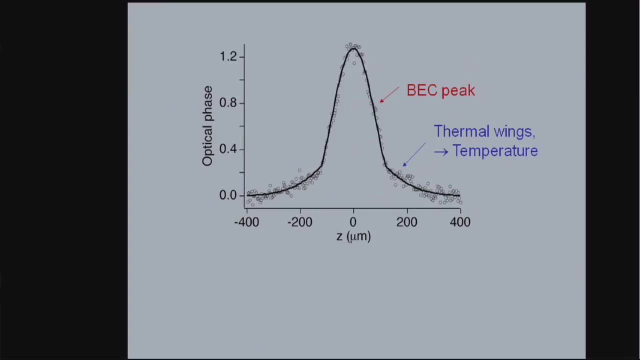 was dark ground imaging. This is now phase contrast imaging And if you take a profile, we clearly see the condensate wave function And we see the thermal wings. When we look at the size of the condensate wave function, you realize what I just meant, that the ground state. 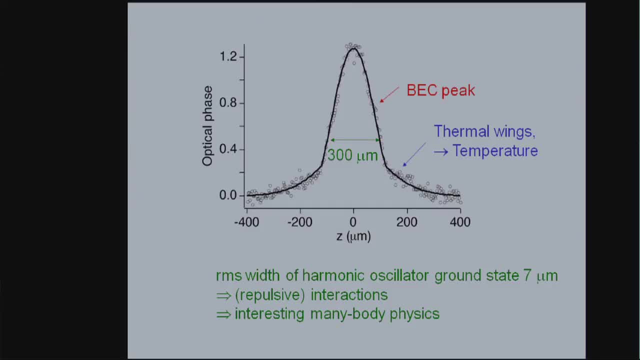 wave function. the harmonic oscillator length is 7 micron in the axial direction, But here we have 300 micron. So this condensate is completely dominated by interactions And it fulfills very nice and pretty much the whole shape, except maybe some details. 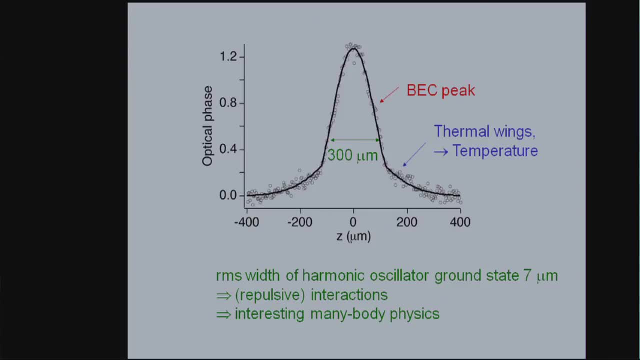 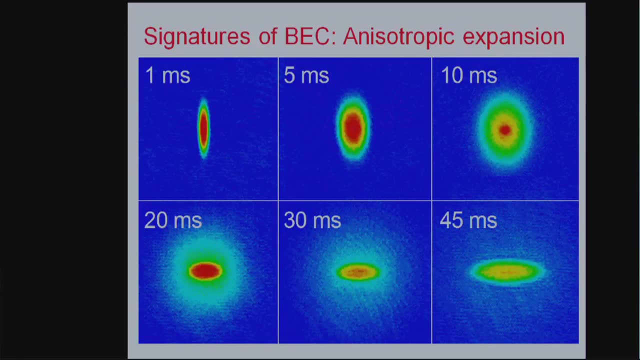 In the wings are quantitatively described by the simple approximation I have explained to you. So just a little bit show and tell. We have this Kros-Pitayevsky equation. The Kros-Pitayevsky equation has, as Schrodinger's equation: 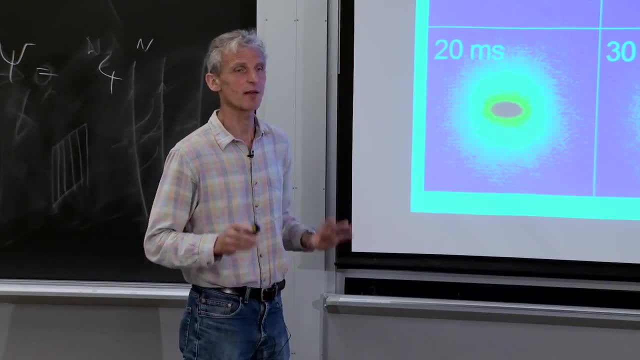 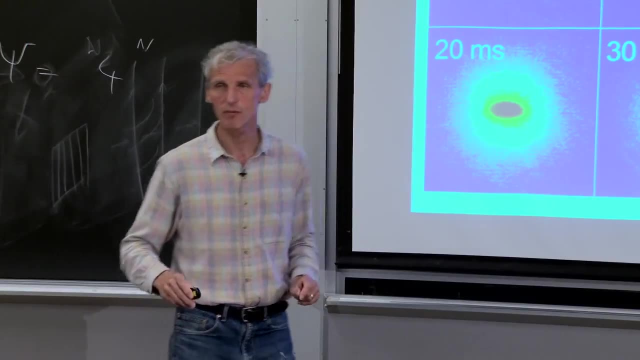 a time-independent form. to get the ground state, It has also a time-dependent form. You simply replace the energy by the derivative of the wave function. This is a time-dependent form. Everything is very simple And you can do many body physics. 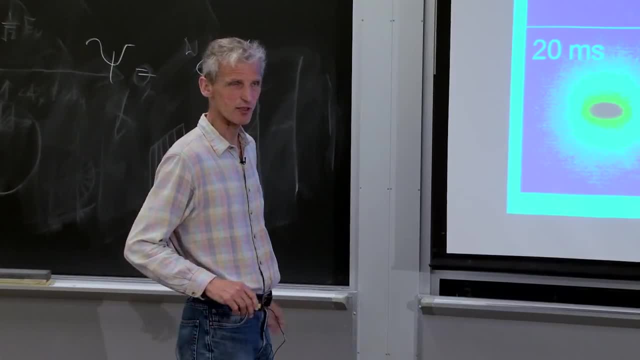 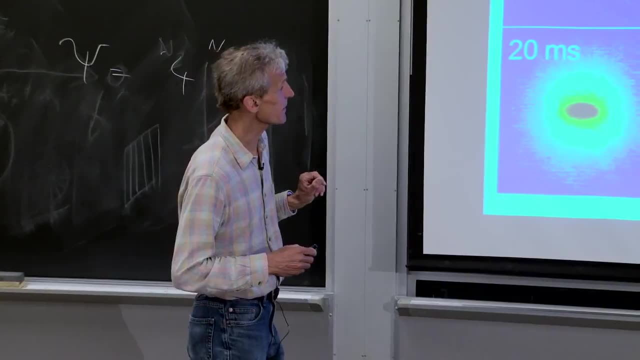 But on your computer you pretty much look for single particle wave function and take them to the power n. So some areas where the Kros-Pitayevsky equation has quantitatively explained experiments- One is the expansion of a Bose-Einstein condensate. 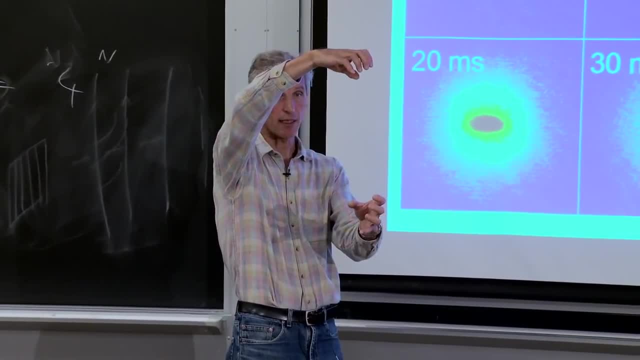 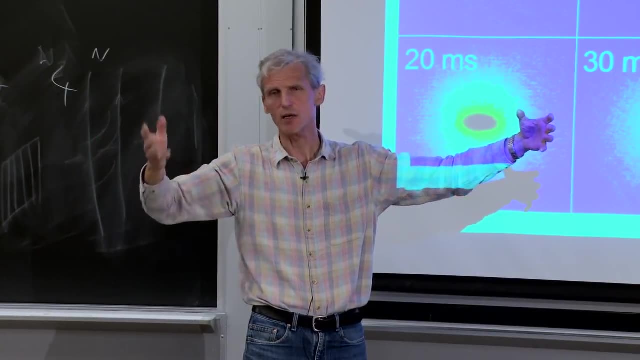 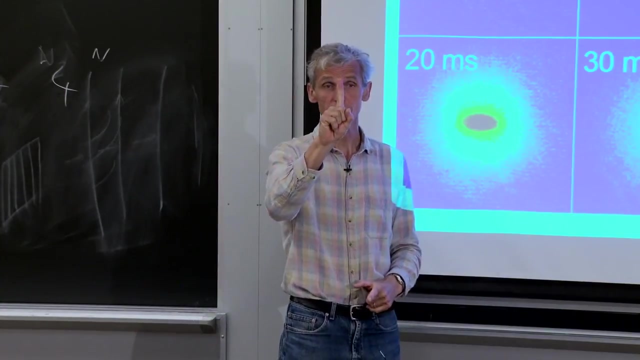 It's this famous situation: when you have an elongated condensate and let it expand, It expands faster in the radial direction. One simple argument is: the pressure of the mean field is larger and leads to a faster acceleration. So therefore, if you have a cigar-shaped condensate, 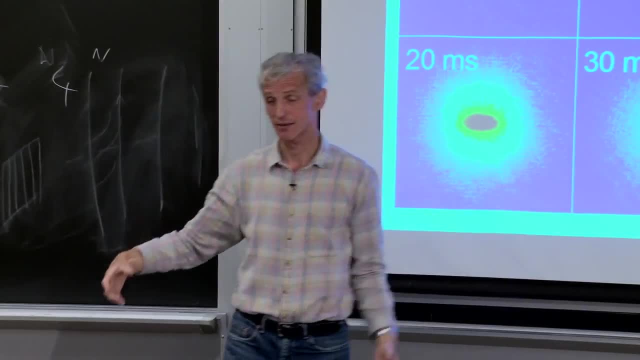 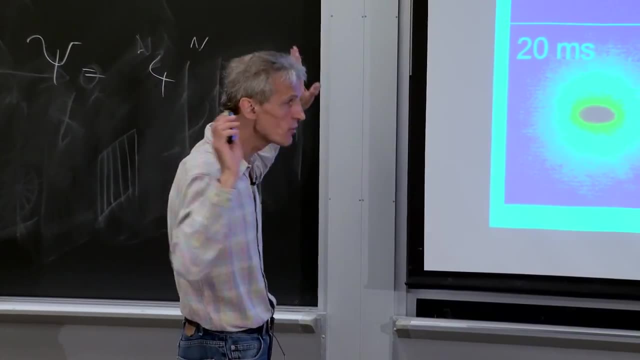 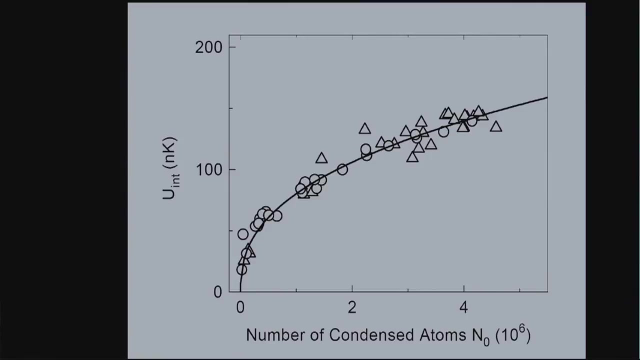 and release it, it turns into a disk. It inverts the aspect ratio, going from a cigar shape to a disk shape, And that has been beautifully and quantitatively described by the Kros-Pitayevsky equation. Here we have measured the interaction energy. 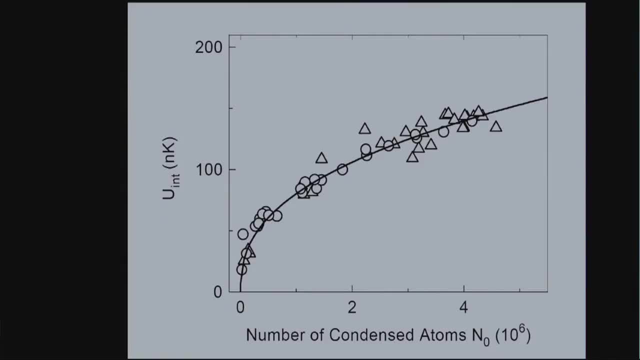 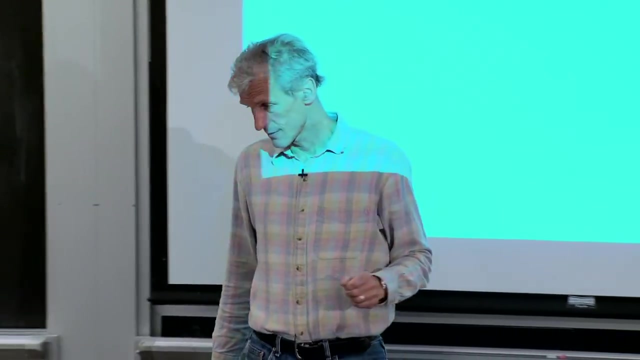 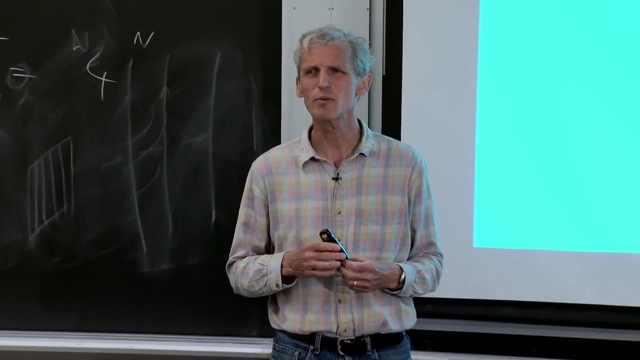 as a number of condensed atoms. And I mentioned to you That this x parameter comes often with powers 1 fifths and 2 fifths, And this here is a fit to the power 2 fifths, beautifully confirming the theory. So the Kros-Pitayevsky equation was invented in 1962,. 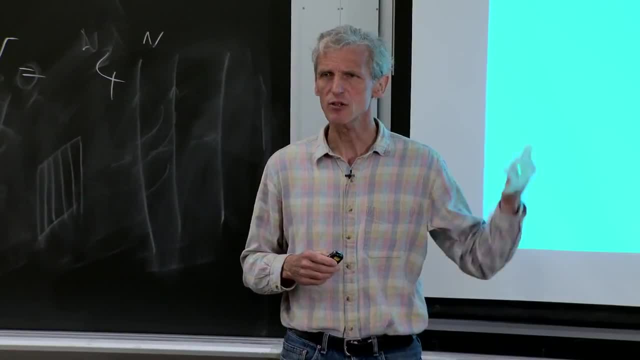 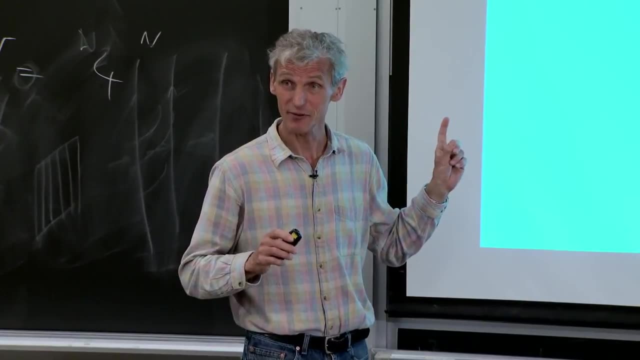 about 50 years ago by Kros and Pitayevsky to describe vortices, Actually Lev-Pitayevsky. Lev-Pitayevsky is still alive, going strong and publishing papers. One of his latest predictions was: 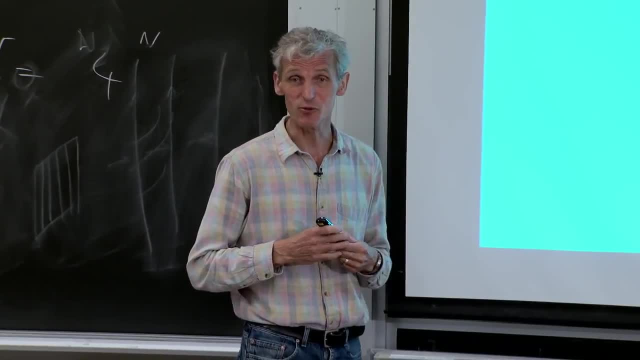 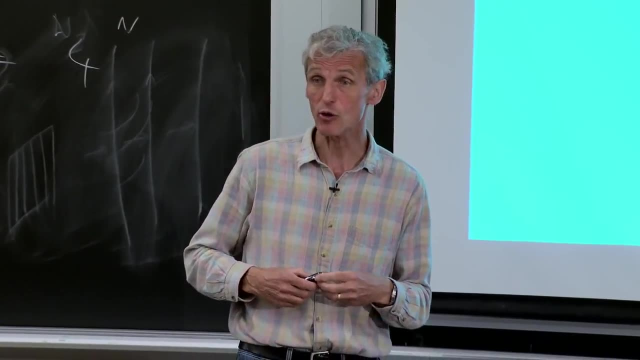 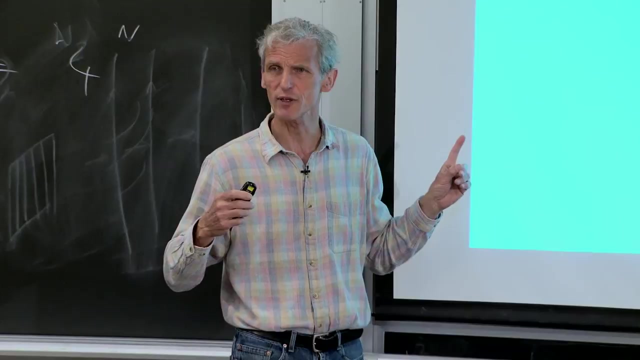 solitons in thermogases And I know in Professor Zwierlein's group one of his lab just looked at the same physics and compared to the theory of Lev-Pitayevsky. And this year we are celebrating- I forgot the 85th or 90th birthday of him. 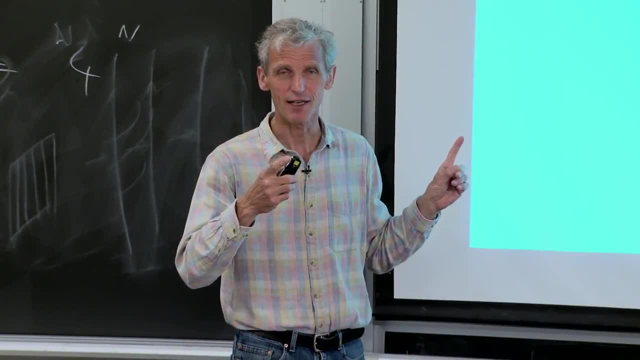 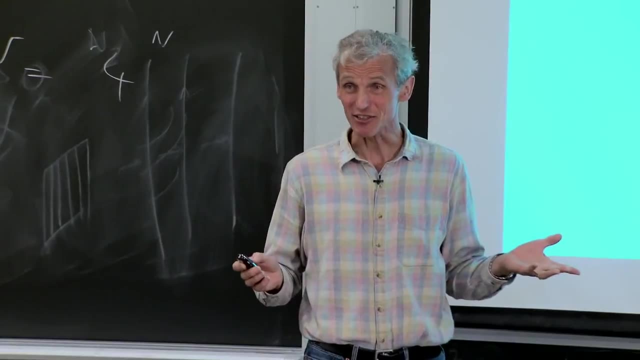 90. Pardon, 80.. 90? On a poster? I know there's a poster next to my door, but I forgot which anniversary. So I mean he's a legend, but he's still walking, He's still doing science. 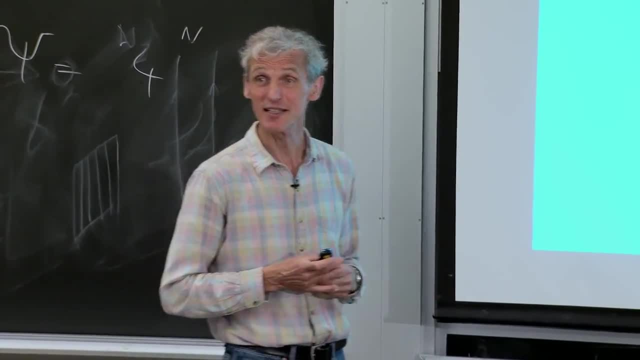 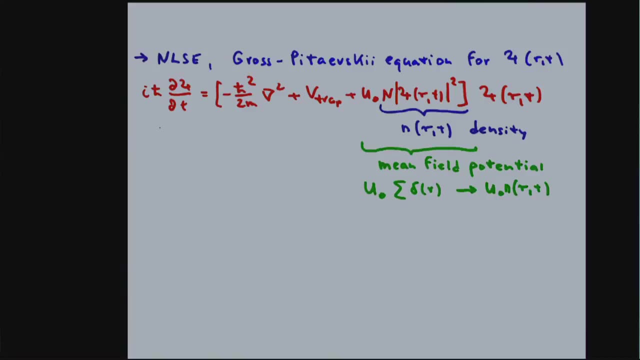 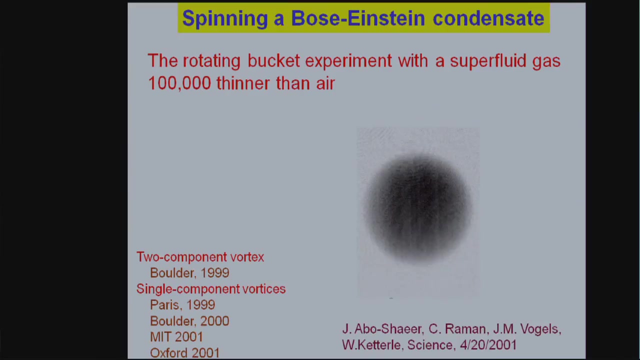 So if you meet him, you go back to 50 years in history. Anyway, it is this Lev-Pitayevsky, and he invented his equations to describe vortices. So anyway, We have this nonlinear Schrodinger equation. 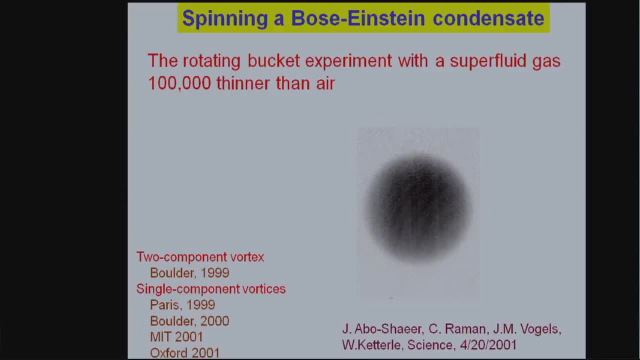 Let me just show you what vortices are and how they are formed. Vortices come if you solve the cross-Pitayevsky equation or if you have ever any quantum fluid or quantum gas and you add angular momentum. The angular momentum cannot lead to rigid body rotation. 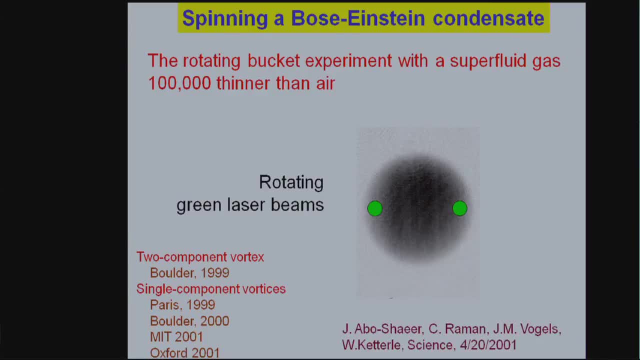 This would violate the fact that the velocity field has to be irrotational to make sure that the phase of the wave function is well-defined. So if you rotate the system, it can absorb angular momentum only by forming vortices, And vortices are singular points of the wave function. 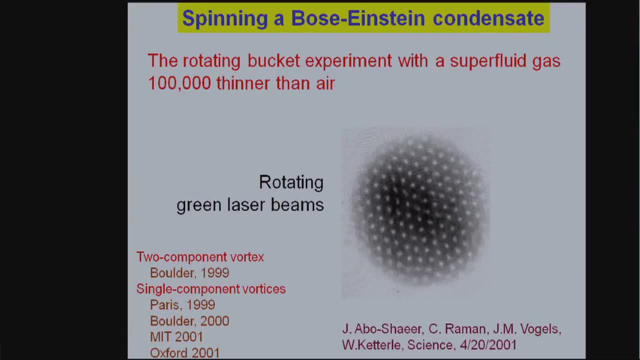 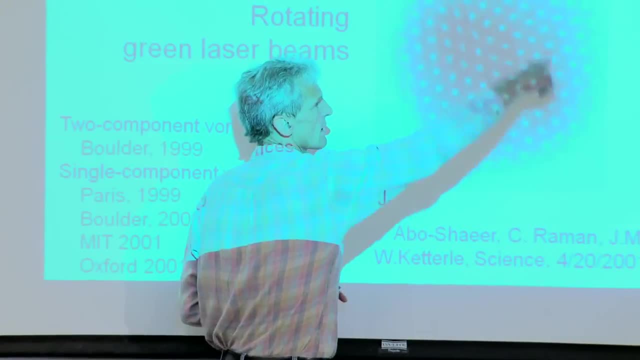 singular points where the density is 0. In other words, I don't have time to be exhaustive here. but when something rotates there is a dynamic phase, you can say, because there are meta waves going in circles And the integral of the phase has. 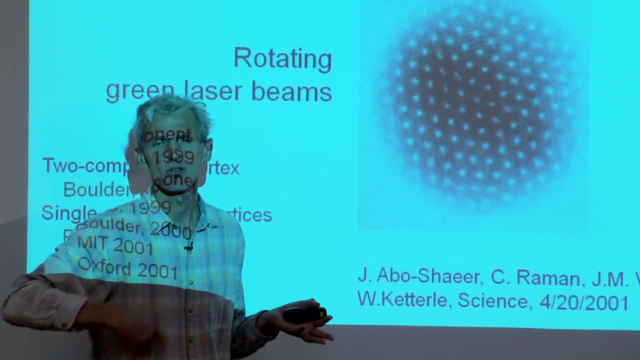 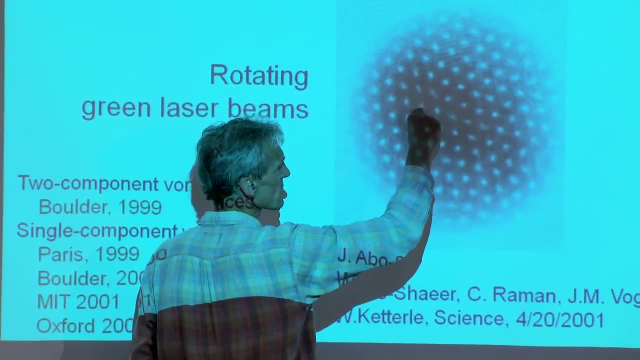 to be an integer number of 2 pi's, Otherwise you would not have a well-defined phase of the wave function. And if you now say you make a circle which is 2 pi, you make the circle smaller, smaller, smaller. 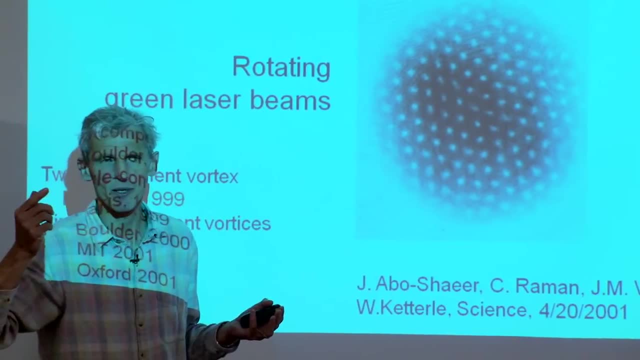 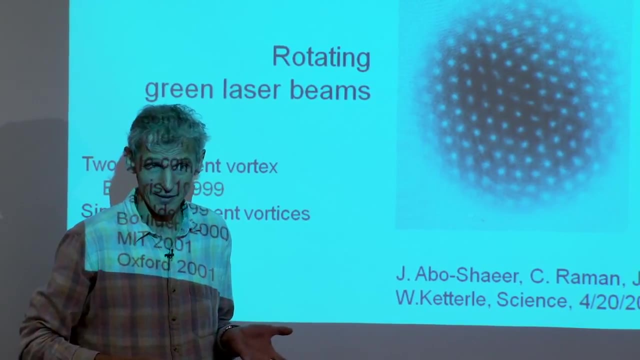 in the middle of the circle you go around, the wave function changes by 2 pi. But what should the wave function do? on one point, Which number between 0 and 2 pi should the wave function pick? Well, the wave function says I can't pick. 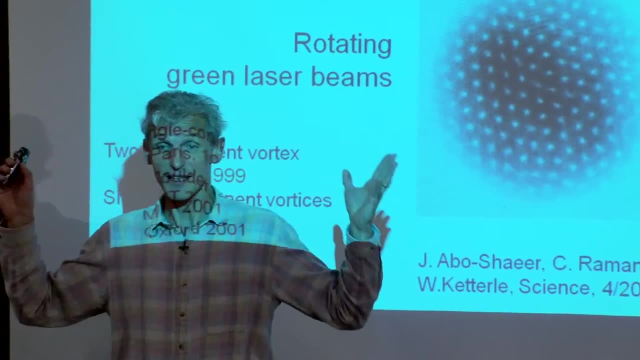 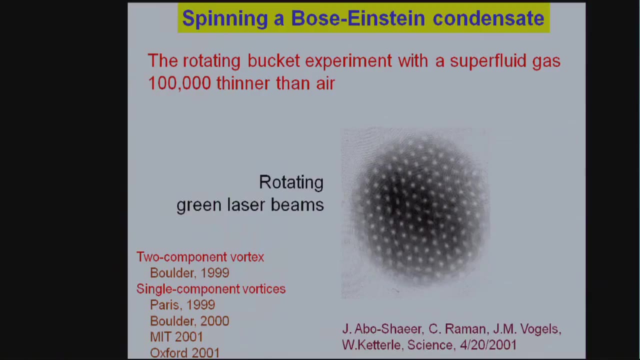 I just go to 0. And a 0 value has no phase, and I'm fine. That's exactly what the wave function tells you. So therefore, if you want to describe vortices, you want to now describe the Kros-Pitayevsky equation. 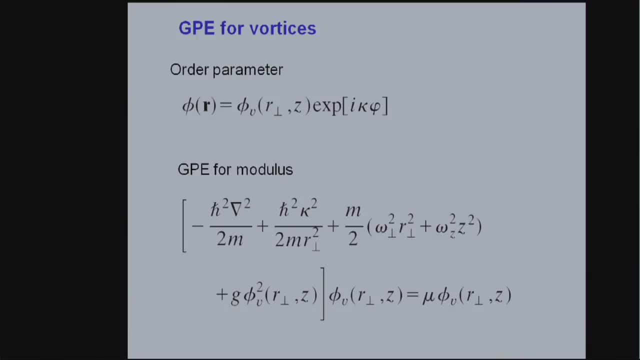 but with the boundary condition that the wave function goes to 0. And if you want to describe one vortex, you want the wave function to go 0 in the center of the cloud, And so you make corresponding ansatz: You allow the phase to wrap around by 2 pi. 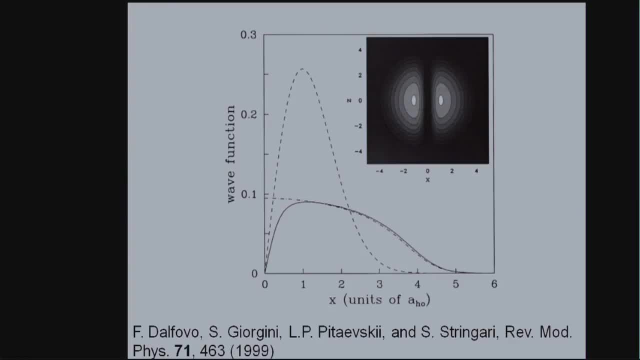 when the angle phi is varied And then when you solve it, you have of course put in that there should be a 0 of the density at the center, And it's now nice for me to. there's an important review paper which describes all that and more. 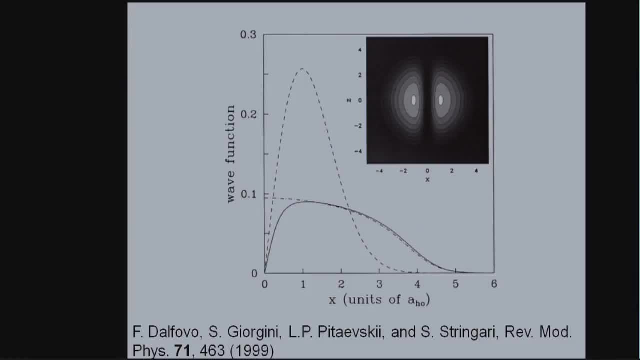 But it's nice to show you now the two extreme cases of the ideal condensate without interaction and the strongly interacting condensate, The ideal condensate. well, we are in the first excited state of the harmonic oscillator potential And this is the dashed line. 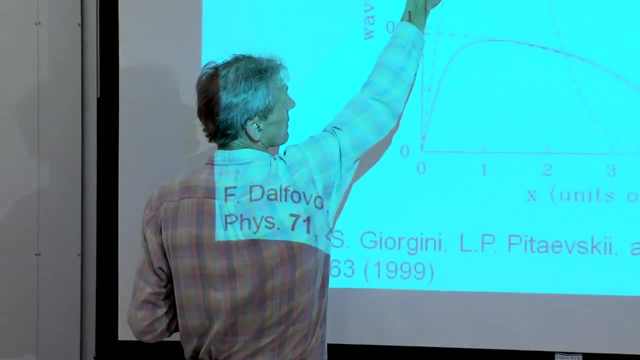 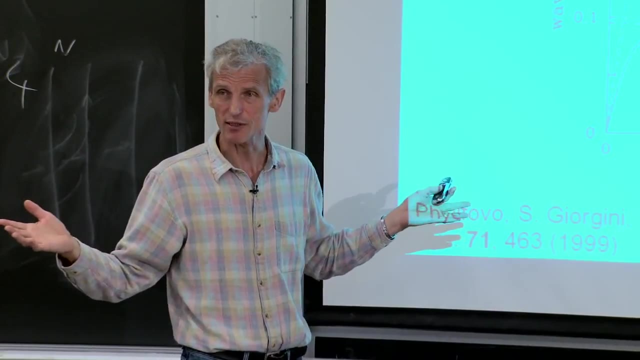 And of course the size of the hole, the 0, is pretty much on the order of the oscillator length, because there is no other length scale in an ideal harmonic oscillator. But if you have the interacting system, remember what interactions are doing. 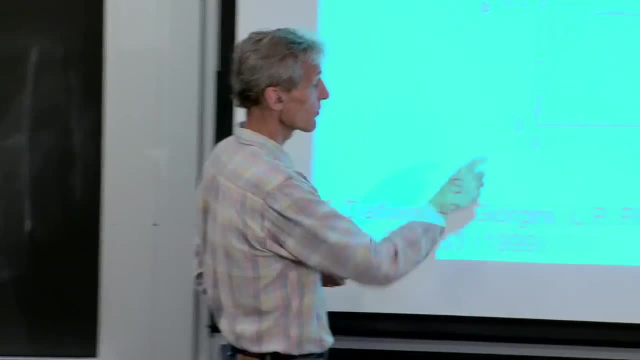 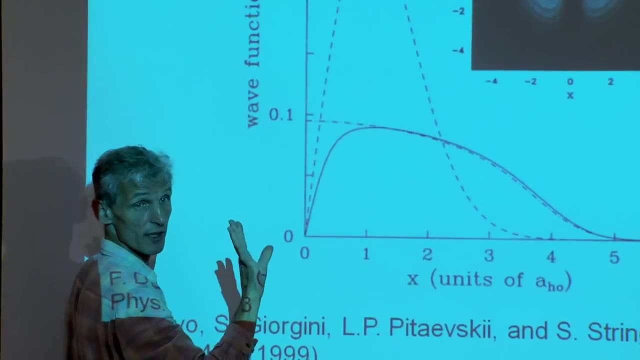 They want to keep the density as constant as possible. Well, we are not in a box potential, We are in inverted parabola potential. And remember our Thomas Fermi solution, which neglects kinetic energy, is the inverted parabola. 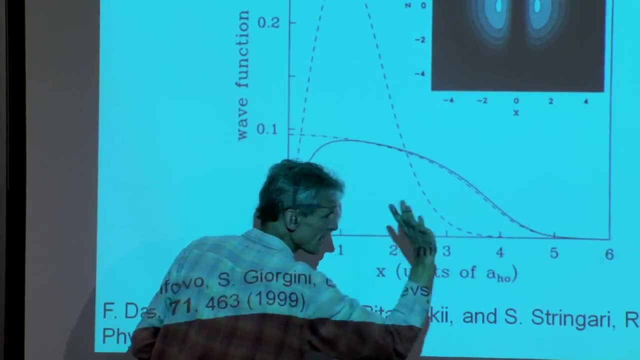 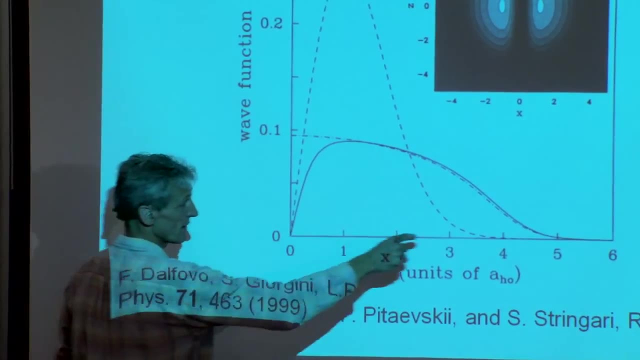 up to here, And then the tail is when we can no longer neglect the kinetic energy. But if we now say, OK, fine, But now in addition we want a vortex in the center, the wave function out there says no. 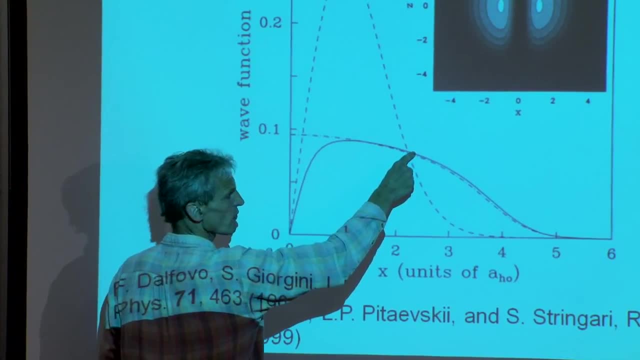 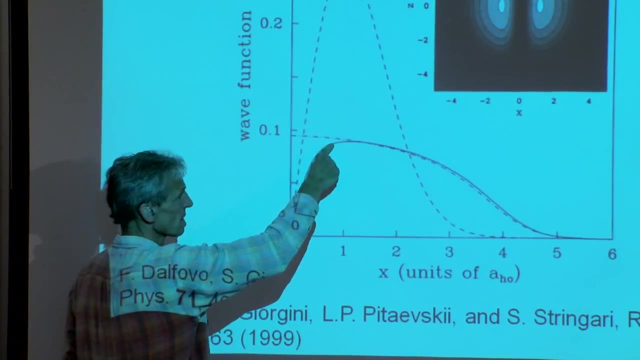 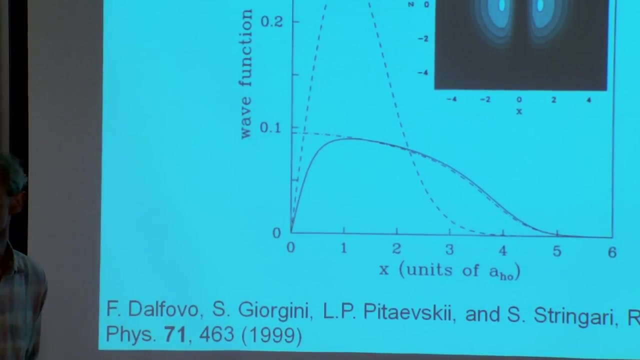 We do what minimizes kinetic energy and what minimizes repulsive energy. We follow the inverted parabola And only at the very last moment, on the scale of the healing lengths, the system meets the required boundary condition that the density goes to 0.. 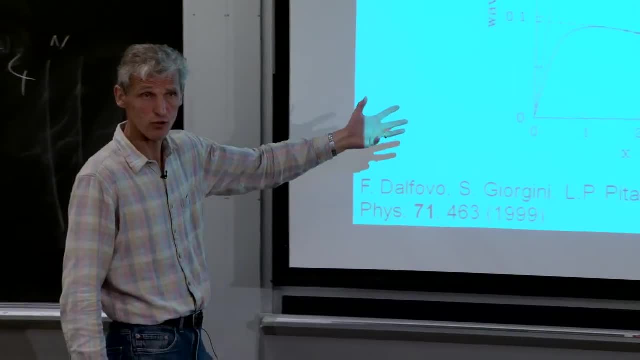 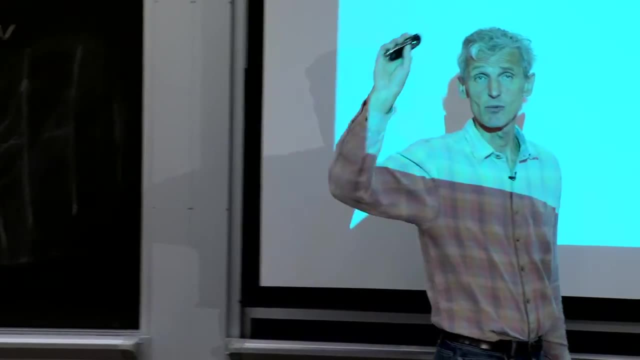 Anyway, with this qualitative understanding, you can get a lot out of those. You can immediately understand the salient feature of this solution. Timo, I know we're not talking details. Is there a simple, maybe intuitive, reason why, when you spin a cosine-sine constant? 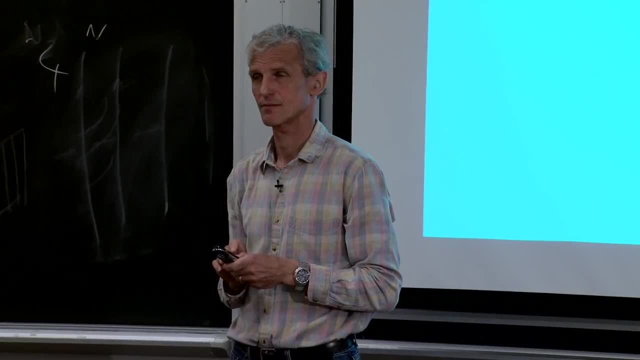 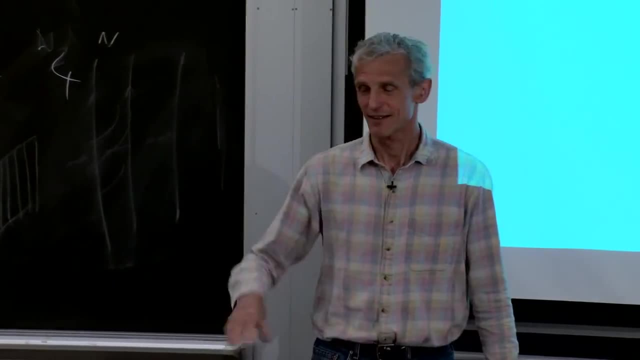 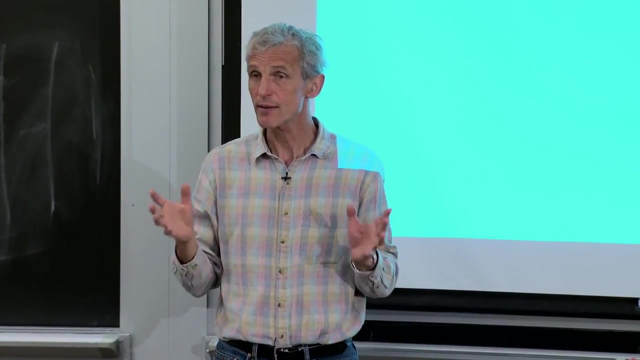 you get many vortices, but when you spin your coffee in your cup, you just get one big one. Yes, OK. So the question is, if I have a wraparound of 4 pi in phase, whether the system should have a doubly charged vortex. 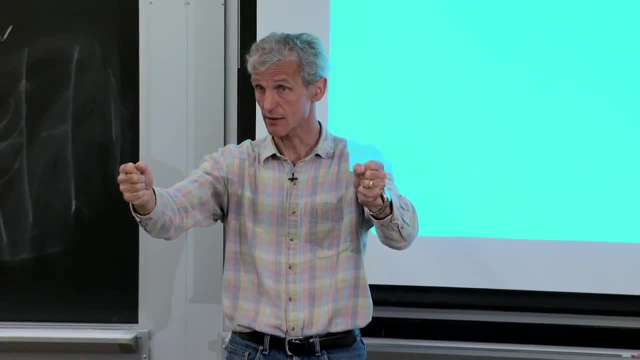 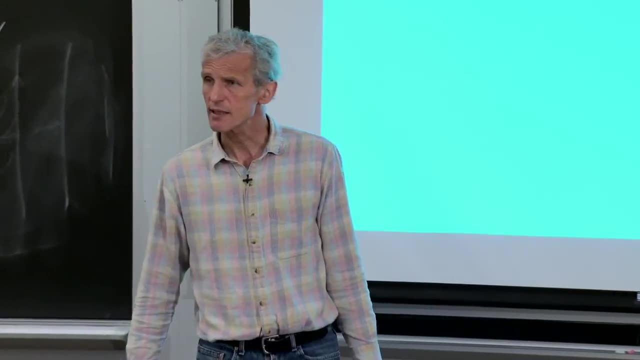 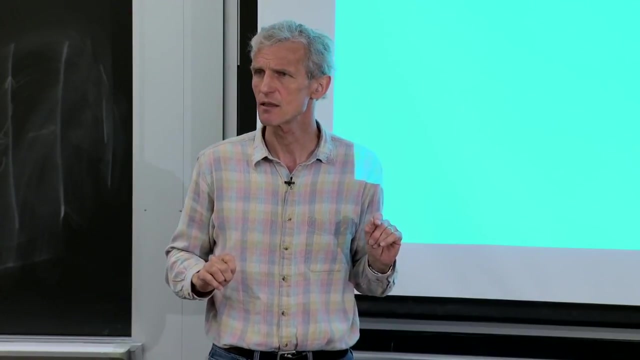 or two singly charged vortices. What is the difference in energy? Well, what happens is doubly charged vortices are unstable. My group, at some point, were the first to create doubly charged vortices, but we saw that they immediately decayed. Pun. Initially we couldn't observe. We just saw that it was unstable. But it's a decay into two vortices. But it's easy to understand: If you put two vortices on top of each other, what is the energy of the system compared to one vortex? 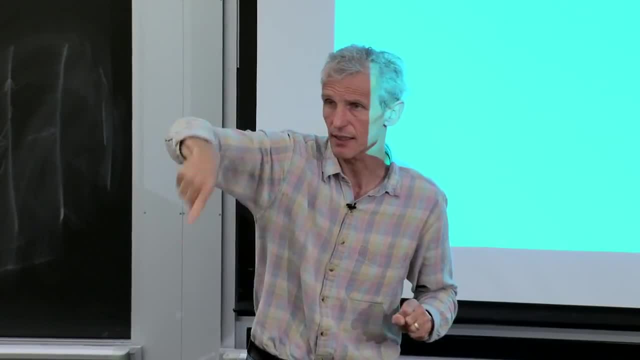 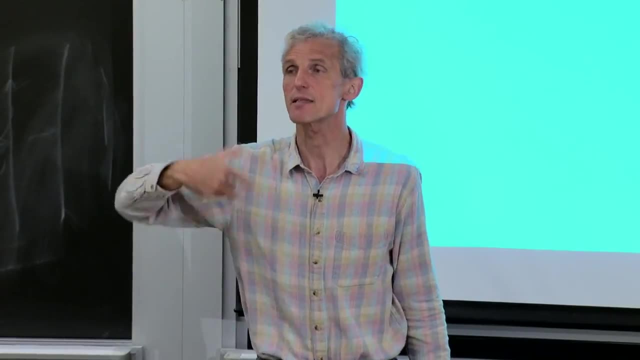 Well, the energy of a vortex is the rotation. There's a rotational field around it And if you superimpose two vortices, the velocity around the doubly charged vortices is twice the velocity of one vortex And therefore the kinetic energy is four times. 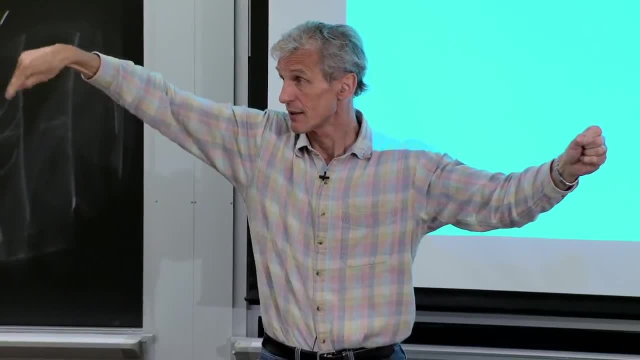 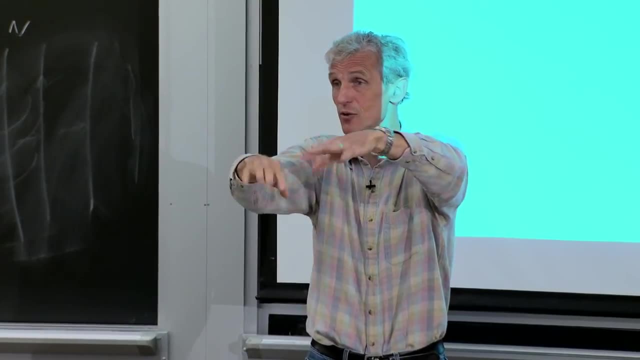 If you have two vortices which are far separated, that it has its own velocity field. It has its own velocity field here, And when the two velocity fields come together, the velocity is already so low that you don't have to consider that. 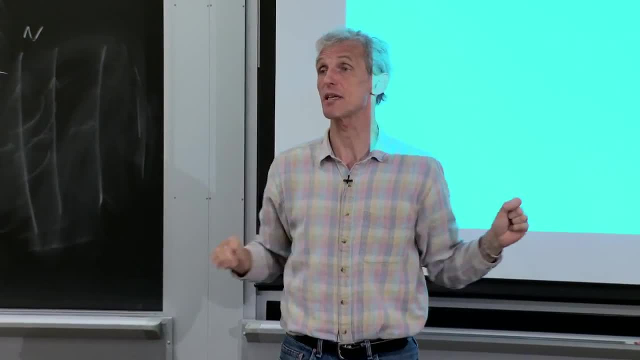 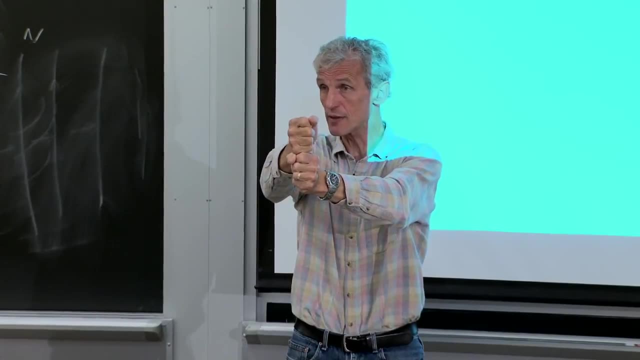 Then those two vortices. These have an energy which is two times the energy of a single vortex. So therefore, when the two vortices, they start out with four times the energy of a single vortex, And when they dissociate and repel each other. 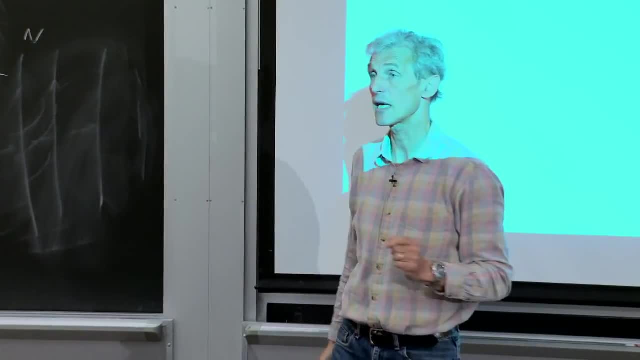 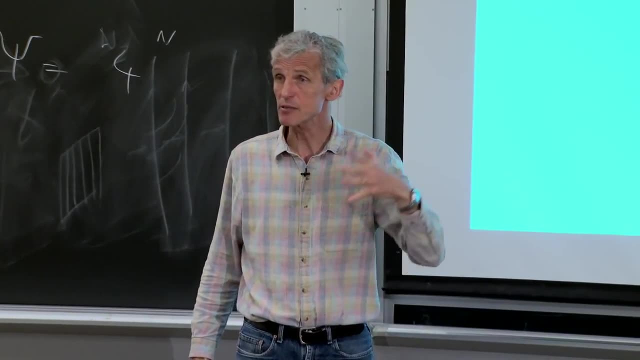 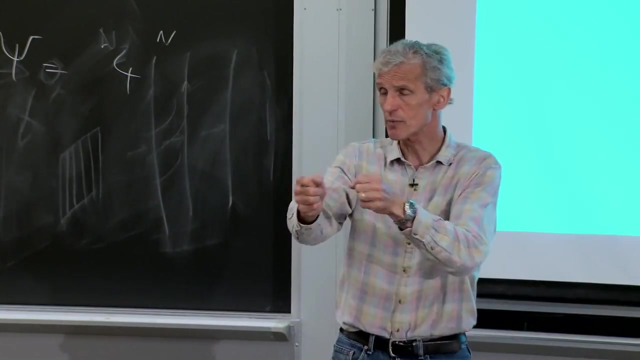 they have shaded half of the energy. So this argument tells you immediately that vortices are in effect repulsive And therefore any multiple charged vortex will spontaneously decay. It's also this net repulsion between vortices which makes the vortices arrange in a regular lattice. 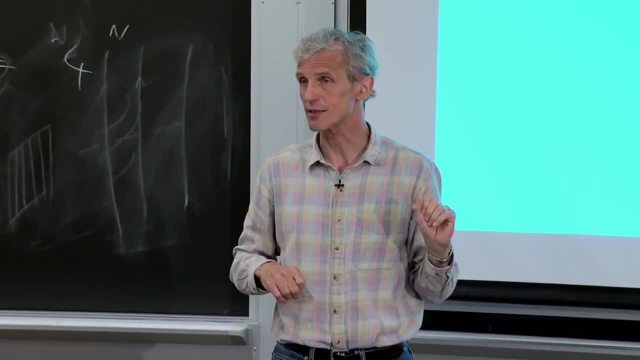 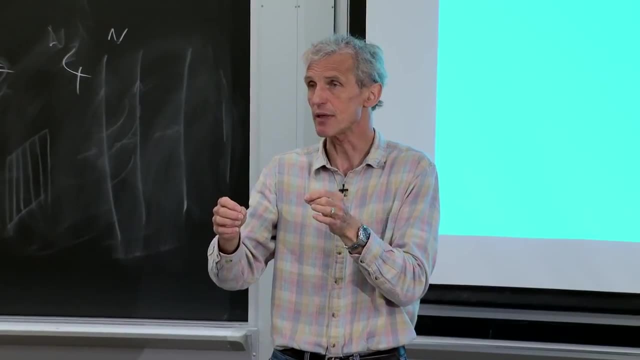 The regular lattice which you saw before is nature's answer to how can we minimize the energy of all those vortices, And the idea is let's keep the average distance between them as large as possible, And the answer is a hexagonal lattice. 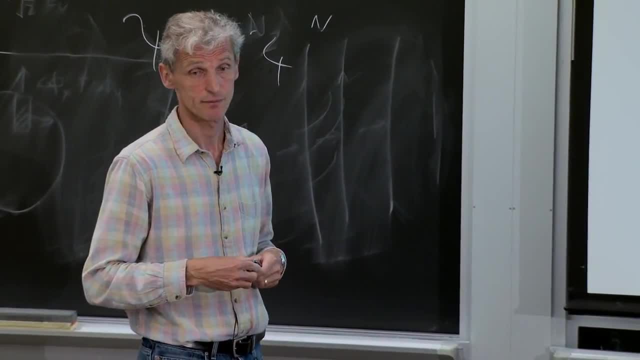 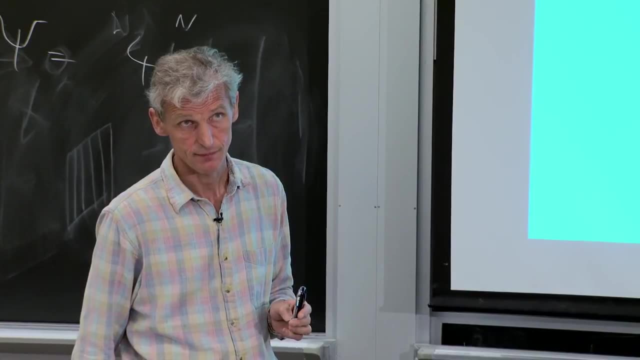 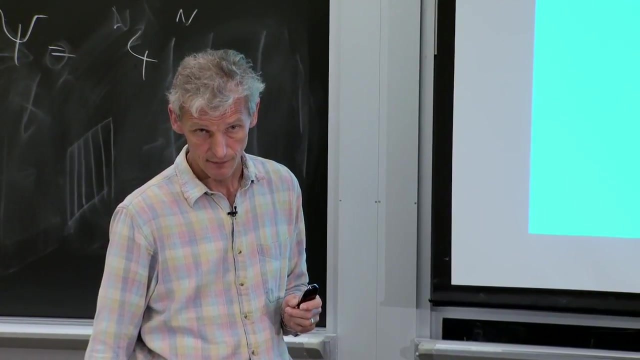 Matt. So a few slides back. you plotted sort of we arrived at the GP equation And you plotted for the box potential, the ground state, the first excited state, comparing the GP equation to the typical single particle solution. And so I guess I'm a little bit confused. 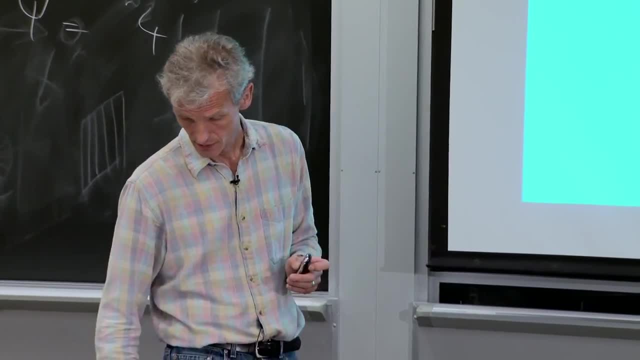 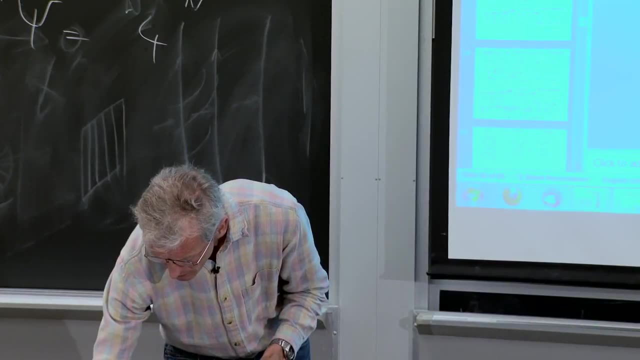 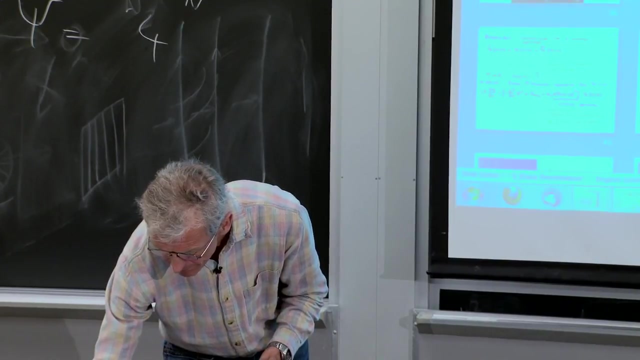 about how excitations manifest themselves in a system. Because in some sense, if you were to solve the GP equation then would you arrive at, say, a spectrum of solutions And I guess I'd be confused whether the excitation manifests itself into that spectrum of solutions. 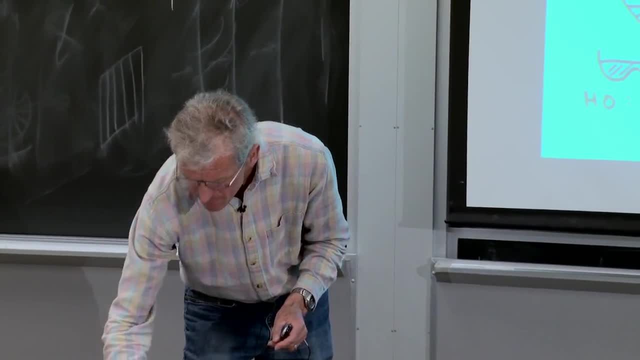 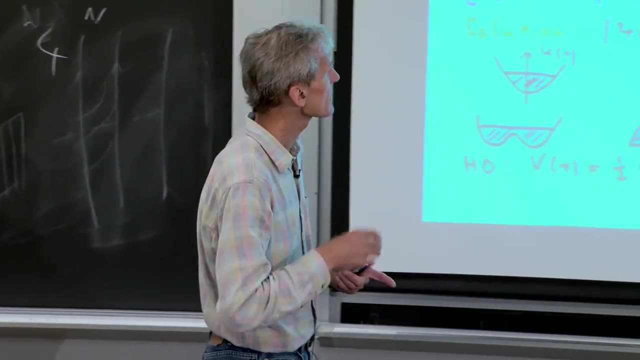 or rather than they become excitations like sort of deviations from the mean field. as you know, including the extra Matt, you're now asking about something more complicated. You're asking what are the excited states of the many-body system? 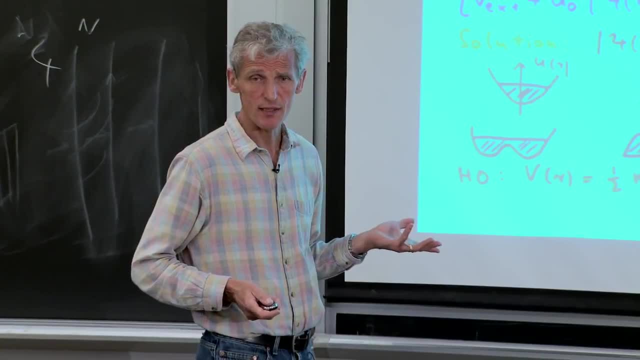 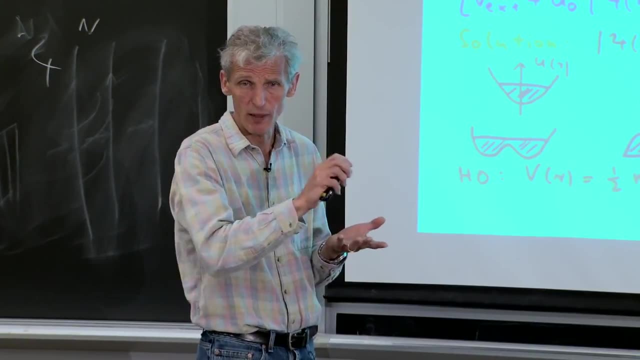 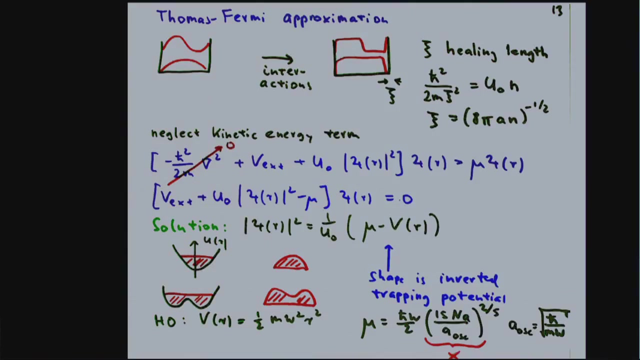 And actually we have already found one answer, And this is, if you want this, small excitations. it's: one particle becomes a phonon or one particle becomes a quasi-particle. What we are talking about here is what happens if the whole macroscopic wave function. 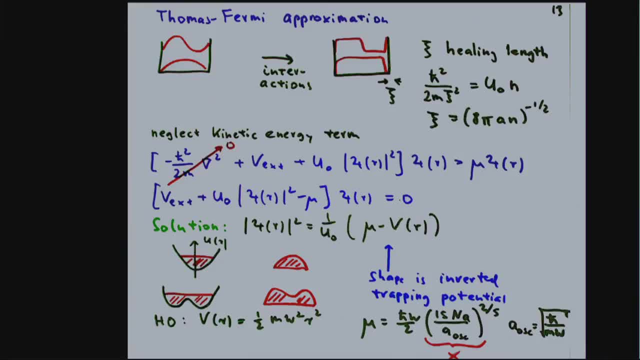 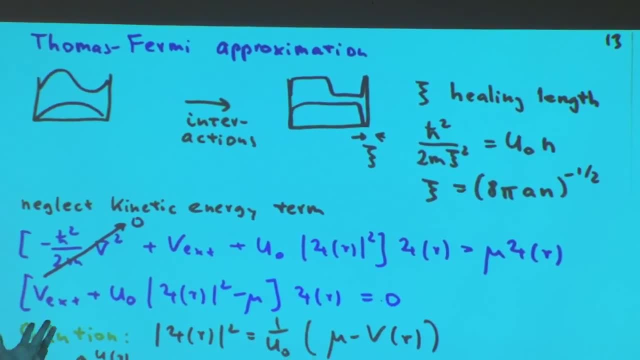 is in an excited state. So we are asking here in the box potential what happens if we force all n atoms to have one node in the wave function, And this is what I'm talking about here, So the excitation energy of this state. 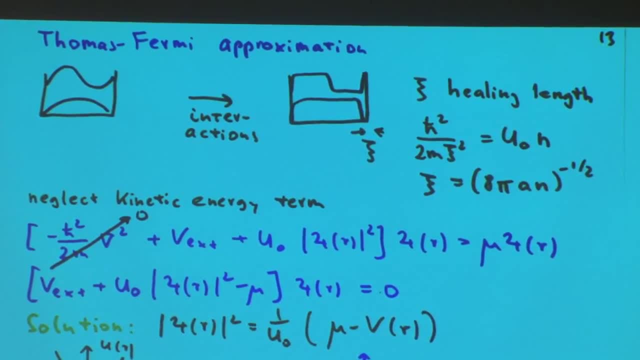 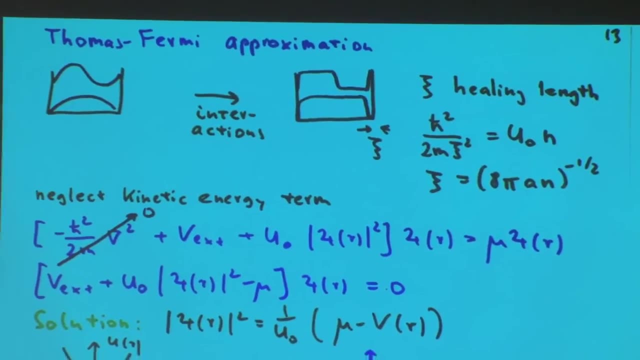 here is much, much higher than of single quasi-particle excitations. I'm not sure if I'm addressing that. I'm not addressing your question here, but So with single quasi-particle excitations are those essentially sort of deviations in the mean field? 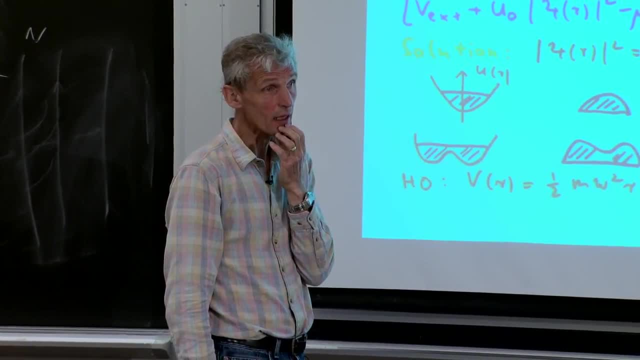 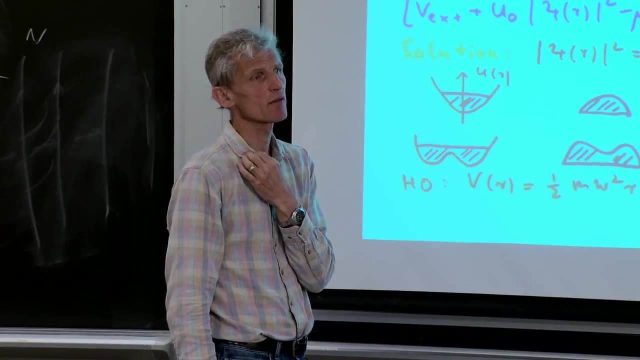 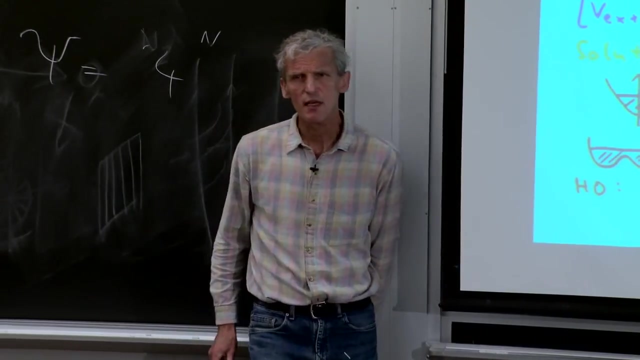 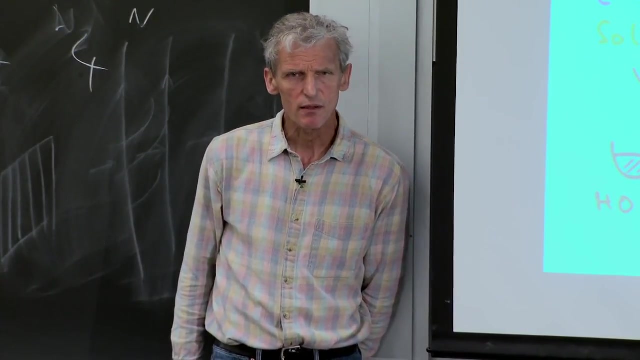 Yeah, because you know. No, they are. You really look for many-body. physics mean field deviations probably. what you do is in that sense: yes, You're allowing in this answer that psi operator is psi average plus fluctuations. 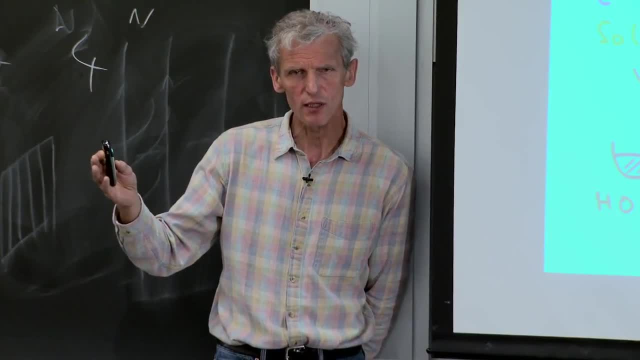 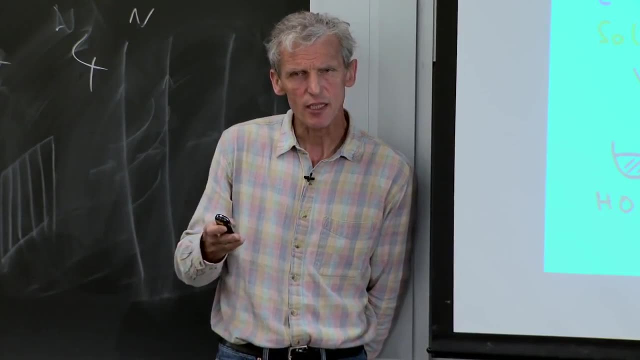 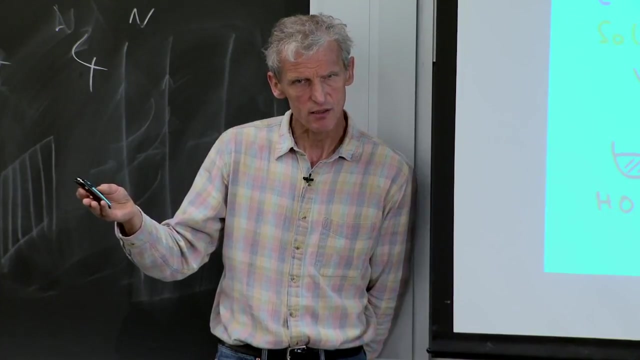 You now look for fluctuations and you're looking for the energy eigen spectrum of those fluctuations And the answer are quasi-particles. So it is actually the solution for the spectrum of the fluctuations And the answer is the dispersion relation I presented to you. 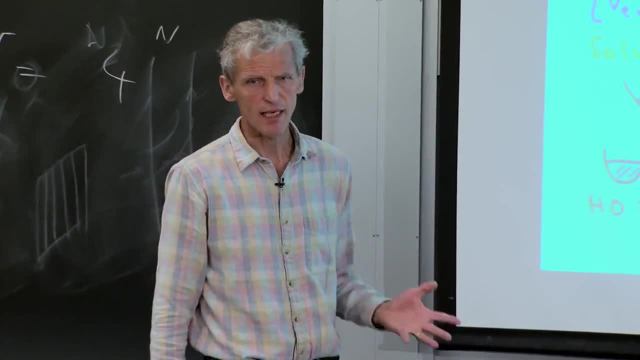 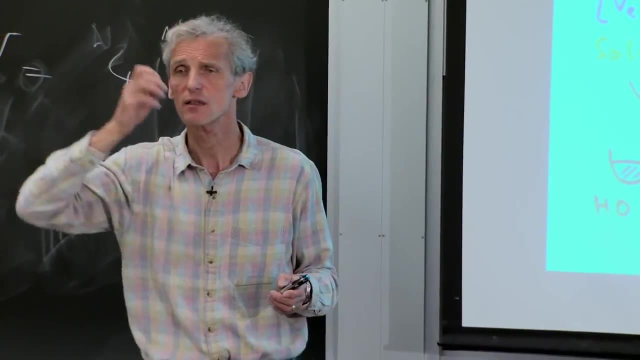 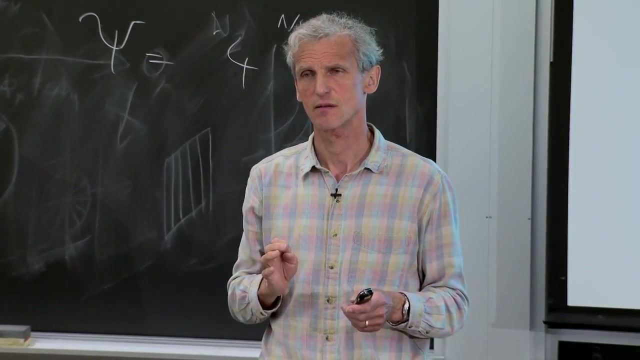 Whereas here we are asking what are excited states of the macroscopic wave function? It's a very, very different question which we have addressed here, Colin. So when you stir the condensate, do you view it as do you stir, sort of, at the trap frequency? 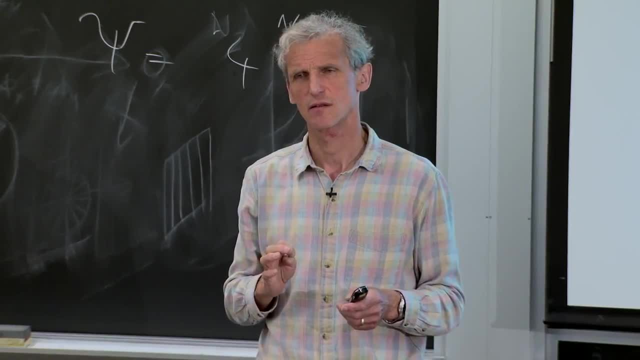 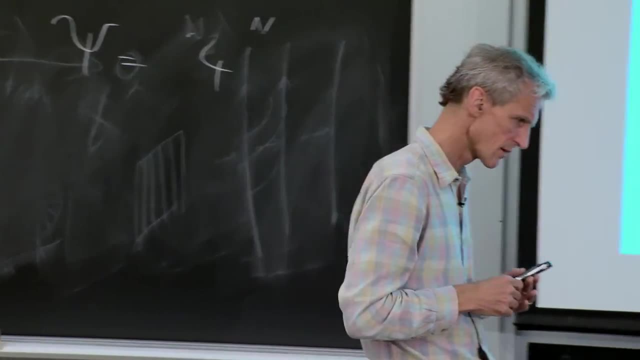 So I do sort of n single excitations, Or do you stir at n times the trap frequencies? You do 1.. You do sort of n particle excitations. Well, the experimental answer is: you want to stir at the quadrupole frequency, which? 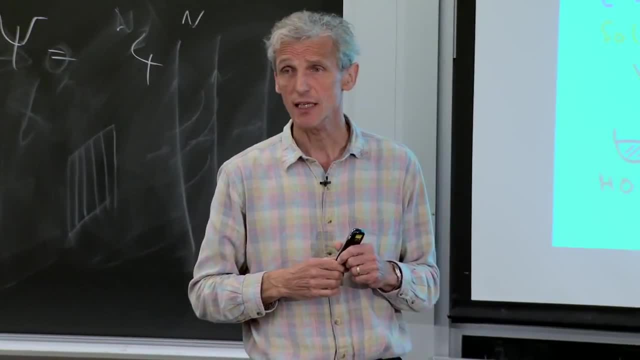 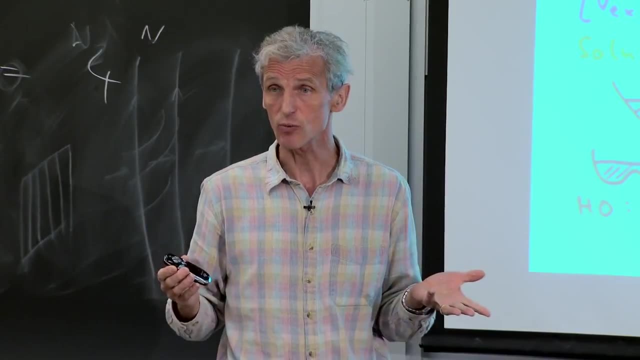 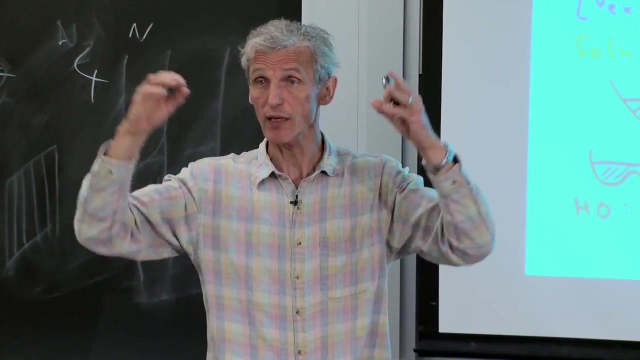 is square root, 2 times the trap frequency. Then you create quadrupolar excitations. The quadrupolar excitation can be regarded as a standing sound wave, But you create a macroscopic number of those excitations, So you make actually the whole condensate wave function. 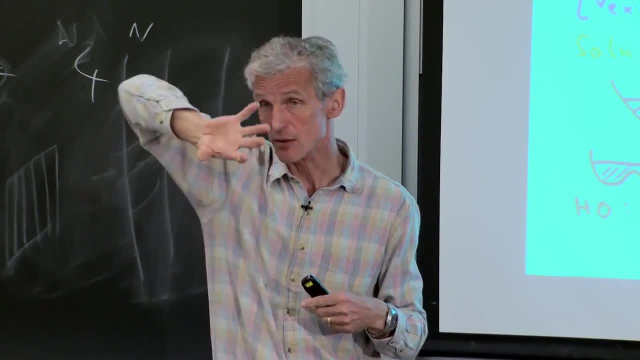 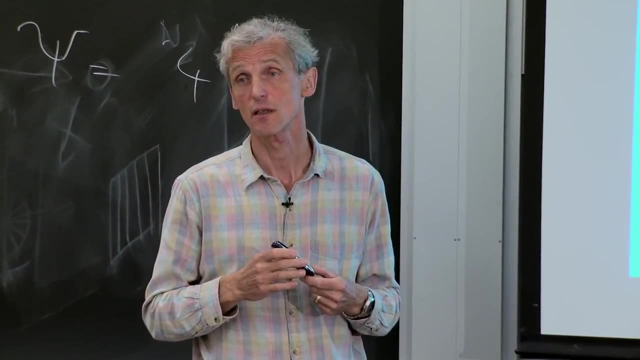 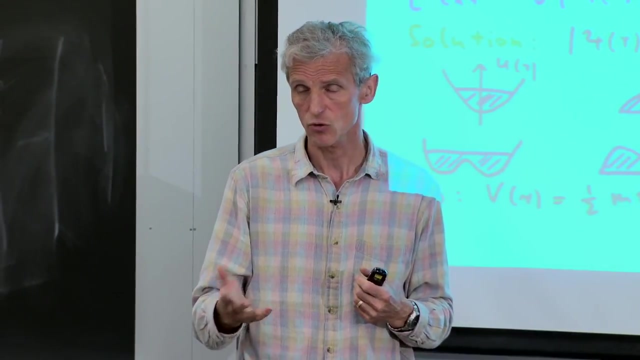 oscillate in a quadrupolar pattern, But it's a rotating quadrupolar And that eventually then rearranges itself and leads to vortices. So I think the correct answer is the most efficient way to create vortices would be to excite quasi-particles. 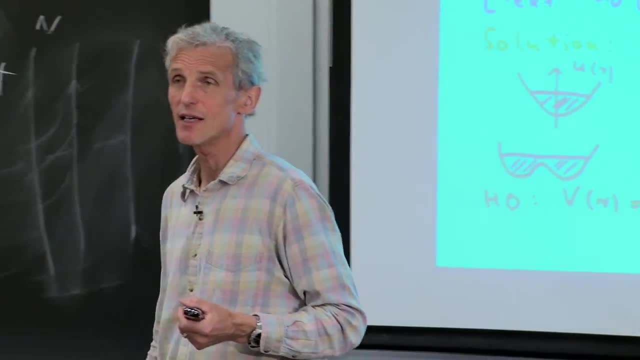 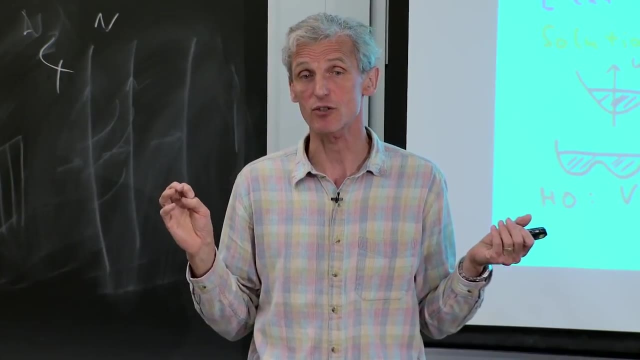 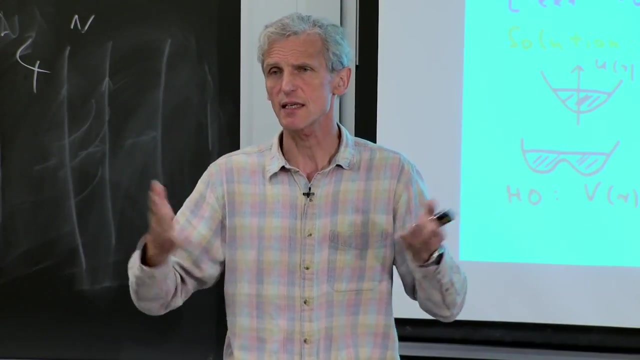 but then excite so many- and this may relate to Matt's question- create so many quasi-particles that you have really a time-dependent and oscillating macroscopic wave function. So eventually you have a coherent excitation of quasi-particles and that eventually 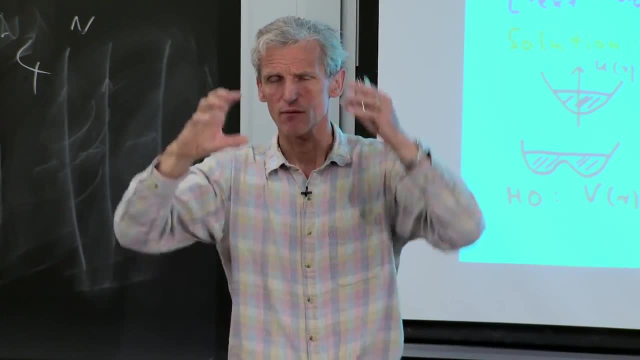 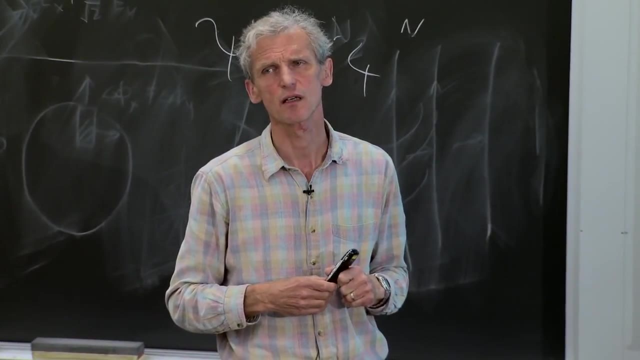 means the condensate moves in a quadrupolar pattern, But it's a quadrupolar pattern with rotation and that eventually turns into many vortices. But that's a really very rich question which you're asking, which has been studied. 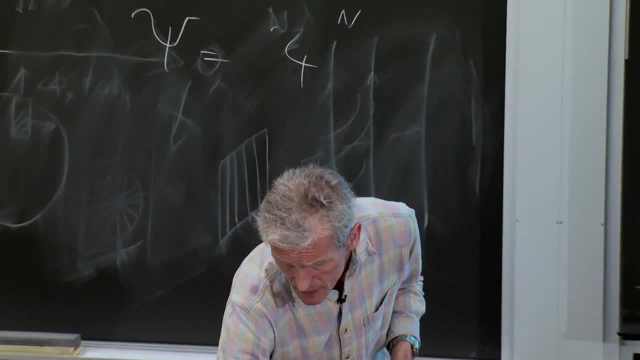 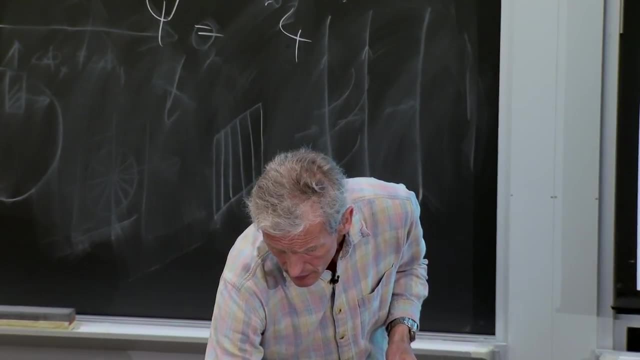 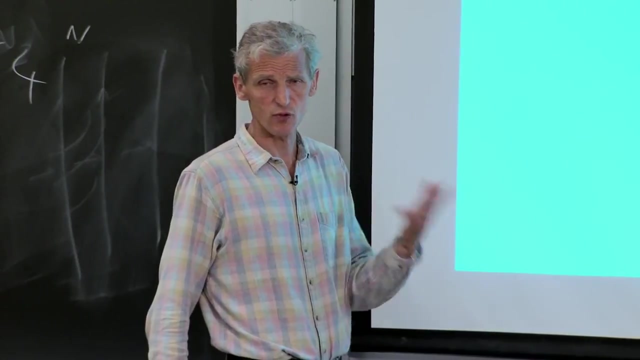 in. a lot of different aspects of that have been studied. OK, So we've talked about Bose-Einstein condensates in a homogeneous system, just to lay the groundwork. We've talked about Bose-Einstein condensates in traps in inhomogeneous system. 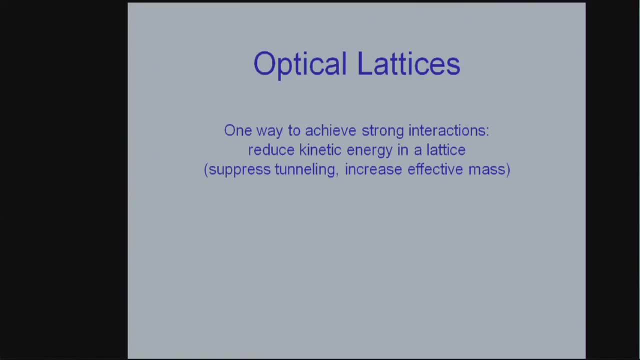 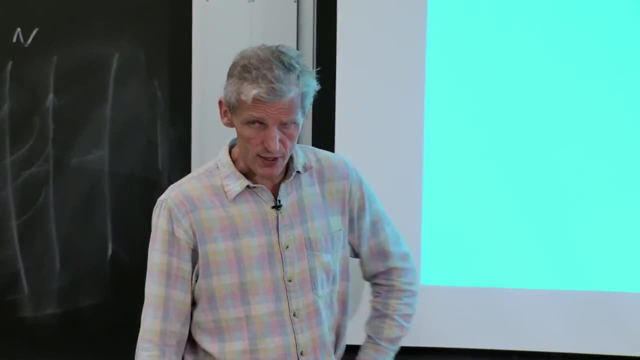 Now we want to talk about Bose-Einstein condensates in optical lattices. Well, there are two reasons why we want to do that. One is we want to use the Bose-Einstein condensate. We want to use the Bose-Einstein condensate. 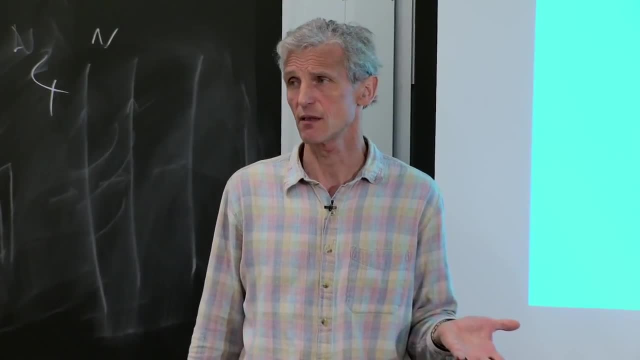 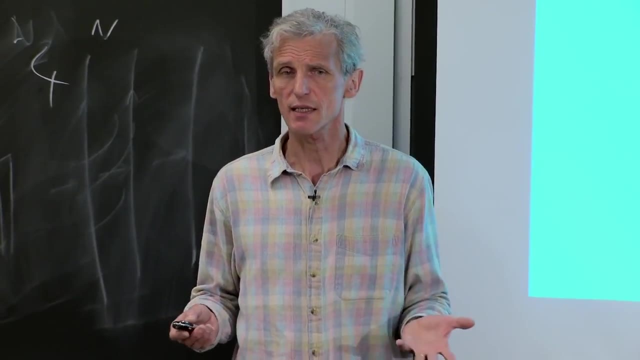 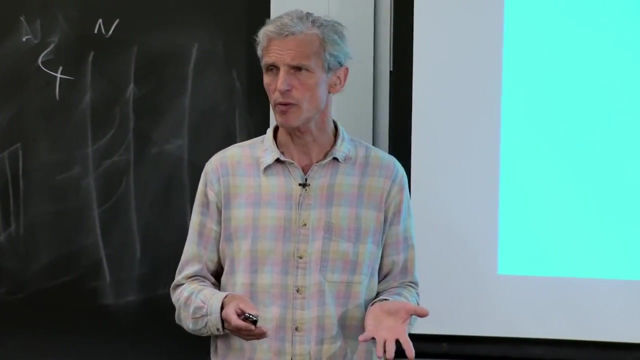 to obtain deeper insight into the properties of matter, And a lot of forms of matter appear in periodic lattices. So if you put a Bose-Einstein condensate into a periodic potential, we can at least understand some of the properties of crystalline matter. 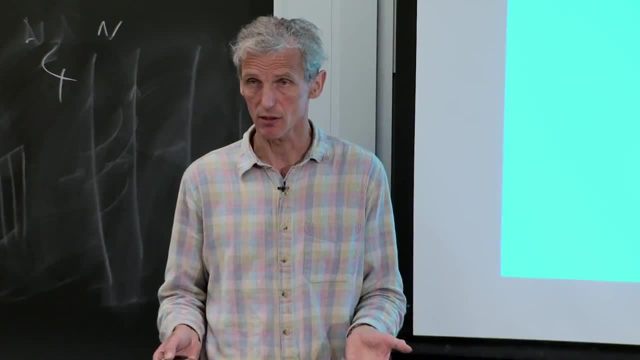 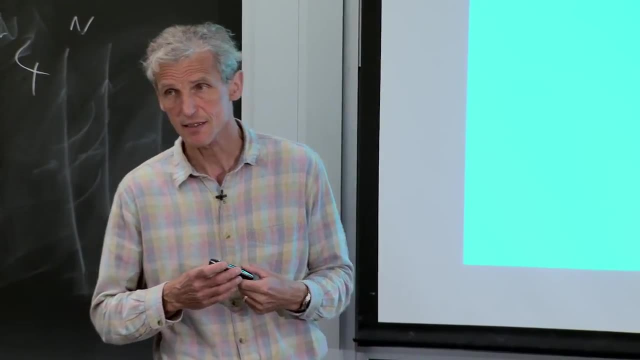 or electrons, which are Bloch waves in a periodic potential. So this is one reason why, OK, OK. The other reason why we want to go to optical lattices is the following: Ideal Bose-Einstein condensates are trivial. 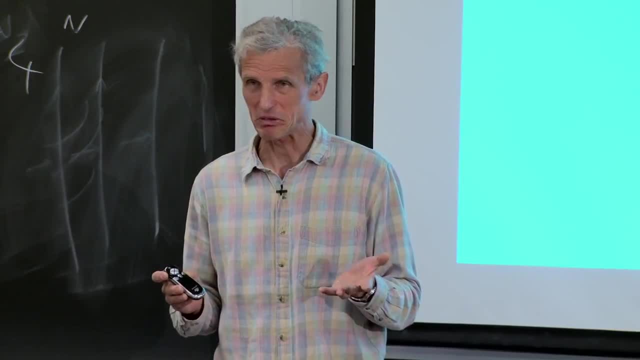 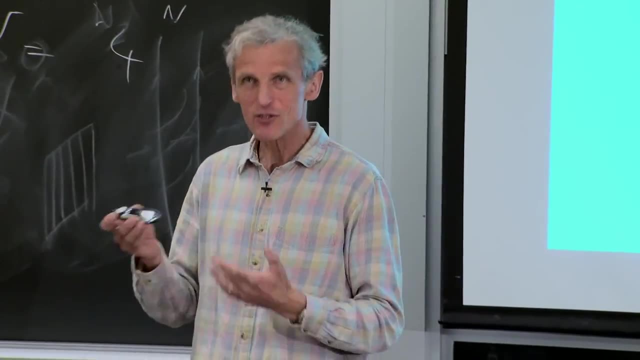 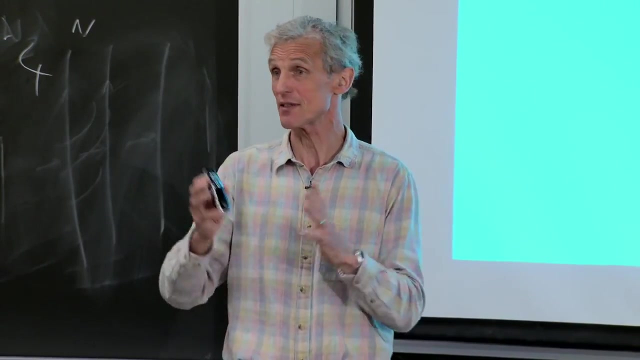 Weakly interacting. Bose-Einstein condensates are entertaining And you can write a lot of papers. have a lot of fun of it, develop your methods. Also mildly intellectually interesting, because how those weak interactions manifest itself in vortices and all that is really rich and interesting. 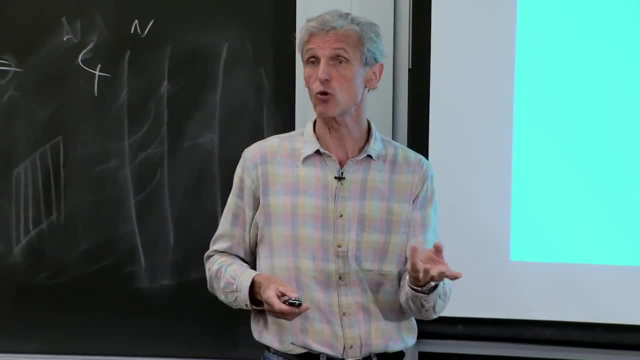 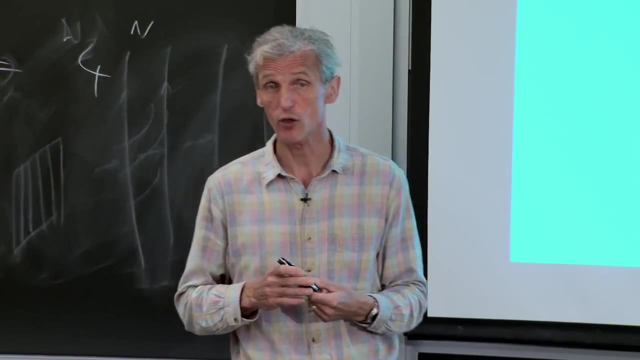 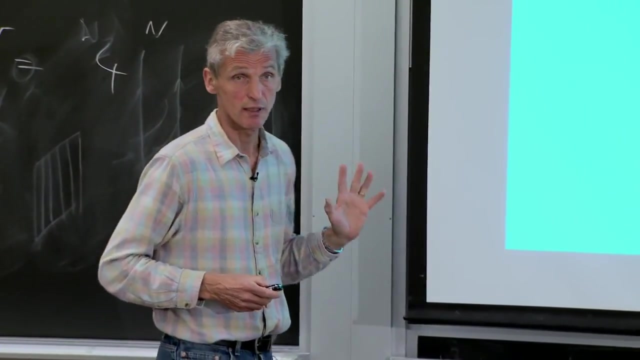 But the conceptional problems appear when you go to strong interactions. Strongly correlated matter is where mean field descriptions no longer work. This is really the frontier of our understanding of many-body system And when you want to be there, you want to create a strongly correlated system. 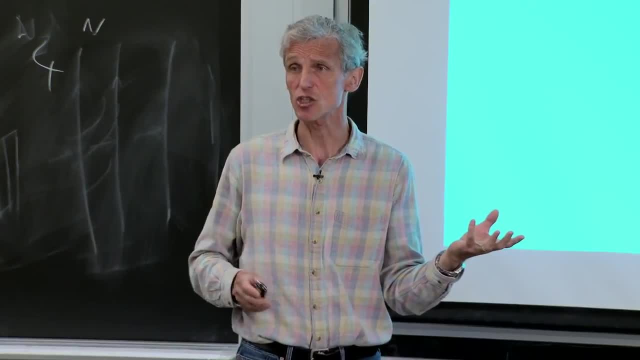 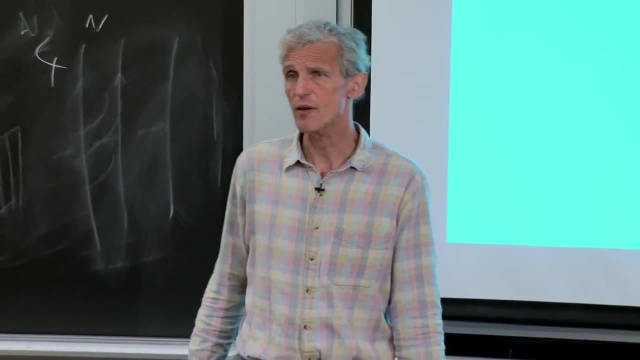 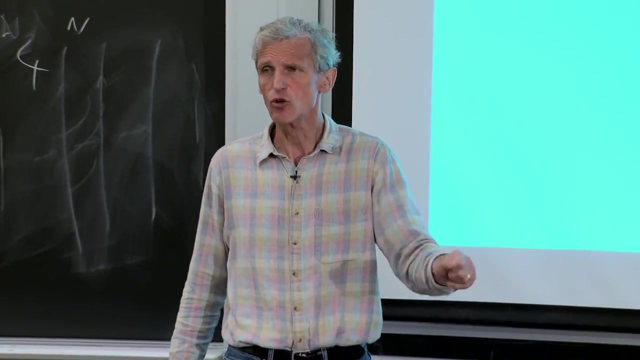 And strongly correlated systems means that the interaction energy dominates over kinetic energy. OK, In Bose-Einstein condensates you can only go so far with increasing interactions via Feshbach resonances because you get into some inelastic collisions. So that's one knob to turn. 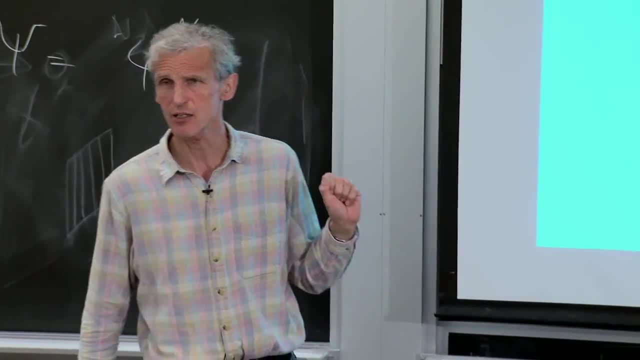 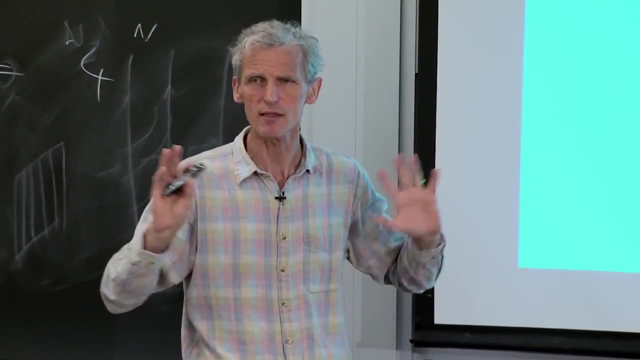 You go to larger and larger scattering lengths and crank up the interactions. But if atoms strongly interact they start to do bad chemistry, They start to spin, flip, They do other things And in some cases you keep it under control, In others you just can't keep it under control. 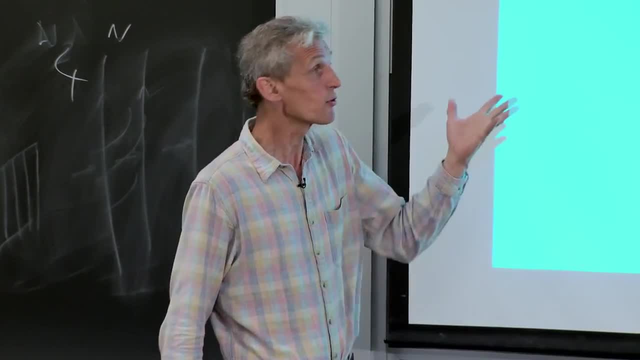 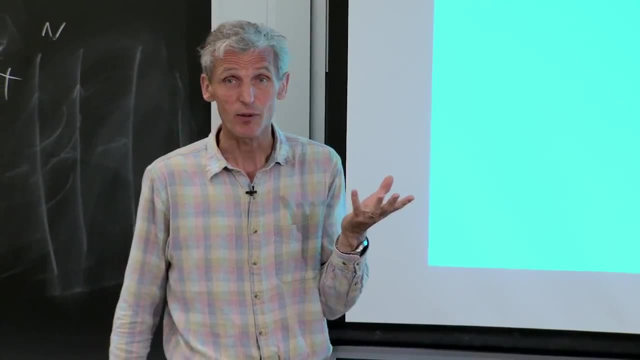 But another way to get to strong interactions means you reduce the kinetic energy. It's the ratio of the two which matters. And when you put particles in a lattice, well, the lattice actually reduces the kinetic energy. You may know from condensed matter physics: 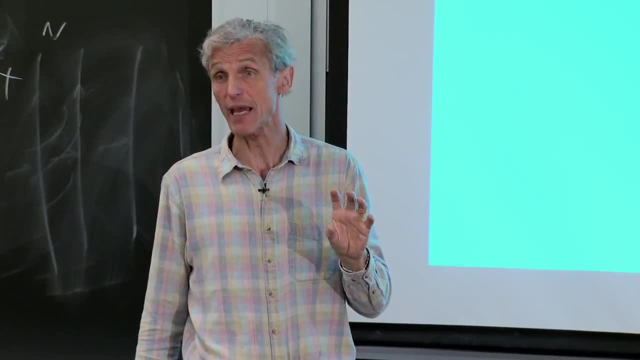 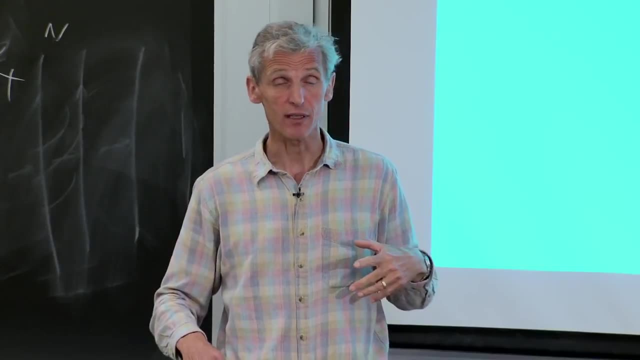 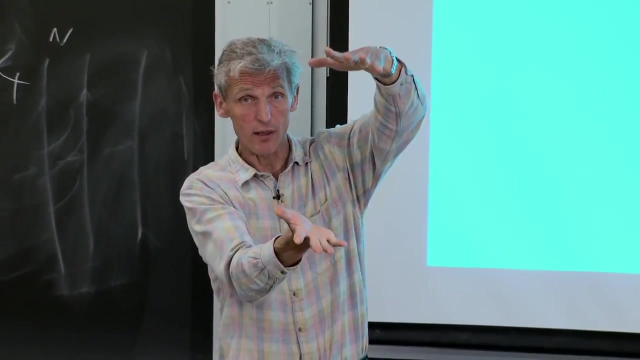 that in a lattice there's an effective mass which is higher than the bare mass. Therefore you have reduced the kinetic energy. Or, if you want another hand-waving approximation, the kinetic energy is given by the bandwidth, And if the tunneling becomes slower and slower. 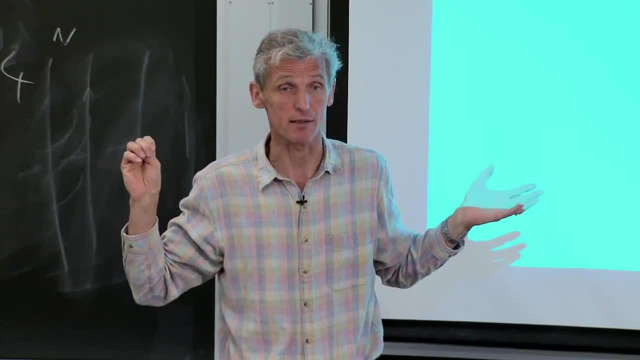 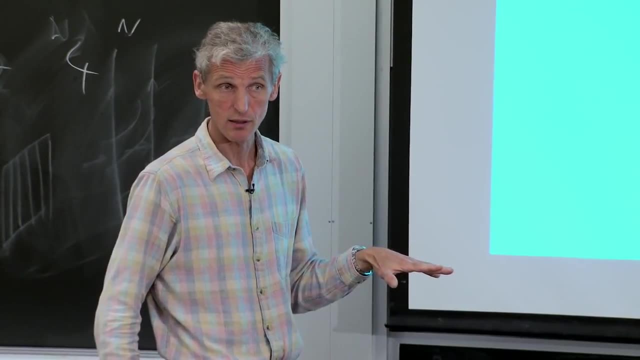 the width of your band becomes narrower and your kinetic energy is less. So anyway, I can give you many hand-waving approximations why, in a lattice, kinetic energy is reduced And repulsive energy is probably enhanced, because, instead of having your atoms spread out, 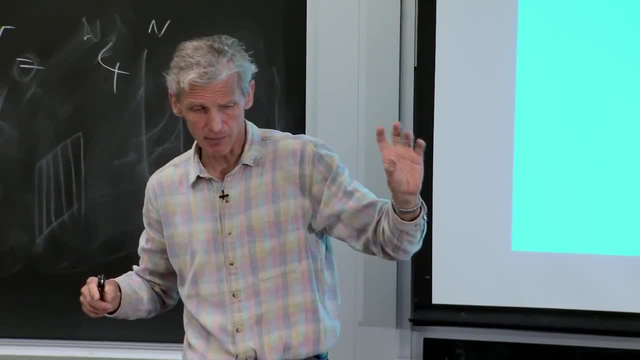 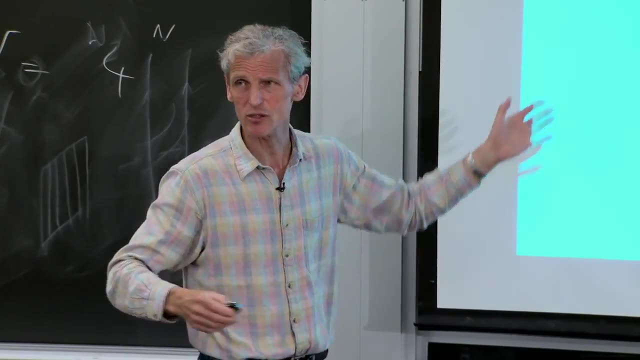 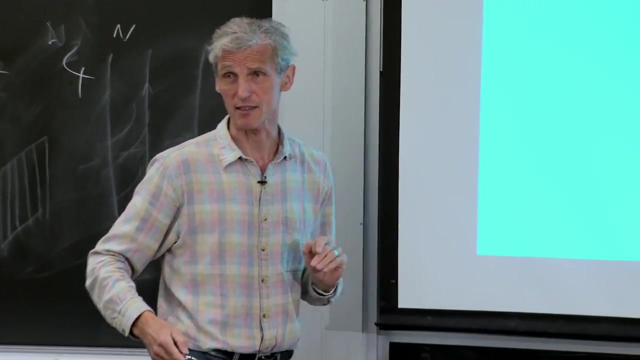 they are bunched up at each lattice side into a higher density cloud. So anyway, Maybe you're interested in periodic potentials, or you're interested in quantum systems with strong correlations. For whatever reasons, you want optical lattices. Now I have here a few slides which 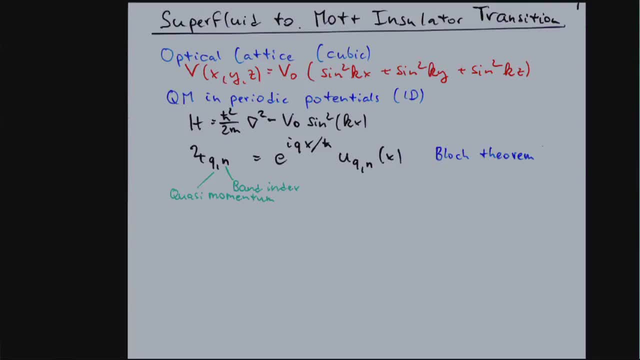 introduce periodic potentials, but it is really just the single particle physics in a periodic potential. It has nothing to do with quantum gases. This could be the first lecture of how to describe electrons in a matter, So let me just Quickly go through, assuming that almost all of you 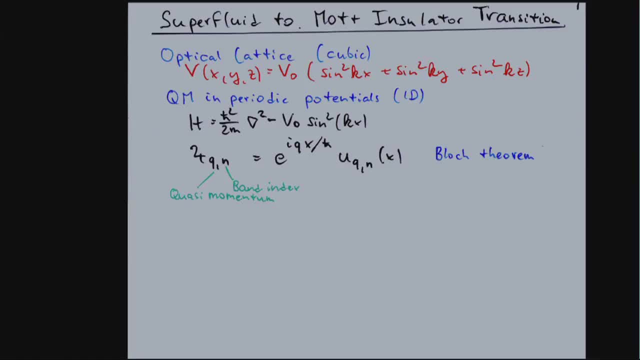 are familiar, But I use those slides also just to give you a few definitions and introduce a few symbols. So this is simple, boring, exactly understood physics. We have a Hamiltonian which has kinetic energy and a periodic potential which is our lattice potential. 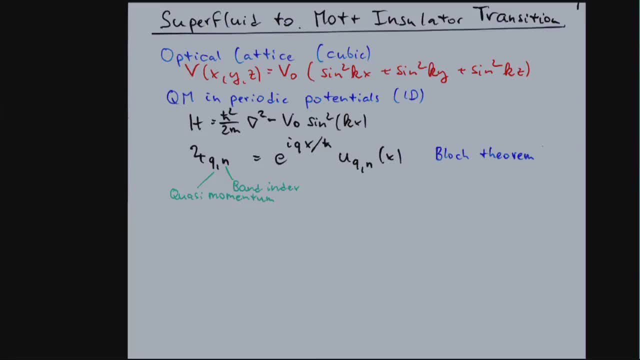 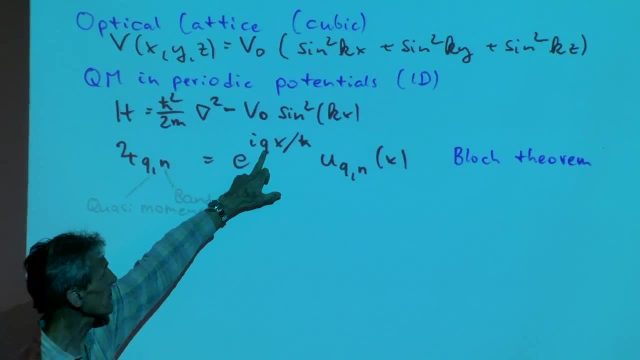 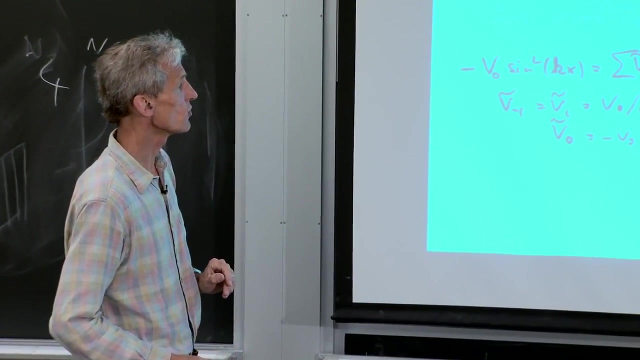 It's rather trivial to solve that exactly For your wave function. you use Bloch's theorem And write it by an exponential factor with quasi-momentum times, a periodic function. And if you now solve Schrodinger's equation you want to use Fourier space. 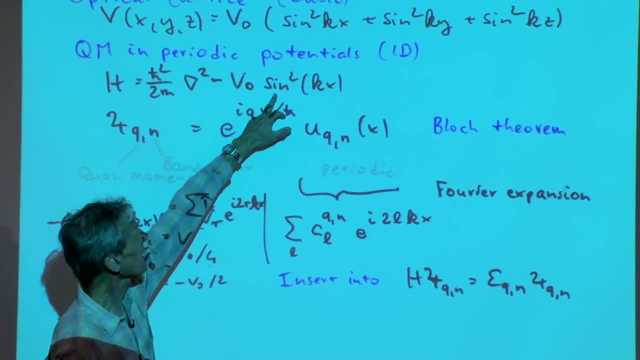 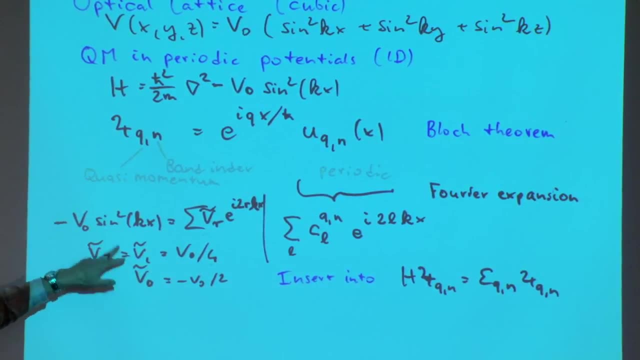 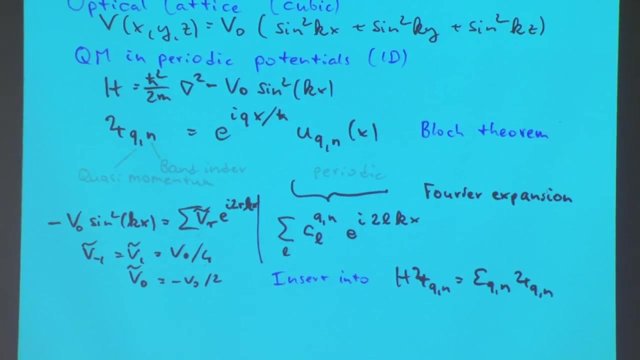 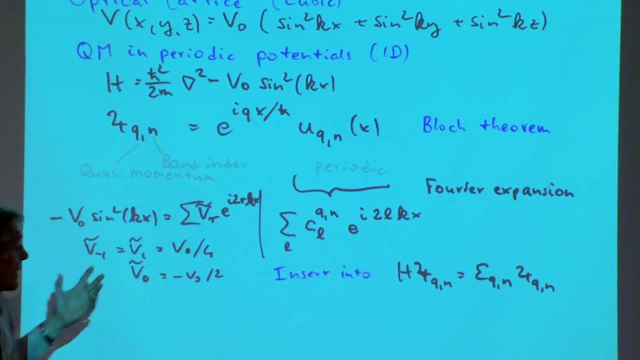 You Fourier analyze the wave function, You Fourier analyze the potential. And since the potential is periodic, sine square, potential has only three Fourier components. at 0 plus minus 1 times The periodicity of the lattice, You do a Fourier expansion for your periodic wave function. 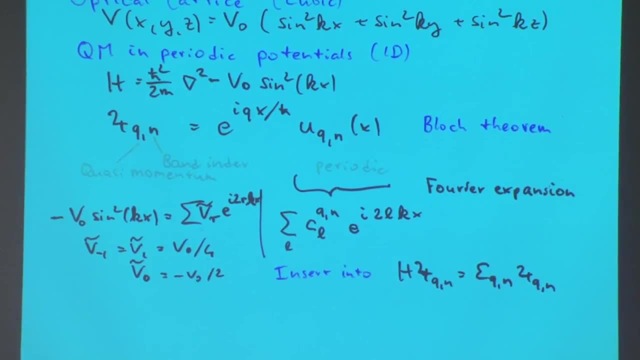 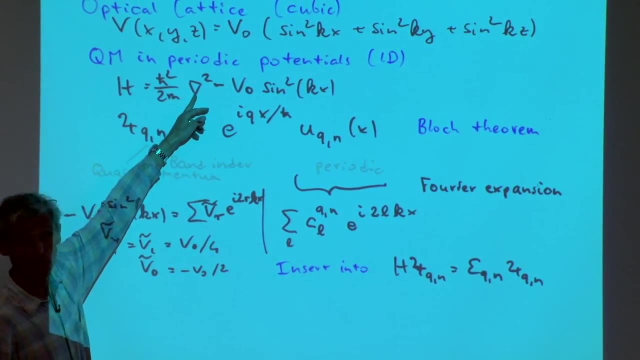 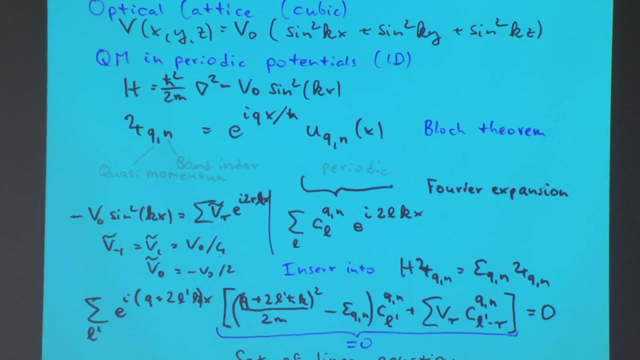 And if you insert that into Schrodinger's equation, well, the Fourier transform has turned the differential equation into an algebraic equation, Because the second derivative simply becomes now k square or q square. So in other words, you have a set of linear equations. 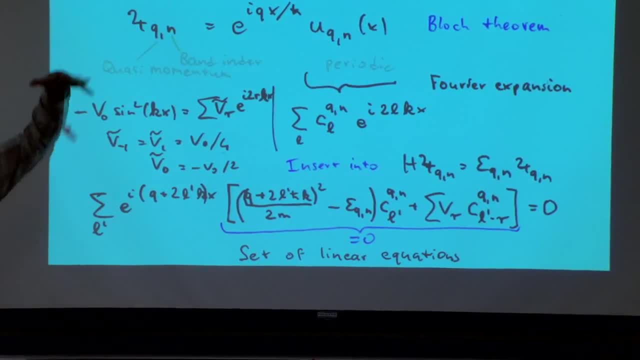 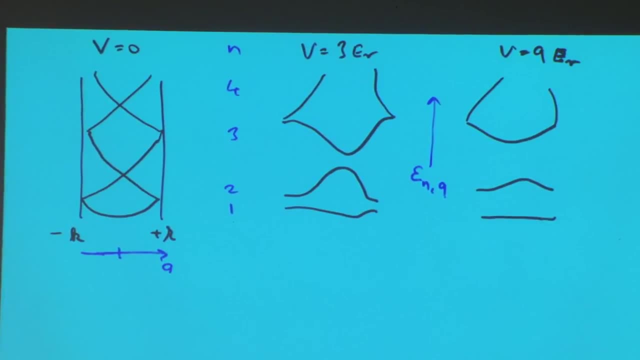 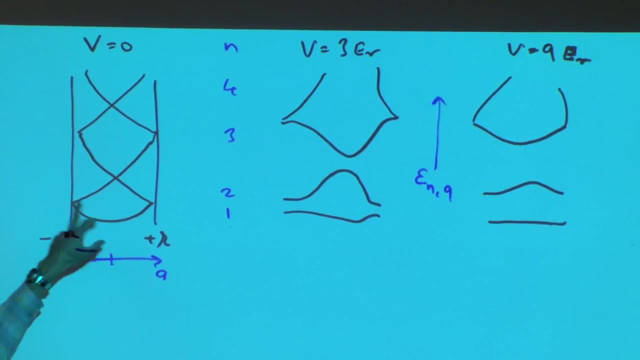 There is an index which is the bend index. How high do you want to go? And usually you truncate it, But it's the same. It's really the same trivial story which is told in all textbooks of condensed metaphysics: If you have no bend structure, well, you have the parabola. 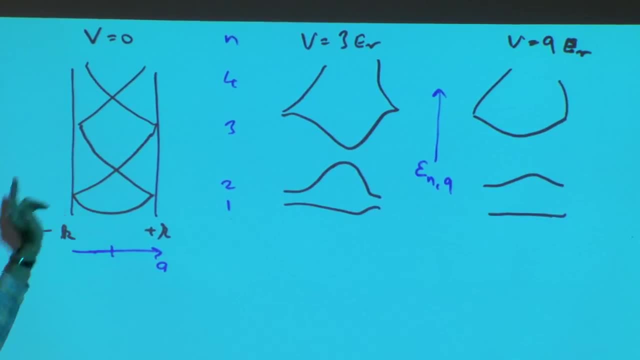 But to prepare for bend structure. I've broken it down here in the first briozone And if you now introduce a lattice, you introduce bend gaps And you go from the left to the middle, to the right for stronger and stronger lattices. 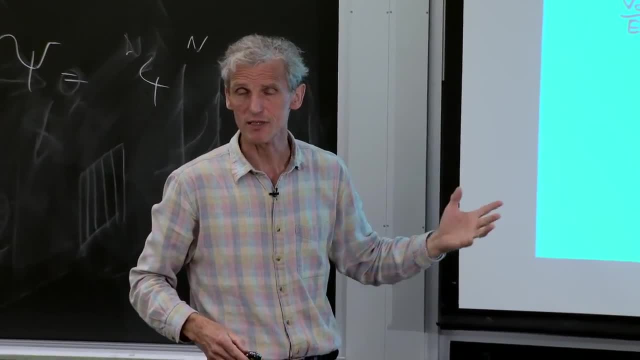 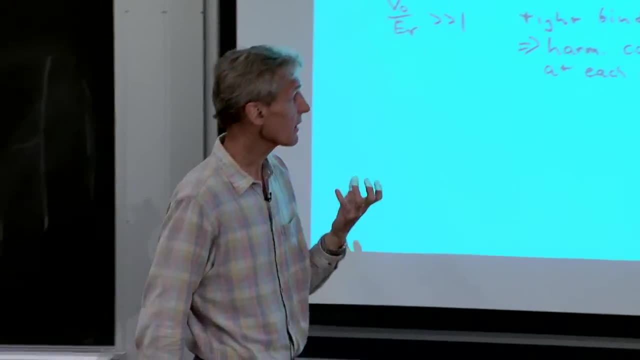 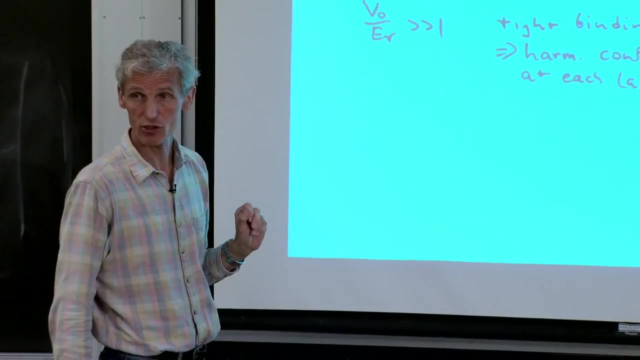 So the case which I will be focused on, because it is the most extreme case away from free space, is this case which is called the tight binding limit, where the potential energy of the lattice is large, And large means Mm-hmm. 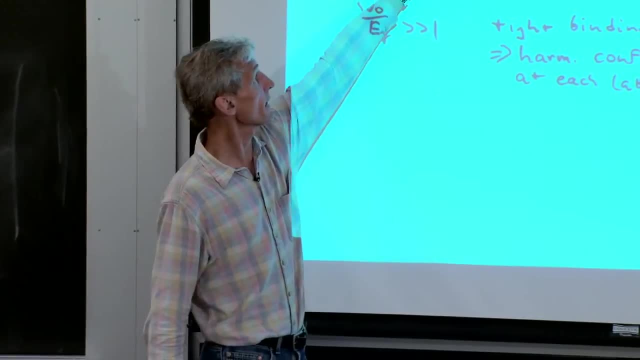 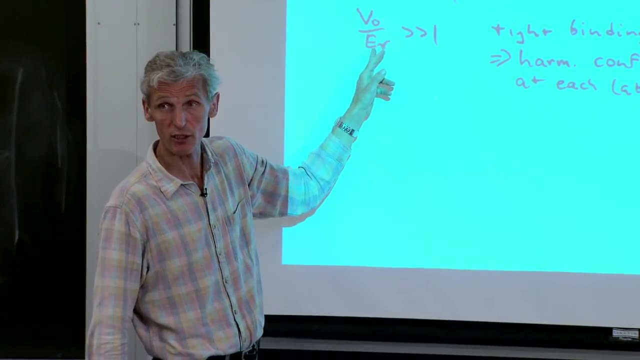 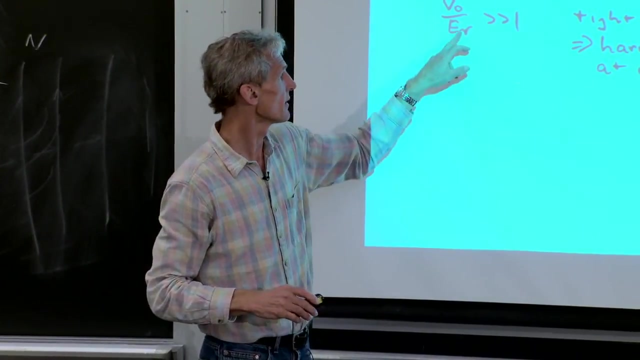 OK, OK, Compared with the kinetic energy at the briozone, which is k square, k is the lattice momentum, k square over 2m, And that's the recoil energy. So our dimensionless parameter here is the depth of the lattice measured in recoil energies. 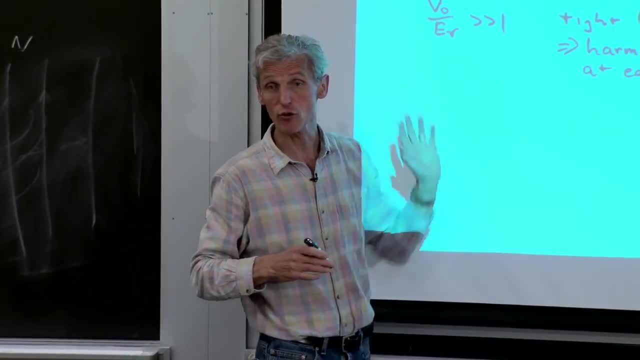 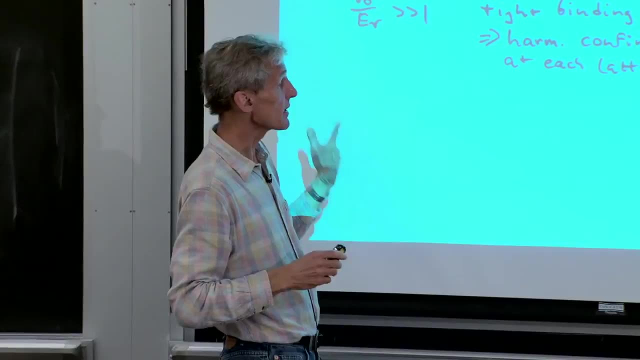 recoil energies of the photon, because that is the kinetic energy of the free gas at the briozone. OK, There are a few things which immediately simplify. Simplify that Once we are in the tight binding limit, our lattice is really deep. 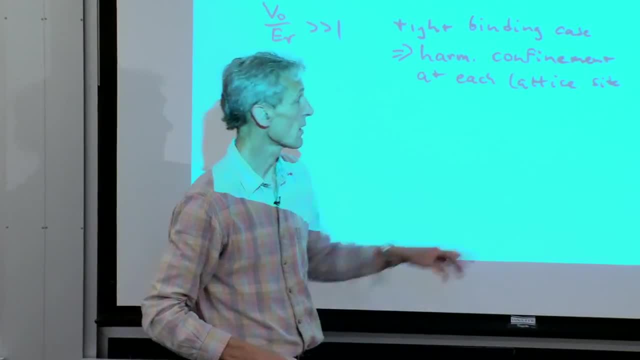 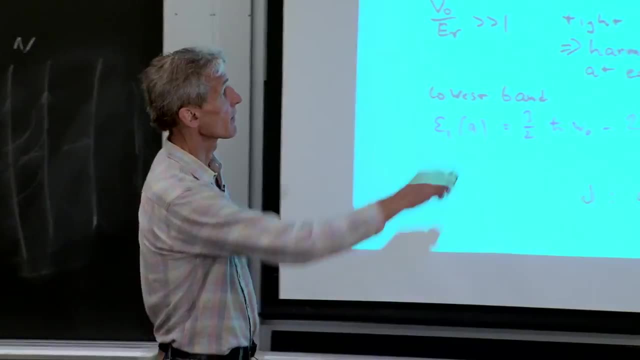 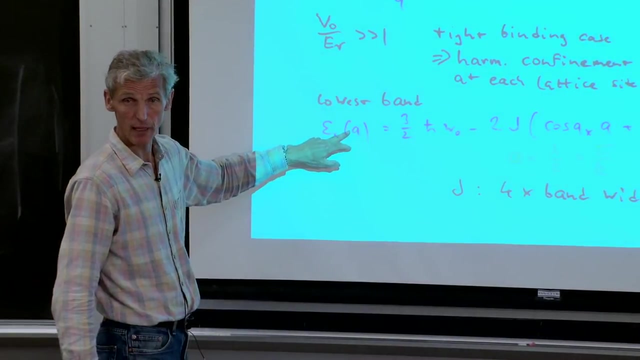 And each side forms an harmonic oscillator. And the harmonic oscillator frequency is analytically given by the depth of the lattice And the solution here for the lowest bend is that the lowest bend, the energy, in the lowest bend, the dispersion relation is well we 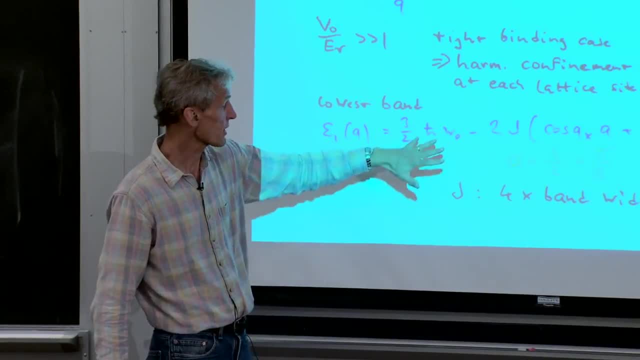 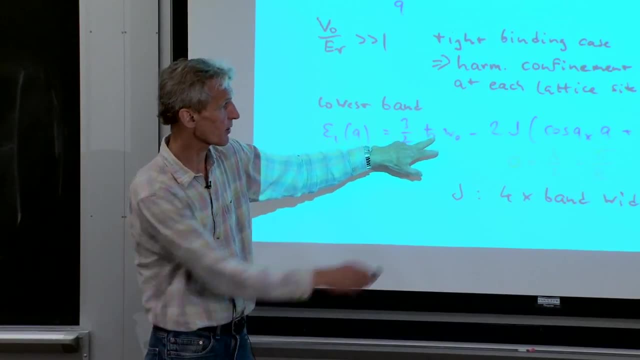 have a harmonic oscillator at each side in x, y, z. So The average energy in the lowest bend is the zero point energy in x, y and z, 3 half h by omega naught, And then we have a cosinusoidal bend structure. 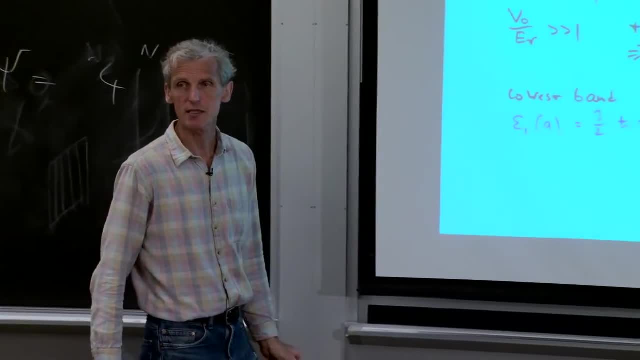 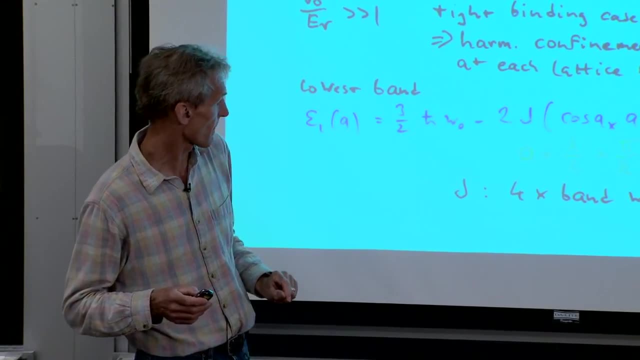 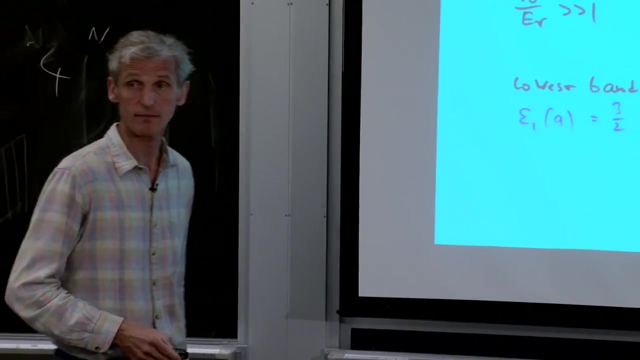 where q is the quasi-momentum, And what appears here as the only interesting parameter is j, And j is, I think this 4 should be- 4j is the bend width. So what appears here now for the first time is j. 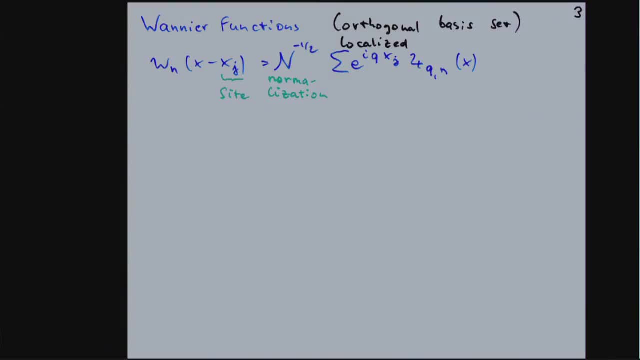 It appears here as the bend width, But let me immediately give it another interpretation, as a tunneling matrix element, in the following way: Right now we have formulated the physics in Bloch wave functions, which are infinitely extended. The Bloch wave functions are for the lattice. 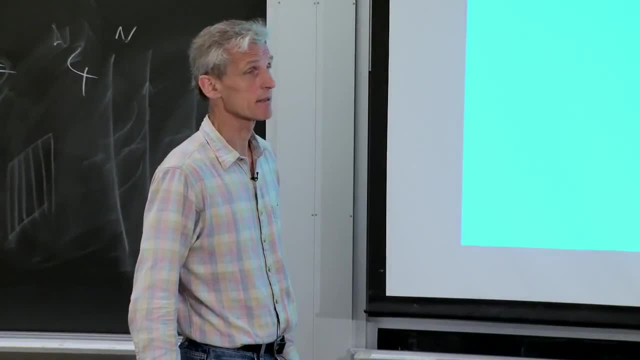 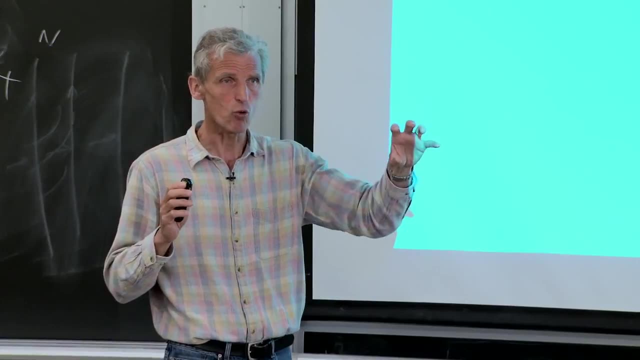 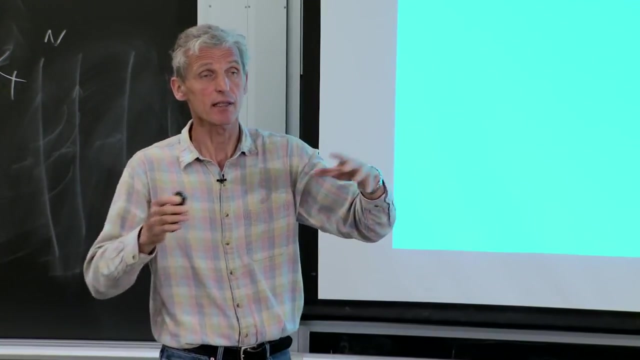 What plane waves are for free space. But if you have tight binding limit, there is another limit which is important, Namely a particle is localized and hops around in the lattice. The localized particle, of course, is in free space. It would be a wave packet, a superposition of plane waves. 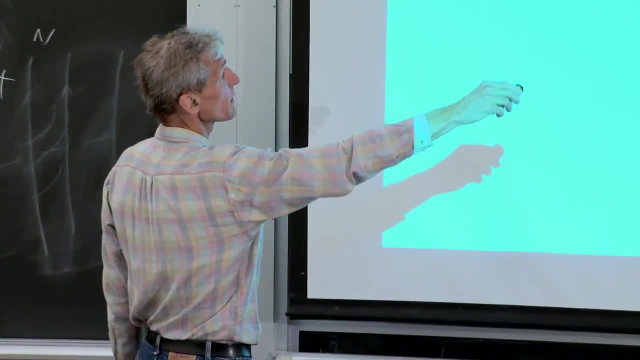 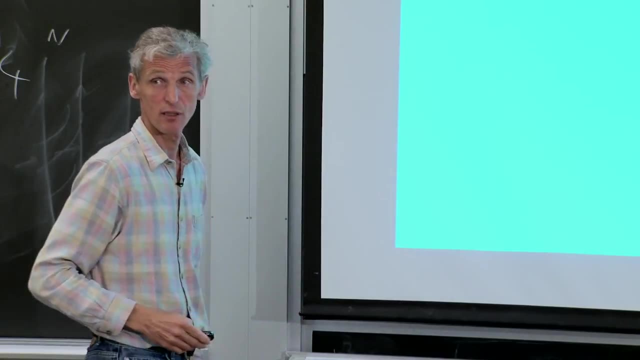 So let's do the same in the lattice. Let's construct superpositions of Bloch waves And these are our wave packets. And the wave packet is now called the Vanier function And there is a mathematical procedure how you should pick the phases here. 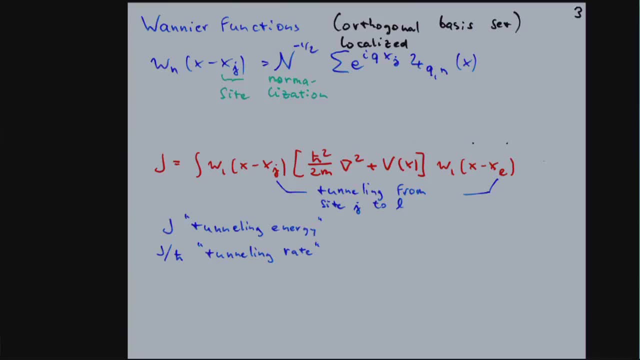 to get the maximum normalization. But the simple picture is those Vanier functions are very, very close to the Gaussian ground state solution of the harmonic oscillator. at each side The wings are different, but I don't want to go into that. It is you transform from an orthonormal basis of Bloch wave. 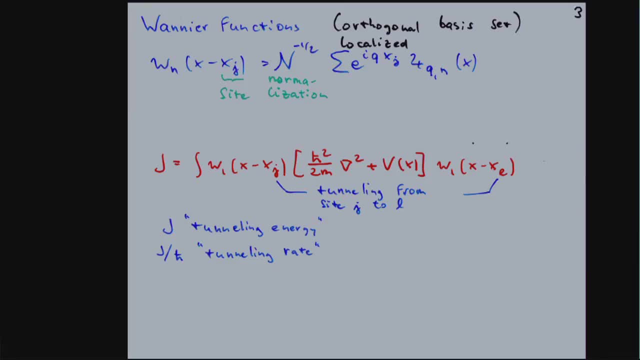 function to another orthonormal basis Or Vanier function, And the Vanier functions are as well localized as possible. That's the procedure, And now we can simply rewrite our total Hamiltonian or everything we are interested in, not in Bloch wave functions. 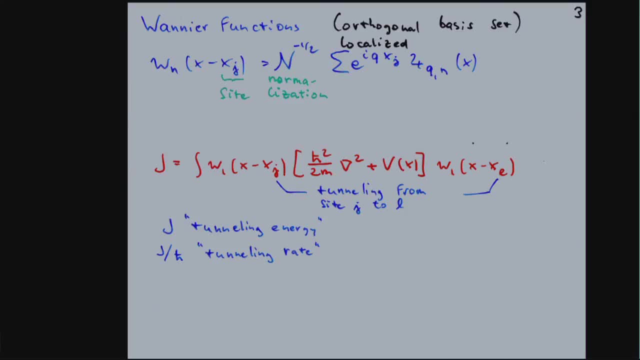 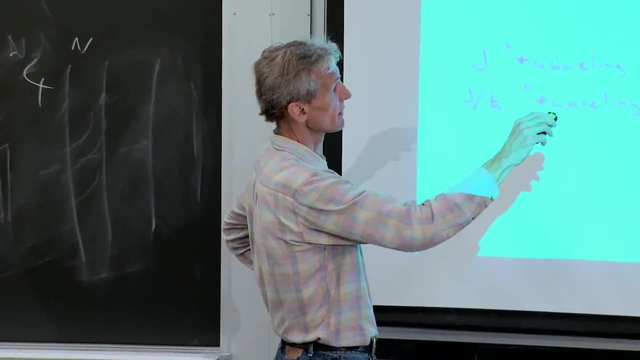 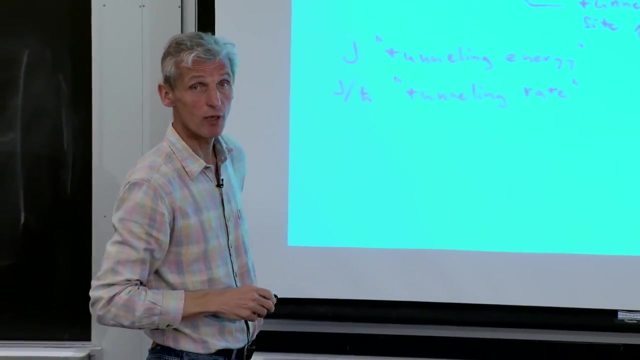 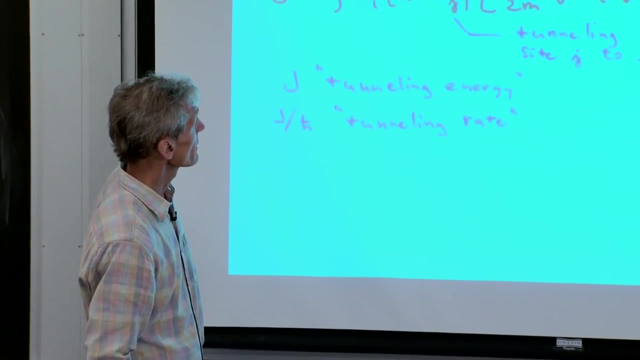 but in Vanier wave functions. And what comes out now is that the bandwidth J is nothing else than our Hamiltonian with kinetic energy and the periodic potential. But J becomes now a matrix element between two Vanier functions. But the Vanier functions have now 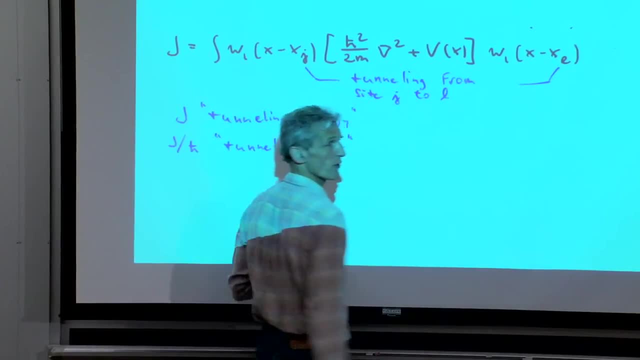 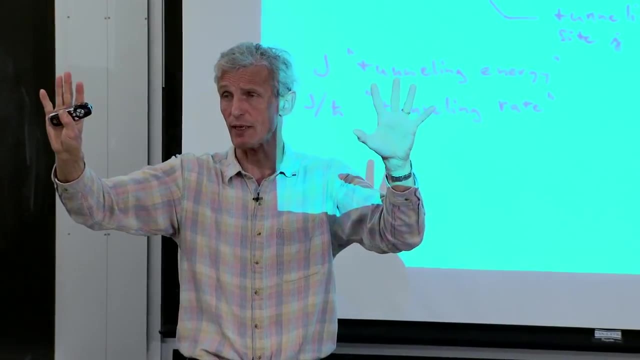 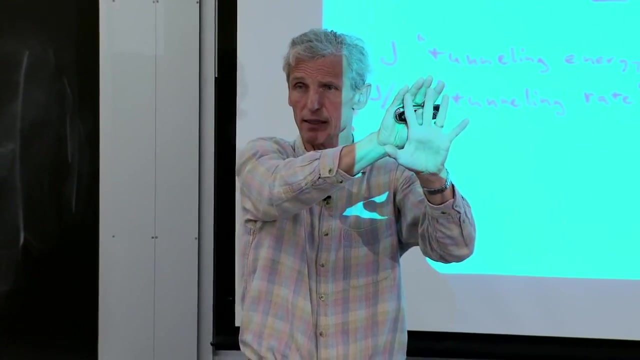 I put in some indices in a moment, connect now two different sides. So it is: you have one Vanier function, you have the Hamiltonian and connect it to another Vanier function. So it is the amplitude That with the Hamiltonian the particle. 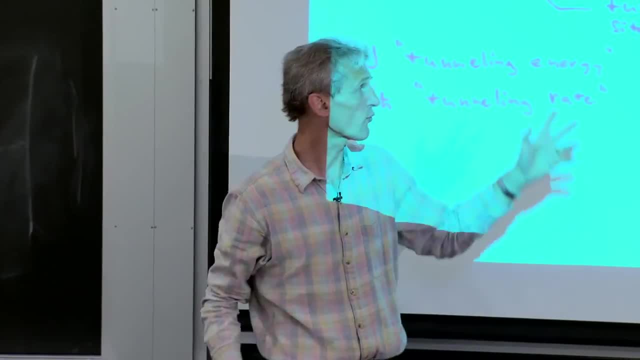 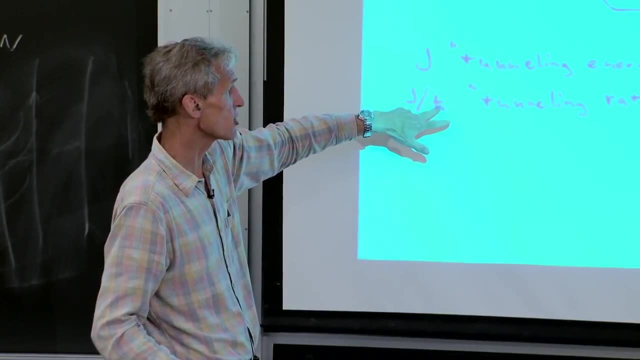 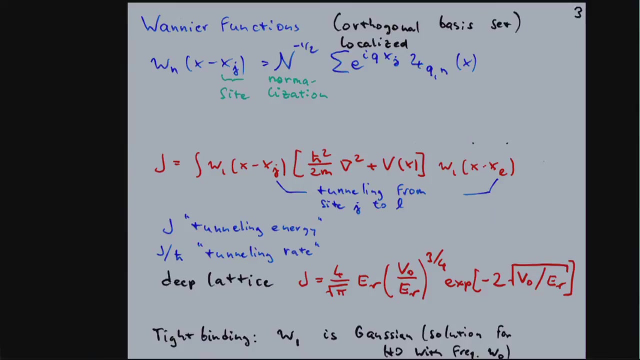 can hop from one side to another side. So therefore, J, which was the bandwidth, is now the tunneling energy divided by h bar the tunneling rate from one side to the other side For very deep lattice. everything is analytic. 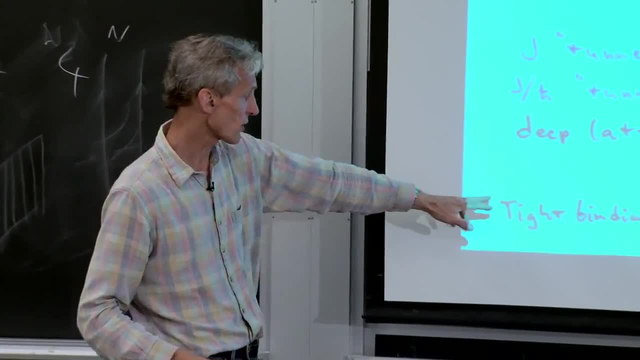 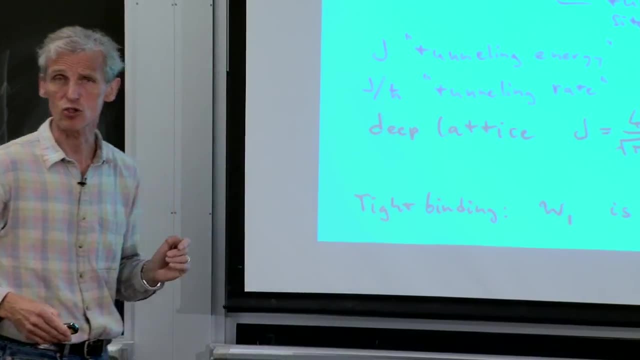 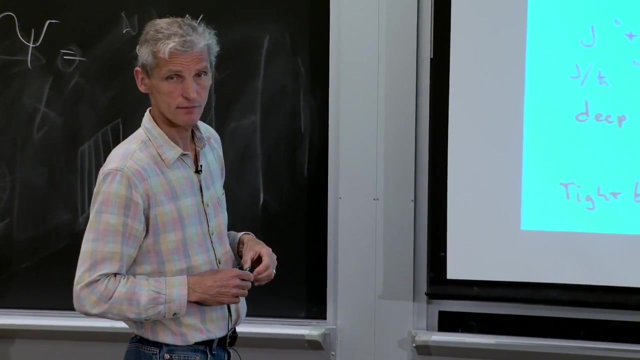 and it can easily be solved. And I mentioned already in the tight binding approximation, you should think about your Vanier function as just, oh, a localized Gaussian eigen solutions of the harmonic oscillator. Yes, So qualitatively this question sounds sort of silly. 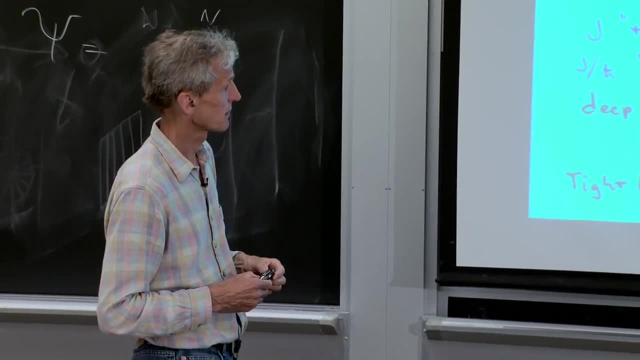 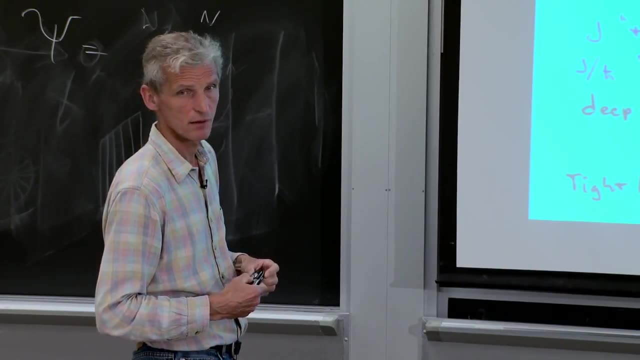 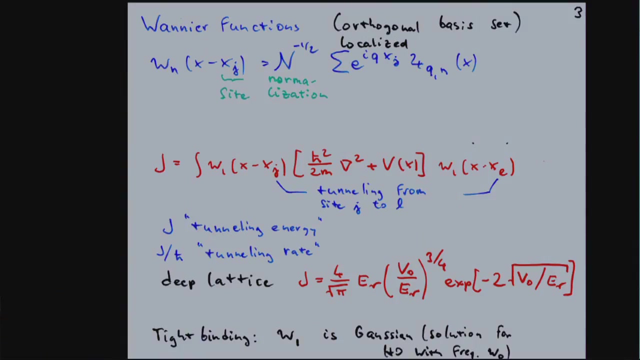 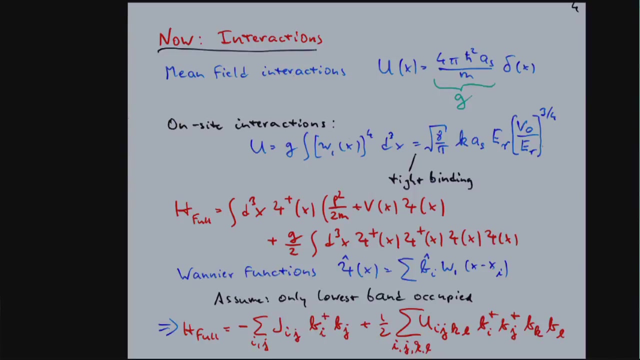 But normally we write down the solution for J. We're only considering the nearest neighbor hopping, But sort of from the math, I don't immediately see why we wouldn't include i equal to J. Give me one more slide. So I should have actually what I should have done. 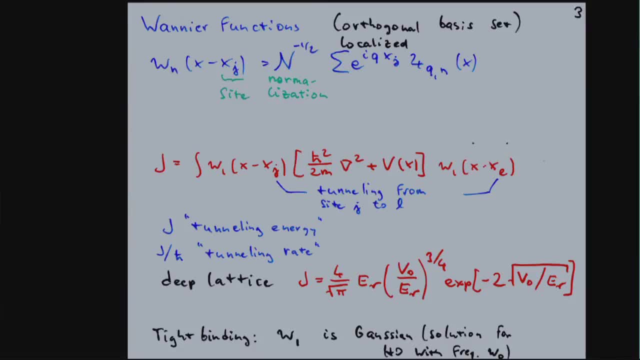 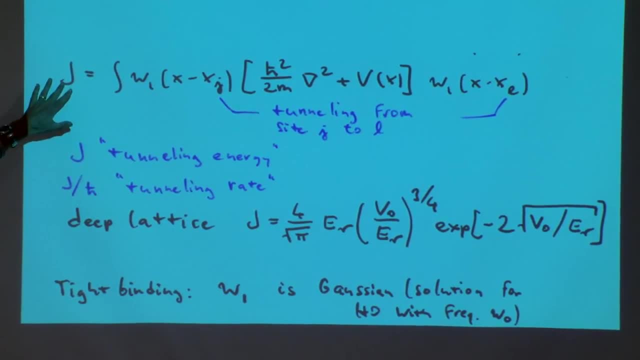 is that J has an index here. I just didn't want to overload it with indices. I will immediately. I mean, this is sort of just telling you what J is in its simplest form. It is loaded with indices And I will show you in a moment where those indices come in. 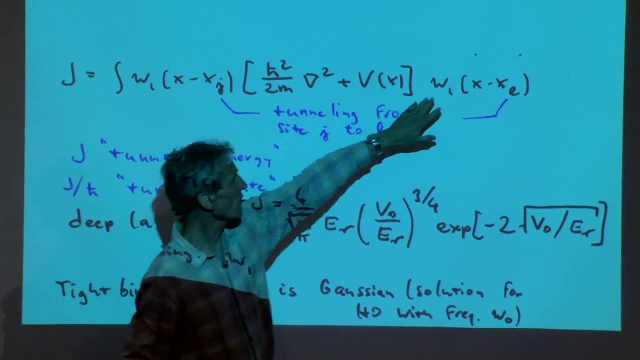 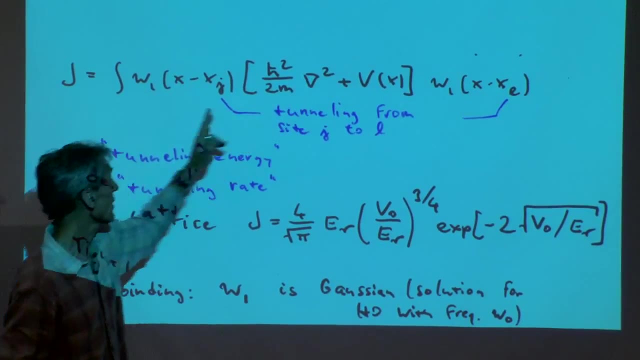 So I just wanted to give you the idea that we want to have one Vanier function. We hop from one Vanier function to the other one And the operator is the Hamiltonian, And therefore there should be an index J and L. 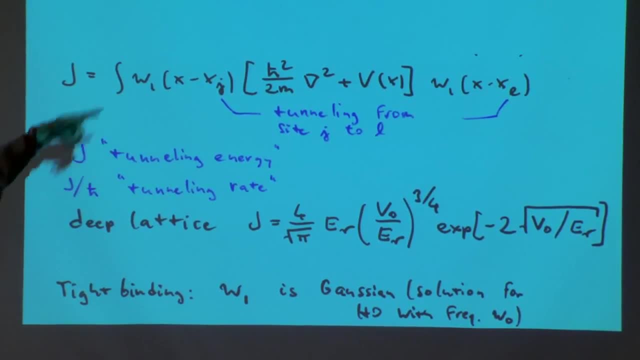 And maybe let me just do the next step first and then come back to it. But I wanted to tell you here what I'm aiming at, namely interpretation of J of tunneling from one side to the next. But right now I haven't really told you. 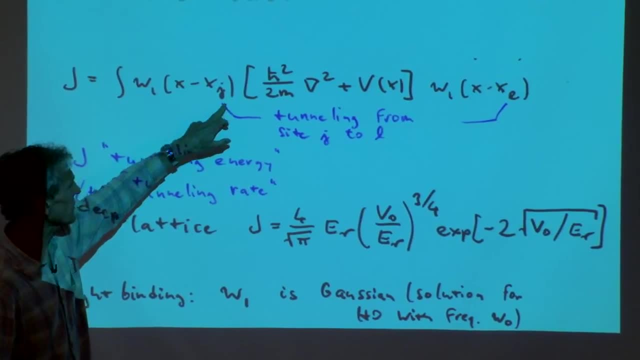 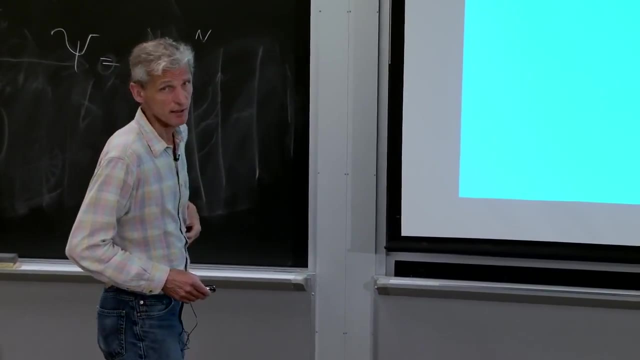 which J I really mean There should be based. on the right-hand side there is a J which has two indices, And I will make the indices disappear in a moment. But before I make those indices disappear, let me introduce the other relevant parameter, which. 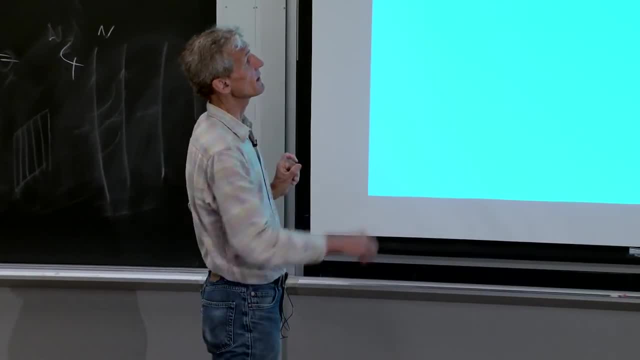 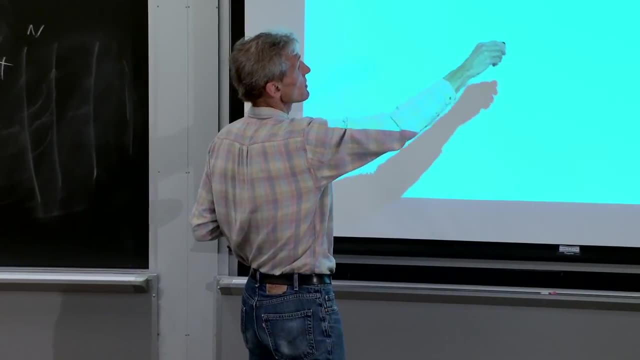 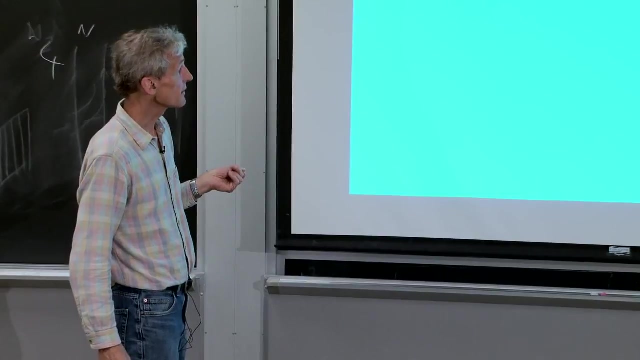 will also have indices And that is we have to bring in the interactions. We want to describe an interacting system. We describe an interacting system using the short range approximation, by assuming that two particles interact with a delta function And if you have two particles on site, 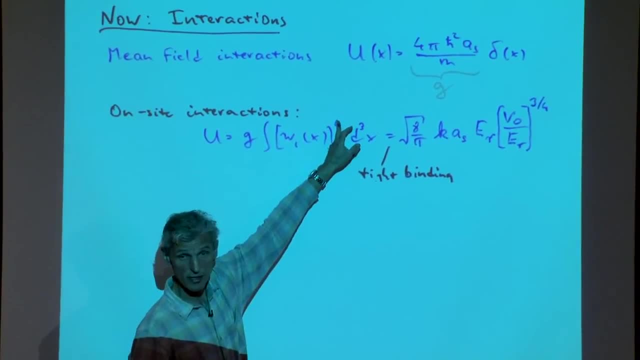 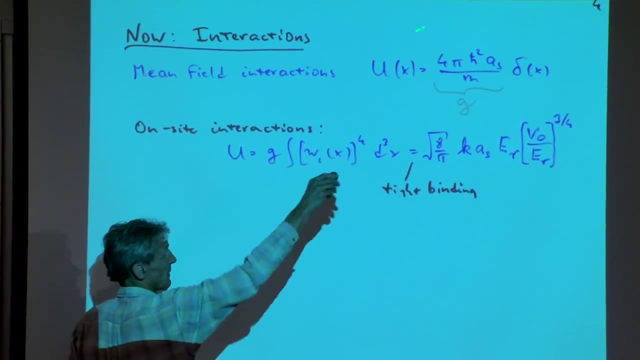 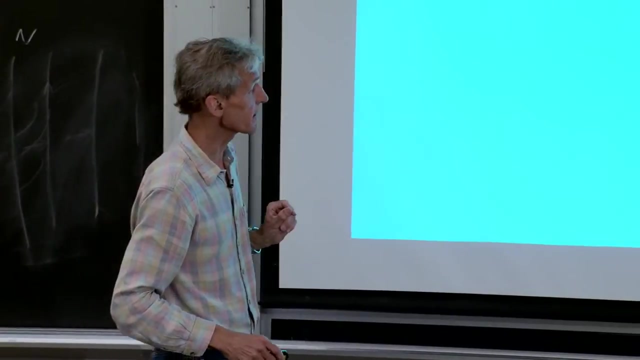 each of them has a density which is the Vanier function squared, And the product of the two densities integrated gives us the expectation value for the repulsive energy, And this is given here. So the moment we introduce interactions, we are now interested. 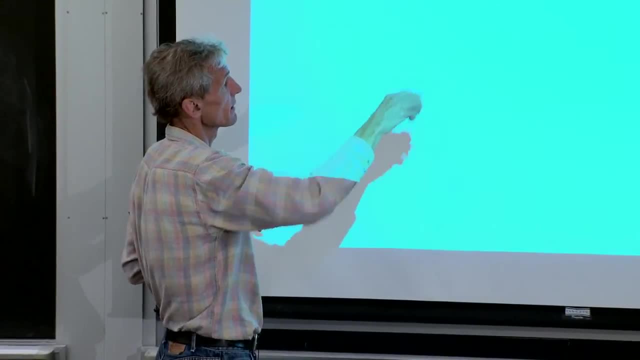 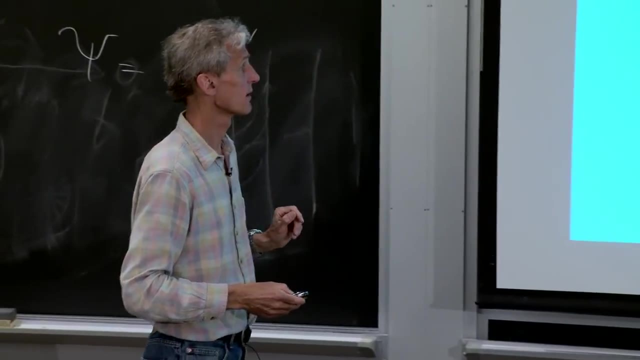 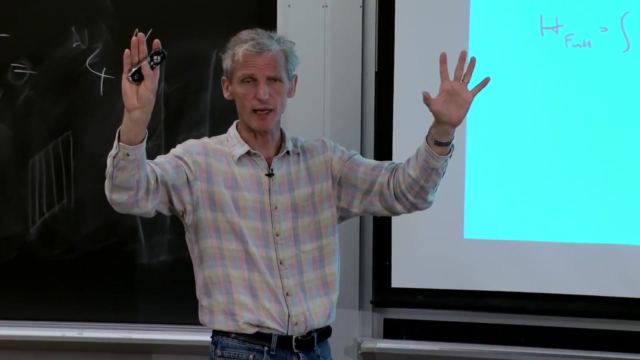 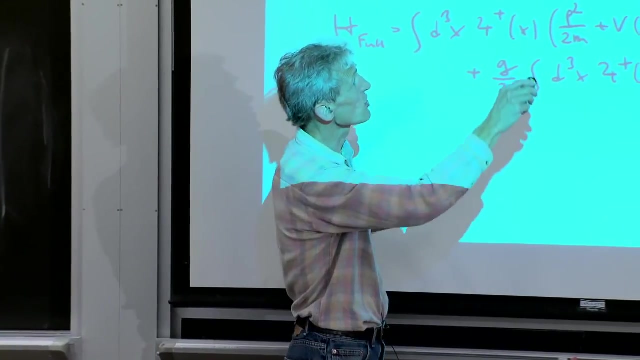 In the interaction energy between two particles which, in this case, occupy the same site. OK, so I've tried to introduce what sort of J is. J is a matrix element between two Vanier functions with a Hamiltonian in between, And U is the matrix element of two Vanier functions. 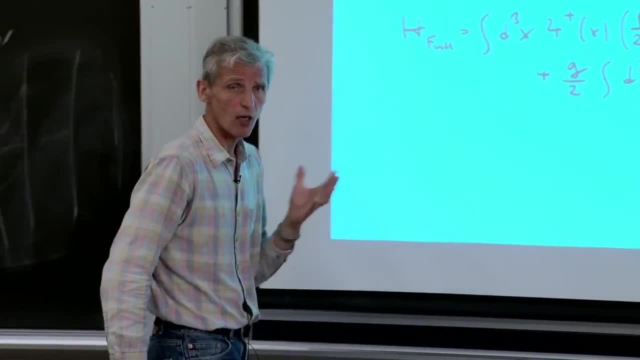 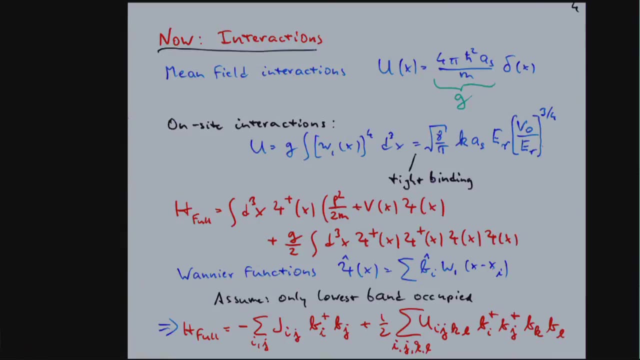 with the interaction operator in between. And now I want to use that concept. I want to take my full Hamiltonian and transform from field operators localized at x to Vanier functions. So the B operator are now creation operators. They create an atom in a Vanier function. 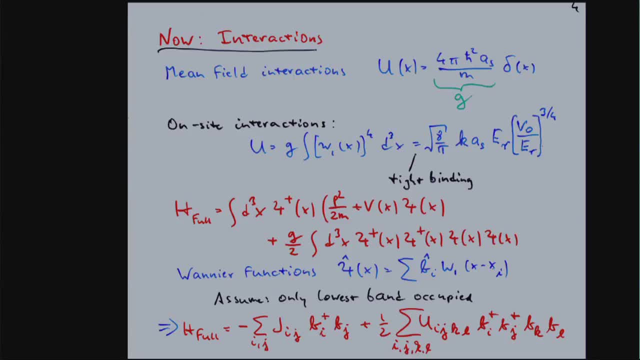 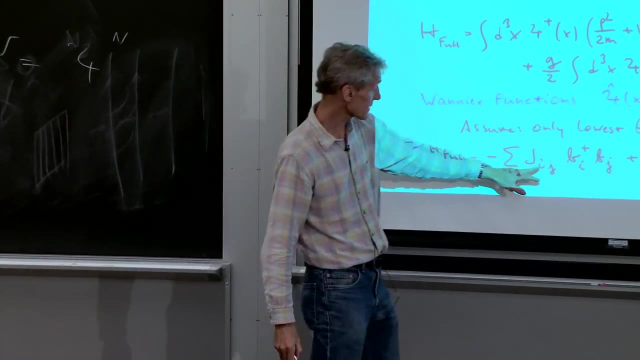 In other words, B dagger means you have a particle in a Vanier function at site i And I just use that as a basis transformation And the exact transformation of this Hamiltonian is now into this form. So what I have right now is I have the tunneling matrix. 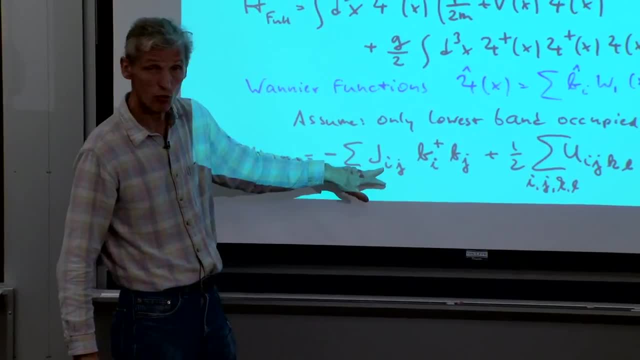 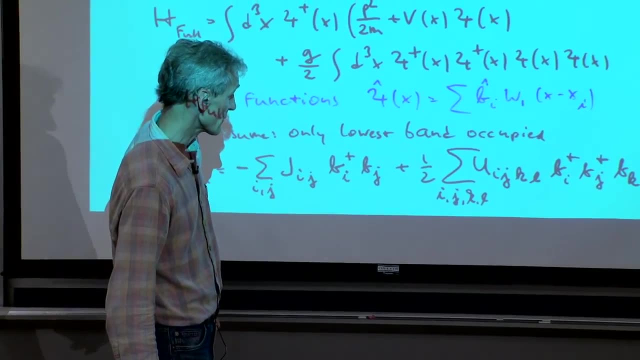 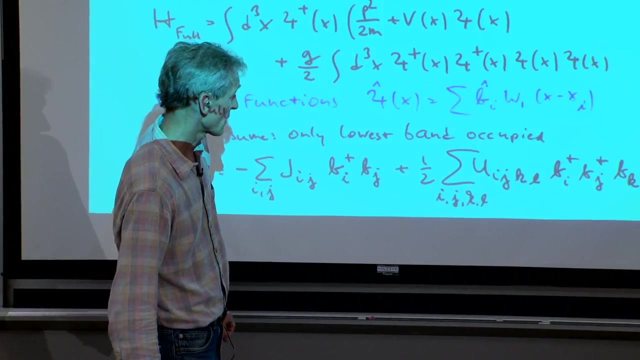 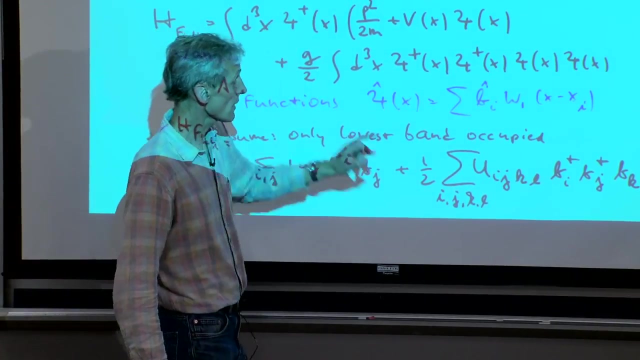 element between particles at site i and j And I have to sum over all of them And, in terms of interaction I can take, I can calculate this matrix element by using Vanier function with four different indices And ask what happens. 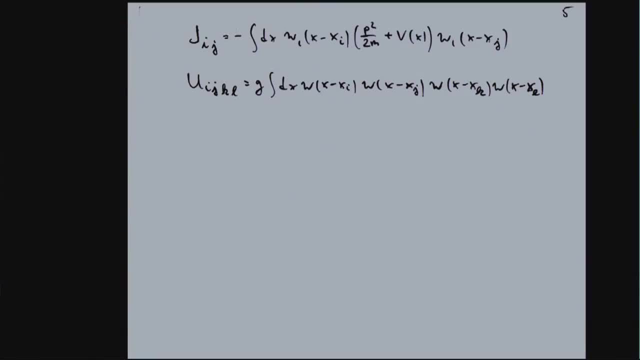 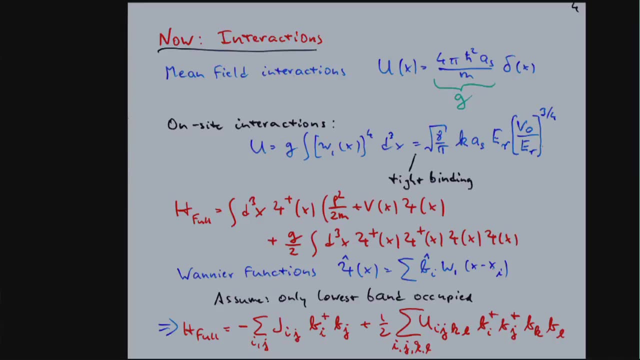 And this is simply an exact way of rewriting it, And here I've given you the definition. So if you want, Matt, forget everything I told you about J and U, I've done a transformation, an exact transformation, from field operators to Vanier function creation operators. 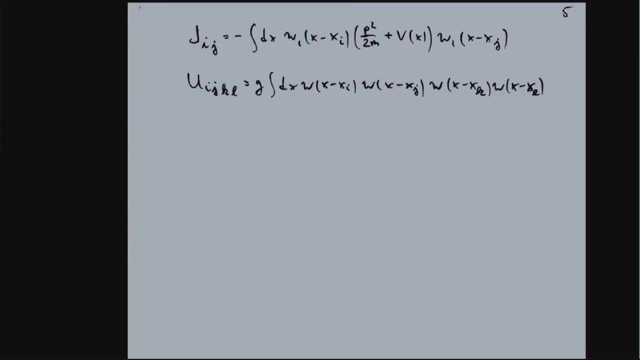 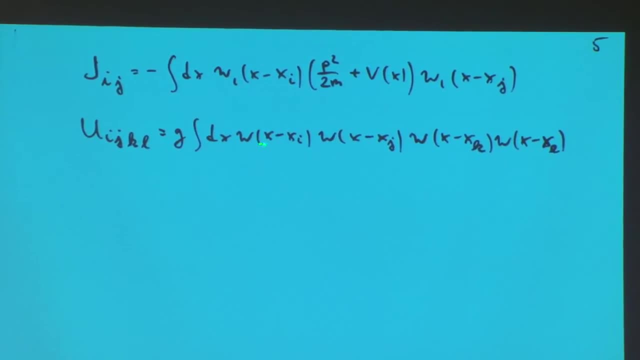 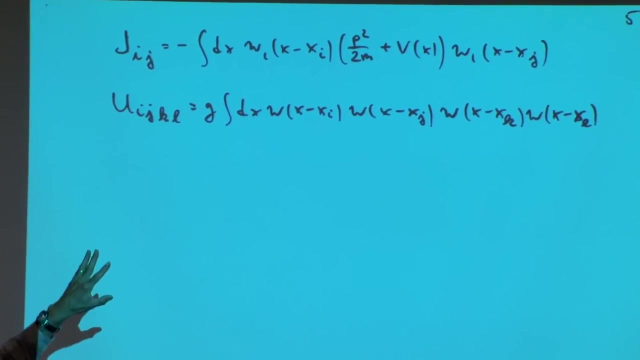 And this introduces tunneling terms like this: from site i to site j, And this here includes products of four Vanier functions which are responsible for the interaction term. Actually, if this is not complicated enough, I've suppressed bend indices here. 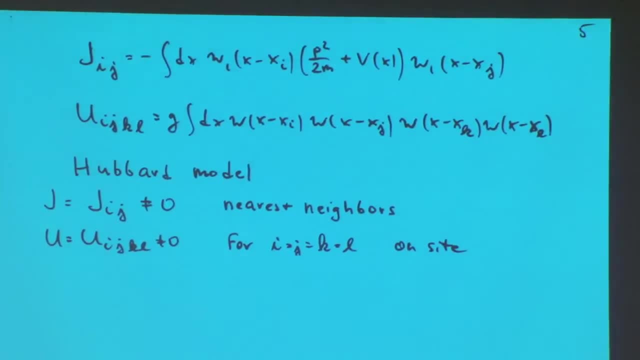 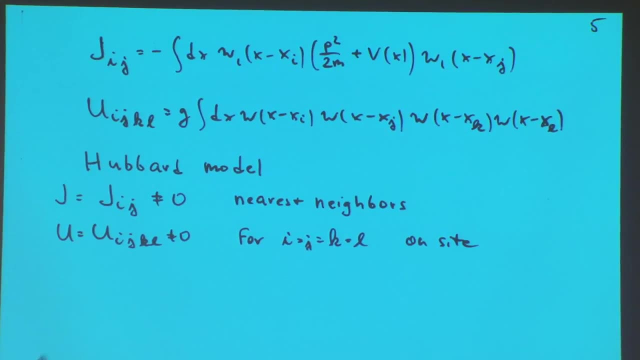 I should also now sum over all possible bends. But OK, I want to come now to the leading approximation in a tight, binding model, And that is where I mean those Vanier functions are overlap. Two neighboring Vanier Vanier functions barely overlap. 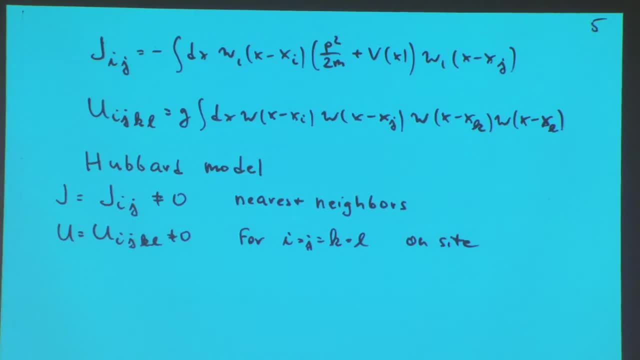 If I go further away, the overlap becomes even smaller. So the most dominant term are nearest neighbor interactions. And the nearest neighbor interaction is where i and j differ by 1. And this is what I call j without indices. And similarly, when it comes to the interaction term where 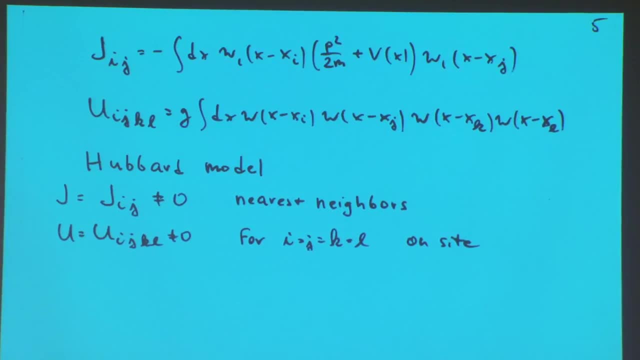 we have products of four Vanier function and we want to get the overlap of all four. we have to do this And then multiply it with g, the pre-factor of our delta function, to get an interaction term. Well, the best overlap is if all indices are the same. 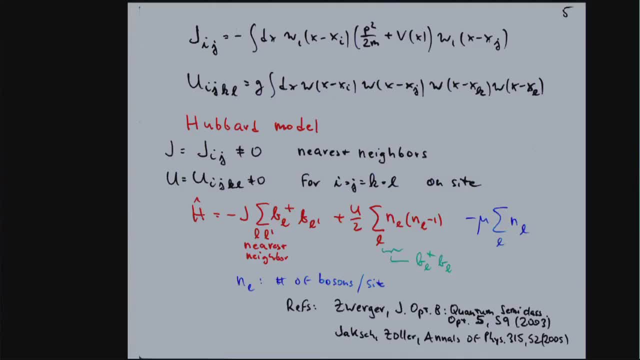 And this is what I call u. So in that limit, in that tight binding limit, my Hamiltonian is now very simple. It consists of a tunneling term parametrized with j and an on-site interaction term parametrized with u. 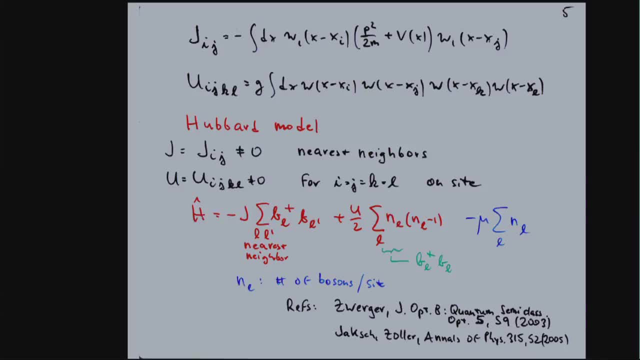 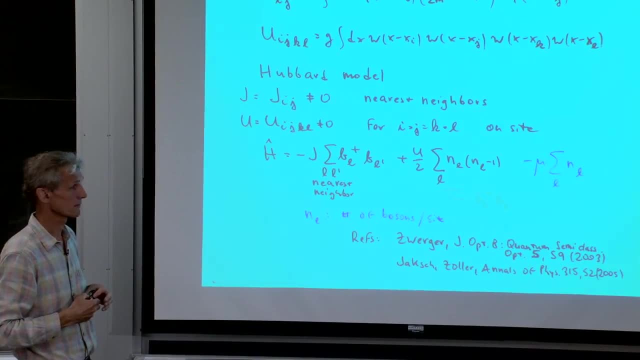 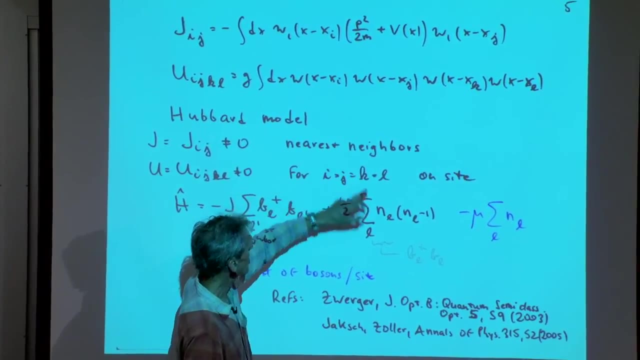 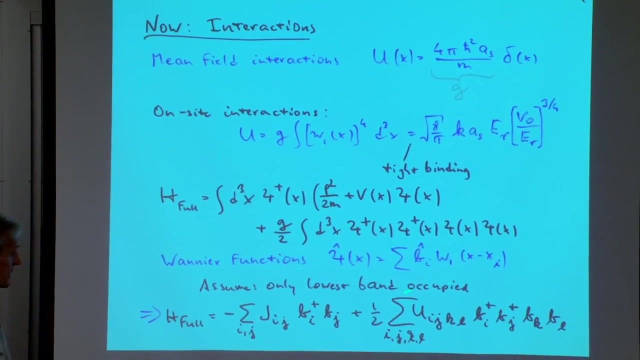 Yes. So when we are saying i, j and k are all the same, so the interaction is with the particle itself: No two particles per side When the four particles are the same, it turns into this Hamiltonian here has: all indices are the same. 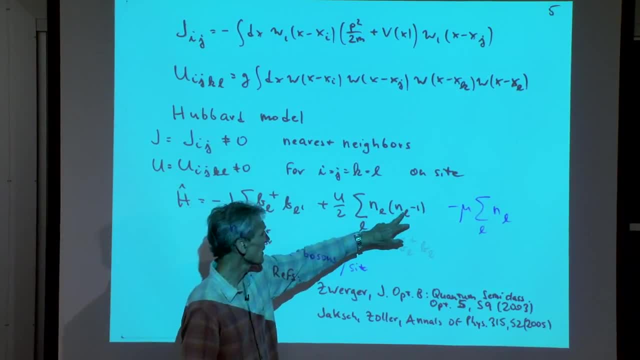 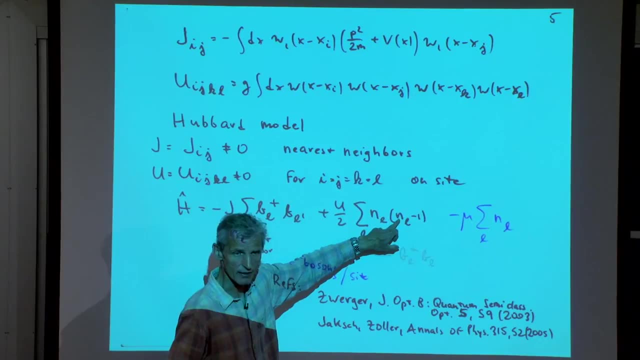 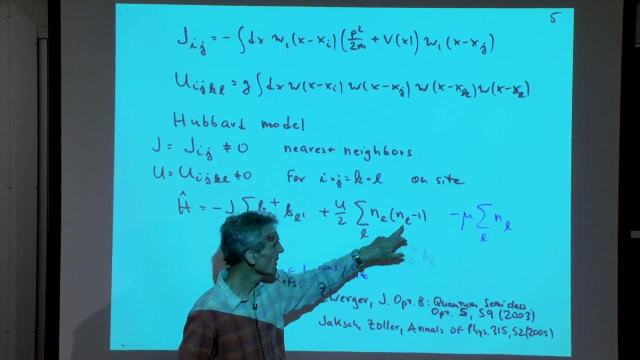 And if you calculate that, If you calculate that it turns into a product of two Bb dagger is the occupation number at each side, But if you are careful with commutators it becomes occupation number times occupation number minus 1.. 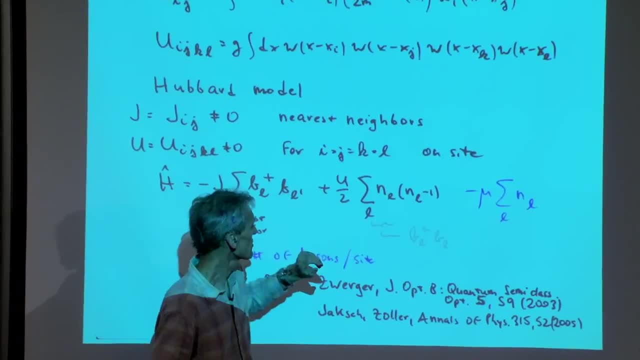 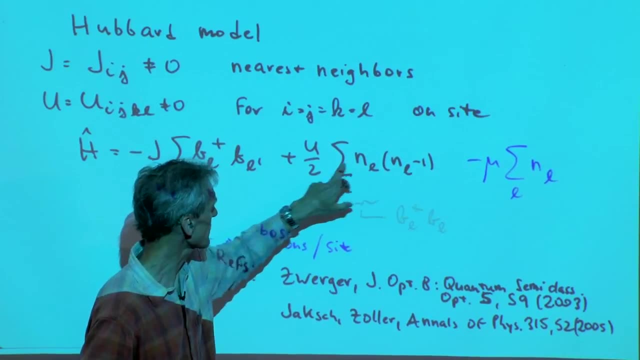 If you have only one particle per side, this term is 0.. So technically u is if you put in 2 times 1, if you have two particles per side, u is the interaction energy between two, Between two particles. 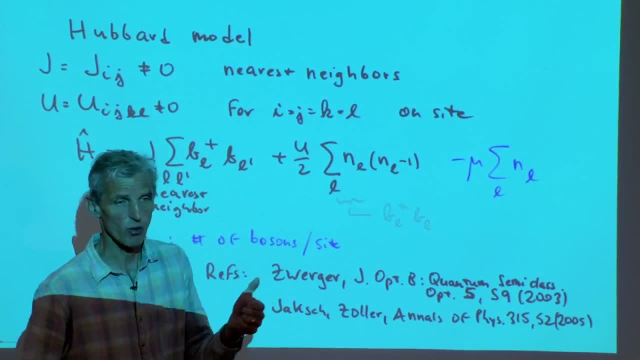 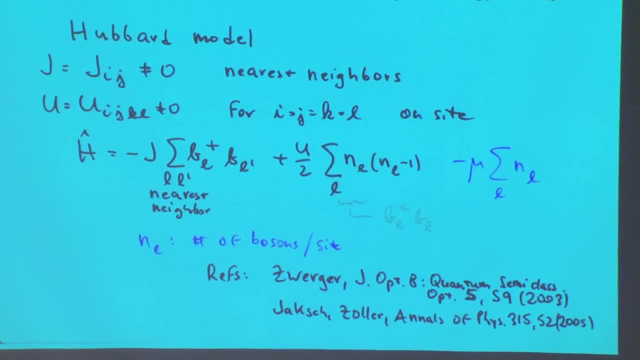 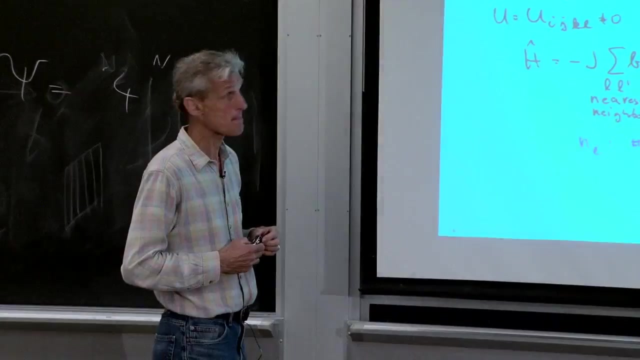 Just use this expression to figure out what it is for 3 or 4.. But for one particle you get 0.. The self-interaction of a particle is absolutely 0.. One particle does not interact with itself. I guess back to my question with the hopping. 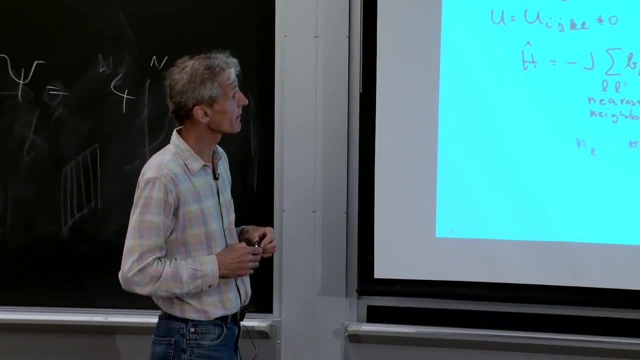 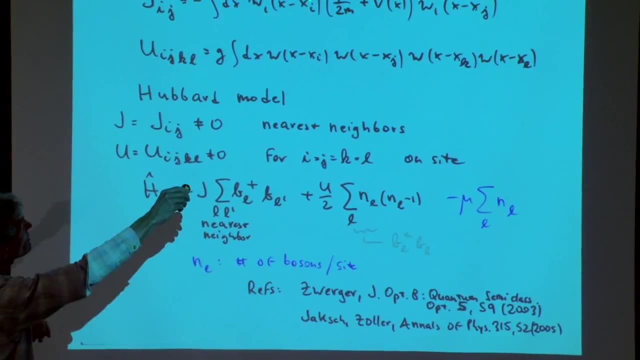 So when you have i equals i or i equals j for the hopping term, do you just absorb that? No, I assume i, j is nearest neighbor. I assume that the index i and j differ by 1.. Oh yeah. 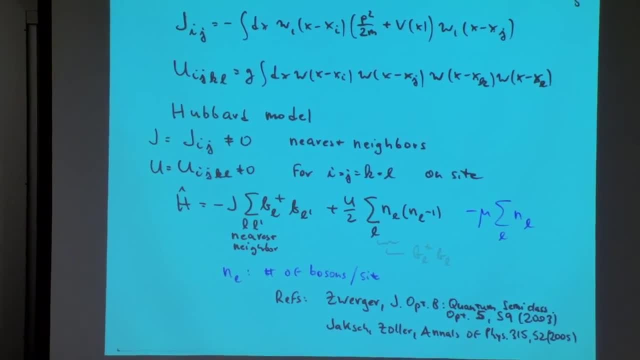 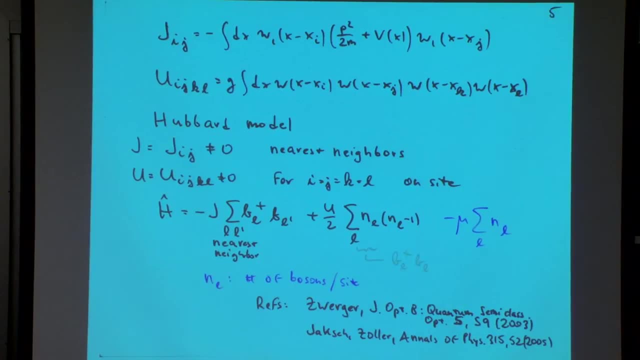 I mean. so your argument was that the best overlap is between nearest neighbors. Yes, But so I mean an overlap of the one-year functions with like at the same site is sort of the kinetic energy term like. is it approximately 0?? 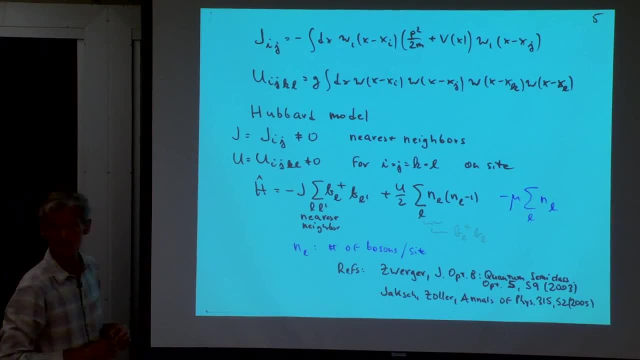 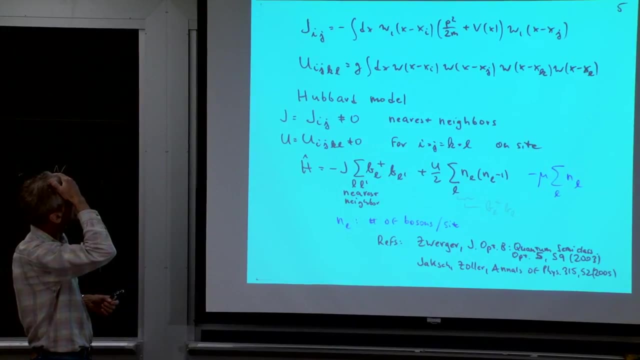 Or you just absorb that to the chemical potential. This is 0.. The lowest band is the 0 point. energy. It's the common Right. P squared is Exactly So we're only looking at nearest neighbors. So are we essentially saying the case where i equals j? 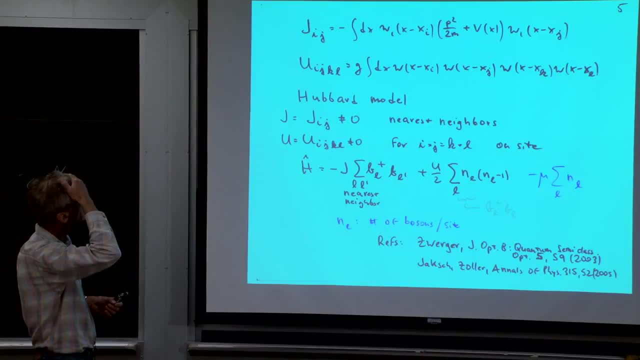 is a function of 0, you say it's just common. Yeah, because it's a matrix element of the Hamiltonian, So p, the kinetic plus the lattice operator. So if I take my function, which is built out of eigenvalues of that equation, you 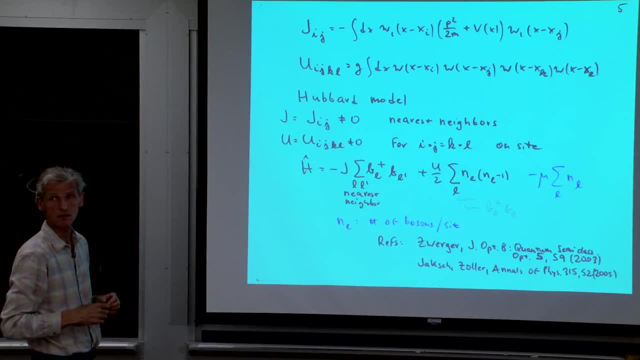 get a sum of a bunch of energy terms on every site that are sort of the same. So you have a common mode of energy that you can just Right, But then it's multiplied by the b dagger b. So in some sense it would have to be. 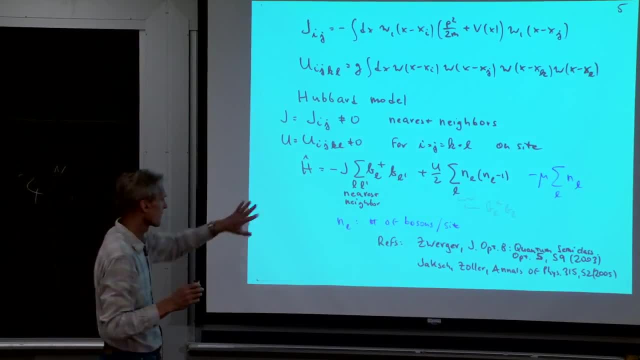 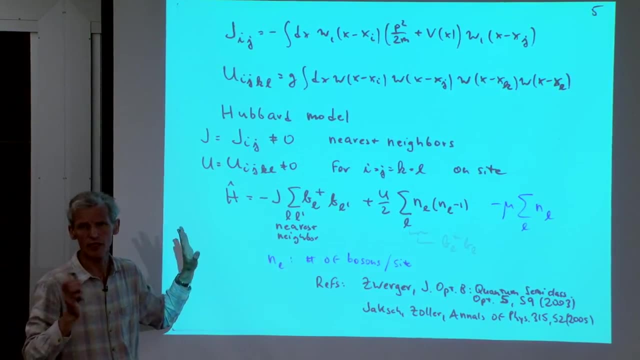 the chemical potential. My gut feeling is- and this is why nobody considers it- it's just the constant energy, which is probably something like the 0 point energy times the number of particles, which is not affecting any dynamics. It's pretty much a constant which can be simply dropped. 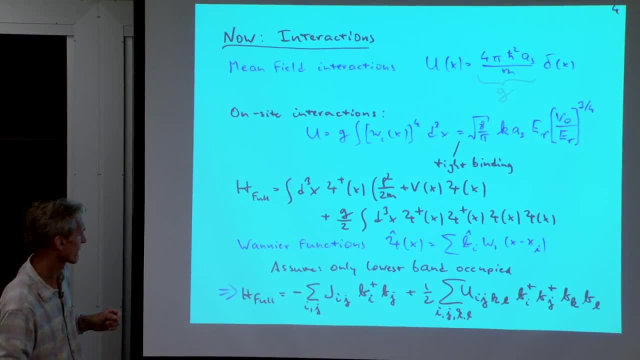 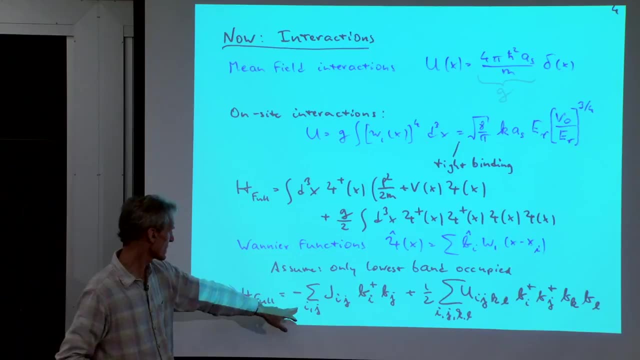 Let me just go back to that slide. I hope Let me just look up the reference. I haven't looked at it recently. When we do this exact transformation, there should be a reference whether i and j are. what happens when i equals j. 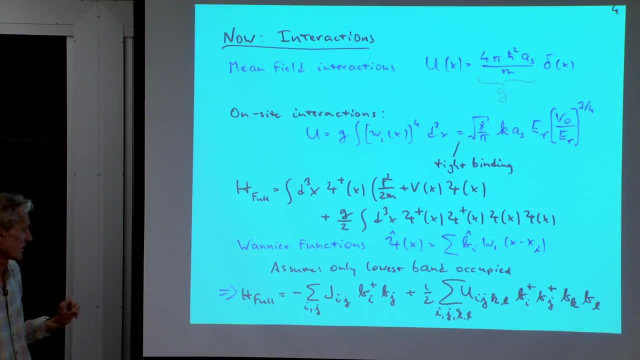 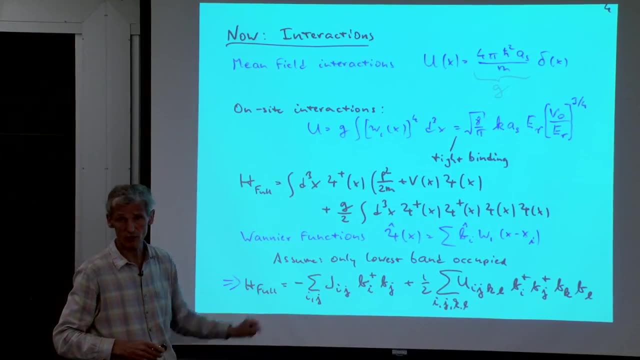 I think it's just a constant term, Because if you sum it over every single lattice site, so you get the number of particles times 0, point energy, Yeah, but even mathematically it gives just the constant term here, which is neglected. 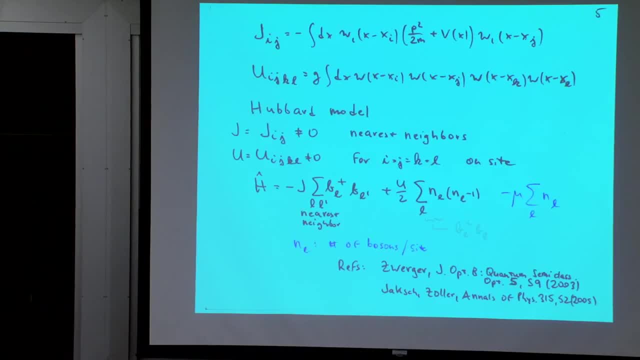 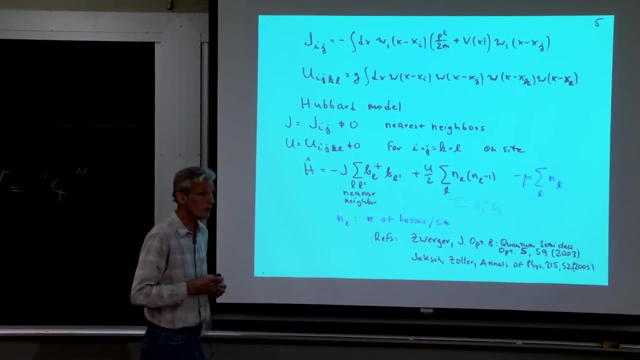 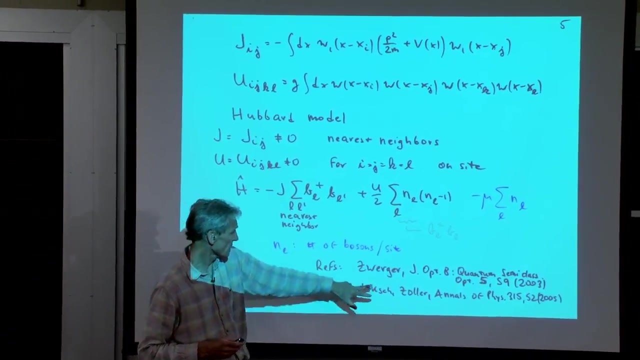 OK, Thanks, It was good to clarify it. OK, I think within the next 20 minutes I can step you through the superfluid to mode insulator transition. I'm first. references for what I've just said are given here. 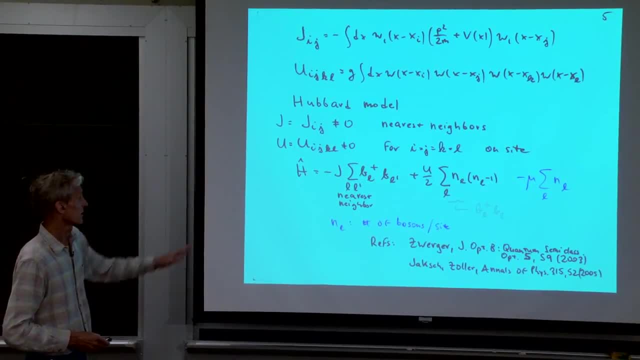 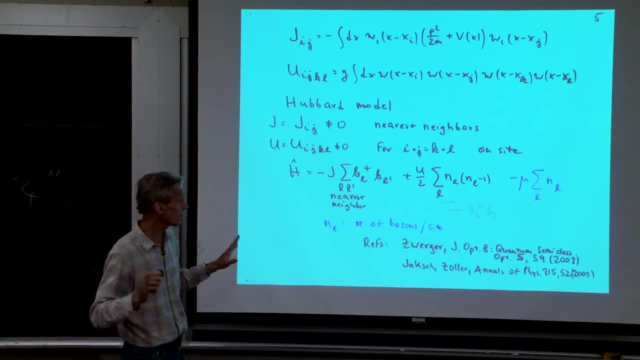 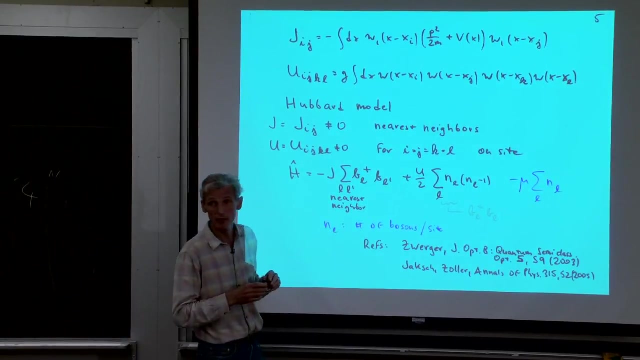 But let me now come take this Bose-Hubbard model and discuss. OK, it's two limiting cases. One case is where u is much larger than j. The other case is where j is much larger than u. These are the two limiting cases. 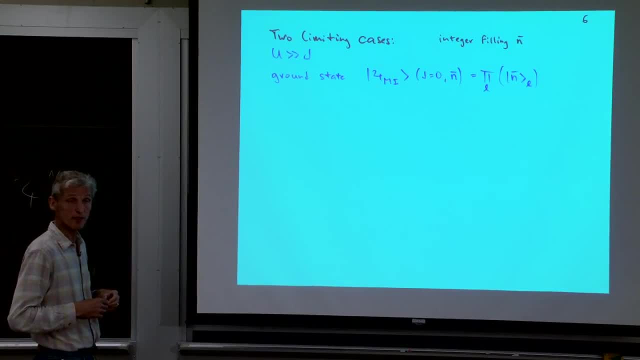 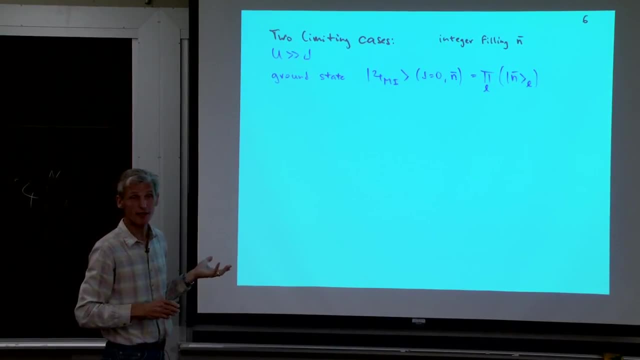 And it will turn out that one is an insulator and one is a superfluid. I mean, that makes perfect sense, of course. If u is much larger than j, I can set j equals to 0, if I can neglect it. 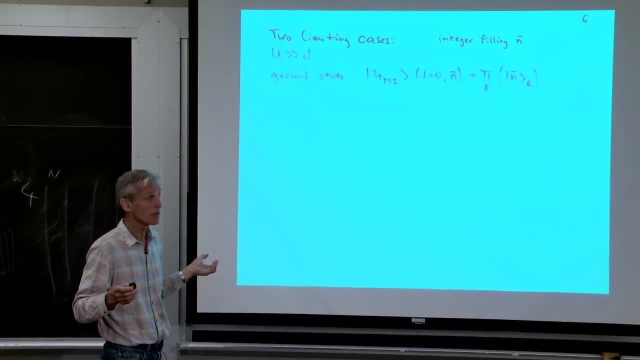 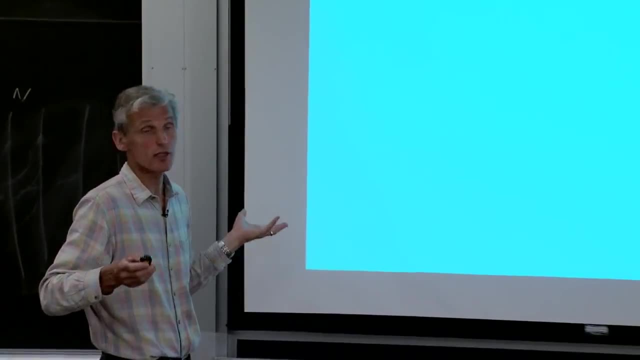 No tunneling means no transport and that means an insulator. OK, OK, OK, OK. It's very clear that when there is no tunneling, that the system is really described by a product of so and so many particles per site. 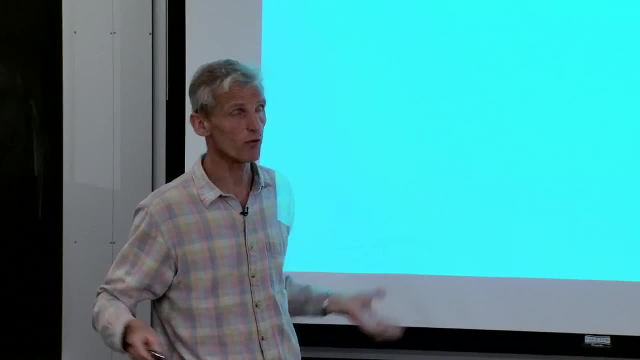 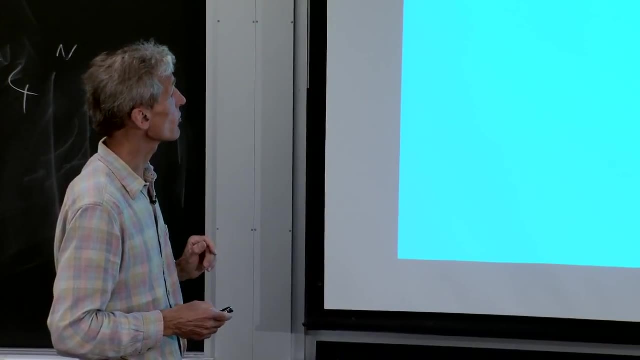 So it could be one particle per site and I have a product of over all sites or two particles per site. So this will be the ground state and it's called the ground state of the mode insulator. It's also trivial to discuss what 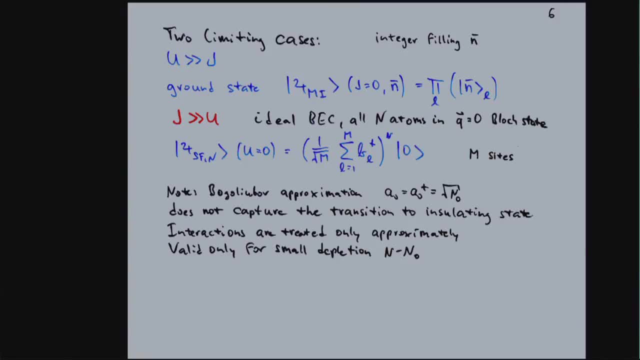 happens if j is much, much larger than u, because then I simply neglect u and I have a free gas. Well, a free gas of Bloch wave function, but it's the same as a free gas of planar wave function. 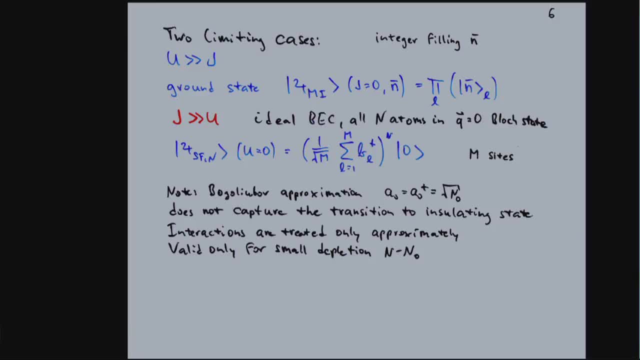 It's just that quasi-momentum replaces momentum And if you have just an ideal Bose gas in a periodic lattice, instead of Bose-Einstein condensation in the lowest momentum state, you have Bose-Einstein condensation in the lowest quasi-momentum state. 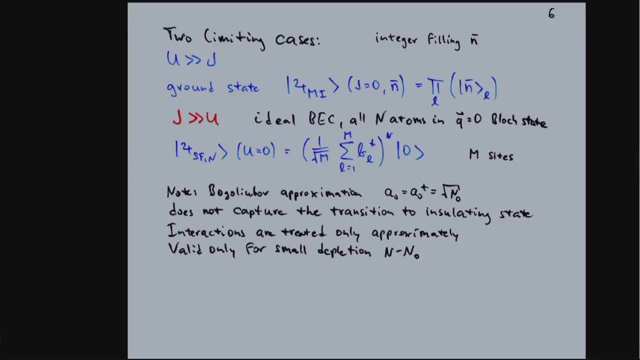 The lowest quasi-momentum state is a superposition of all Vanier function. I mean the zero momentum state in free space is a superposition of all position delta functions. The plane wave is delocalized And the lowest quasi-momentum state 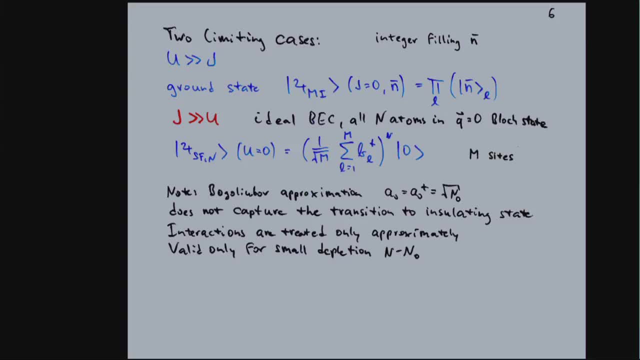 is just completely delocalized over all Vanier functions. But this is nothing else than the. q equals 0, quasi-momentum Bloch wave. The interesting question- And this has led to hundreds, if not more, papers in the literature- How do we go from one limit to the other limit? 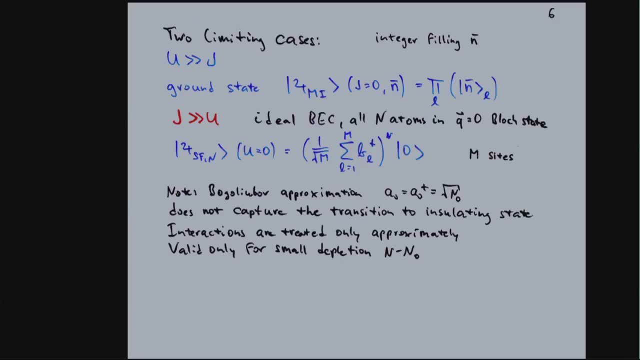 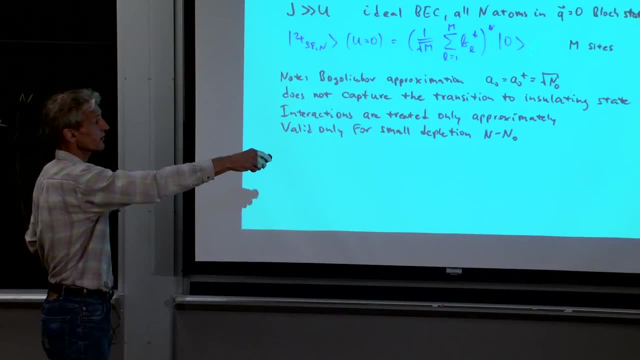 And now you would say, well, maybe we should use what has worked so well. We should use the Bogoliubov approximation. Just assume we have a condensate. Replace all those kind of a0 operators for the lowest Bloch waves. 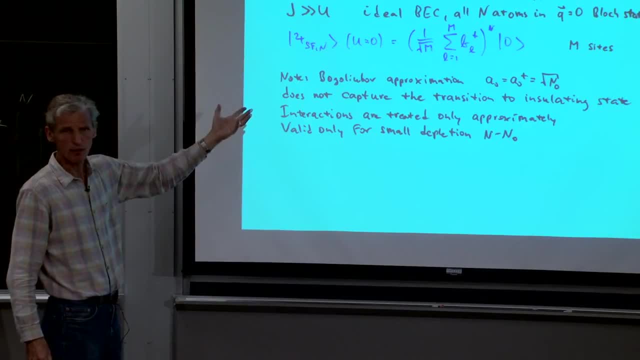 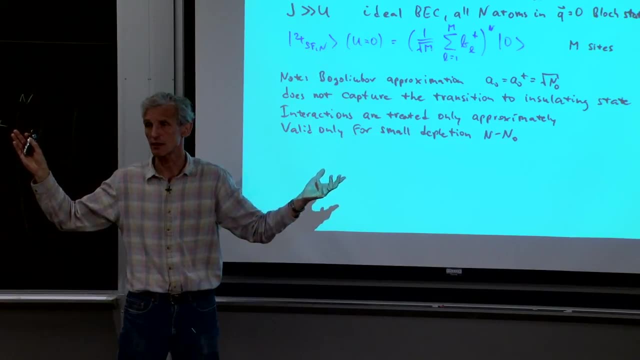 However, this doesn't work because the interesting thing here is To find the transition from the superfluid, from the Bose-Einstein condensate, to an insulating state. The nature of this approximation is that you need n0 to be large. 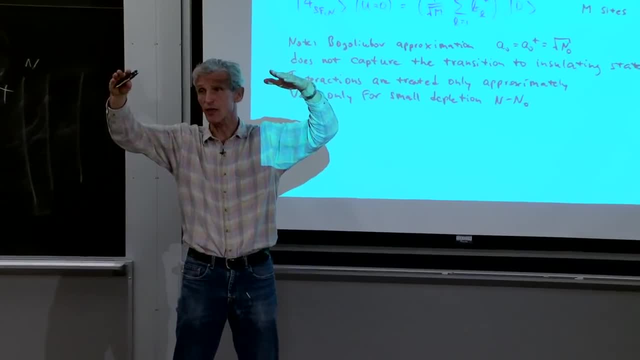 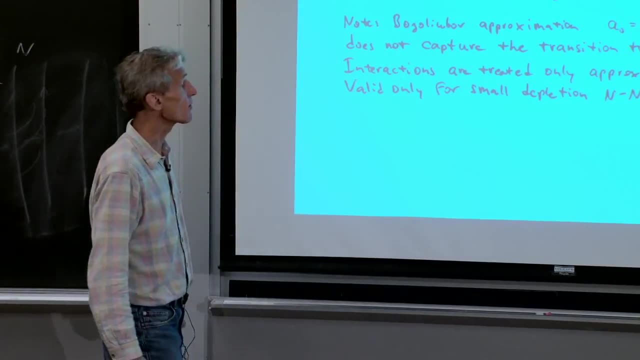 But we are interested when the number, when the condensate wave function turns to 0, and in the insulator it becomes 0. So we are actually interested in the opposite limit And indeed, if you would ignore everything I've just said, 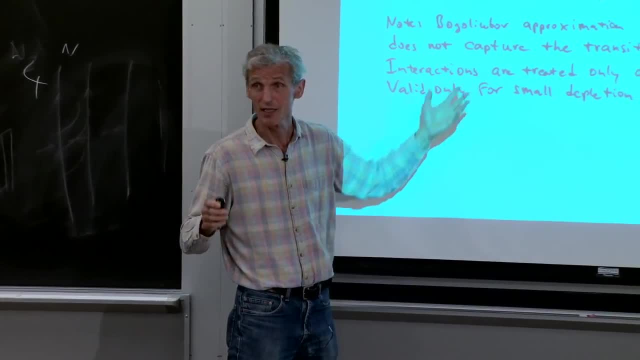 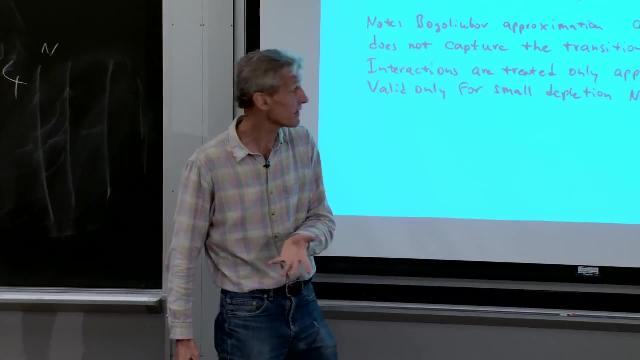 that it doesn't make sense to make this approximation. you make it nevertheless, You will find that you never get the insulating state, because you've pretty much eliminated the possibility to describe an insulating state by doing this approximation. So I want to show you now that we 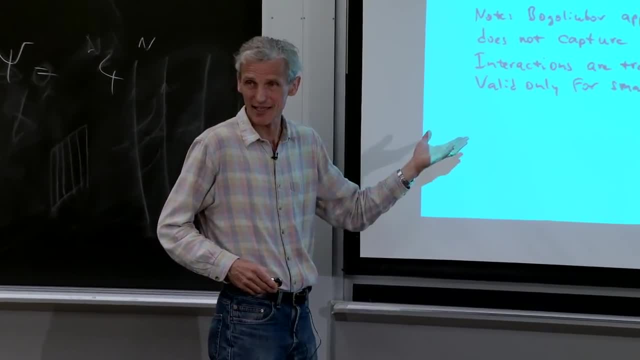 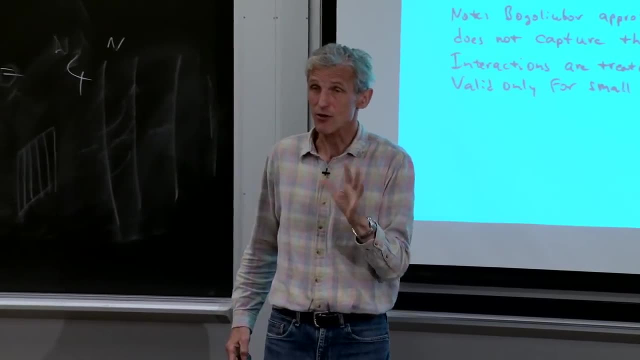 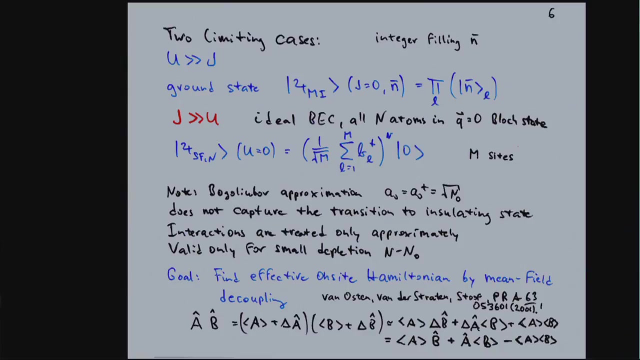 have to do another mean field approximation, which is actually nice. It's very different from this Bogoliubov approximation, But it's also mean field approximation which will describe our system. So the goal is now that I want to Find an effective Hamiltonian which 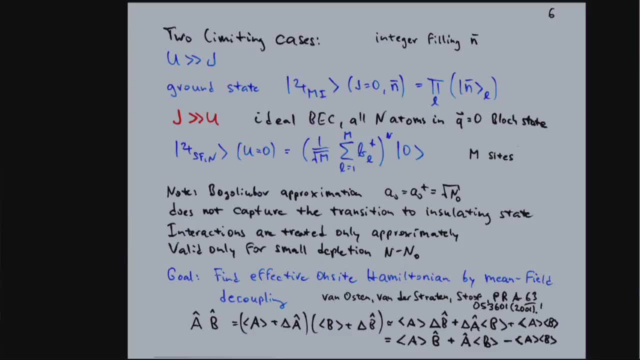 describes the transition from here to there, And the important approximation I will use is the following: Again, I have to get rid of operators. Products of too many operators cannot be solved, And so what I will do is I will use products of operators. 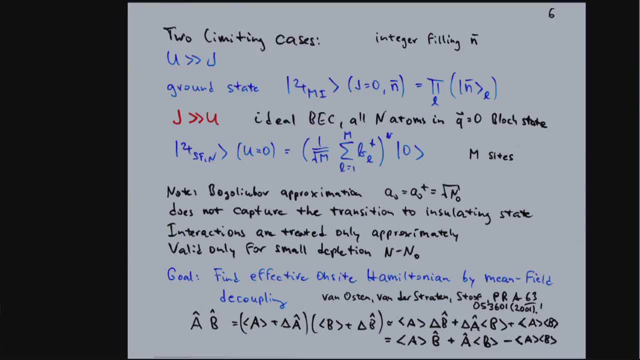 write them as average value plus fluctuations And then when I multiply that out, I take the product of the average values and I include the fluctuations in leading order. So I take delta A times B and delta B times A average, but I neglect the product of those fluctuations. 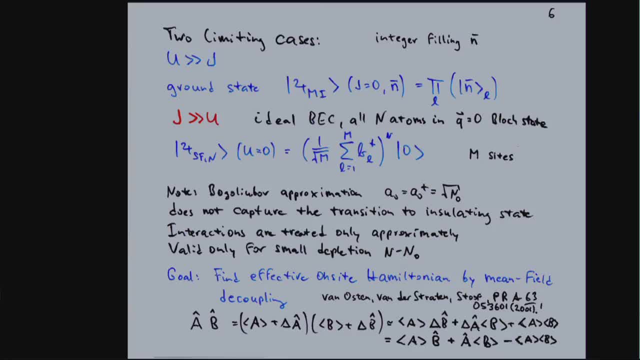 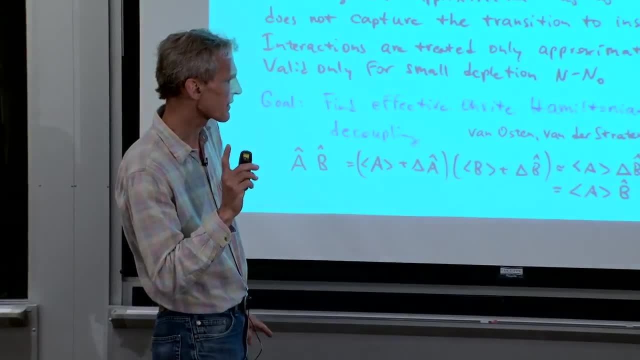 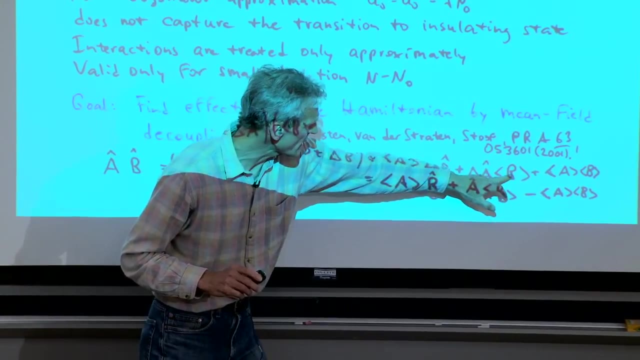 You can say I neglect the correlation of fluctuations here, So this is spelled out here. But since I want you to, the sign is important. Just look at this equation: A delta B plus delta B, with B plus A average times B average. 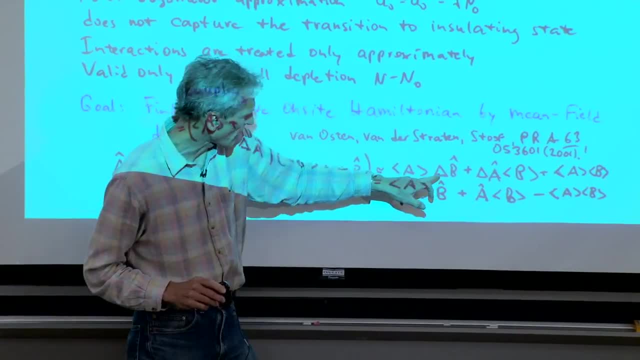 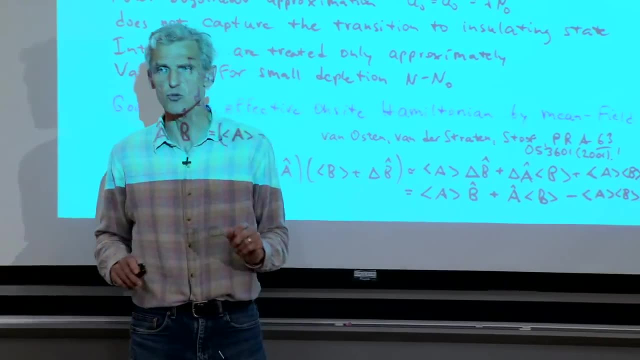 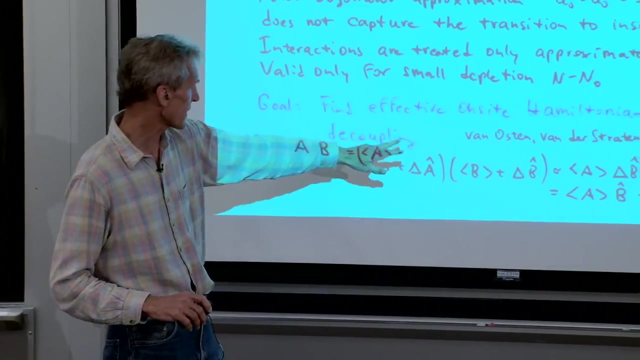 If I absorb A times B by upgrading delta B to B, but I do the same here- I have to subtract one product of the two average values. It's actually this minus sign which will play a role later, But here you see already that I will. 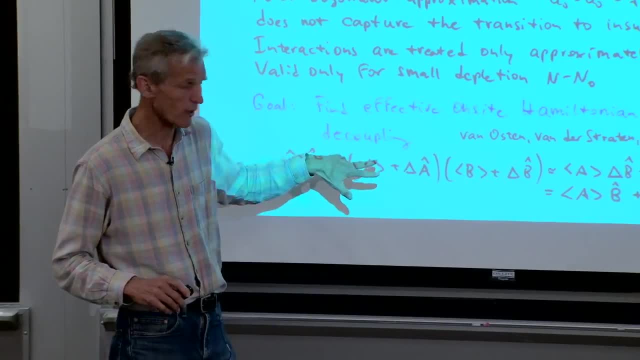 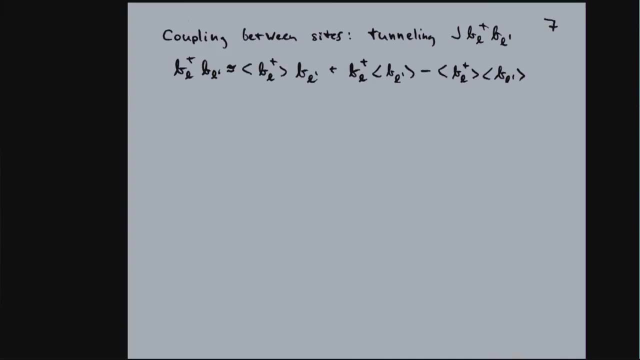 make this decoupling approximation, that I decouple the fluctuations from each other And I write it in this way. There is an important minus sign. OK, so we want to start in the insulating state and want to figure out how does the system develop superfluidity? 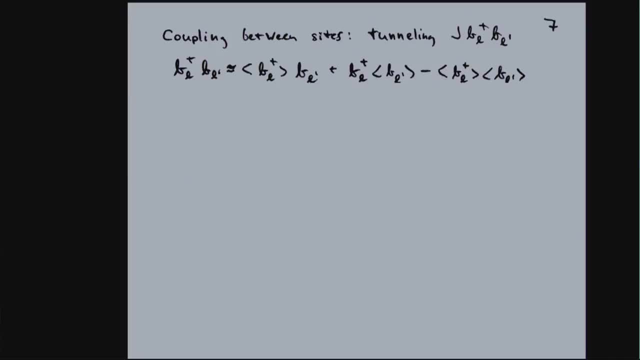 out of the insulating state, And the perturbation operator which takes me out of the insulating state is tunneling. So therefore, the operator which is responsible of breaking out of the insulating state is the operator which induces tunneling between neighboring sites. 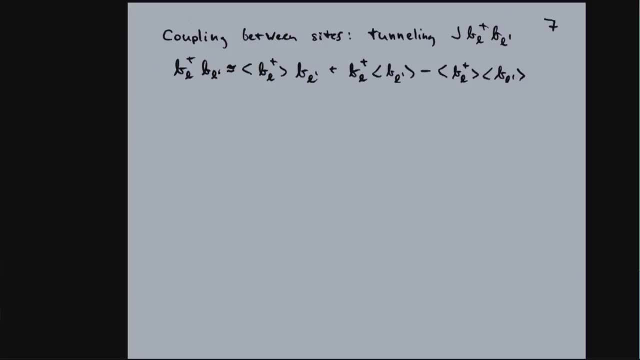 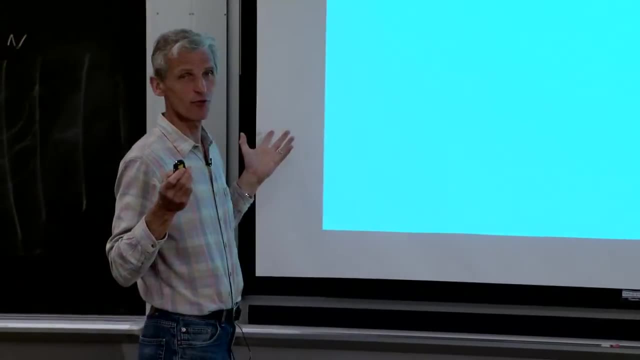 And the tunneling operator in this Hamiltonian. remember the Bose-Hubbard model had J times B, dagger B, This was our tunneling term. This involves now products of operators And I told you we want to get rid of products of operators. 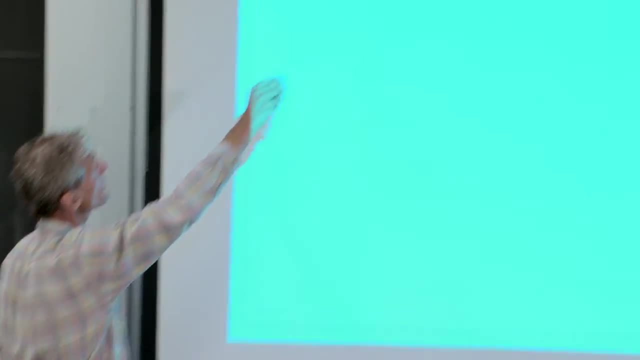 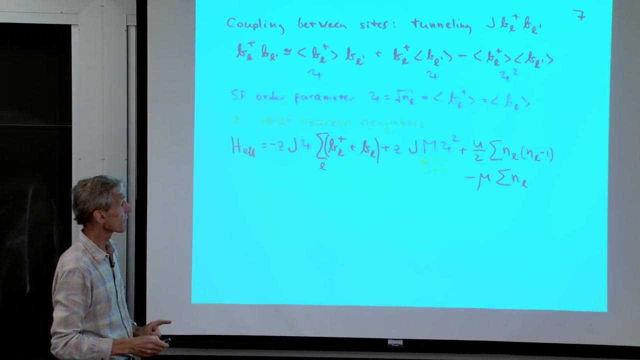 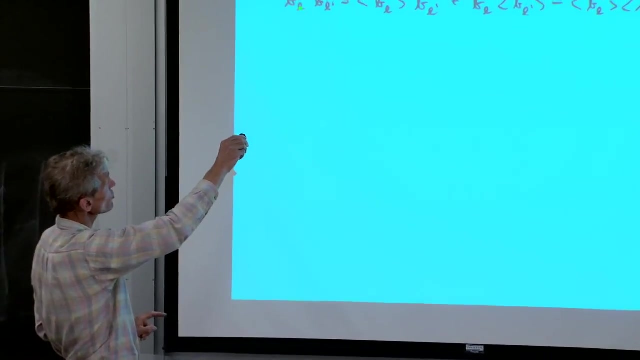 to get something we can easily solve. So we use now this product of operators, Operators on two neighboring sites, And we use exactly this decoupling approximation. So therefore, we replace each operator by an average value And we neglect the product of the fluctuations. 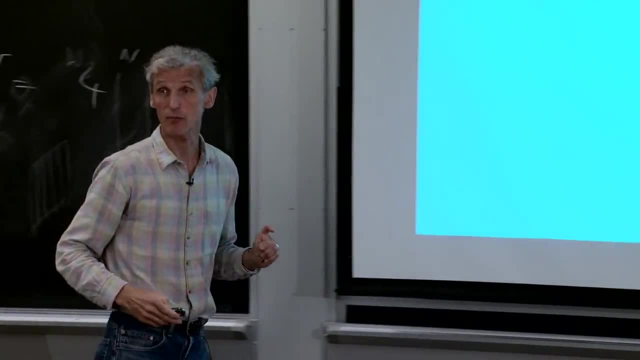 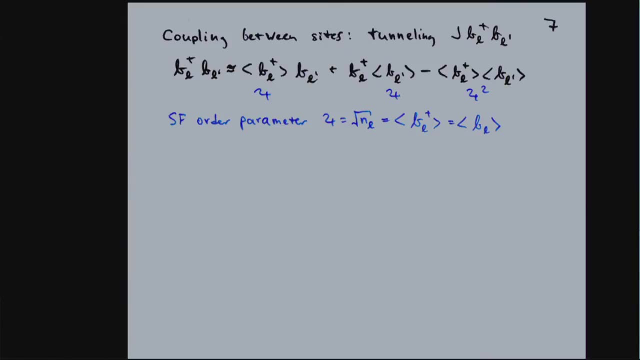 And then we obtain this And I've explained to you where the minus sign came from. So now I call this average value Of the operator BL, I call the superfluid order parameter psi. I think I could have chosen psi to be complex. 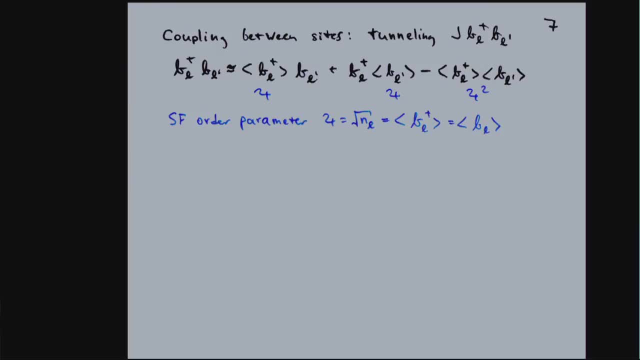 And then BL, dagger, BL would have complex conjugate, But it is sufficient here to restrict the discussion on real numbers And it makes the notation simpler. So anyway, so I introduce that, And what happens now is the following: That I have my Hamiltonian. 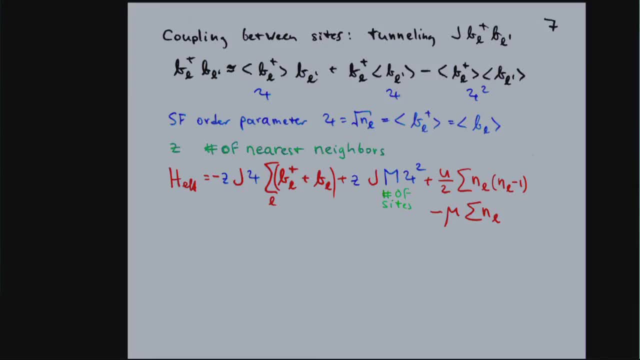 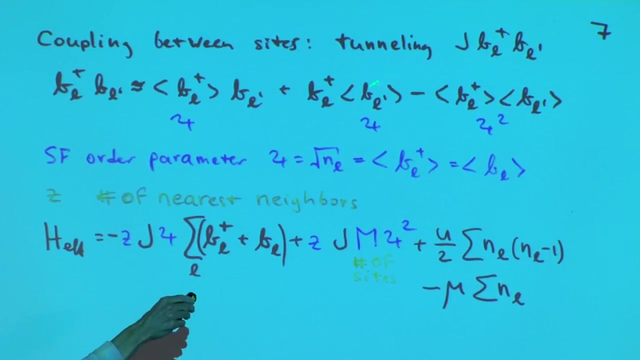 The Hamiltonian had the interaction energy, But the tunneling term is now very simplified Because instead of tunneling from one side to a neighboring side, The other side is sort of absorbed by the mean field, by the superfluid order parameter psi, And therefore- and this here gives me- 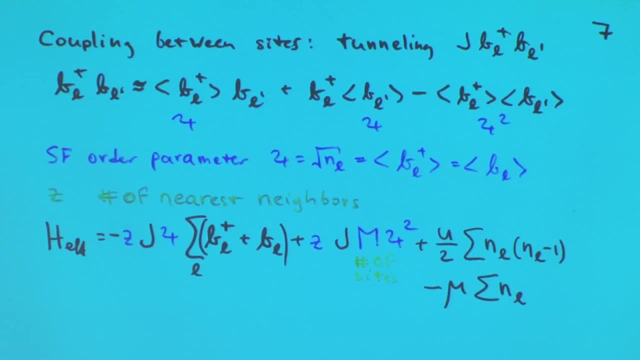 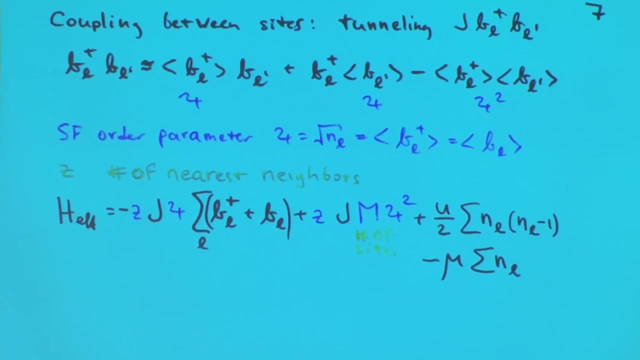 a psi square term which appears here. Trust me, this is just an identical rewrite of the previous Hamiltonian by using this decoupling approximation. So well, what we want to do, what we have gained now, is something really dramatic. 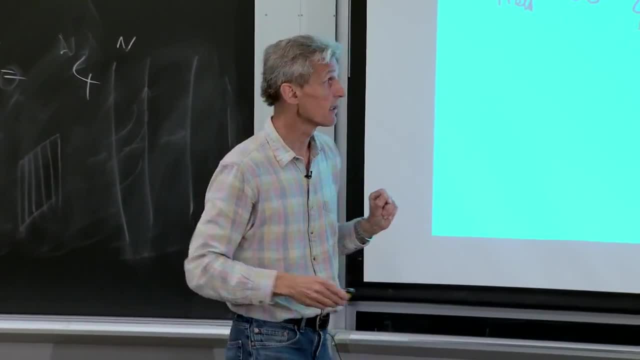 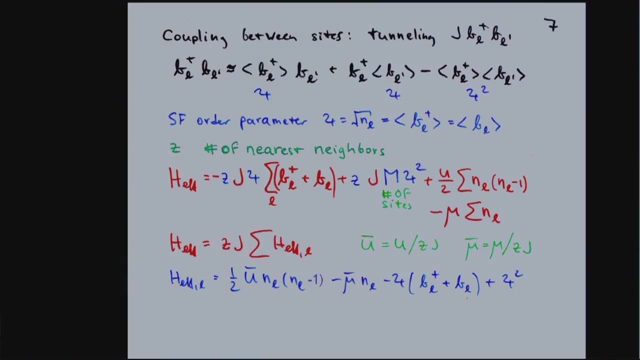 We had sort of many sides and tunneling from side to side. But if you look at it now, we simply multiply the effective Hamiltonian. We take the sum of the effective Hamiltonian over side index L, So our effective Hamiltonian is now: 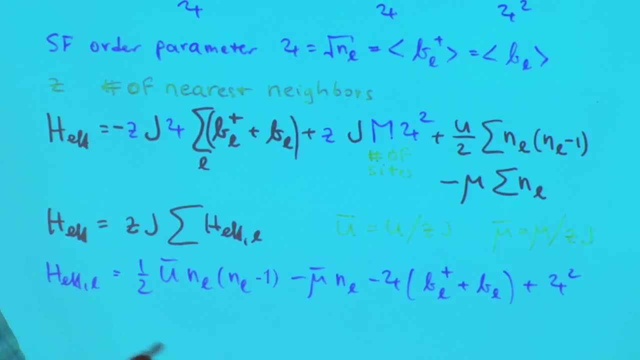 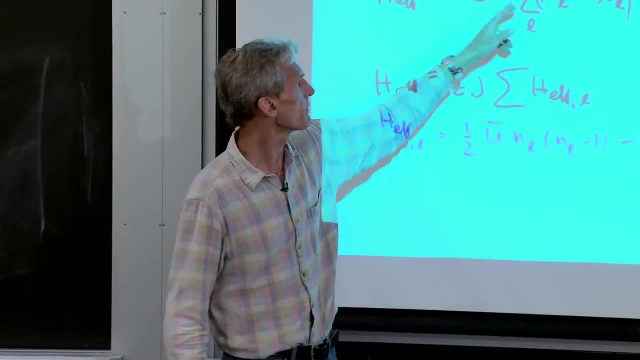 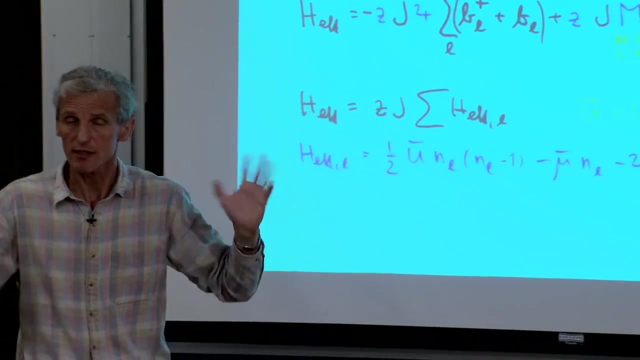 the sum of an identical Hamiltonian per side. The sides no longer interact with each other. Each side interacts with all the other sides Described by the mean field, by the superfluid order parameter psi. So therefore, our many-body problem, which is still a many-body problem. 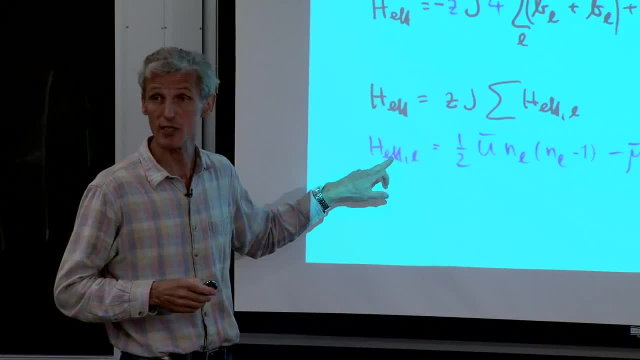 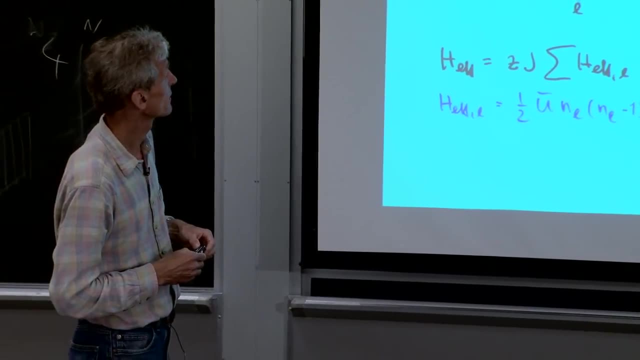 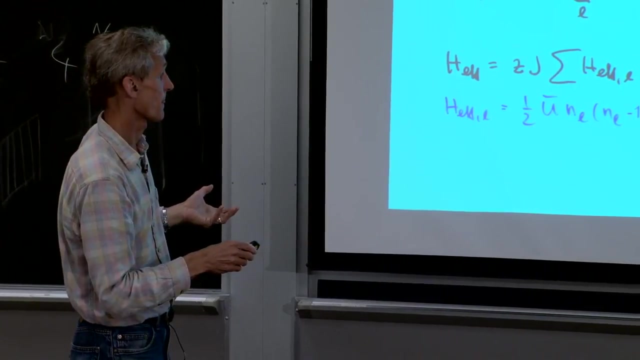 but has turned into an effective Hamiltonian for each side, Because each side has the same Hamiltonian. Colin, What happened to the j psi squared term? This here? Oh, OK, Sorry, OK. So here is now So I can say. 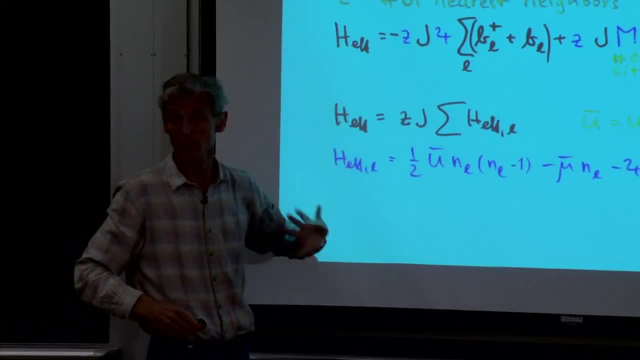 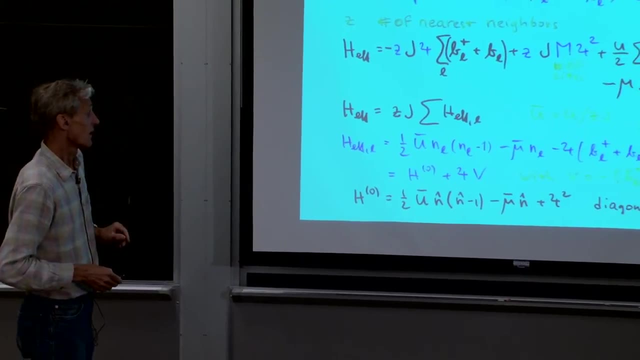 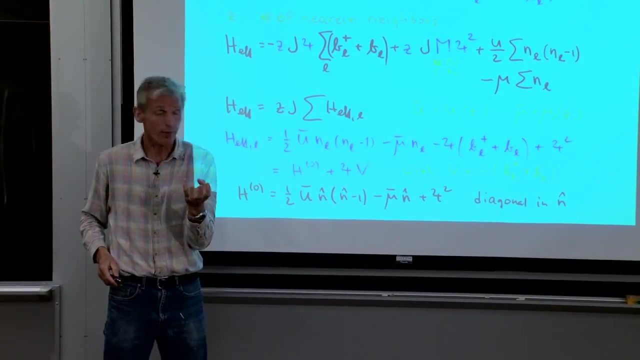 Instead of solving for the sum, I can just solve for each side individually, And this is now my effective Hamiltonian for each side. Now I want to catch the onset of superfluidity, So I want to get this system when psi is small. 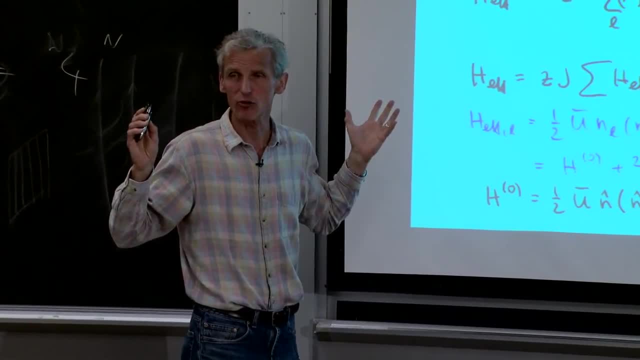 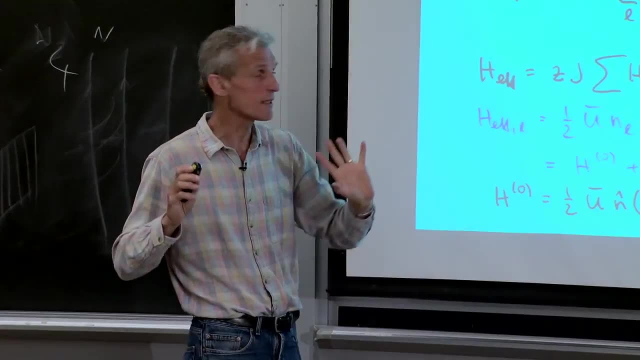 And therefore I can just ask. I don't know what psi is, It's part of my solution, But I'm interested in the moment when psi begins to take off from 0, when superfluidity emerges. So what I can therefore do is I: 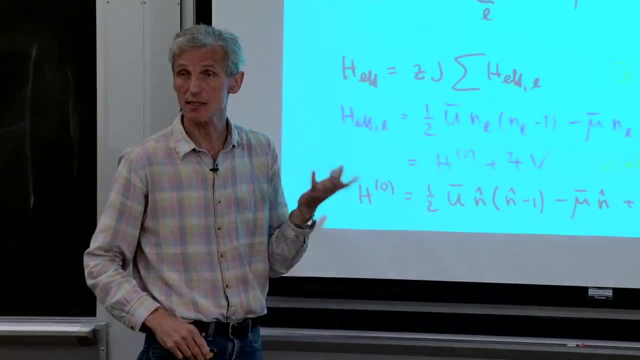 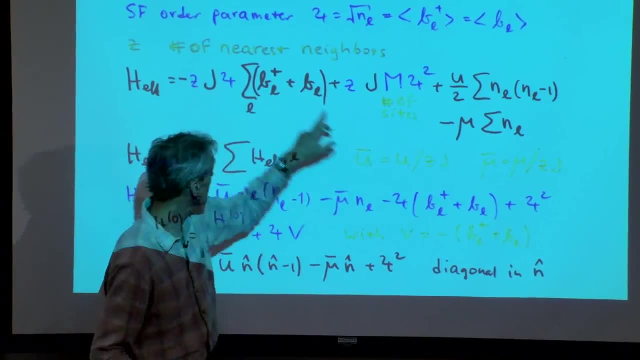 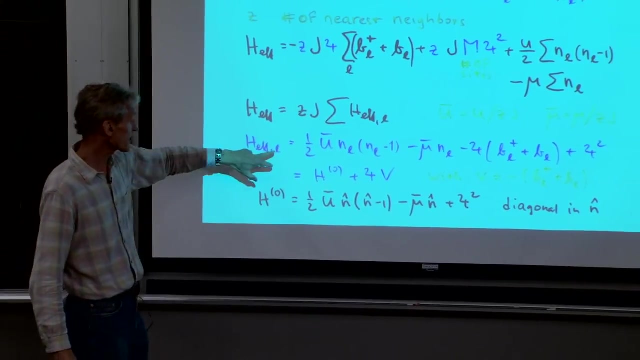 can regard psi as an epsilon parameter, as a small parameter, And the psi parameter comes with an operator v, And this operator v is nothing else than b l dagger plus b l. So in other words, what I'm doing is I'm separating my Hamiltonian into a Hamiltonian which is 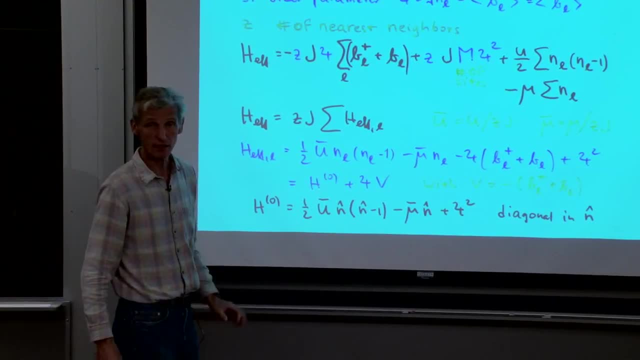 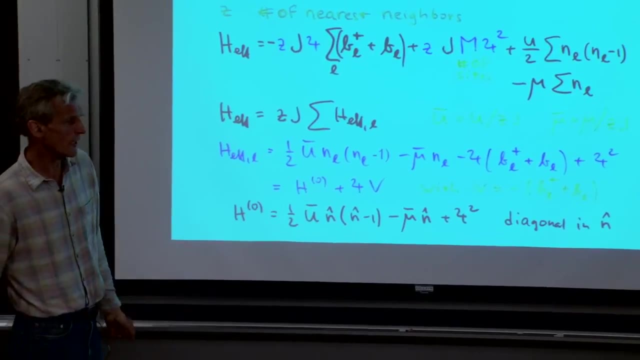 diagonal. It's diagonal in the quantum numbers of the isolating state, Just one, two, three particles per side, And psi square is a z number. The psi square is also diagonal in that. And now the possibility of tunneling, the possibility of superfluidity. 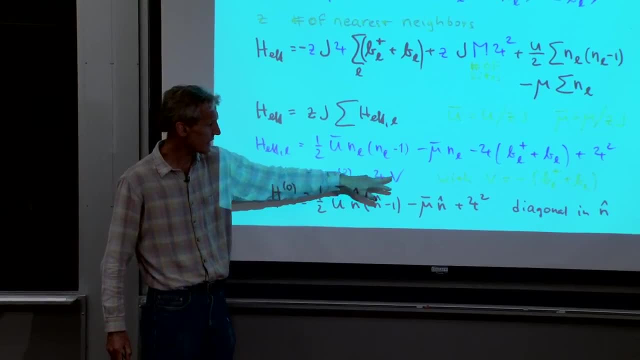 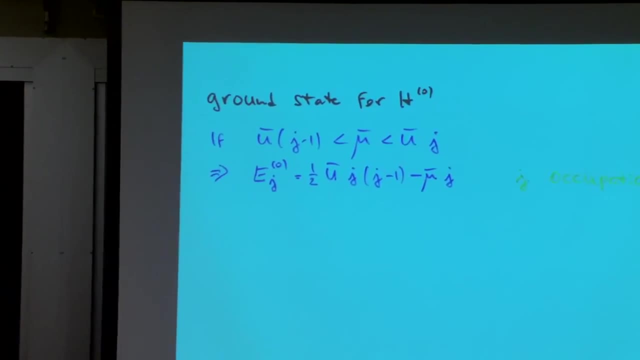 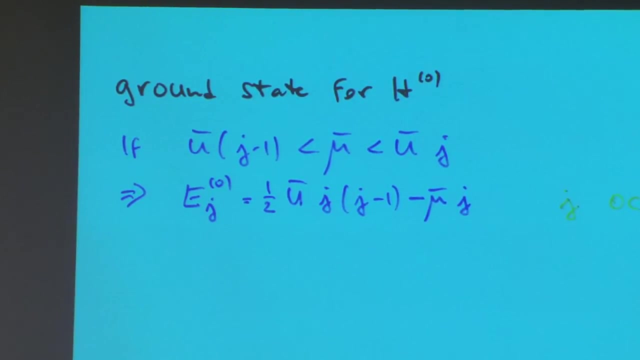 is now perturbative in this term: psi times v. OK, I don't want to explain actually this expression, It just formalizes. I need it as an intermediate step When we have the chemical potential and we raise the chemical potential. 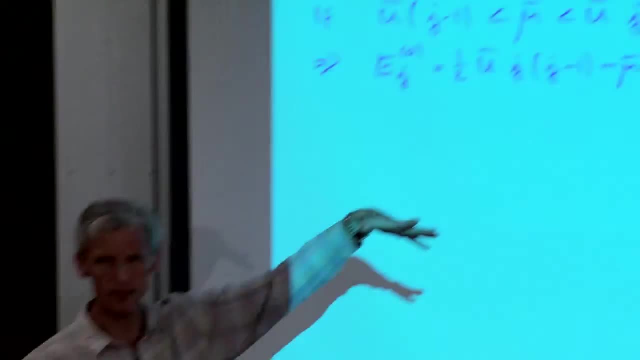 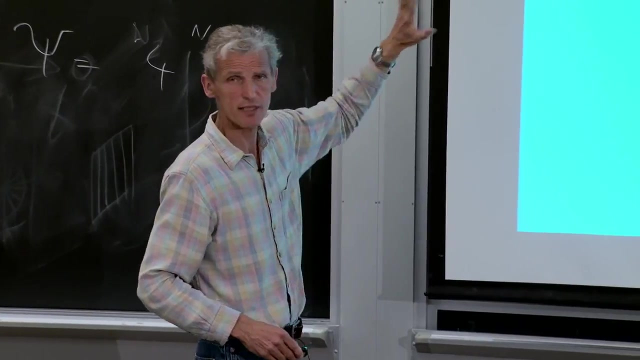 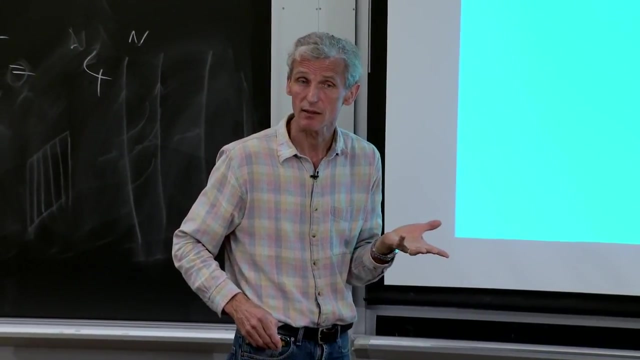 we go from 0 to 1 particles per side to 2 particles per side, And whatever the chemical potential is determines whether we have 1 or 2 particles per side. This is just telling me, as a function of chemical potential, what is the ground state of the insulator. 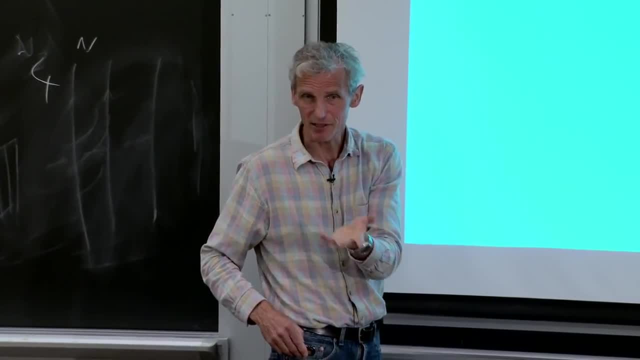 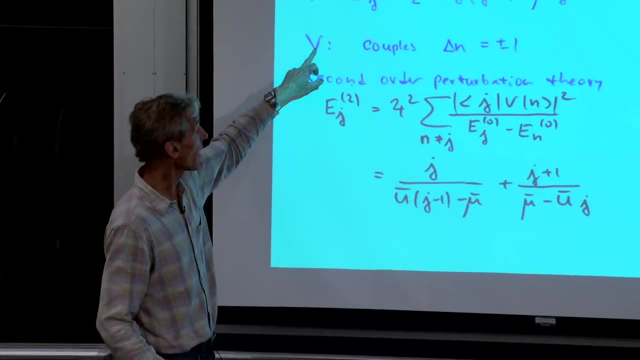 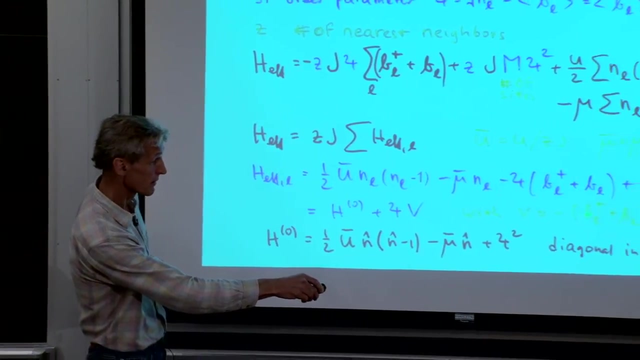 So now we take this ground state. It's actually much easier described in words than by this formula. We take this ground state and do perturbation theory in our term psi times v. Remember the operator is b, dagger b And the epsilon is psi. 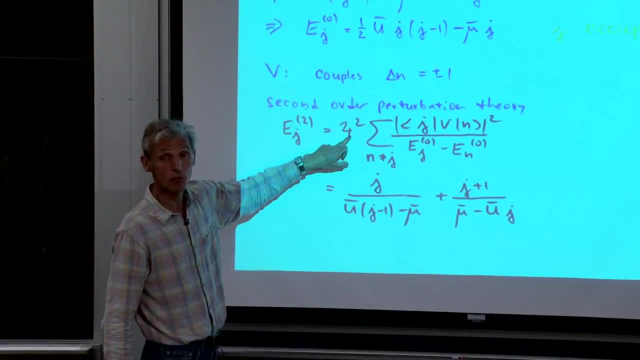 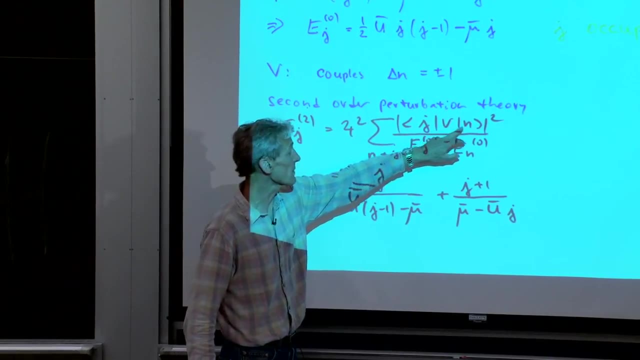 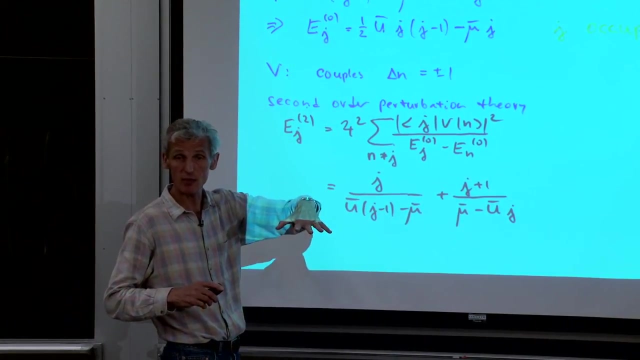 So in second order perturbation theory, we get psi square And then v, because it's b. b dagger is very simple. It only couples one side to the next. It couples one occupation number, n to n plus 1 and n minus 1,. 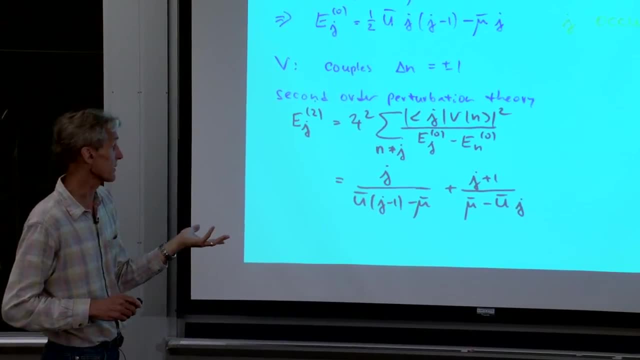 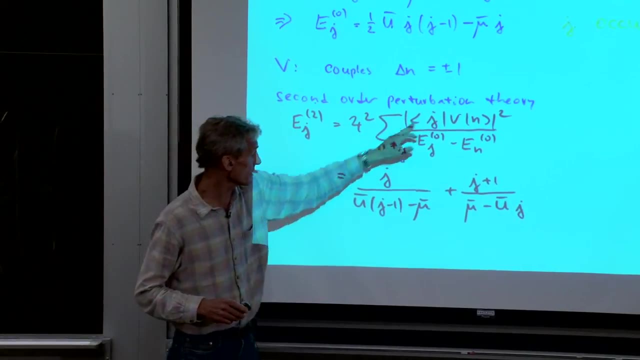 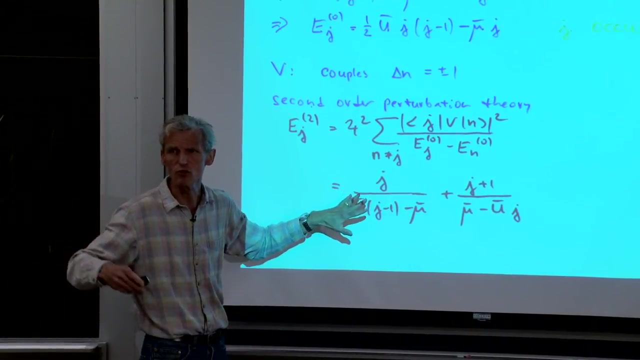 because b and b dagger destroy or create a particle per side. So therefore I can immediately write down what this matrix element is. in second order, perturbation theory. I mean these are all. sorry, it's all defined here. I know I'm losing you now. 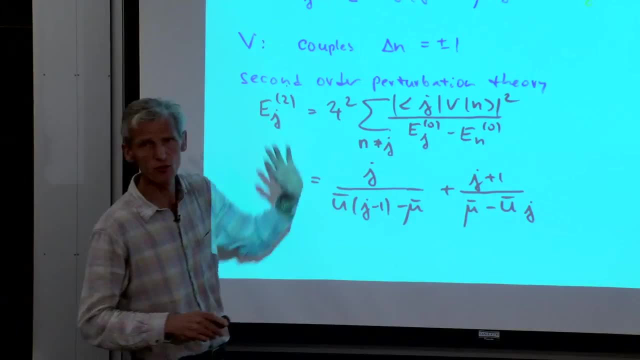 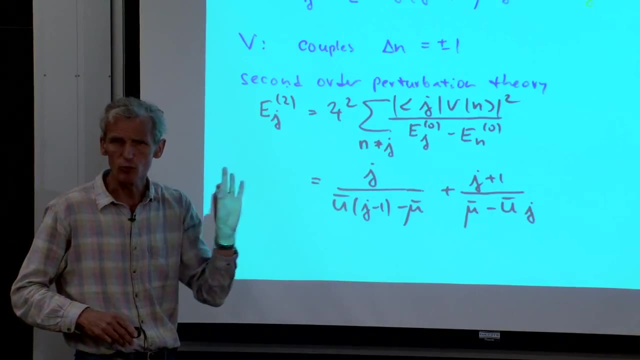 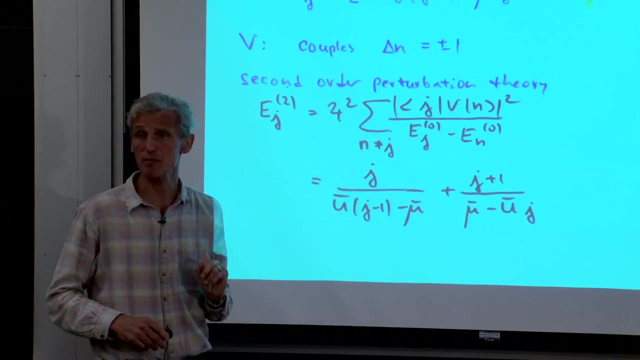 Nobody will tell me what is the difference between u, bar and u, But it's trivially defined. So the idea is we have the isolating system, We do perturbation theory in tunneling And the perturbative operator is psi times b plus b dagger. 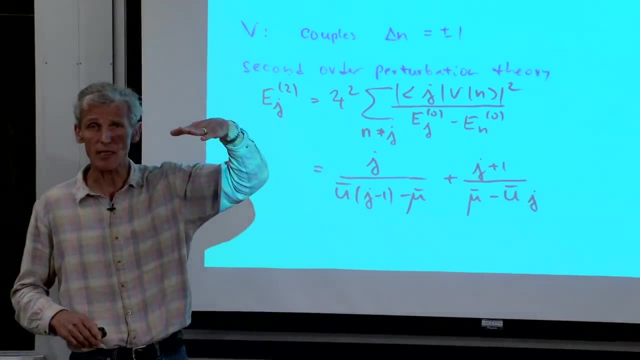 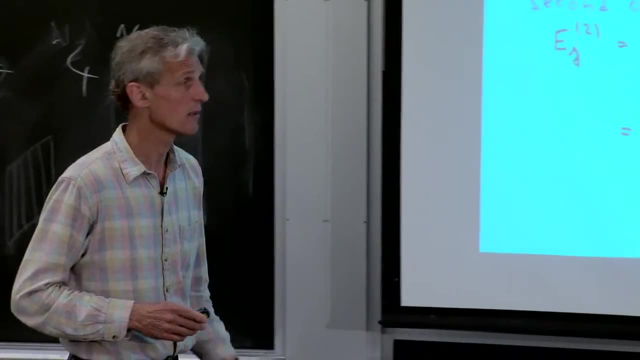 The b plus b dagger matrix elements are trivial because they admix to n particles per side n plus 1 and n minus 1.. And this is what we've done here. And the j's are just occupation numbers. The j is the occupation number of our side. 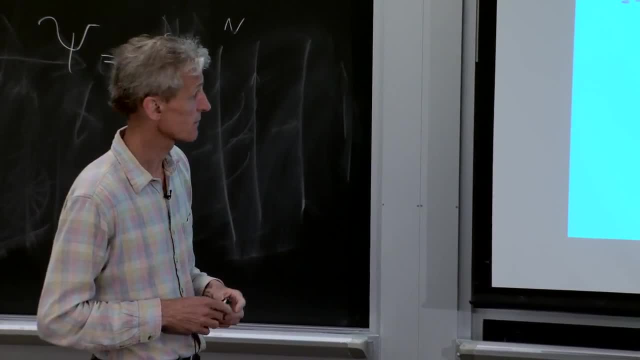 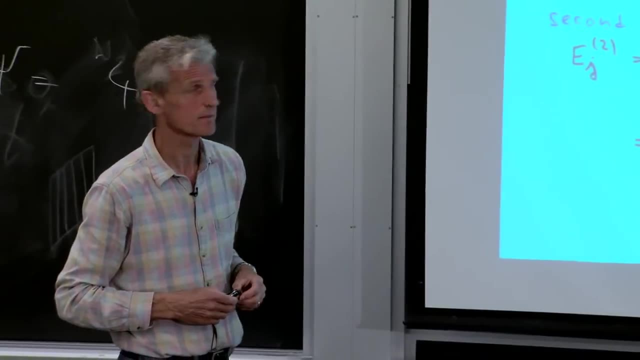 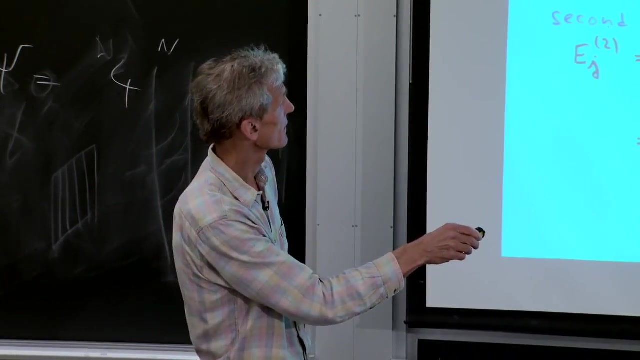 I have two questions. So in the bottom equation, what happens to the psi squared? Sorry, this is the sum. that psi squared is missing. I guess it's the same question for the equation next to the green thing. Is there supposed to be a psi squared in there? 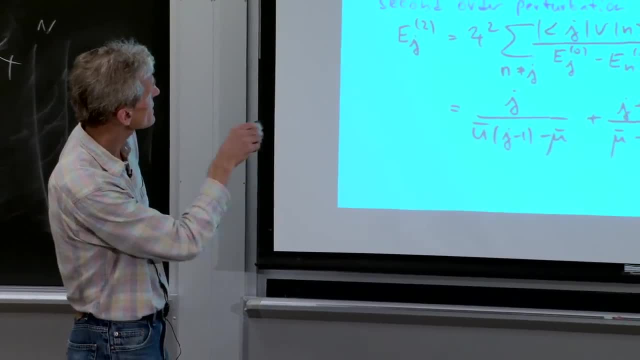 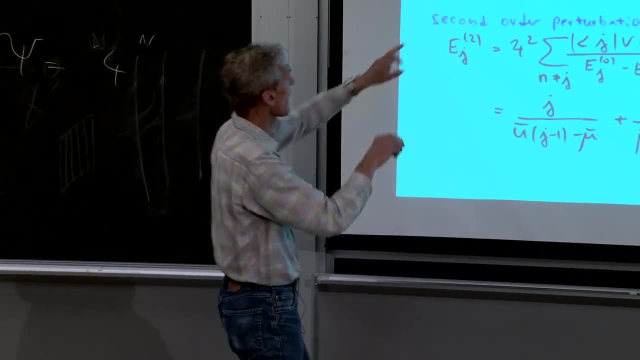 Originally there was a psi squared in the h0.. No, this is the ground state where psi is 0. And now we do perturbation theory in psi v. So we pretty much use. These are the unperturbed energies which appear in the energy denominator. 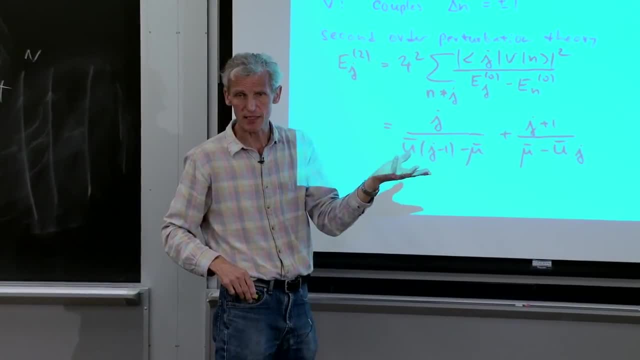 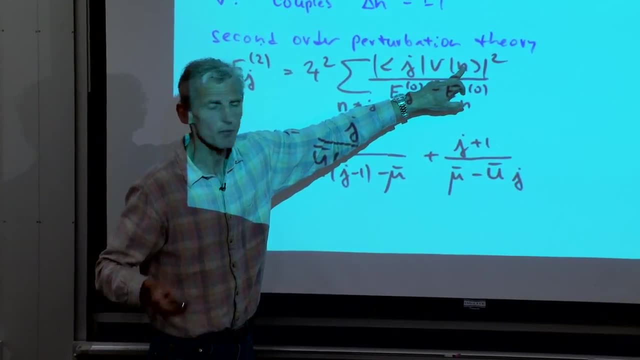 The wave functions we are using are Fock states, number states per side, And here we couple occupation number j to all possible n's. But because of b and b dagger, n has only two values: j plus 1 and j minus 1.. 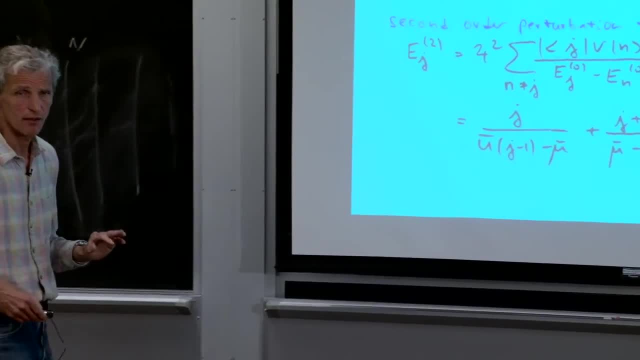 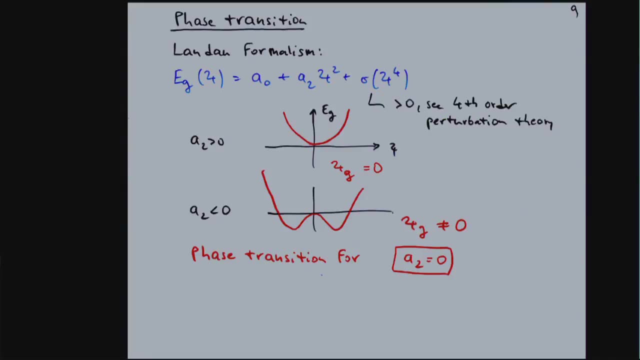 And this is what's given here. It's mathematically trivial. The notation is more complicated than the physics behind it. But now comes again. I think I need five more minutes and I'm done. But now comes the interesting physics. We have to ask: what are we doing here? 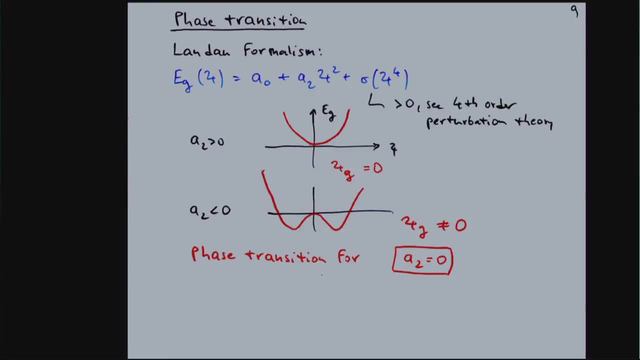 I mean, it's all mathematical And the math is really simple here. What we have done is we have looked at the isolating state And we have done perturbation theory in psi times b plus b dagger, And now we get an energy correction which is psi squared. 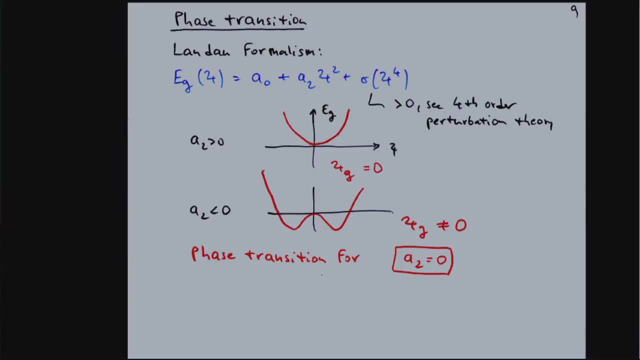 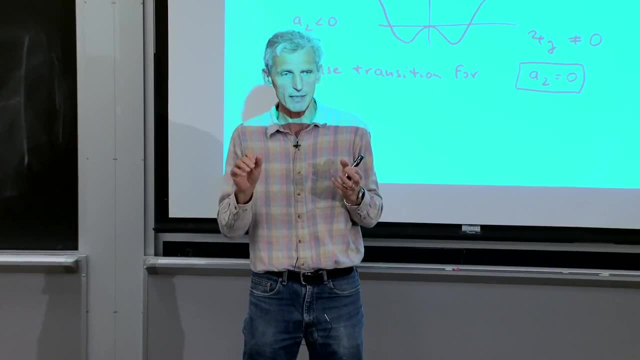 And what are we really doing here? Well, you can say the following: We started with the hypothesis that we have a superfluid state characterized by psi, And psi at the onset of superfluidity is small. But now we have done the calculation. 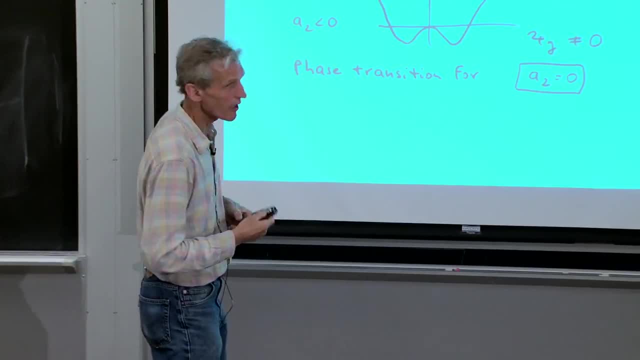 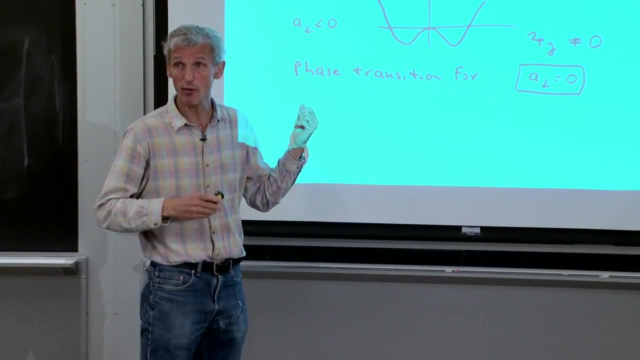 assuming that there is a psi. But now we are turning around and said: have we really done the system a favor by introducing superfluidity? In other words, has our perturbation theory in psi lowered the energy of the state or raised the energy of the state? 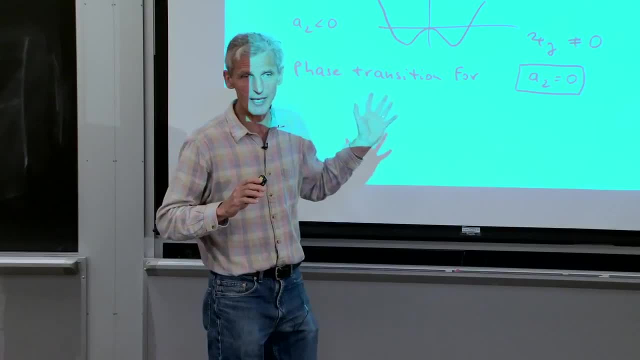 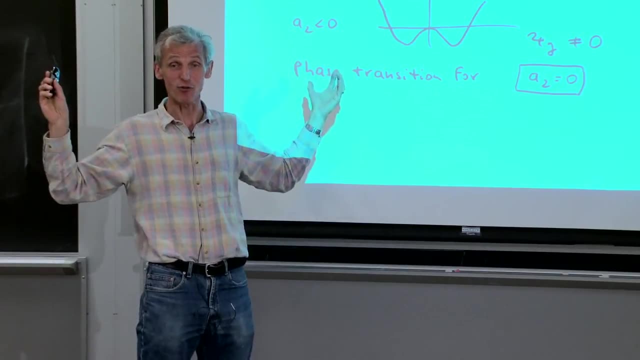 So in other sense, In other words, we've done a hypothetical calculation- Hey, what would the system feel like if there were a little bit of superfluidity? If the system says, great, I've lowered my energy, then we know we are in the superfluid state. 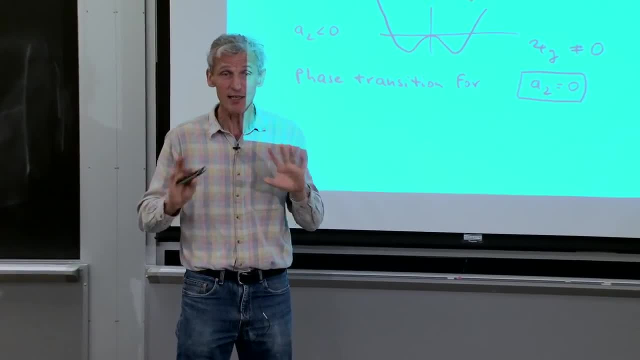 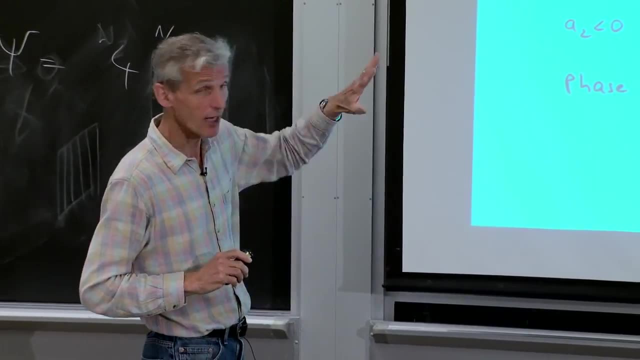 When the system says no, I raised my energy because of the psi, then the system has rejected our idea to introduce superfluidity. So therefore, the question we are raising now is: after we've done the calculation, for what values of u and j is it? 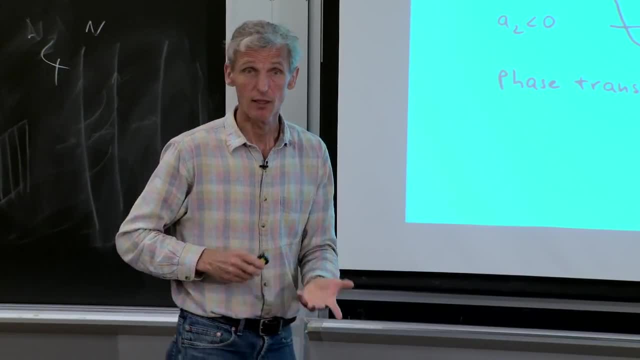 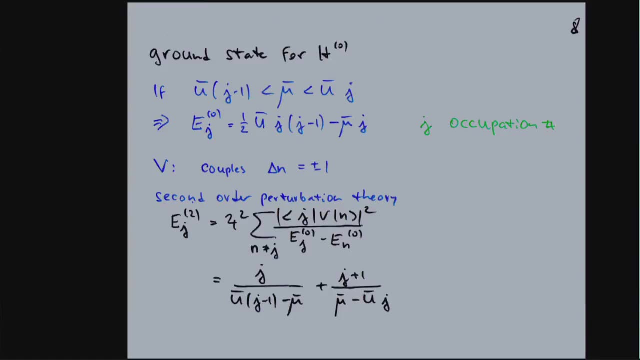 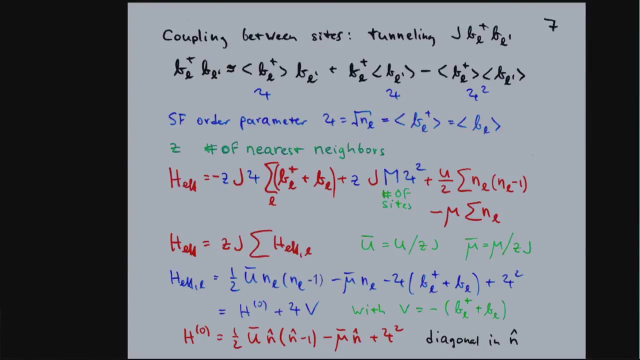 favorable to introduce a psi or not? Now I was expecting the question of some of you that in second-order perturbation theory. second-order perturbation theory always lowers the energy. But remember, this is why I emphasized the minus sign- We had a psi squared term which came from that. 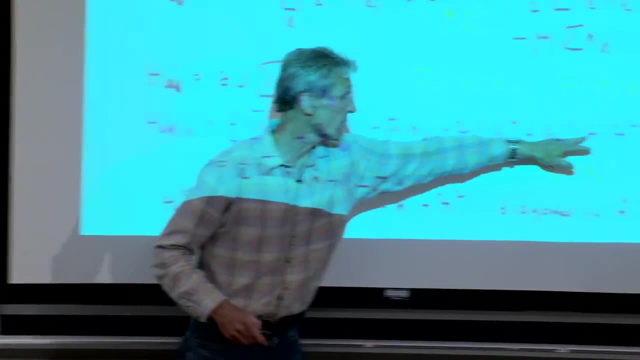 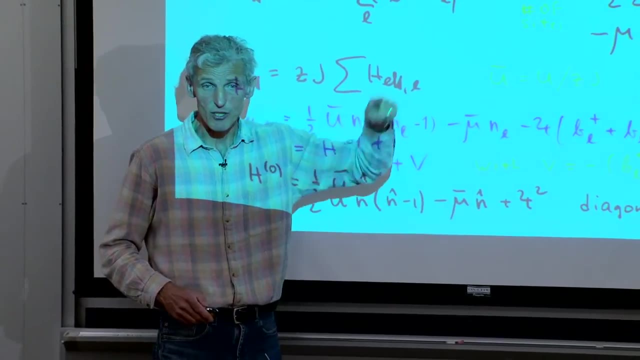 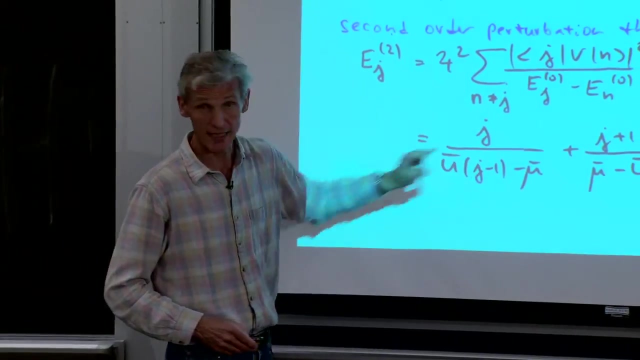 which came from the last term of the decoupling approximation, which had a minus sign, And therefore we have in psi squared one term which came from this special sign, I emphasized in the decoupling approximation, And we have a contribution of psi squared. 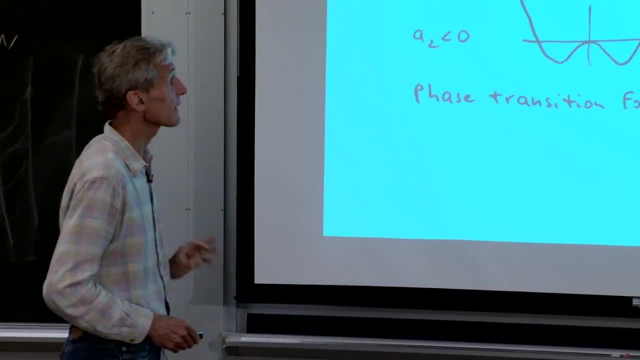 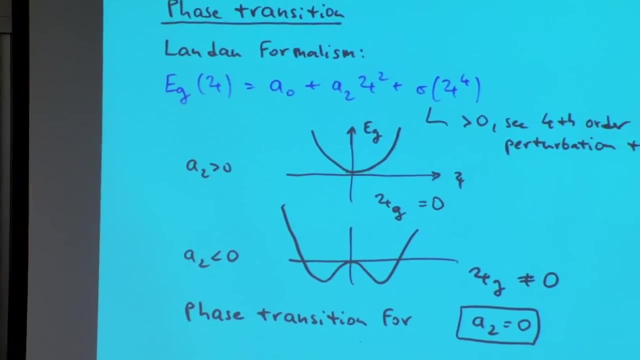 which comes from perturbation theory, And the two together can actually change their sign. So what we have right now is, if we describe the ground state as a function of psi, we have our unperturbed energy of the mod-insulating states And then we have a term in psi, squared. 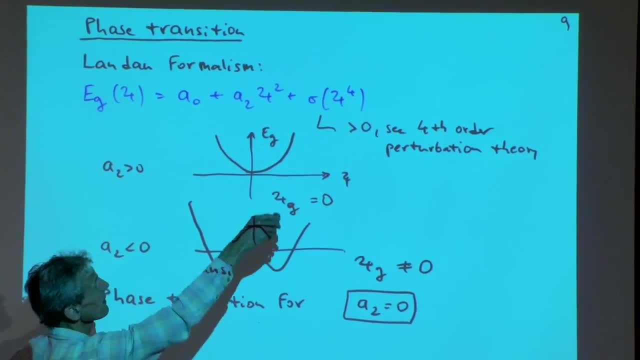 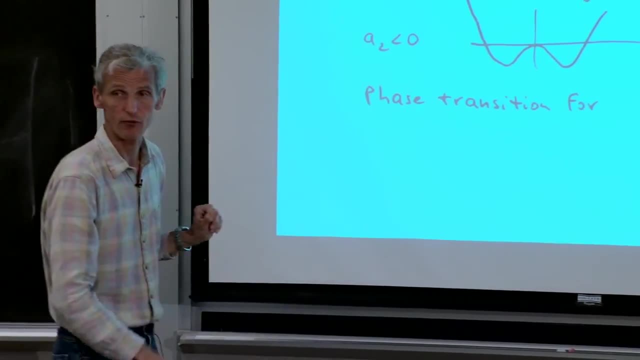 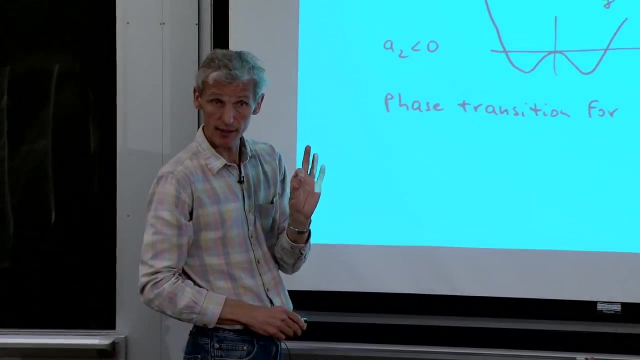 We should and we could, but we don't calculate the next order in psi, to the 4.. And it turns out that in fourth-order perturbation theory this term is always positive. So what happens now to the total energy when this term a2, which we have exactly calculated? 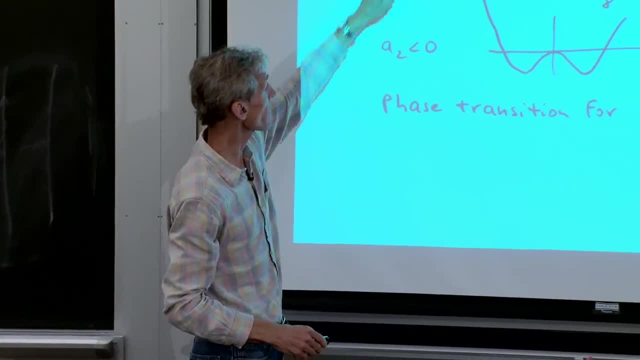 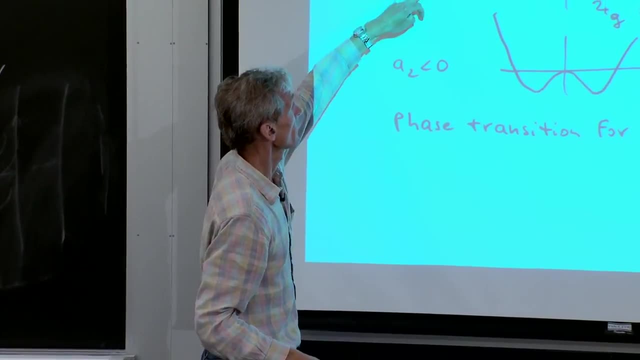 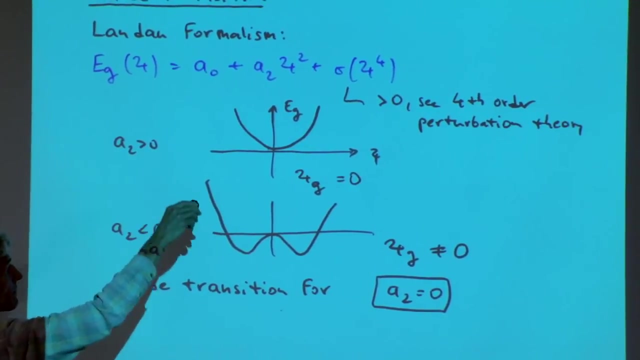 analytically calculated if this term, a2, is larger or smaller than 0?? Well, if you have a parabolic term and a quatic term, in this case, both the quadratic and the quatic term are opening up like in a u-shape. 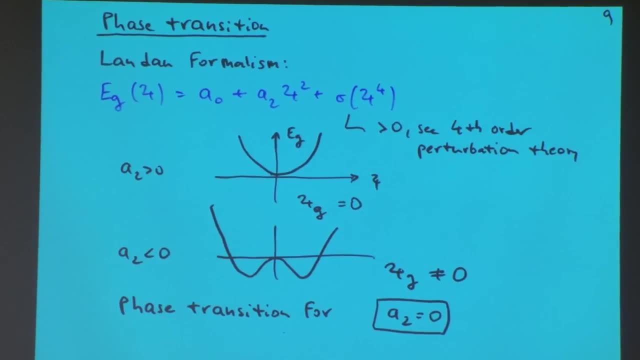 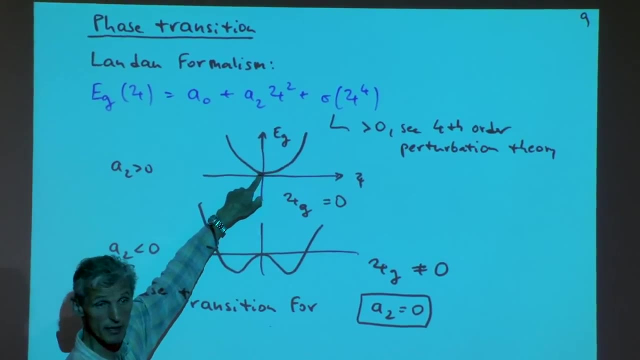 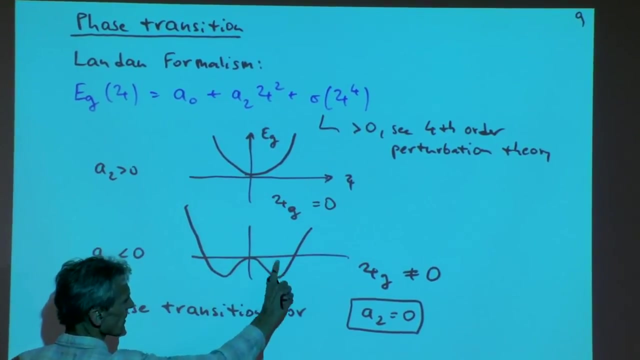 But here the total energy turns into w-shape And the interpretation is fairly simple. Under those conditions the system prefers to have psi equal 0, whereas here it's like the system wants to have a psi parameter which is finite, either positive or negative. 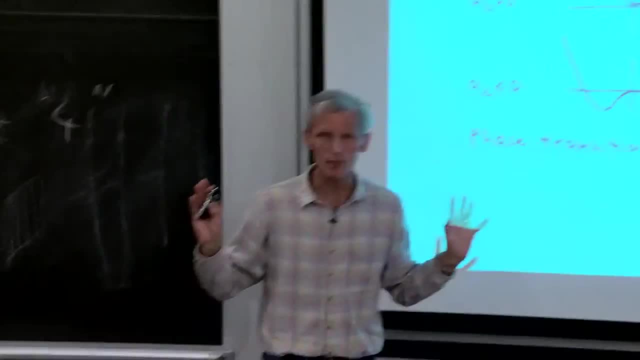 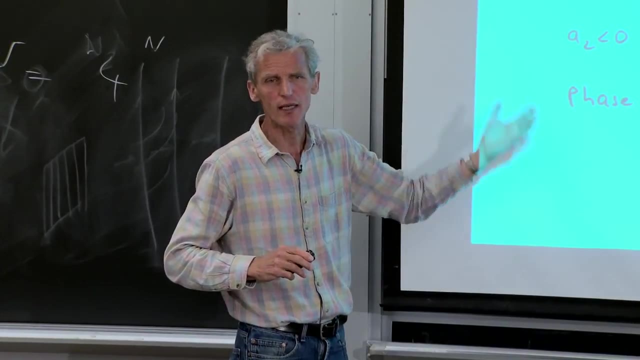 And whether it's positive or negative, it's sometimes called spontaneous symmetry, breaking between two degenerate solutions. What I'm showing here is, of course, very similar to the Ginzburg-Landau theory of phase transitions, where you have an effective potential. 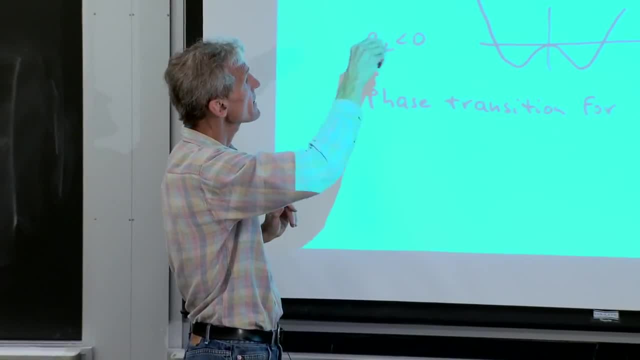 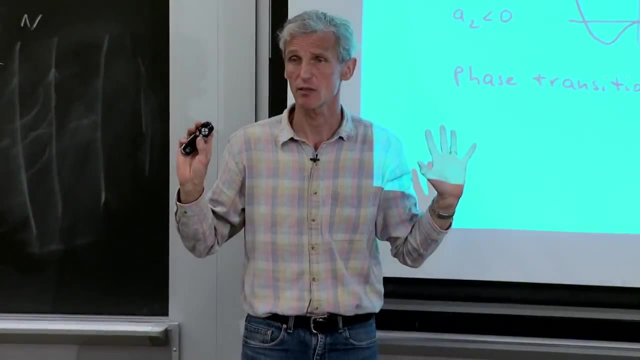 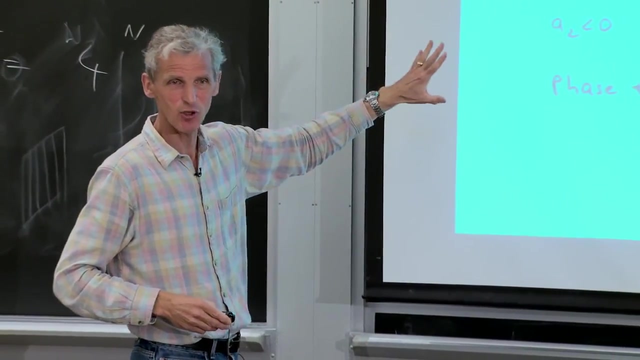 and the phase transition takes place when the second-order coefficient change is sine and the effective potential turns from u-shape into w-shape. So that's what we have done. So anyway, I think this is an example of a nice problem where the interpretation is. 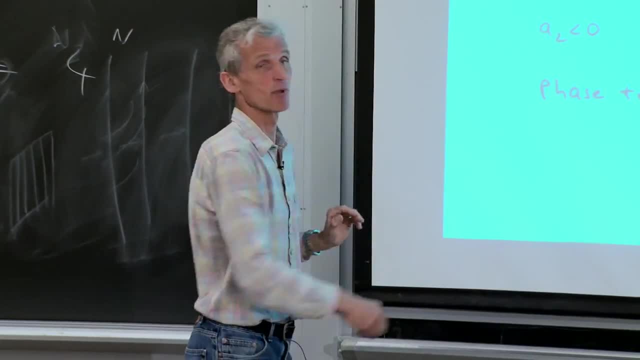 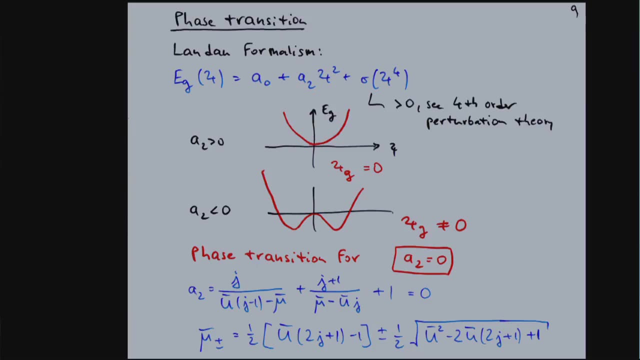 I think, much more subtle than the calculation itself. But we have calculated the phase transition. Everything is analytic. Here is the analytic result, which I know with very indigestible notation. I followed exactly the paper by van der Straaten Stoof. 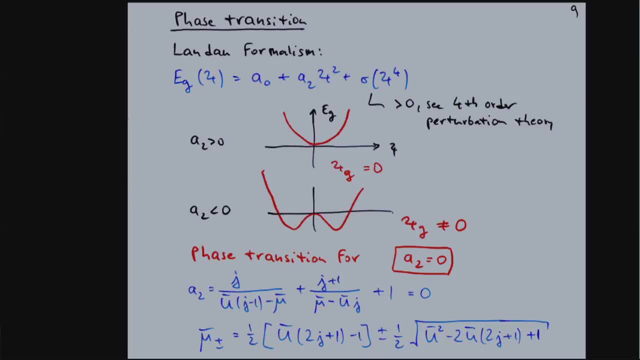 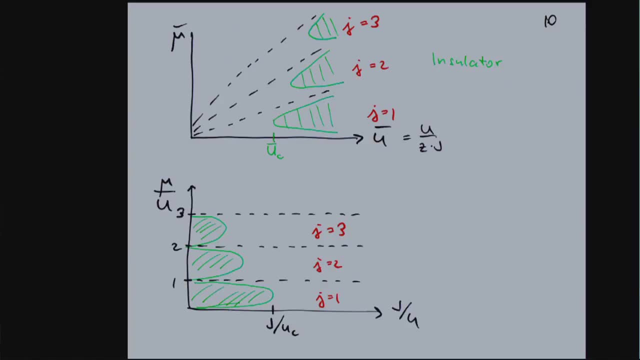 and collaborators, which is posted on the website. You can plot this phase diagram in this way. But if you use, If you use what is more common, normalize the chemical potential by u and normalize j by u- you get these wonderful loops. 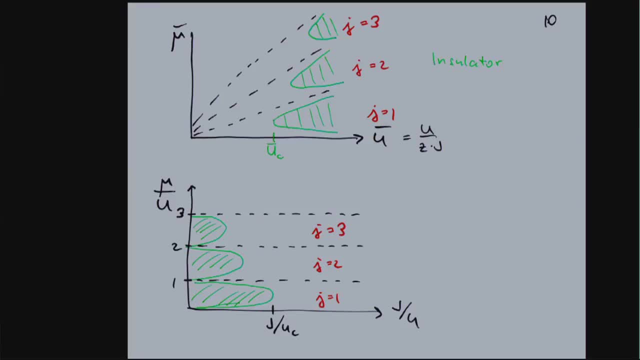 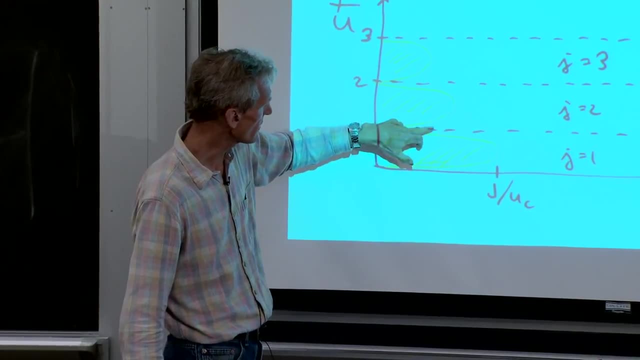 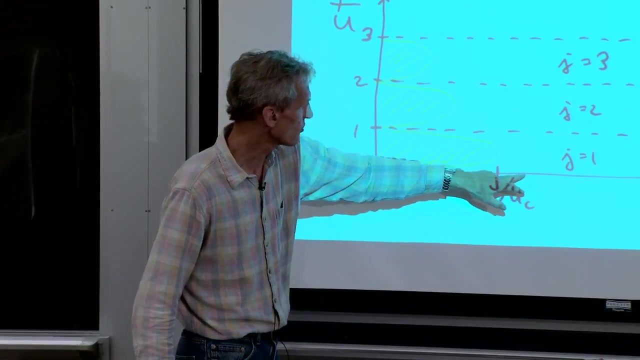 of the modinsulator, where you see that if you increase the chemical potential, you have n equals 1, n equals 2, n equals 3 modinsulator And in between you go through superfluid regions. However, if your tunneling is larger, 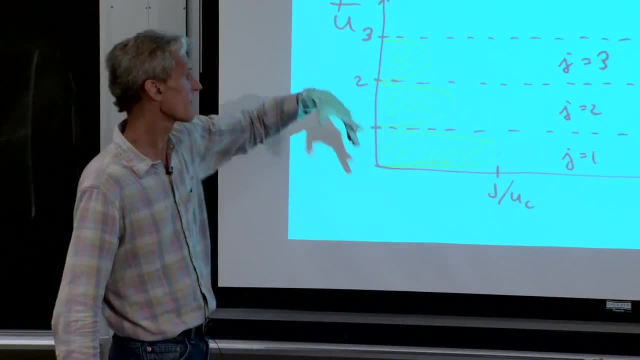 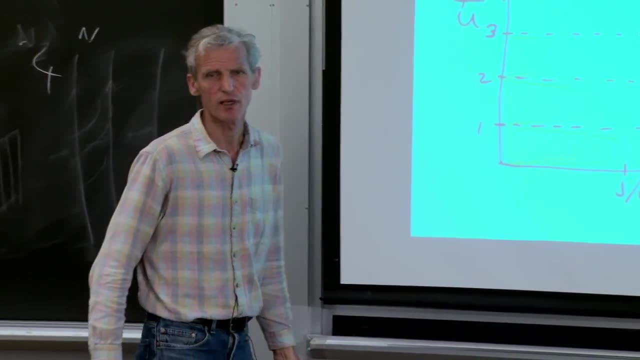 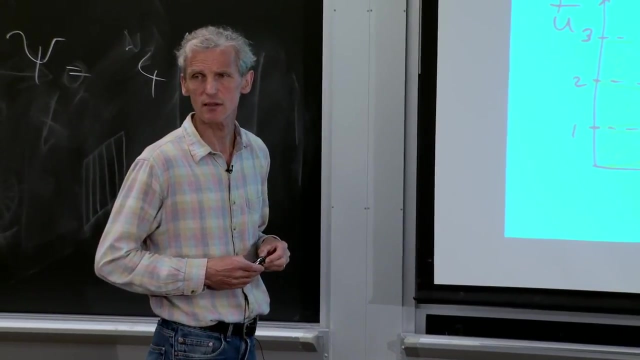 if your tunneling is too large, you're only superfluid. So this is sort of the way how you derive this rather rich phase diagram of bosonic atoms in an optical lattice: Green is an insulating state and white is the superfluid state. 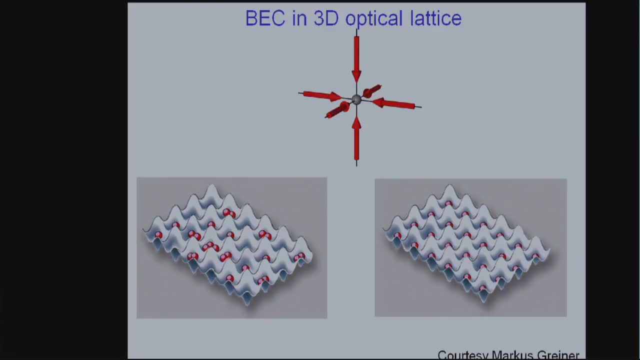 Let me just conclude by showing you a few slides how this can be observed. So in one case we have an insulating state with a definite number of particles per site, And here we have superfluid state which has the normal fluctuations in number. 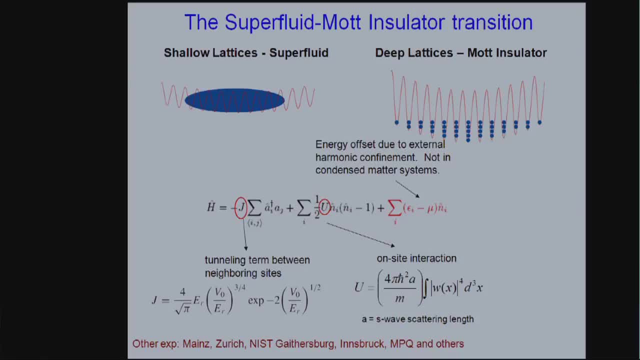 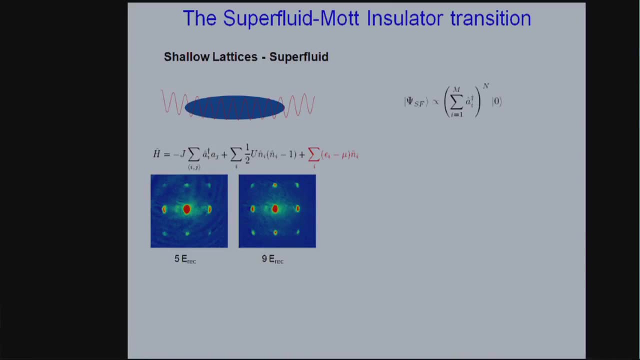 Here's another cartoon picture of a condensate in the lowest Bloch wave function And here you have localized number states. Often you observe the transition by taking the system and releasing it in time of flight into ballistic expansion. If the superfluid is coherent, the wave function. 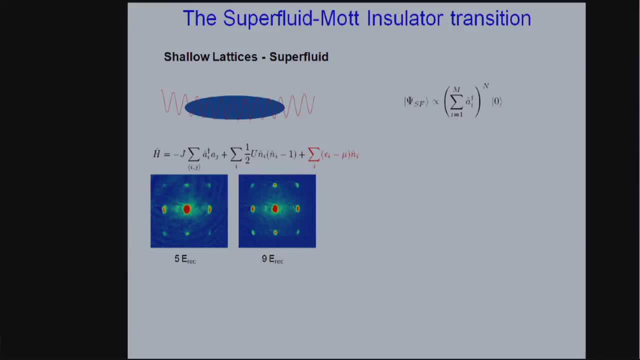 on the different sites is coherent And what you get is a multi-slit interference pattern, which is a diffraction pattern, And you see these characteristic diffraction patterns. It's an n-slit diffraction pattern which characterizes the coherence in the initial state. 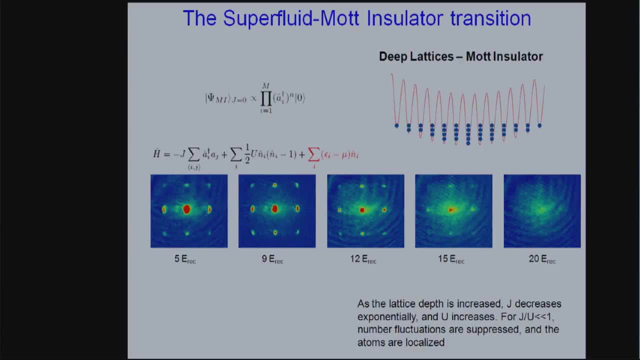 However, if you have a completely isolating state, you have a Gaussian wave packet on each side which has nothing to do with the next neighbor, And then the Gaussian wave function simply expands. It expands in a structure-less way, And so the transition from here to there. 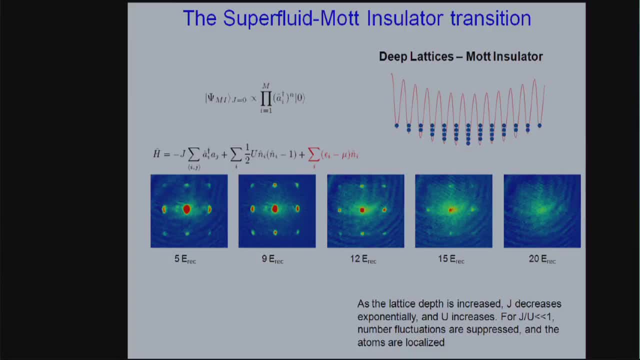 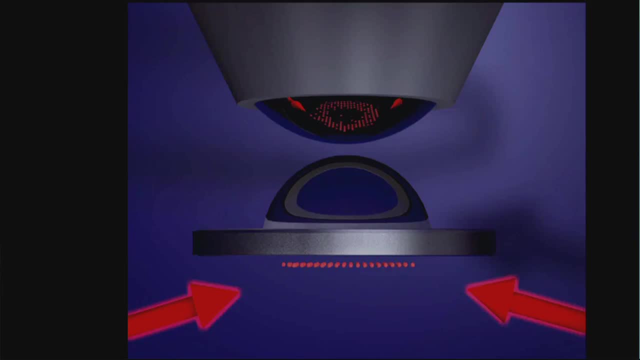 happens exactly when the ratio of u over j crosses the value we have derived. There's another technique of observing that, which is more recent. This is quantum gas microscopes, where you do the same physics in two dimensions, So you have only one plane where this physics takes place. 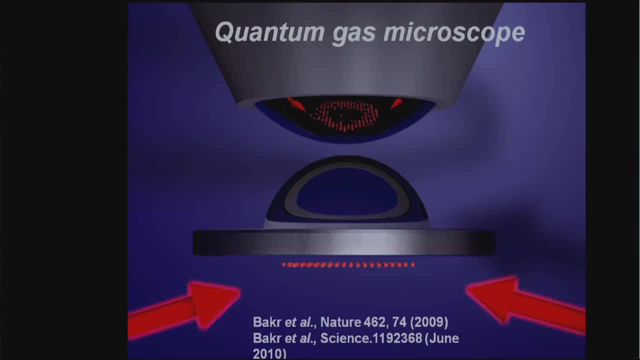 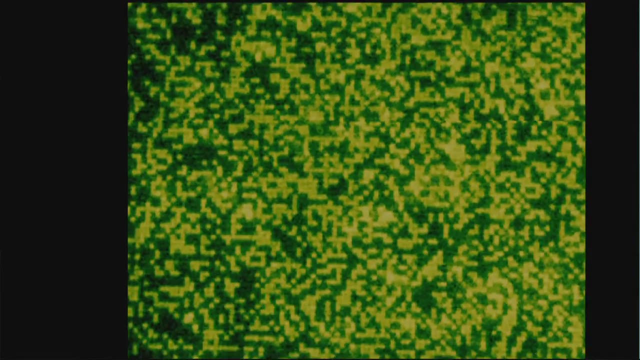 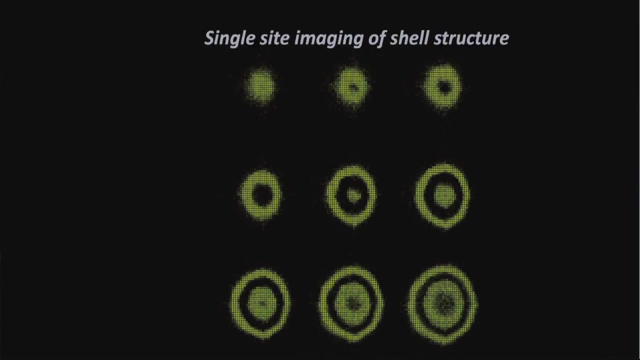 And you can observe atoms. You have atoms now with a microscope, So each green dot here is an atom, If you can sort of zoom in And if you now study the region where you go through the superfluid to the mod insulator. 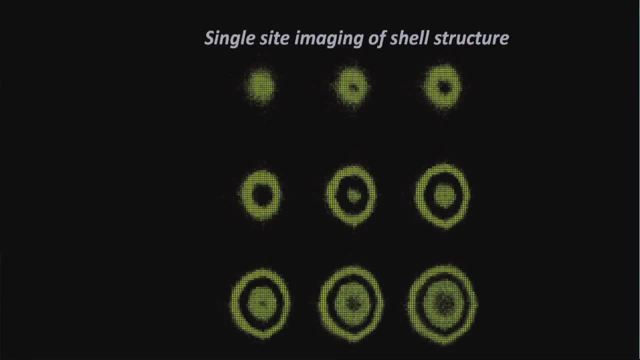 you see that you have exactly one atom per site. If you increase the atom number, you have an insulator with one atom per site And in the middle you have a state with two atoms per site which, for reasons I don't want to discuss, are color-coded here in black.